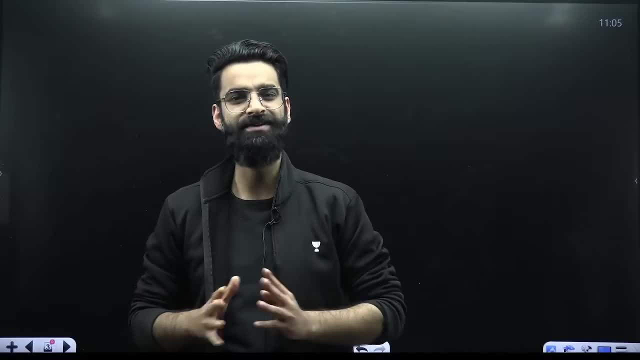 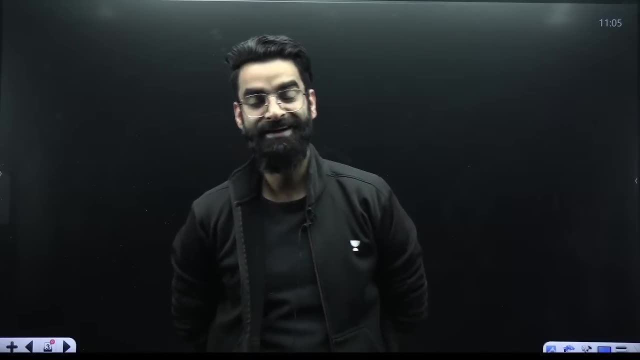 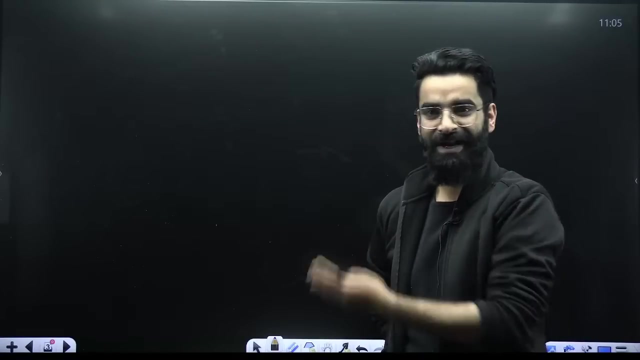 In four to five hours, almost like four or five hundred different types of questions will be covered from the class 11th inorganic part. Right, I know a lot of students are asking about the yesterday's PDF, But, but but let me tell you, you know, due to electricity shutdown, the screen got blank and I could not see. 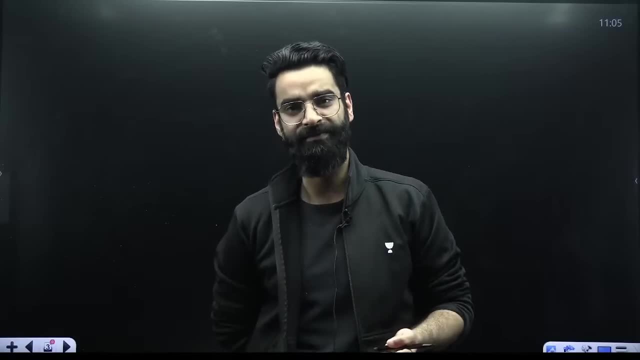 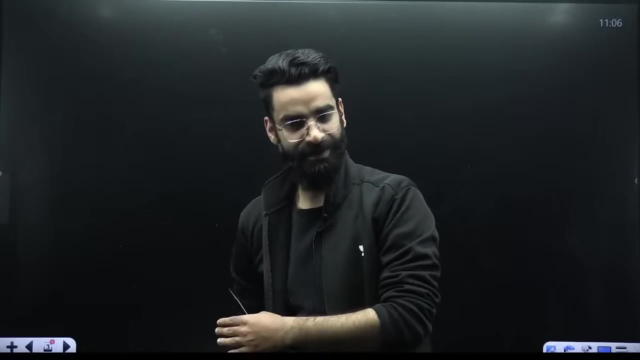 Save the handwritten PDF? Okay, but I'll share the other PDF with you, but that won't be handwritten one, Okay, Okay, Right, It was the technical issue yesterday, so I could not save that handwritten PDF. I hope you get it. 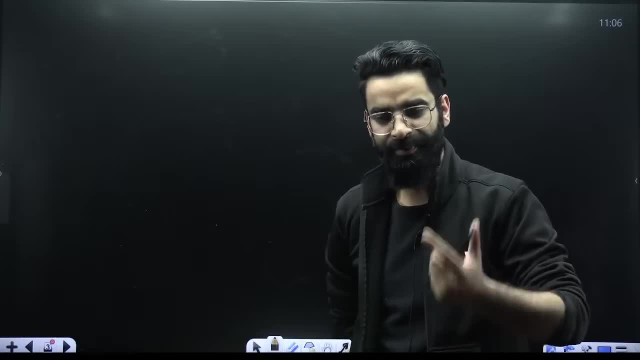 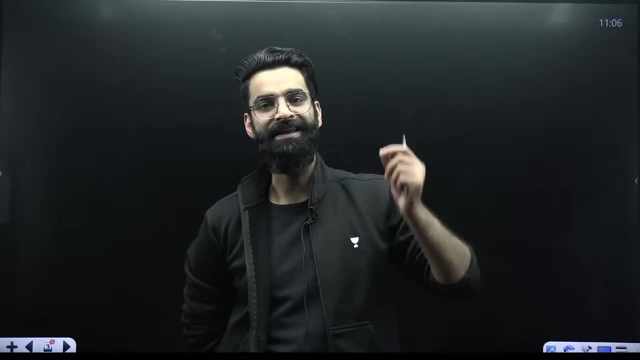 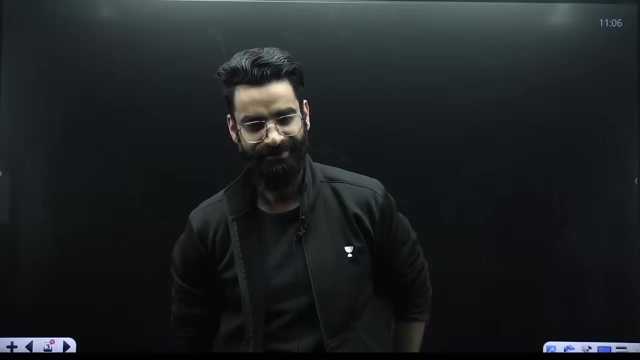 Yeah, I'll share the other PDF with you, but that won't be handwritten. Okay, And one topic which was left in the yesterday's session in the periodic classification. We'll be doing that particular topic in the form of questions directly, right? 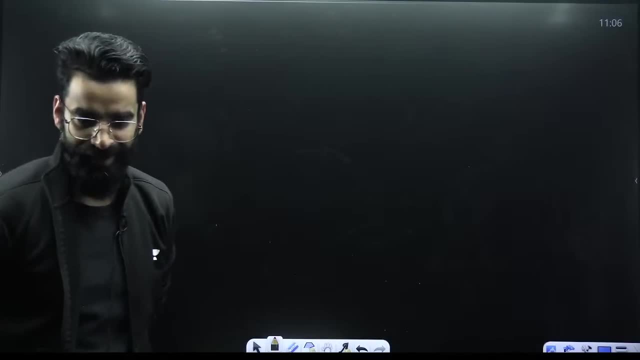 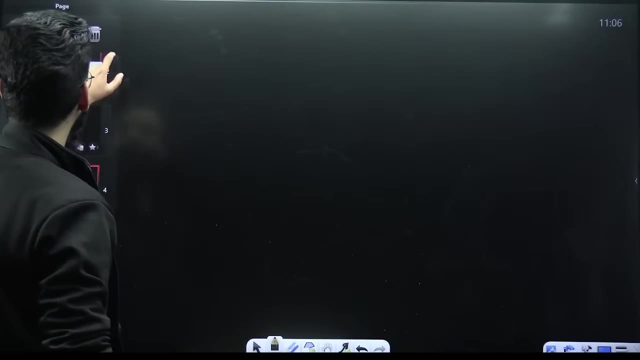 No need to waste any sort of time. Perfect. So which chapter do you want me to start with? Should we start with the chemical bonding questions or period of classification questions? quickly, We have got almost 700 slides over here today. Which chapter should we start with? 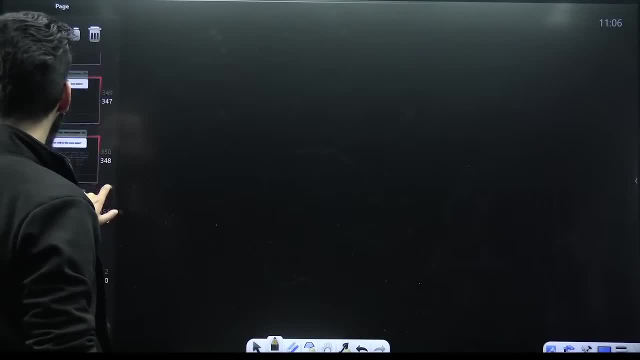 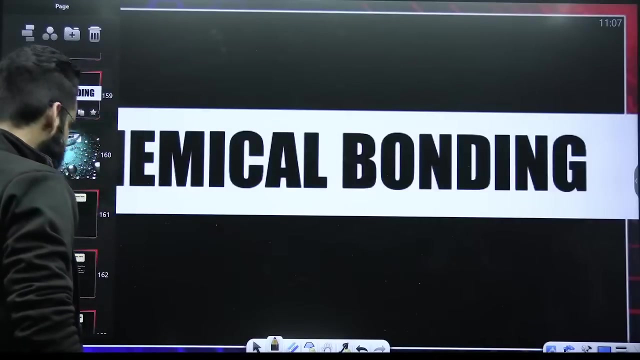 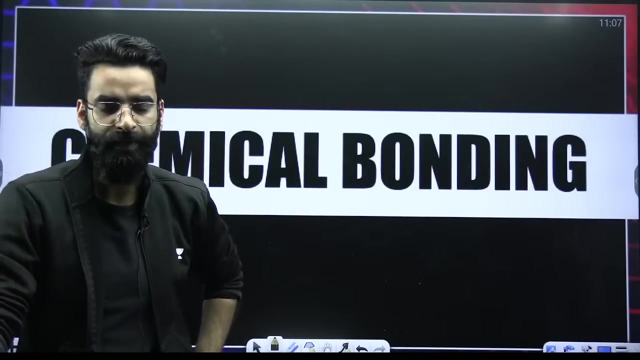 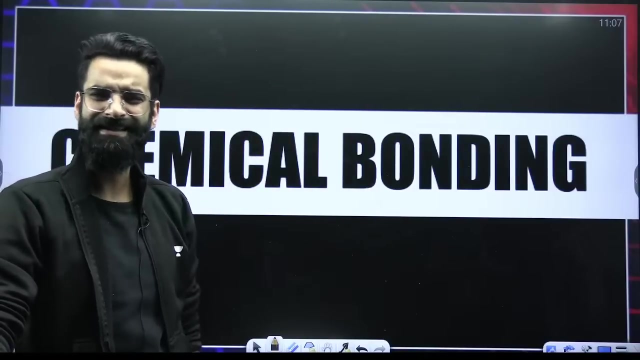 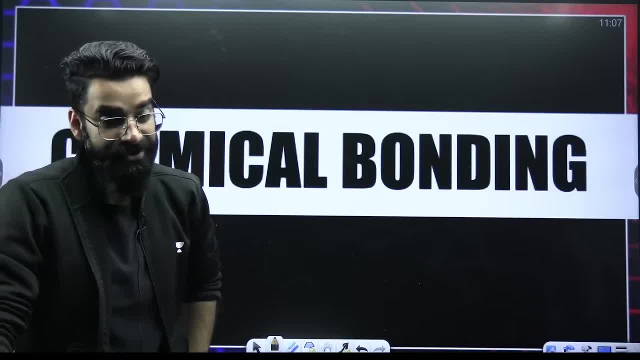 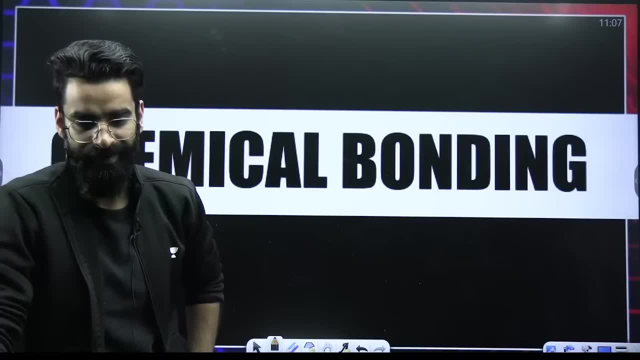 I will come up with. And you guys have to be very active in the chats today because you are the ones who are going to write the answers in the chats And I'm pretty much sure if you have watched yesterday's marathon, you will be able to. 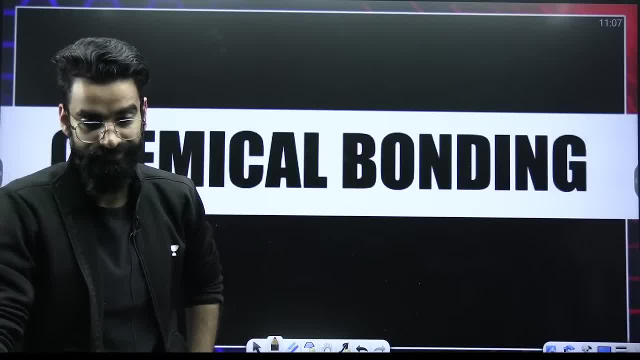 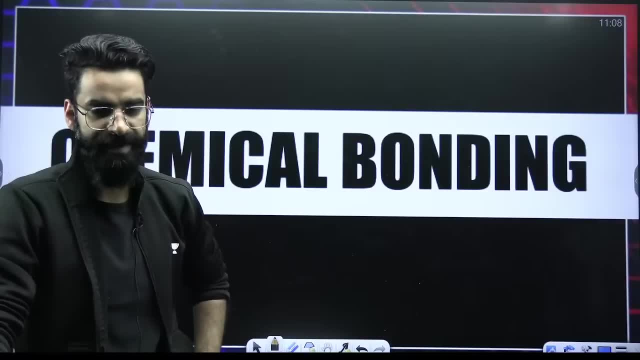 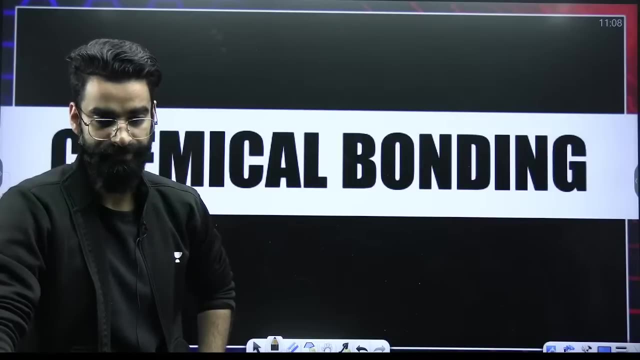 solve each and every question on your own. I'm pretty much sure about that, Yeah, So are you all ready? Are you all ready? people, A P block will be doing in class 12th inorganic marathon. Okay, So, are you all ready? quickly, quickly in the chats. 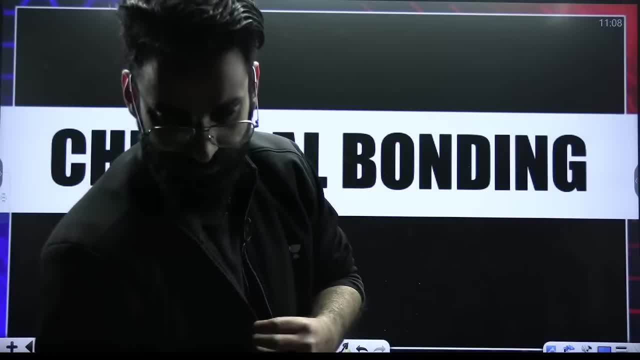 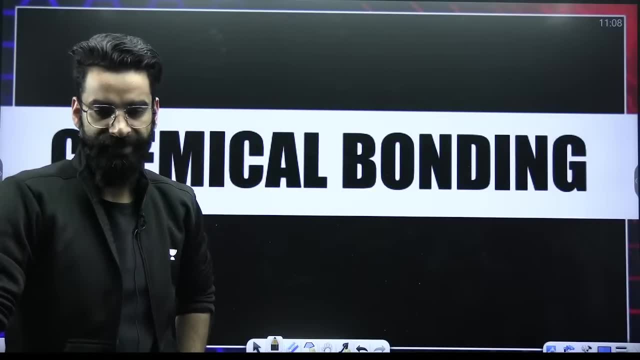 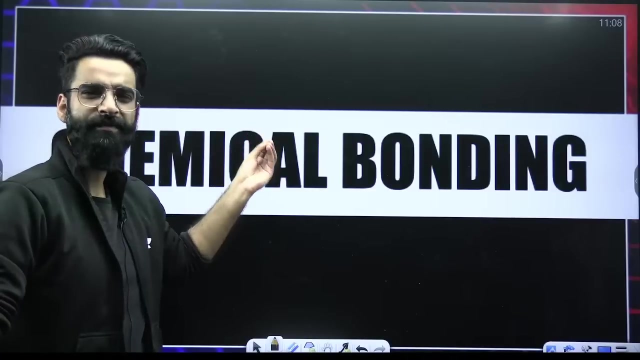 Perfect, perfect, perfect, perfect guys, all right. So I hope you all are ready with your pen and paper, okay, And the first few, like four to five questions will be very easy, which I'll be solving right now. It's very easy. 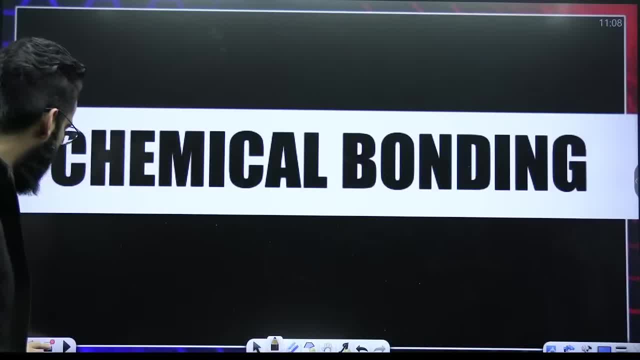 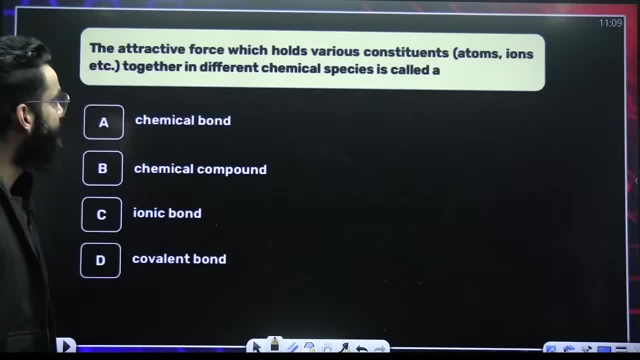 You do not have to use the pen and paper for them right Directly by looking at the questions, you'll be able to answer all of those Quickly. let me know the answer of this particular question quickly: The attractive force. the attractive force which holds the atoms together in a molecule. 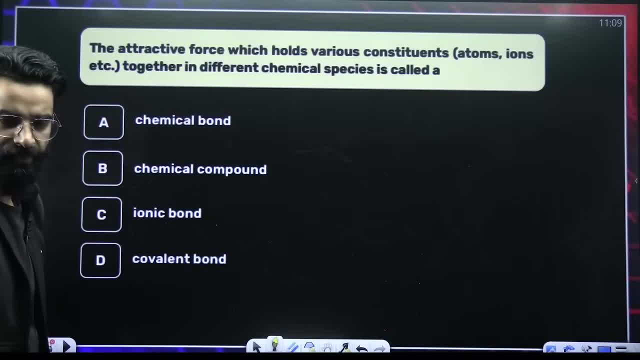 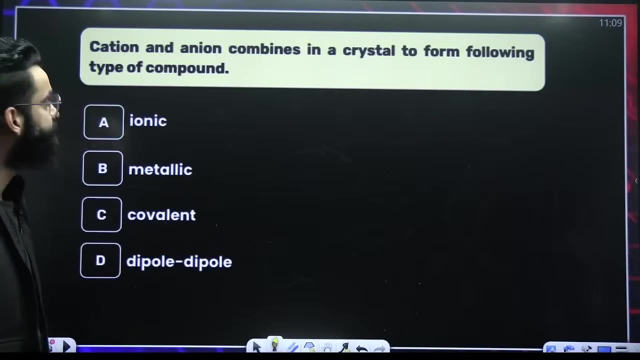 What do we call that attractive force? The attractive force which holds various constituents, atoms, ions, et cetera- together in different chemical species. What do you call that? as You call that as chemical bond done and dusted. Look at the second one: cation and anion. cation and anion combines in the crystal to 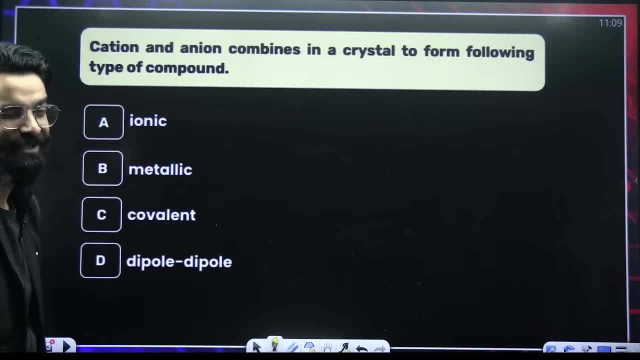 form which of the following compound Quickly, you should be in a position to answer all of these, I'm pretty much sure, In ionic bond. in ionic bond, what happens During the ionic bond formation we saw yesterday? matter loses, electron gets converted to cation. 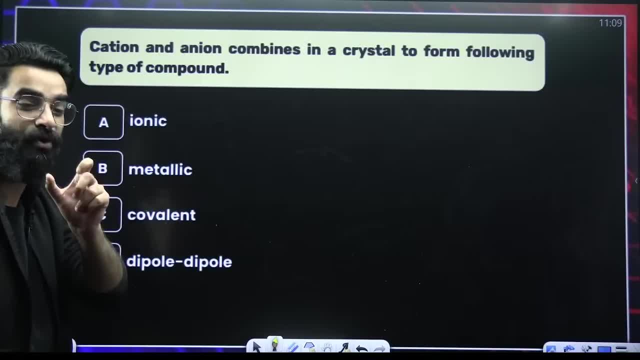 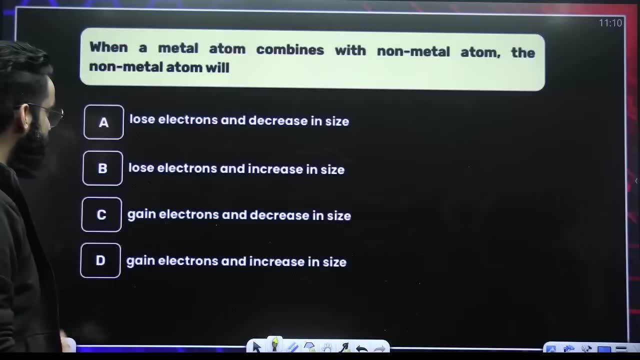 non-metal gains. electron gets converted to anion, then there will be force of attraction between that cation and anion. right, You know it. So it is the ionic one, Perfect. look at the third question. Look at the third question. people kill it. 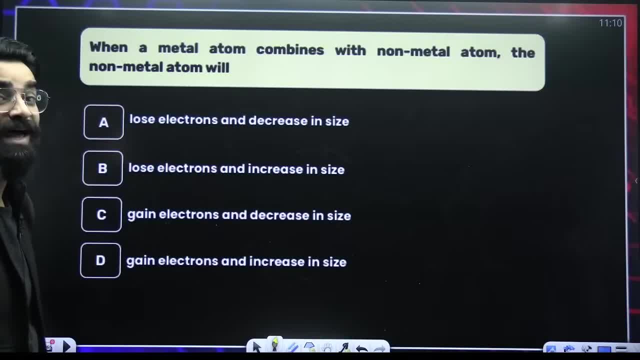 When a metal atom combines with non-metal atom, the non-metal atom, does it lose or gain electron? Non-metal atom gains electron, And if non-metal atom gains electron it's effective nuclear charge will decrease. So there is a force of attraction between the non-metal atom and the cation. So it is the ionic one. It will decrease and it's size will increase. yes, When the non-metal atom gains electron, it's effective nuclear charge will decrease and it's size will increase. So option D: No need to think about anything, right? 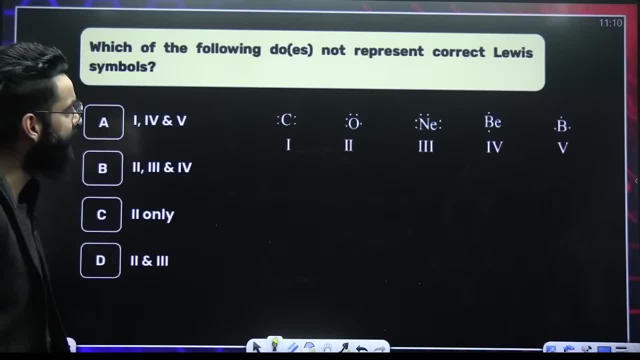 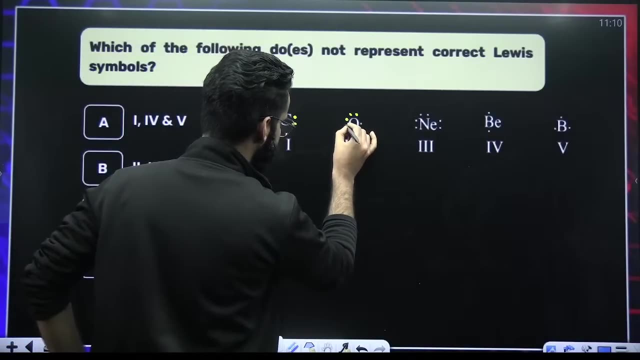 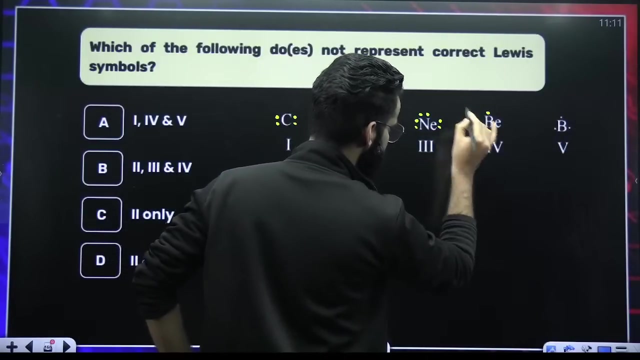 Moving on, Which of the following does not represent the correct Lewis symbols? Which of the following does not correctly represent the correct Lewis symbols: Overhead Carbon- here they have mentioned four electrons. over here, oxygen- they have mentioned five electrons. neon- they have mentioned six electrons. and beryllium- they have mentioned two electrons. 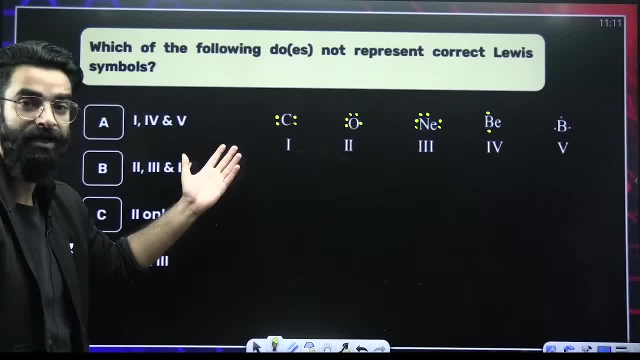 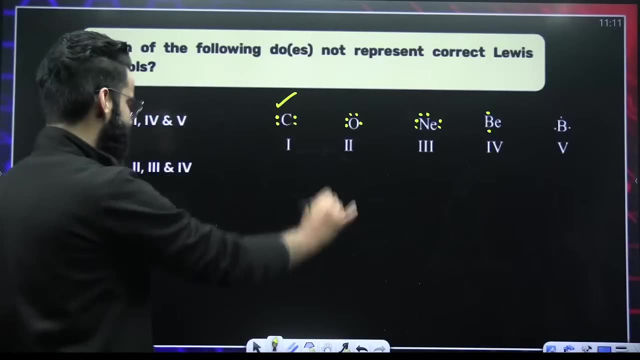 when you show the lewis symbol. when you show the lewis symbol, you need to write the valence electrons, right, you need to show the valence electrons, perfect. so what do you think is the answer? quickly, quickly, people. carbon has got four valence electrons and all the four valence. 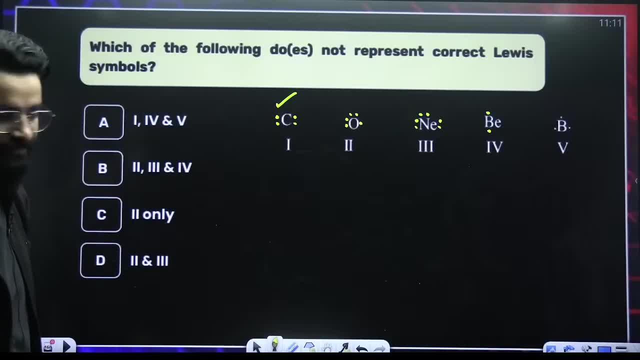 electrons are shown over here. yes, oxygen has got six val valence electrons, but only five have been shown. only five have been shown. only five have been shown. neon, neon. neon has got eight valence electrons, only six have been shown. right, right, rest, everything is fine, i believe. 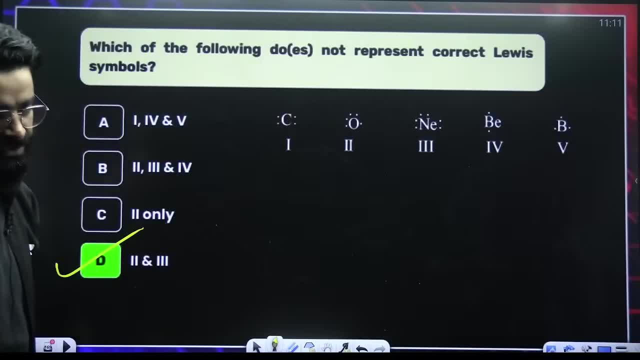 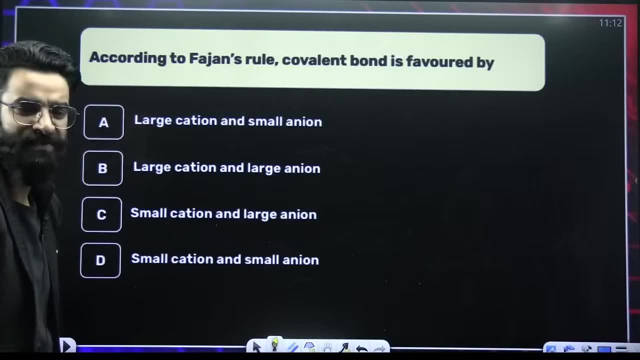 perfect. second and third is the answer of this particular question. you all are absolutely right. i want the answers like this quickly. according to fajan's rule, covalent bond is favored by. according to fajan's rule, covalent bond is favored by. covalent bond is favored by covalent. 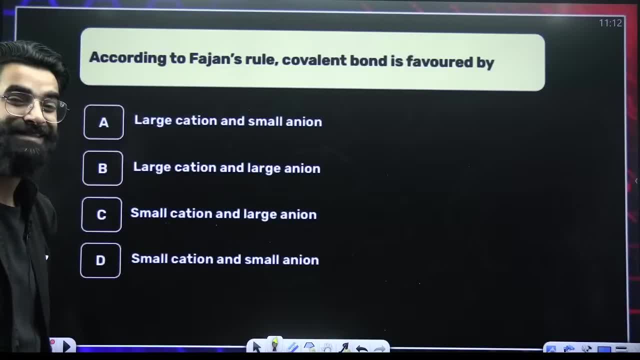 connected in an ionic bond. that is decided by the polarizing power of cation returned. the polarizing part of cation is directly proportional to charge, inversely proportional to size right quickly, quickly, similarly polarizing, similarly coherent corrective is decided by the polarizability of anion as well, and you know, polarizability is directly proportional to. 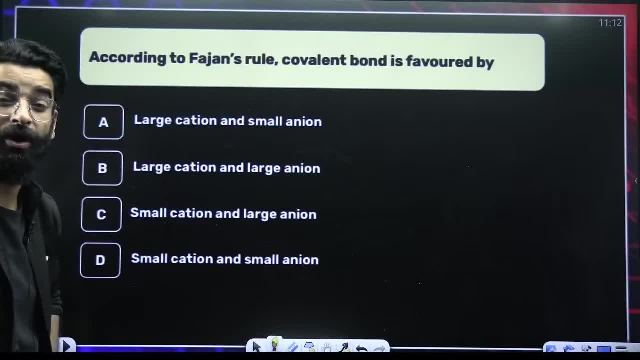 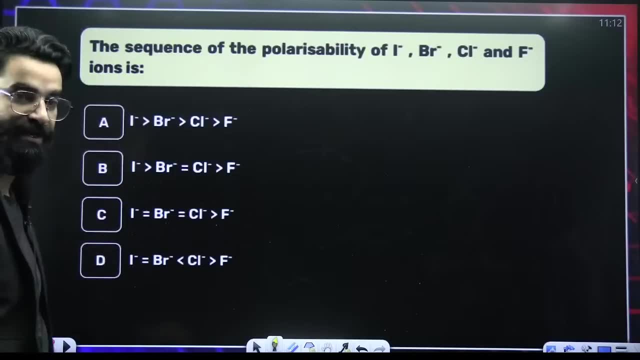 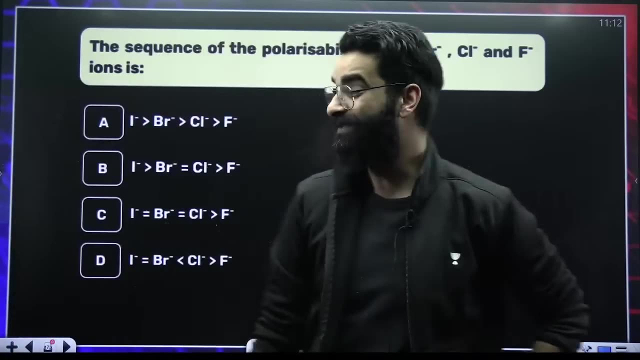 Pajan's rules. covalent bond is favored by smaller cation and larger anion, smaller cation and larger anion, smaller cation and larger anion. This question the sequence of polarizability, the sequence of polarizability of these anions. 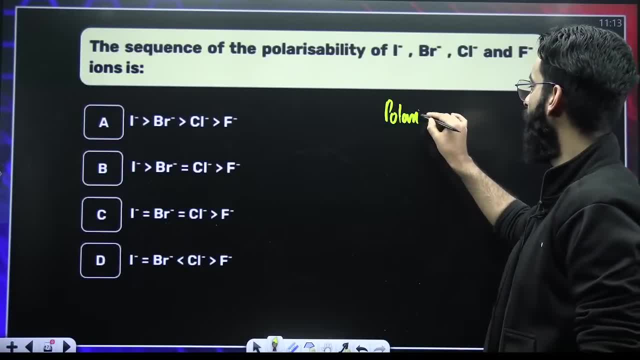 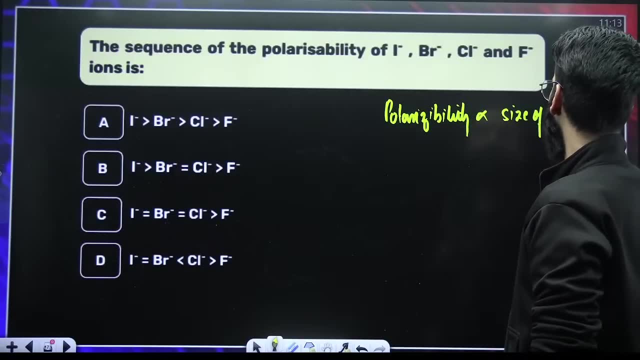 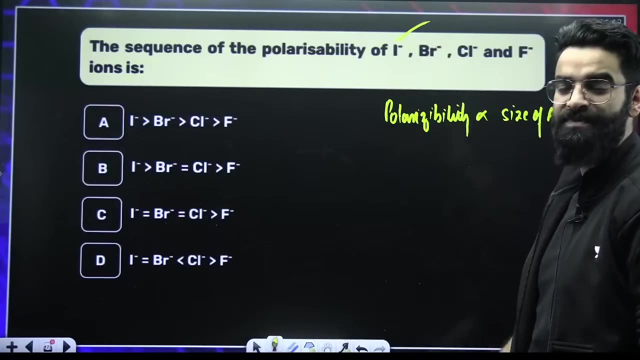 you know, when I talk about polarizability, when I talk about polarizability, that is directly proportional to the size of anion, right, that is directly proportional to the size of anion. Now, you know, among all these anions, I, negative, has got maximum size, so it will show maximum. 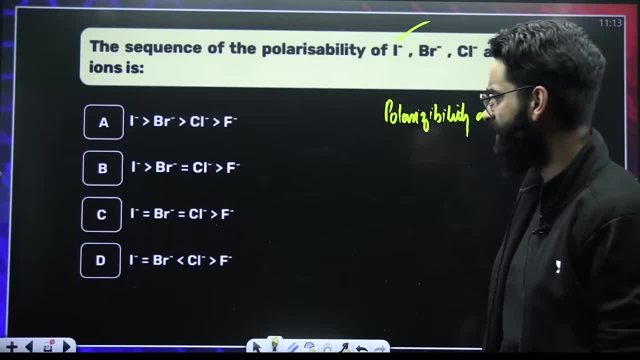 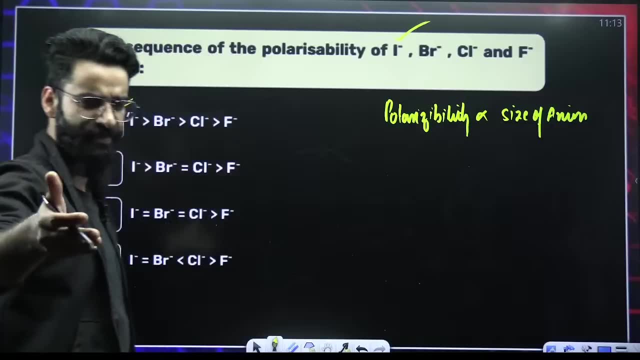 polarizability. Maximum polarizability means it will show maximum covalent character, etc. etc. right, So I negative, Br, negative, Cl negative, F, negative. This is the polarizability order which I believe everyone has written correctly in the charts. 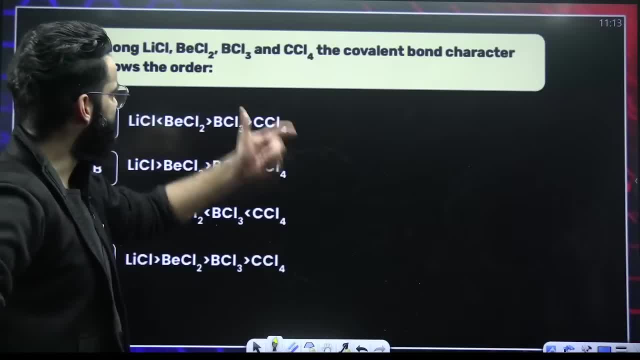 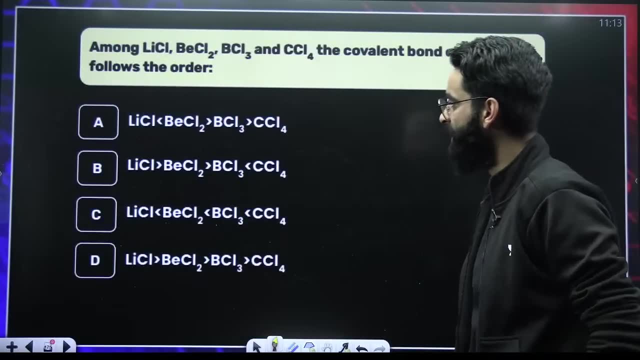 Wonderful Moving on Among these species. the covalent bond Character follows the order, Covalent character order. you have to tell in all these, My dear students, if you look carefully, this is Li positive, this is Be Di positive, this. 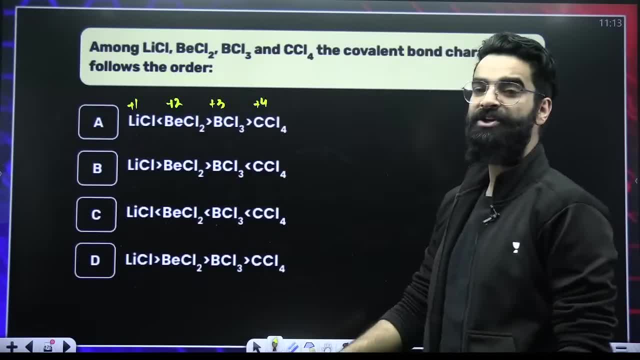 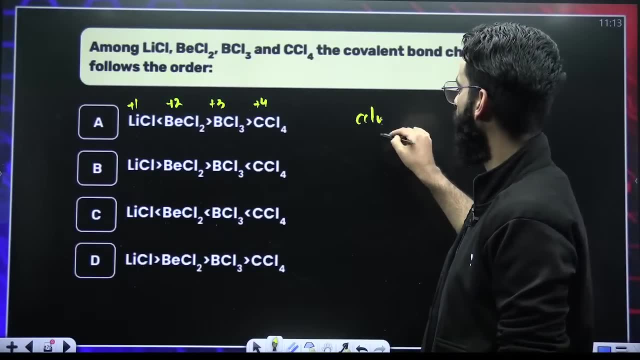 is B Tri positive. this is C plus 4.. More the charge on cation, more the polarizing power, more the covalent character. So covalent character of CCl4 has to be maximum. Covalent character of CCl4 has to be maximum. 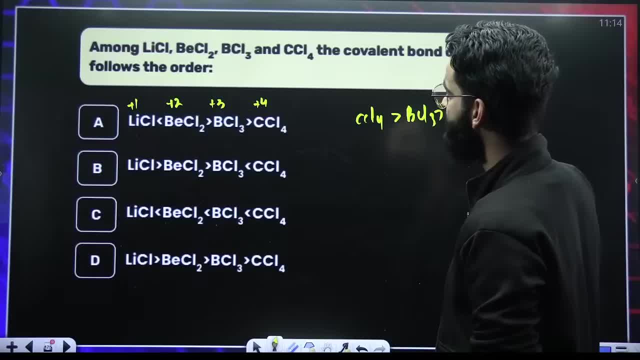 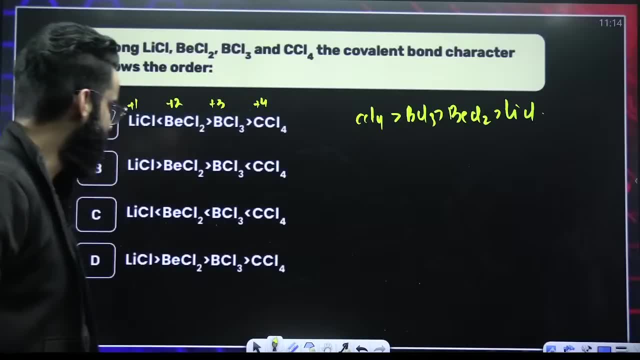 Followed by what Followed by BCl3.. Followed by what Followed by BeCl2.. Followed by what Followed by LiCl Right. Check the answer quickly. Check the answer quickly: CCl4.. 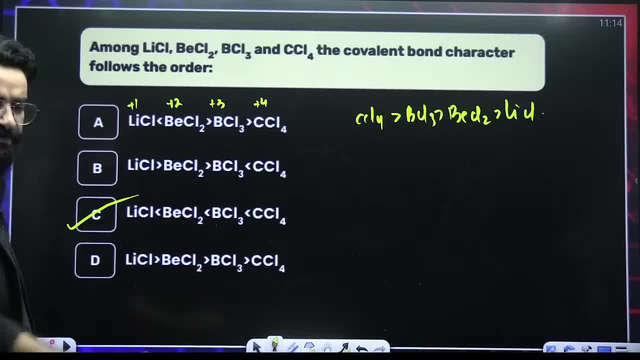 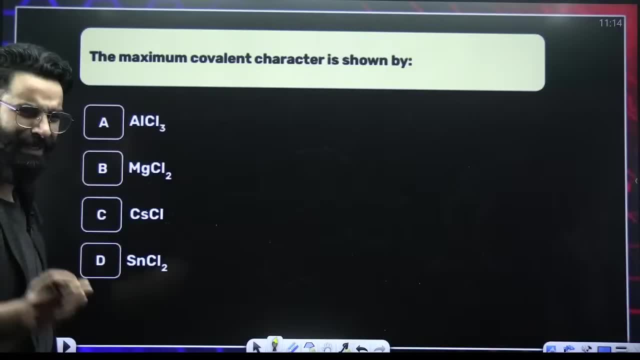 BCl3.. BeCl2.. LiCl. Absolutely, You all are perfectly right. It's option C which is the correct answer of the question. Done and dusted. The maximum covalent character is shown by quickly less than 10 second equation. 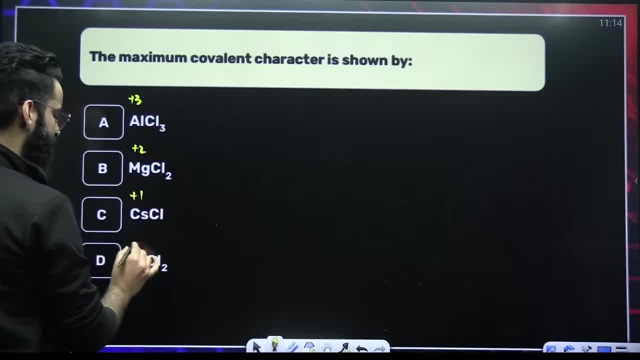 Over here. aluminum is in Tri positive state: Magnesium Di positive, Caesium positive, Sn plus 2. Right: More the charge on cation, more the polarizing power of cation, hence more the covalent character. Right. 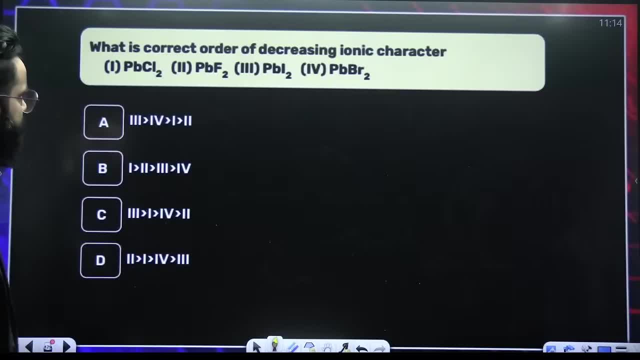 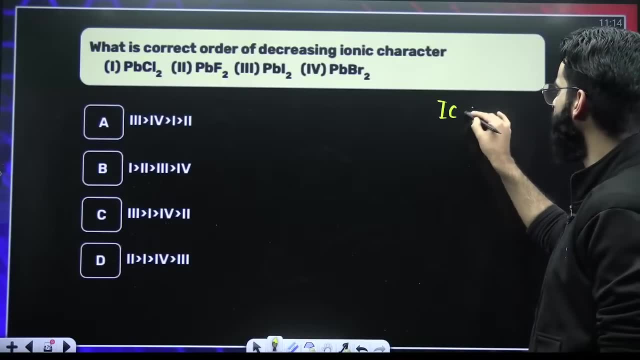 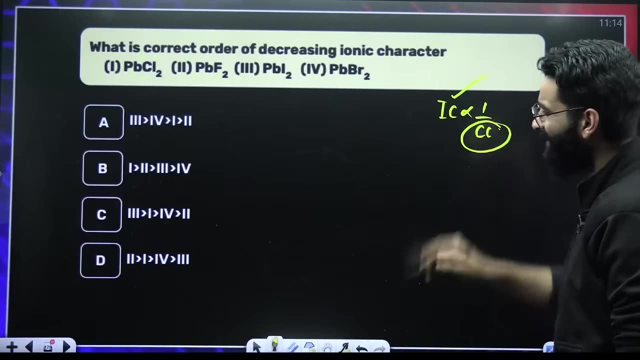 Perfectly done. Look at this particular equation. What is the correct order of decreasing ionic character? Correct order of decreasing ionic character? You know ionic character is inversely proportional to covalent character, Right? So if we get the covalent character order, reverse that order and get the ionic character. 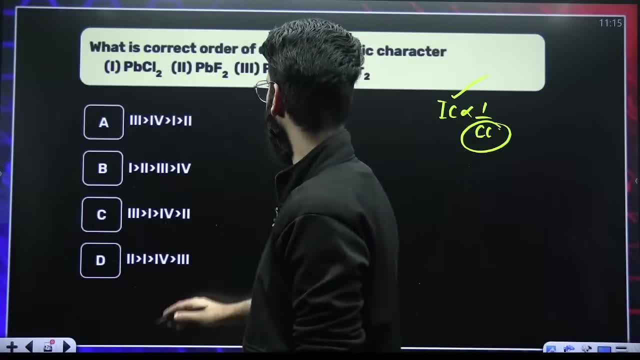 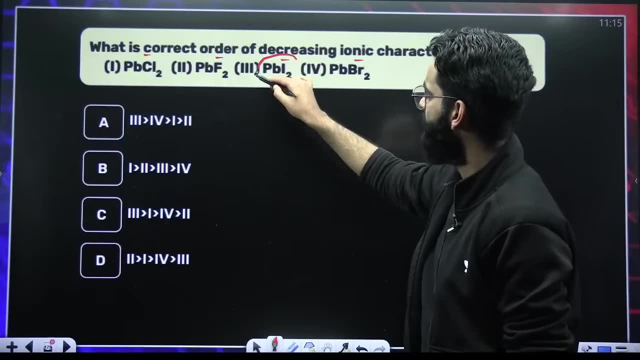 order: Perfect. So, my dear students, look at this particular equation quickly. Over here you have got Cl negative, F negative, I negative, Br negative- Perfect. Which one has got maximum covalent character? This one has got maximum covalent character. 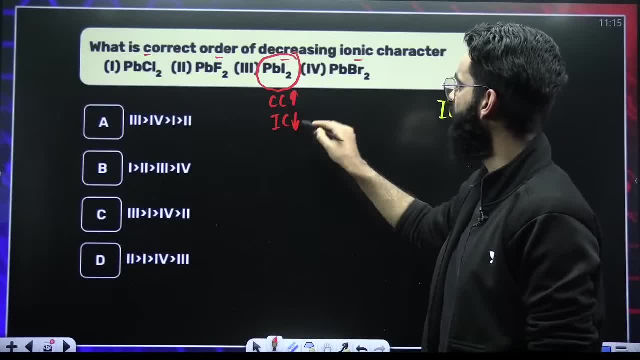 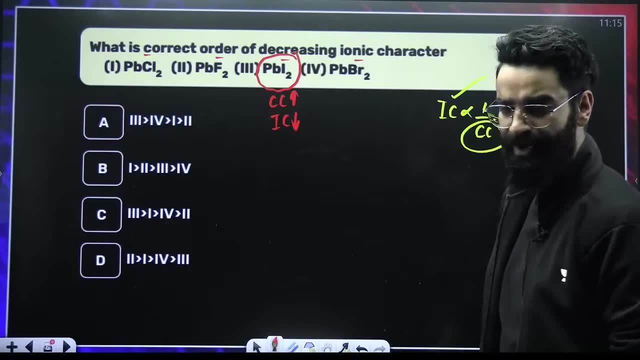 Right, That means it will have minimum ionic character. It will have minimum ionic character. So Pb I2 is the one which has got minimum ionic character. Pb I2.. Third, one is the one which has got minimum ionic character. 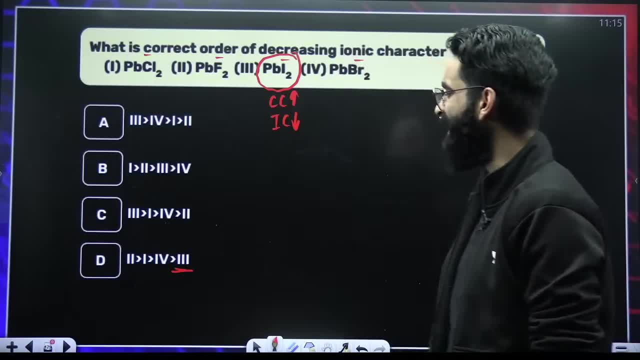 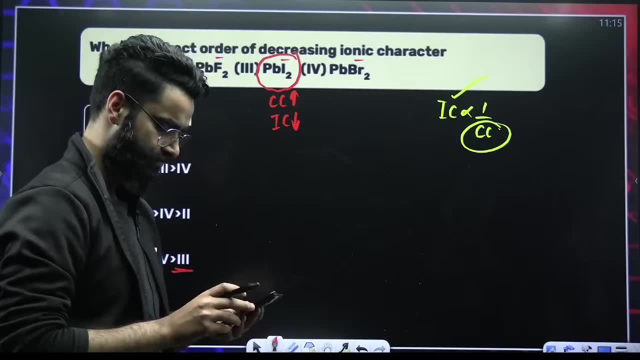 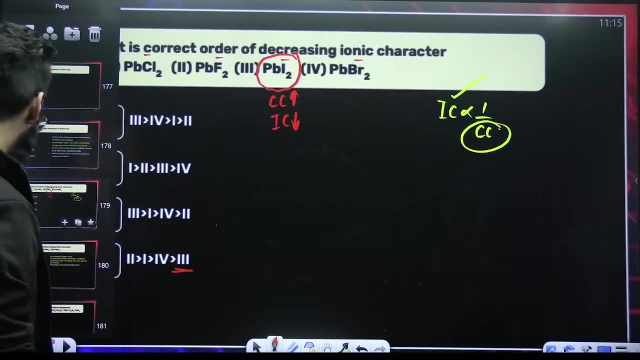 So quickly, Minimum ionic character. Quickly, It is option D, which is saying that third one has got minimum ionic character. Am I clear? Am I clear? Am I clear? Quick, Yes, absolutely, guys. absolutely. going on to one more, they're like the most ionic and most. 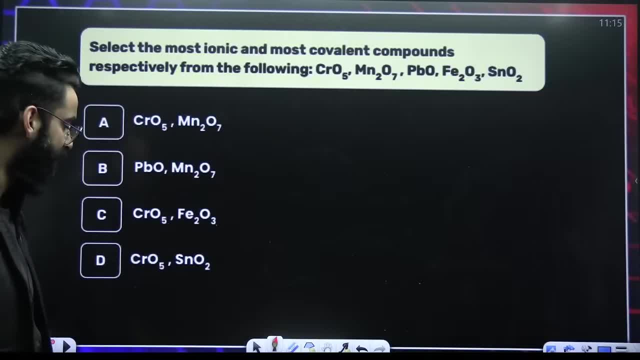 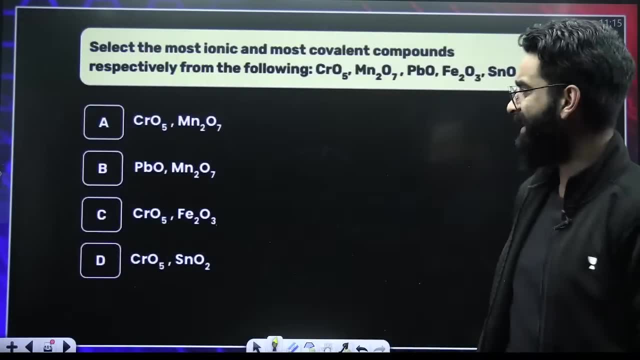 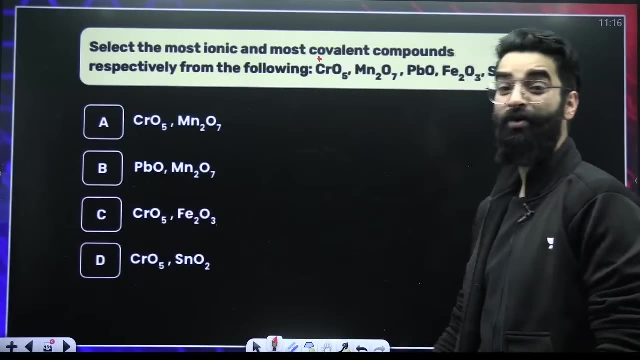 colon compounds, telling the most ionic and most colon compounds. select the most ionic and most colon compounds. let's select the most colon first. if you look carefully, if you look carefully, chromium oxidation state here in CRO 5 and let me know that oxidation state of chromium in CRO 5. 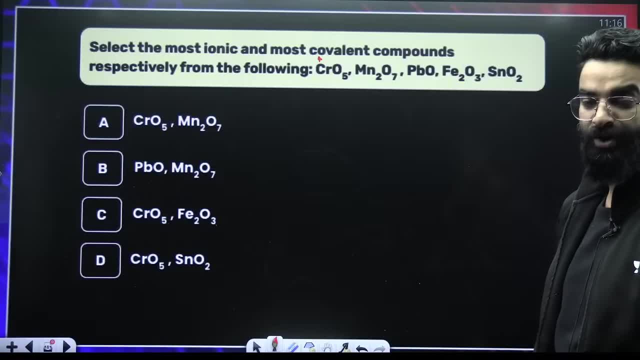 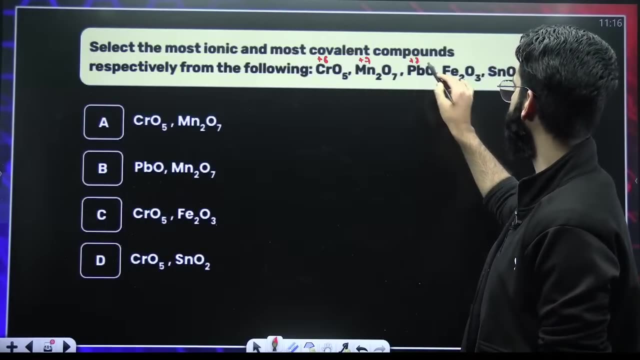 quickly what is the oxidation state of chromium in CRO 5, that butterfly structure, if you remember what is it? absolutely, it's plus six. manganese: here will be plus seven. lead will be in plus two. iron: here is in plus three. in will be in plus four, perfect. so. 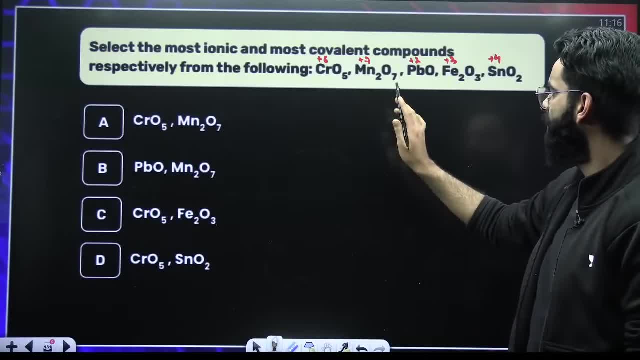 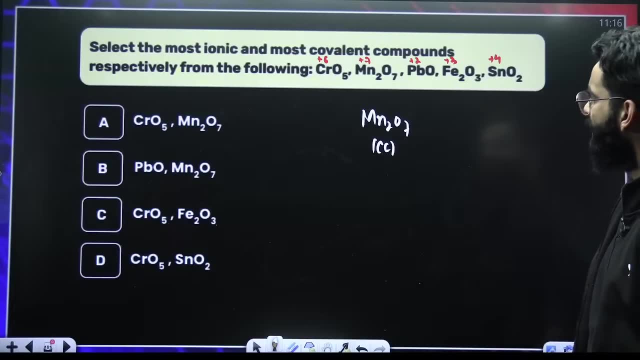 which one is the most covalent? more the charge on cation, more the colon collector, so mn207 is most covalent, most covalent right now. which one is most ionic? most ionic means least ionic. sorry, most ionic means least covalent. which one is least? which one is the least covalent among all? 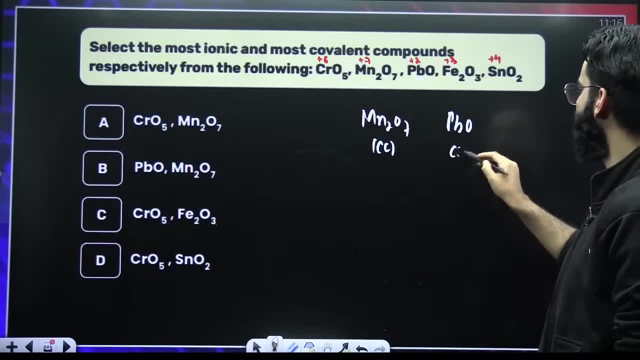 least covalent will be pbo. this is least covalent. maximum covalent- least covalent. that means this is minimum ionic, this is most ionic. the answer is going to be pbo- mn- o207, pbo- mn207. right option b is the one which is correct. 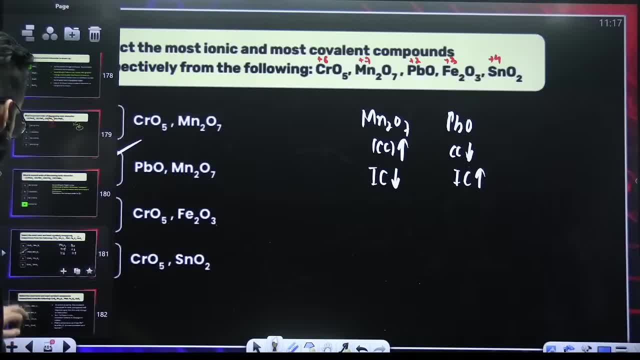 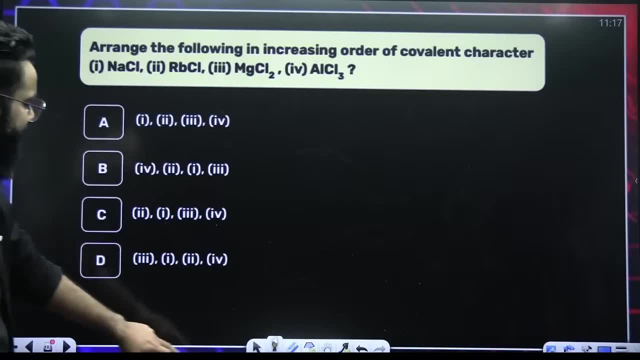 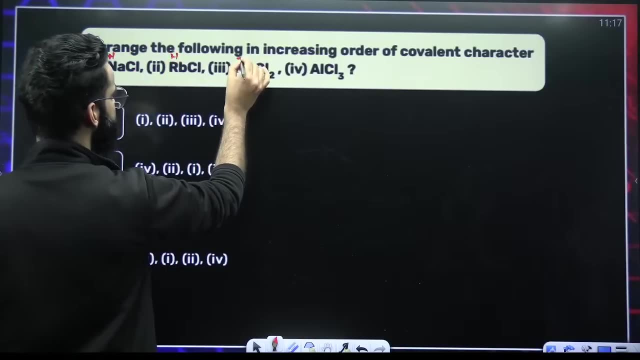 the answer is: what option b is the one which is correct? all of you are perfectly right, perfect right guys. good job, tell me the answer of this question. increasing order of colon character quickly increasing order of covalent character, people. increasing order of coal and character. this is na positive, this is rb positive, this is mg. 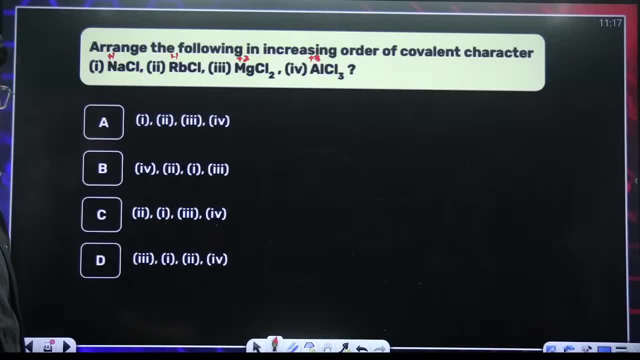 positive. this is Al tri positive correct. more the charge on cation, more the polarizing power of cation, more the covalent character. now which one has got maximum 지금 cation? now which one has got maximum covalent character? I believe it is the fourth one which has got maximum covalent corrector. 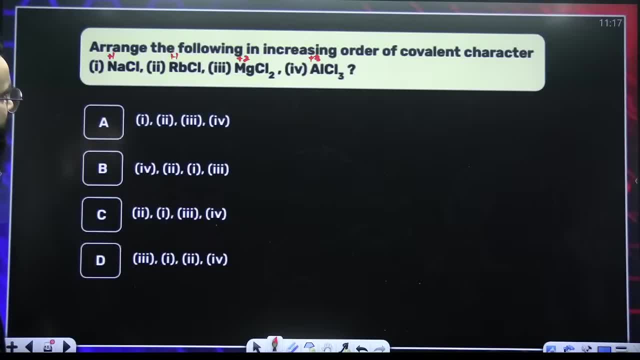 We have to write them in increasing order of covalent corrector right. So what has to be the answer? This is the maximum covalent and this is maximum covalent. maximum covalent right, Maximum covalent. 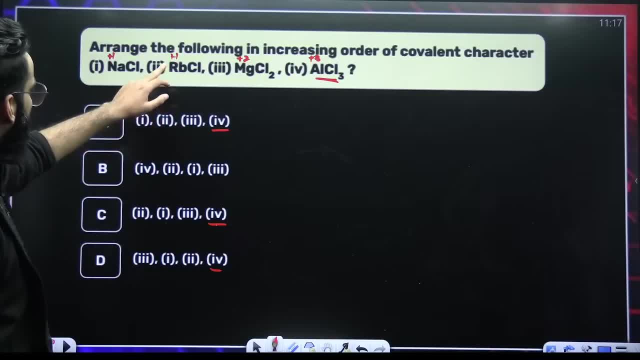 Now, which one is minimum covalent? Which one is minimum covalent? Charge on these two is same. charge on these two is same right, Talk about size: More the size less the polarizing power, lesser the covalent. 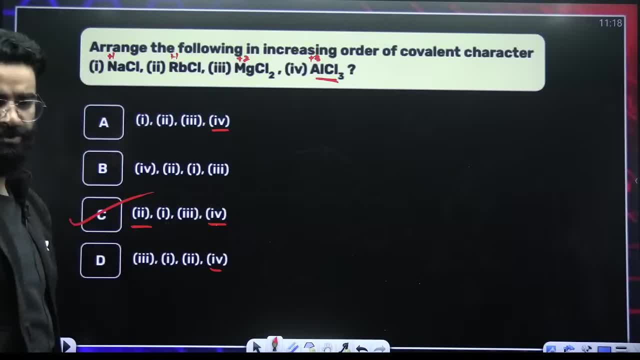 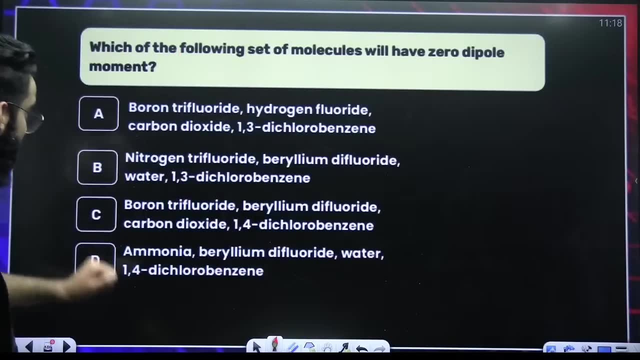 So second has got this one. So it's option C which is correct answer of this question, which everyone has written over here. Great job done. Which of the following set of molecules have zero dipole moment? Which of the following set of molecules have got zero dipole moment? 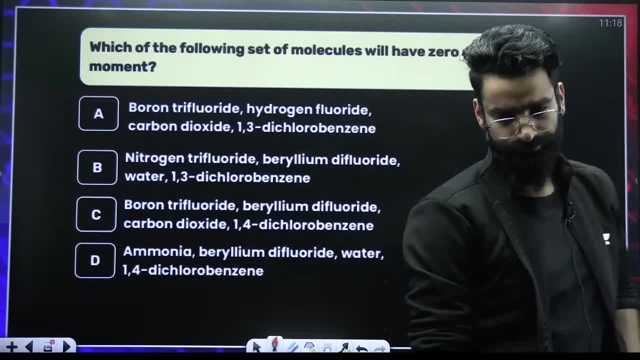 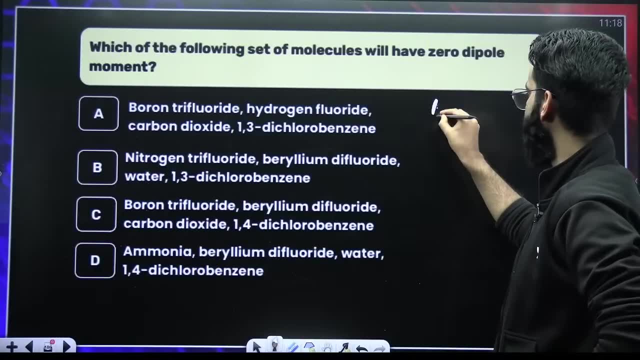 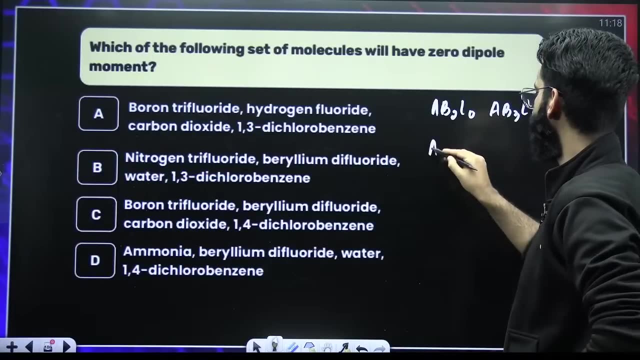 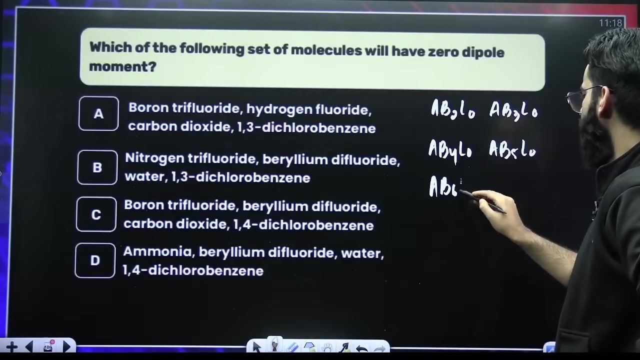 Quickly, Quickly, guys, everyone, zero dipole moment. quickly, I've told you yesterday, if you remember, AB2L0, AB3L0,, AB4L0, AB5L0, AB6L0,, AB4L2,, AB2L3.. 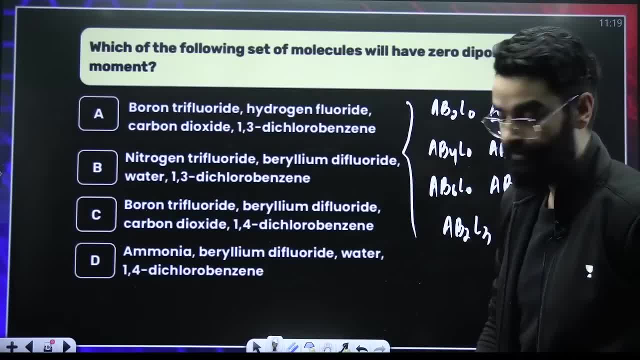 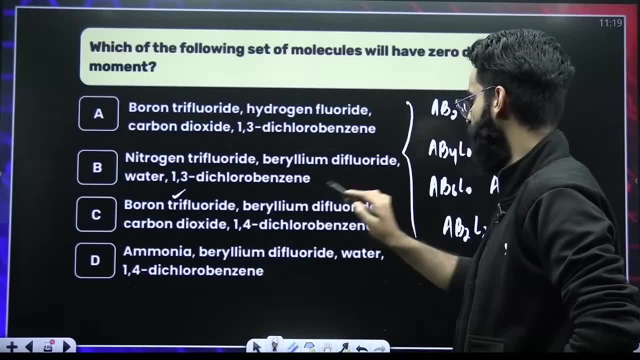 All these species. what do they show? They show zero net. dipole moment right: BF3.. BF3.. AB3L0.. BEF2.. BEF2.. AB2L0.. Carbon dioxide- AB2L0.. 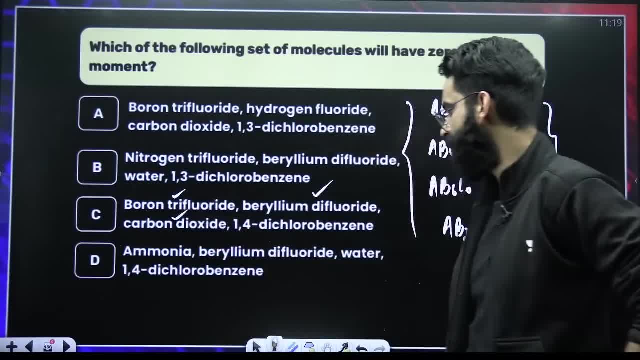 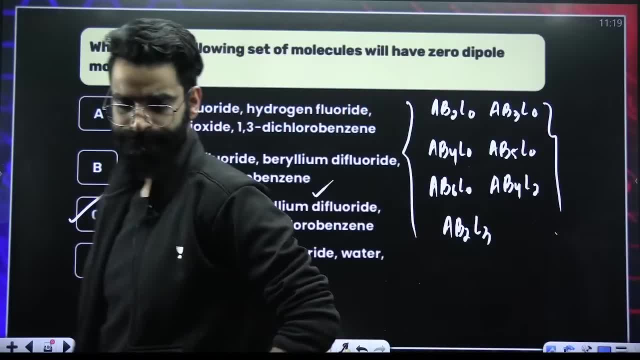 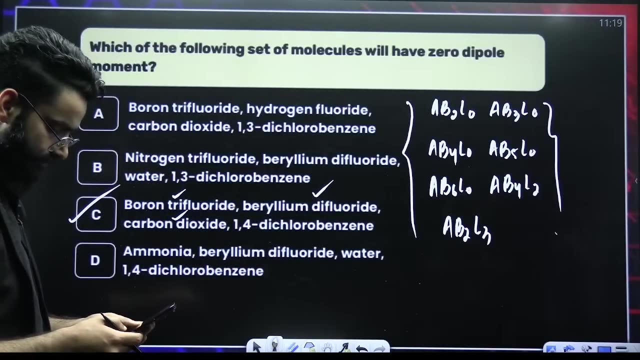 And 1,4-dichlorobenzene. it already has zero dipole moment, so it's option C which is the correct answer of this particular question. I believe it's clear. I believe it's clear. Yes, Right people. 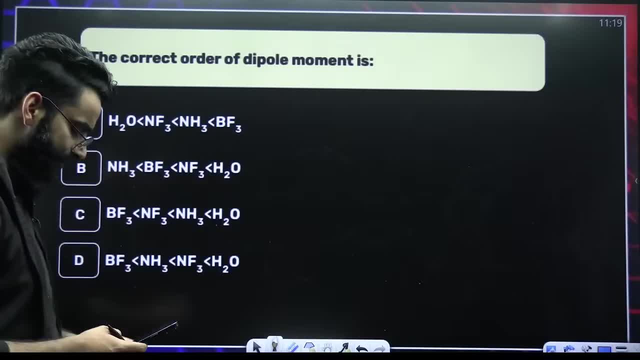 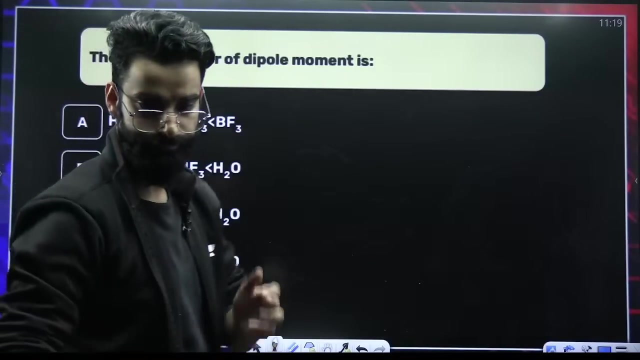 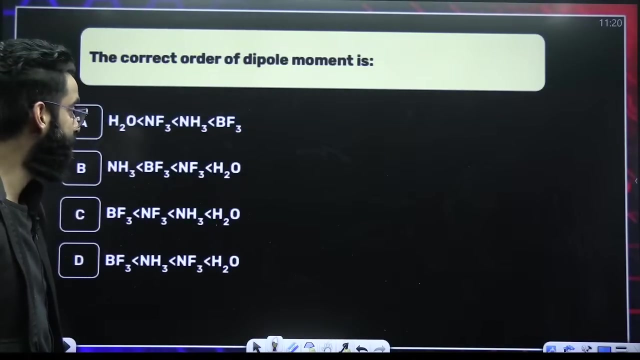 Tell me now, Yes, Tell me the answer of this question quickly, quickly, quickly, Quickly, guys. the order of dipole moment. what do you think is going to be the order of dipole moment? See, first of all, if you look carefully, if you look carefully, BF3 has got zero dipole. 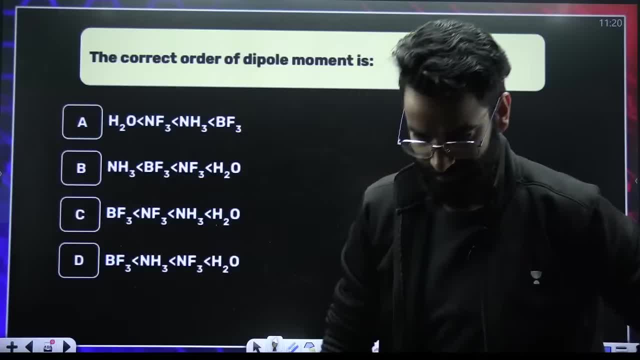 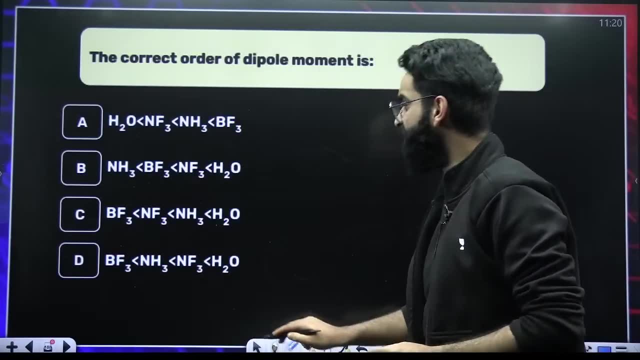 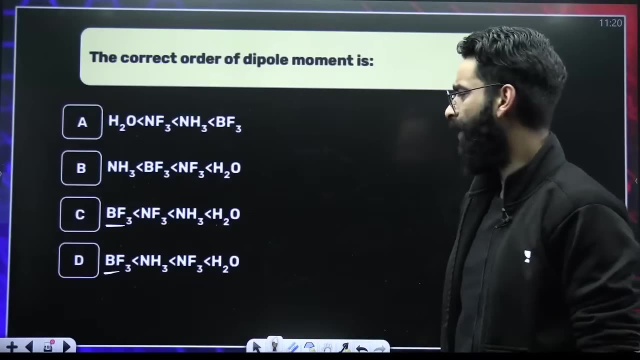 moment. right, Wait, wait. If you look carefully, BF3 has got zero dipole moment. We have to write the increasing order right. Increasing order: BF3 has got minimum dipole moment. Perfect Now among NF3 and NH3, which one has got more dipole moment? 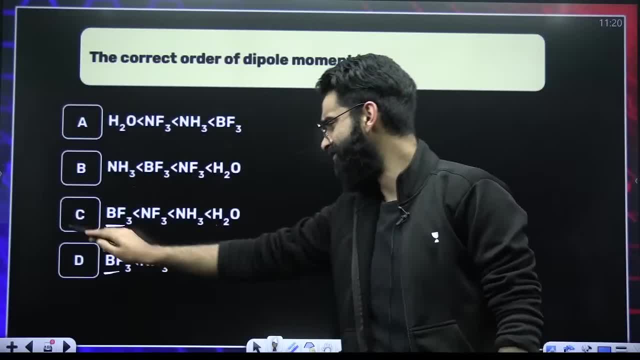 NH3 has got more dipole moment than NF3.. We have discussed that. It's directly option C. Okay, Yeah, Directly option C. We have done it yesterday, if you remember. Tell me A neutral molecule, XF3, has a zero dipole moment. 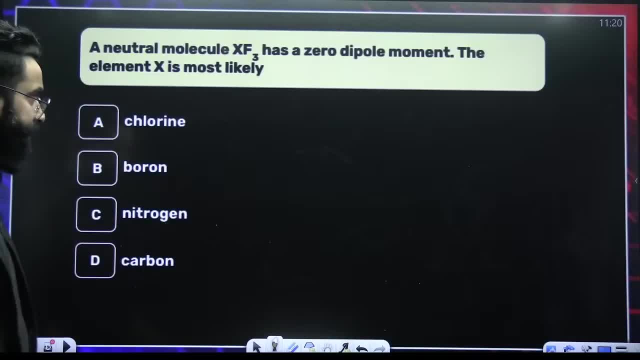 The element X is most likely Quickly Neutral. molecule XF3 has zero dipole. moment XF3.. That means it has to be BF3, right, It has to be BF3.. Perfect, It has to be BF3.. Guys, I want you guys to be active in the chats. 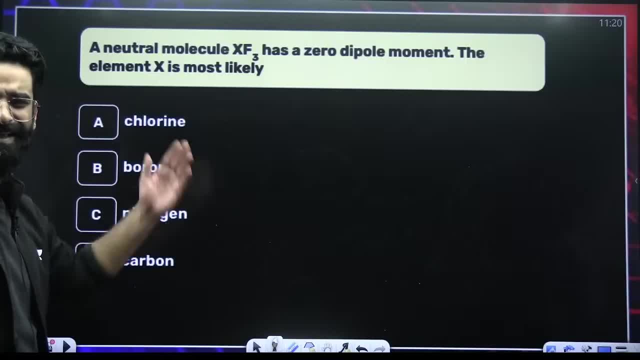 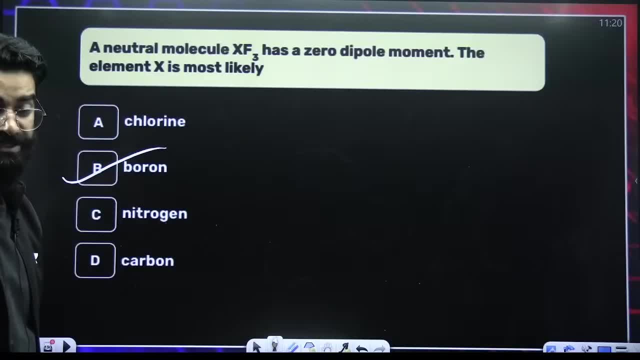 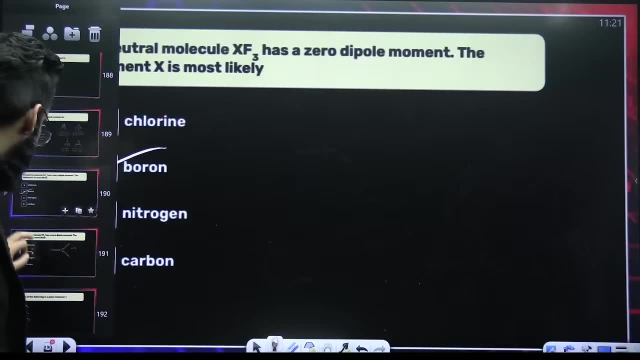 Yes, it has. Yes it has, Yes it has. I want you guys to be active in the chats. BF3 has got zero dipole moment right. You know it, You know it, You know it. Which of the following is the polar molecule? 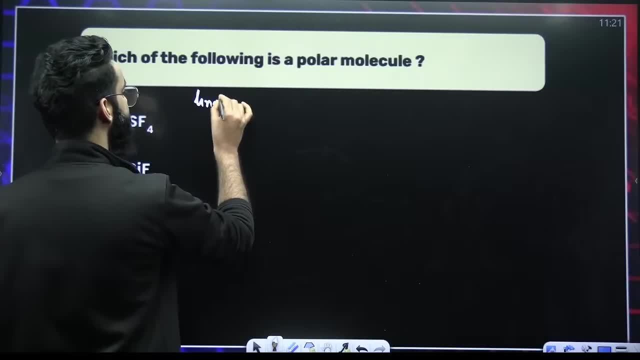 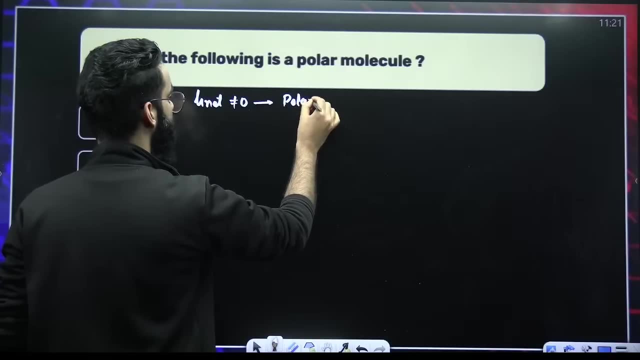 Polar molecule. The one which has got net dipole moment non zero, The one which has got net dipole moment non zero, is a polar molecule. Is a polar molecule. Net dipole moment non zero is a polar molecule. Now talk about the type of this. 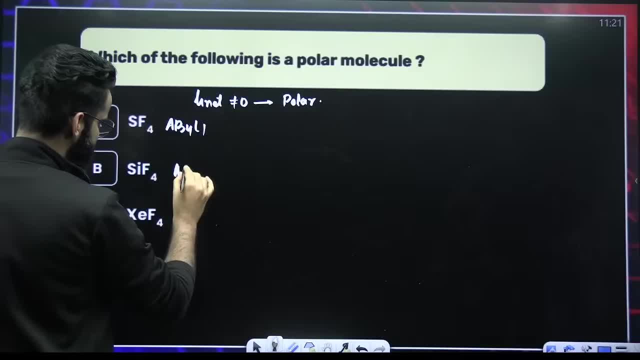 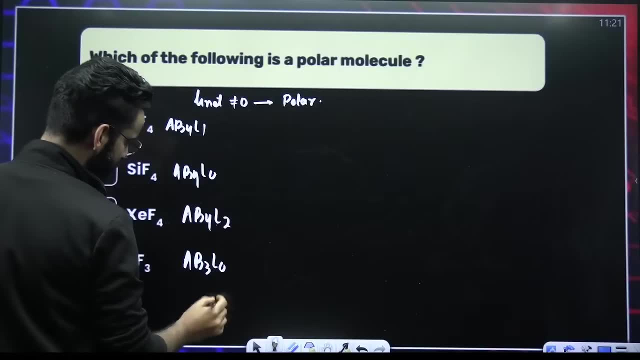 The type of this molecule, You know: AB, AB4L1. this is AB4L0, this is AB4L2, this is AB3L0. so this type zero dipole moment. this is having zero dipole moment, this will have zero dipole moment, this will have some dipole moment, so it's. 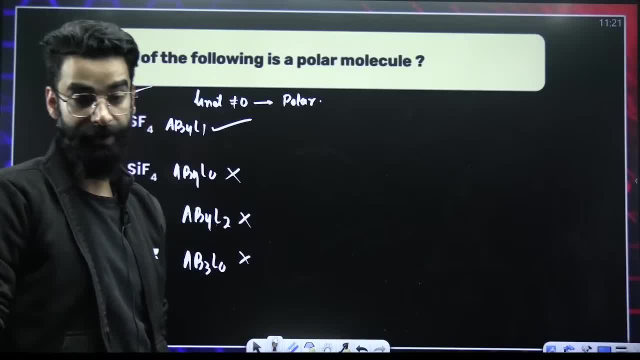 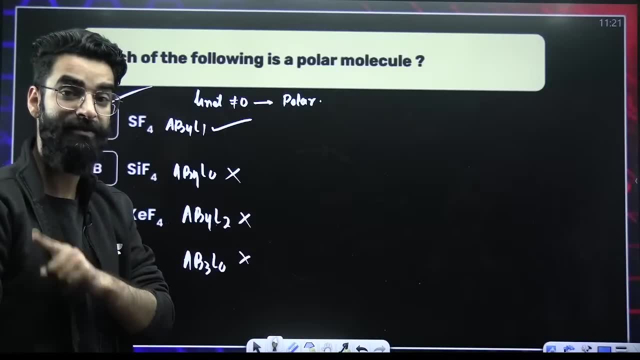 option, A right which has got some dipole moment. so it is polar, perfect, simple. so remember those types which I told you: AB2L0, AB3L0, AB4L0, AB5L0, AB6L0, AB4L2, AB2L3. 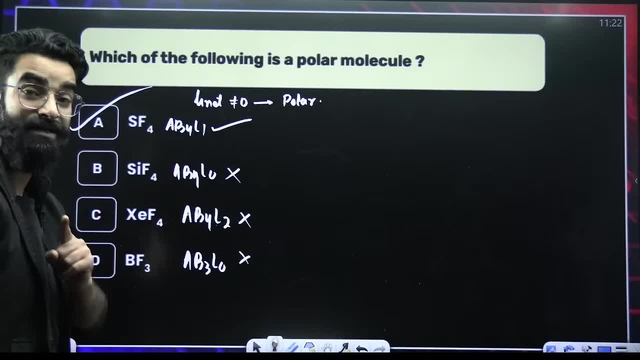 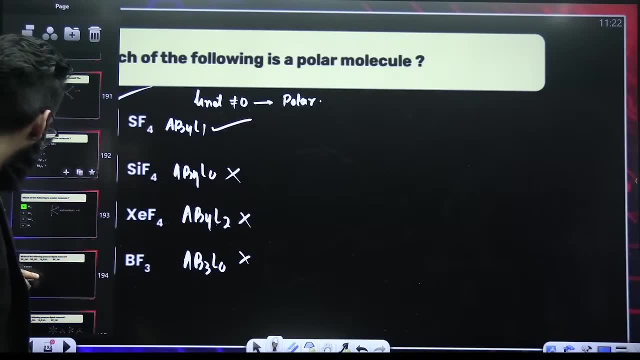 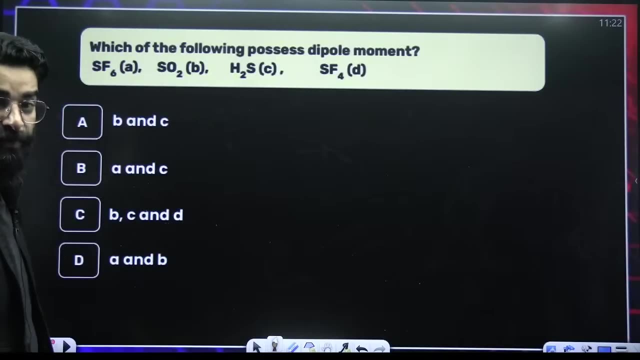 they whenever you see such kind of the molecule, that net dipole moment is that net dipole moment is zero. that means they are non-polar. yeah, moving ahead, moving ahead. tell me the answer of this question. which, quickly? which of the following possesses the dipole moment? which of the following: 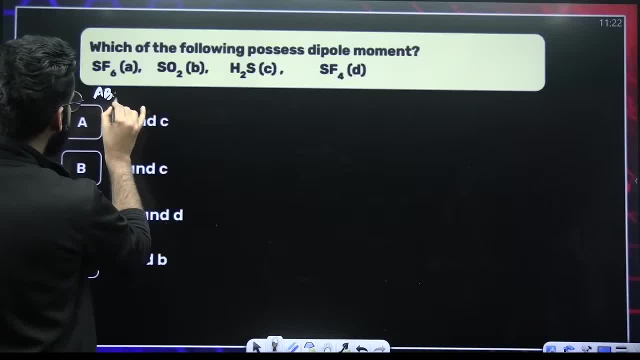 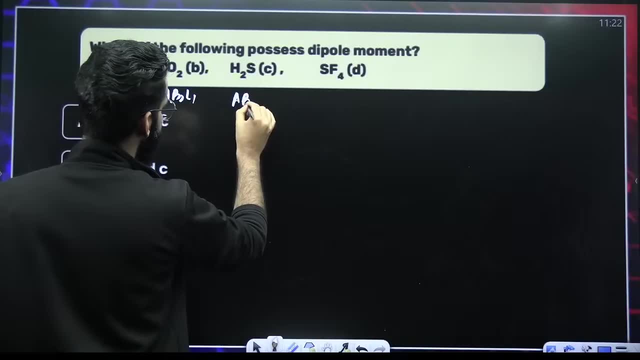 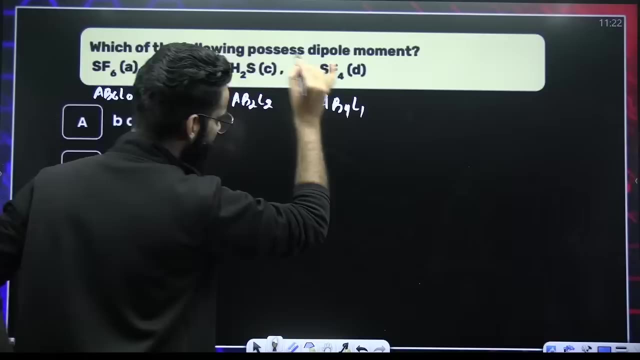 possesses the dipole moment type of this molecule: AB6L0- this one. this one. AB2L1- this one. it is AB2, AB6L0Y, L2, correct AB2L2.. This is AB4L1 type. Which of the following molecule possesses dipole? 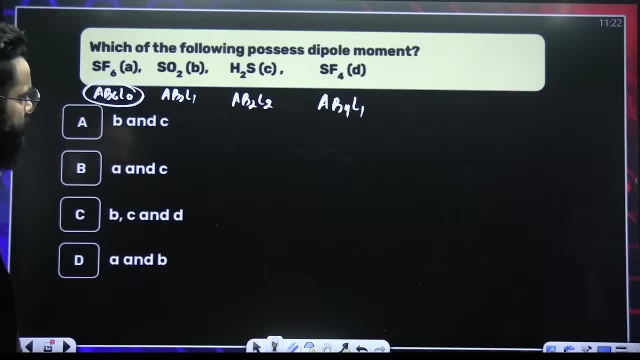 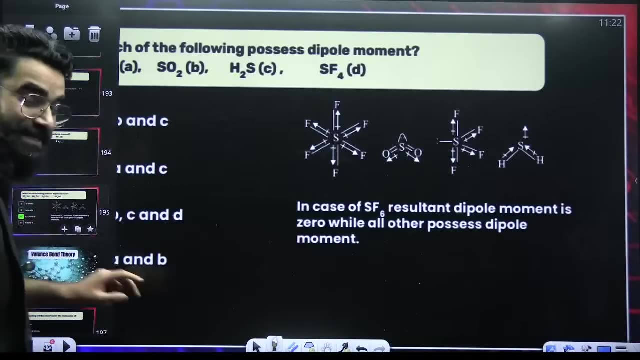 moment. See, the first one won't possess any dipole moment. right Rest, all the three will possess dipole moment. right Rest- all the three will possess the dipole moments. I hope you got it. I hope you got it right. So, basically, that category is important. which? 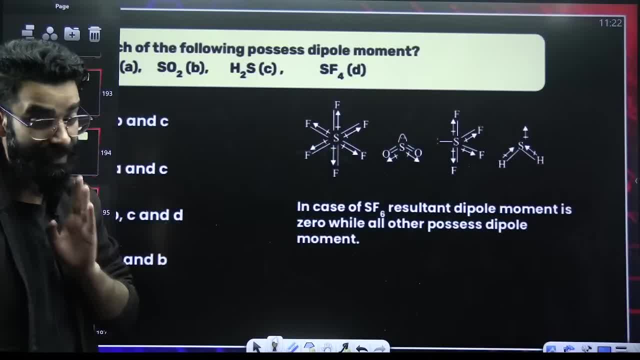 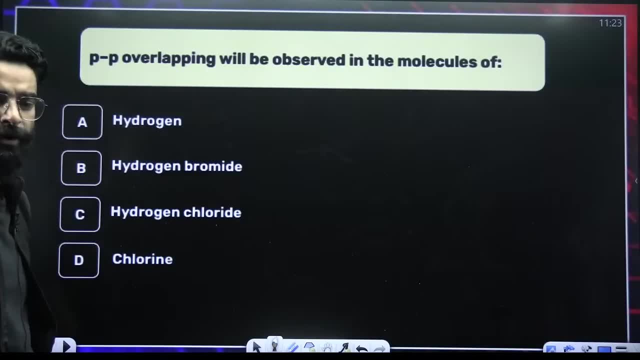 I told you the type of the molecules which show net zero dipole moment. You have to remember those types. You need to remember those types. Tell me the answer of this question: PP overlapping will be observed in which molecule? PP overlapping will be observed in which molecule In hydrogen? 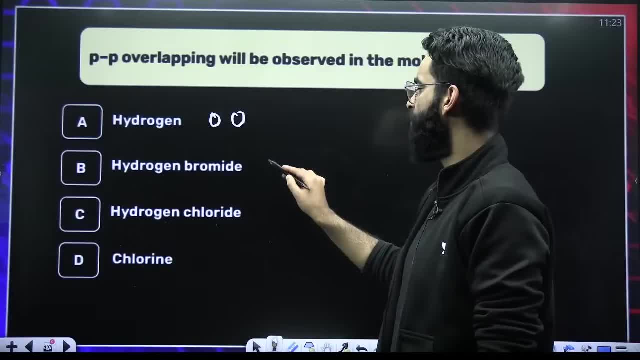 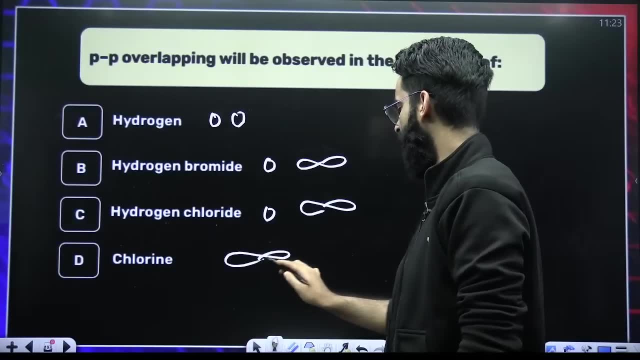 in H2 molecule there will be SS overlapping. In hydrogen bromide, there will be SP overlapping. In hydrogen chloride, there will be SP overlapping. In Cl2 molecule, there will be PP overlapping Right In VBD. yesterday we have discussed how your 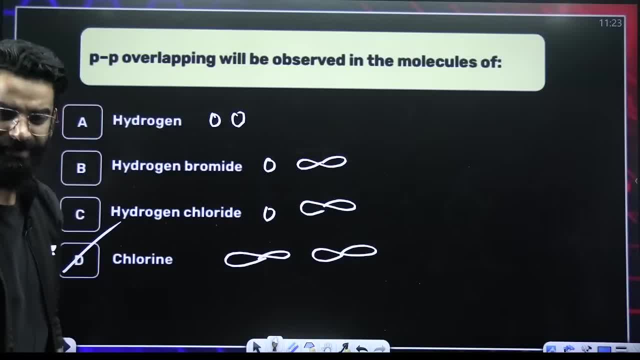 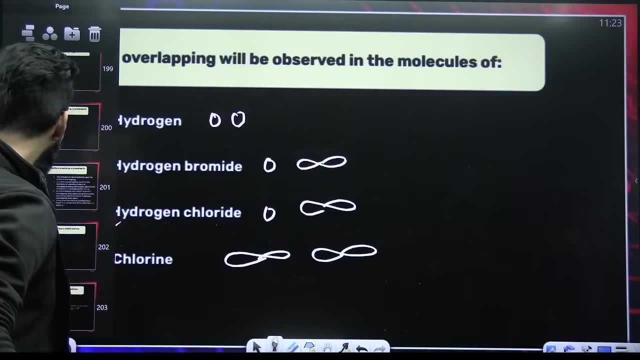 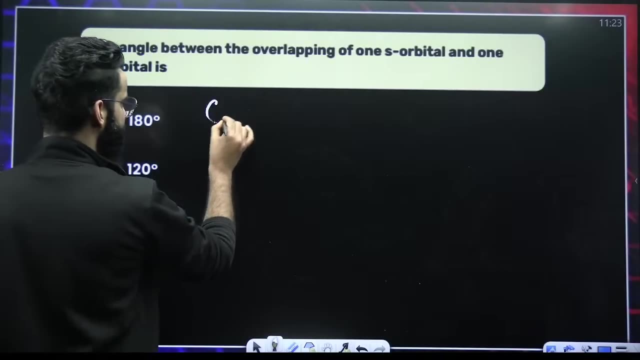 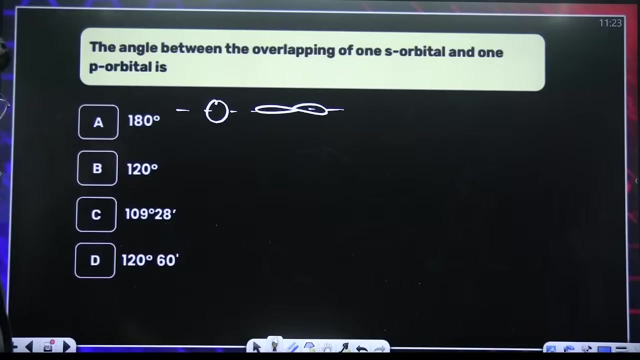 F2 molecule is formed. N2 molecule is formed, O2 molecule is formed right. I am moving ahead. I am moving ahead. The angle between the overlapping of 1S and 1P: If this is 1S and this is P right. The angle of overlapping. What is the angle of overlapping here? The? 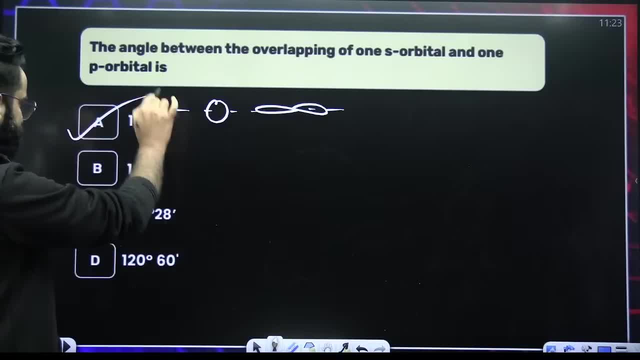 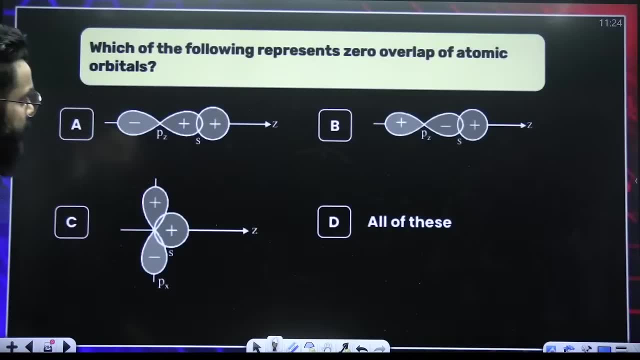 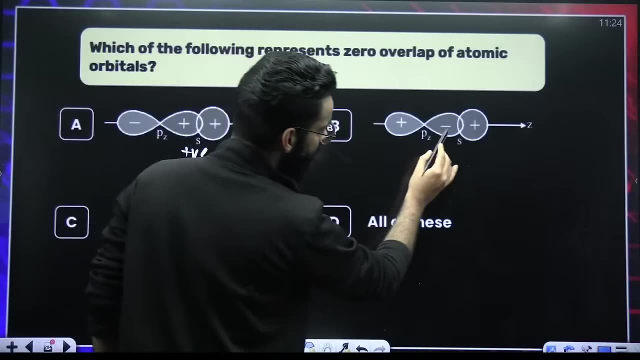 angle between the overlapping of 1S and 1P. What is it? 180.. Discussed in detail yesterday: 180.. Which of the following represents zero: overlap: Same sign- same side. This is positive. overlap Right: Opposite sign: same side: This is negative. 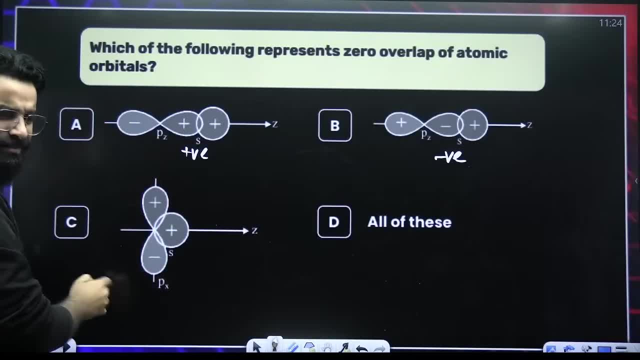 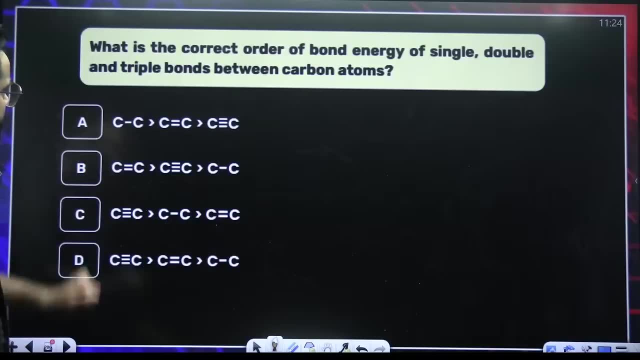 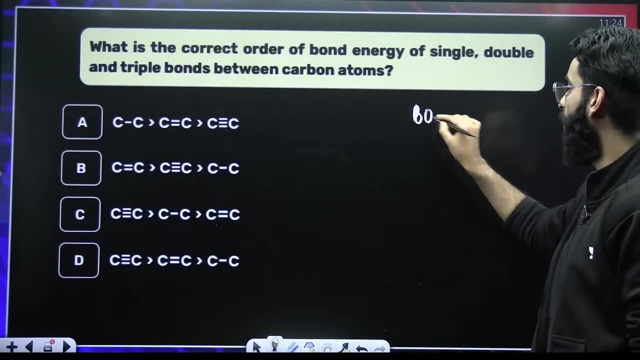 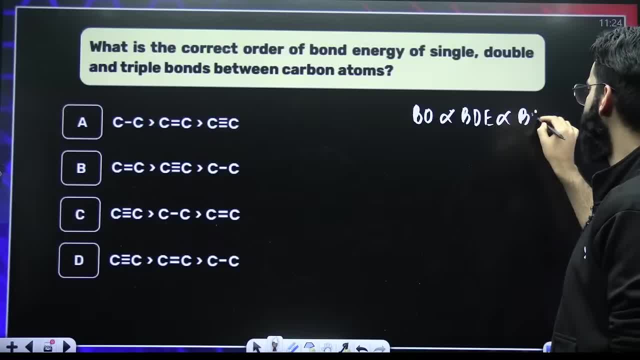 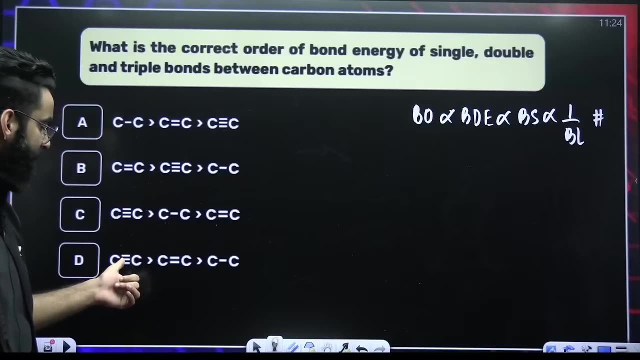 proportional to Bond dissociate energy, Directly proportional to Bond strength, Inversely proportional to Bond length, Inversely proportional to bond length. Right Bond order means number of bonds Correct. So more the bonds, more the bond strength, more the bond energy, Right. So this, this and this. 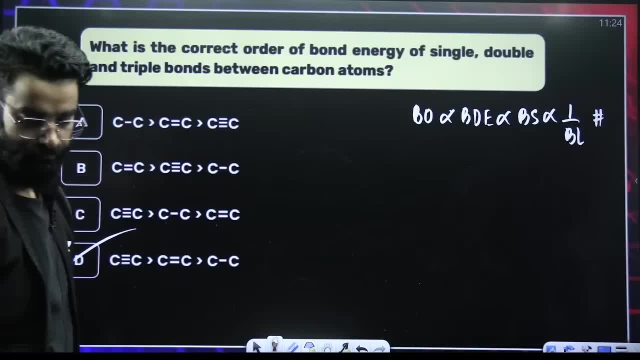 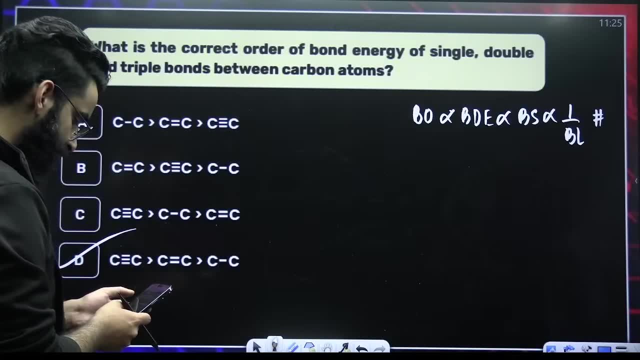 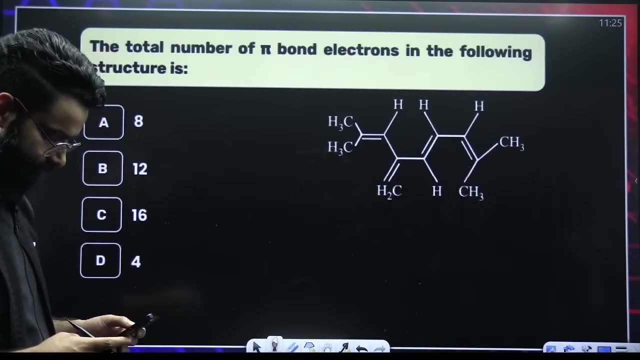 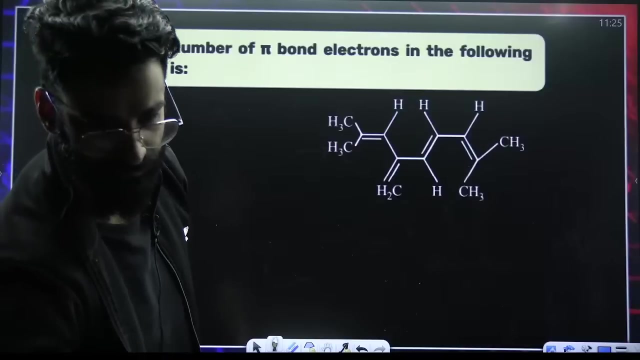 This is the bond energy. This is the bond energy. This is the bond energy order. Perfect, Perfect guys. Answer this question quick. Answer this question quick, Quickly. The number of pi electrons. Let me see how many of you will mark it wrong. 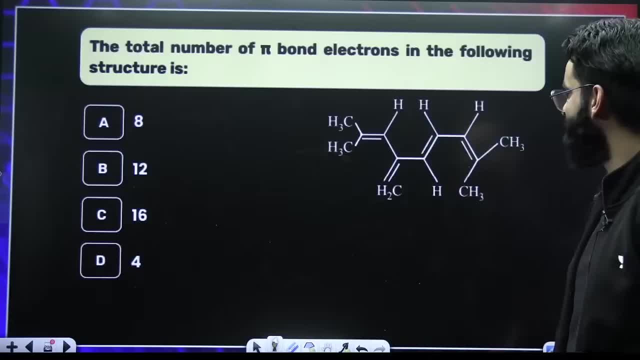 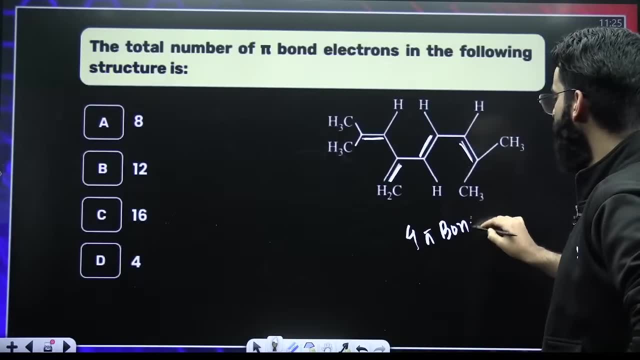 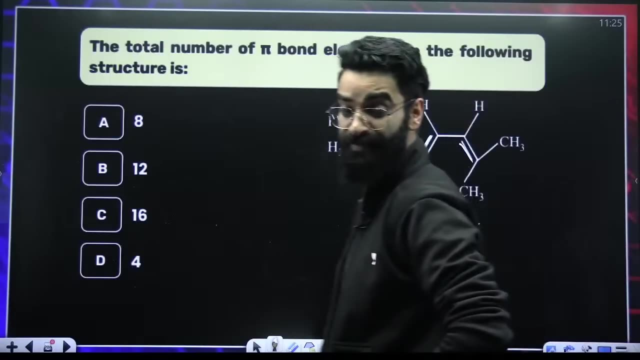 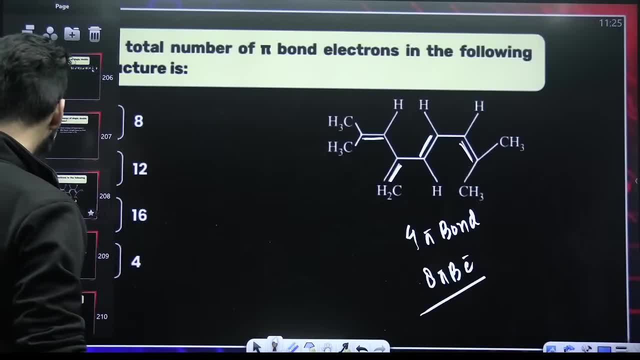 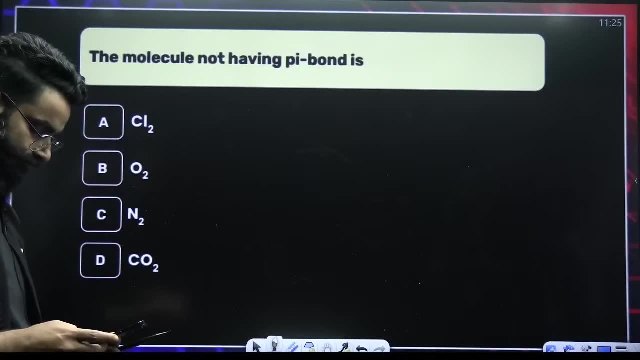 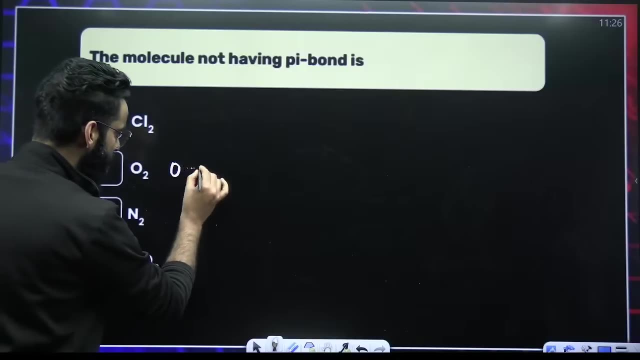 Try, don't write four or something Perfect. Answer this one quickly. Answer this one quickly. Answer this one quickly. The molecule not having pi bond- See guys, O2, you know, In MOT we saw O2A has a double bond. N2: there is a triple bond: carbon dioxide structure. 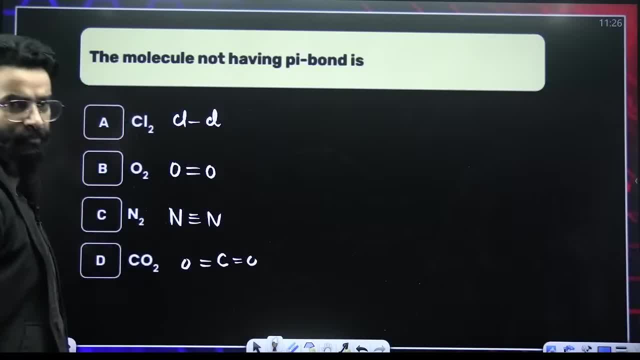 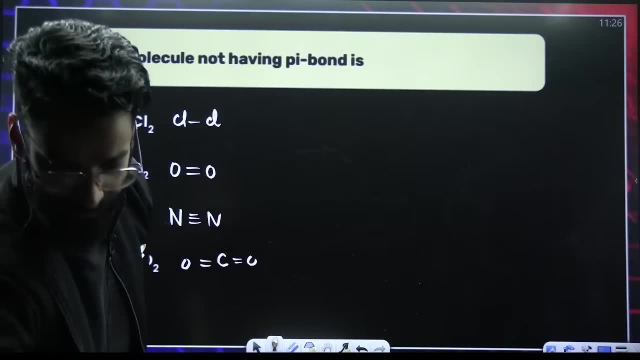 you know Right, Cl2, you know there is a single bond, Bond order is 1. Right. So what is here? It does not have any pi bond. right, It does not have any pi bond. Perfectly done. 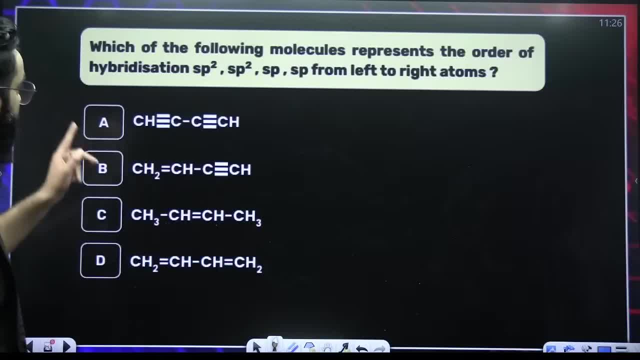 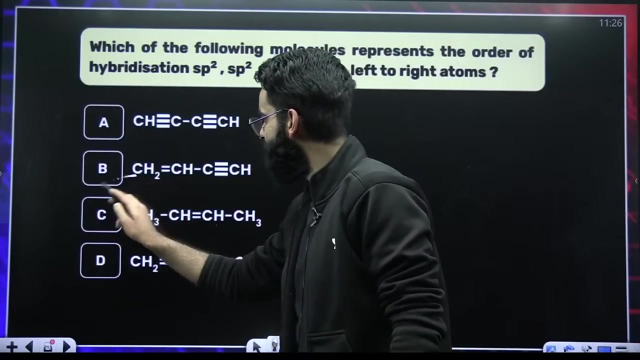 Moving on, Which of the following molecules represent the order of hybridization: sp2sp2spsp from left to right. Quick, Sorry, Quickly, guys, Kill it quickly. This is forming how many sigma bonds: 2 with hydrogen, 1 with carbon. 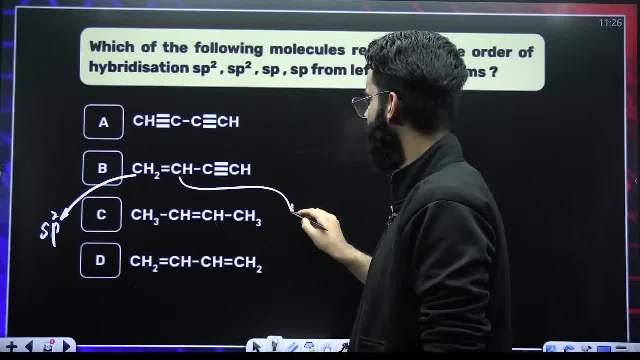 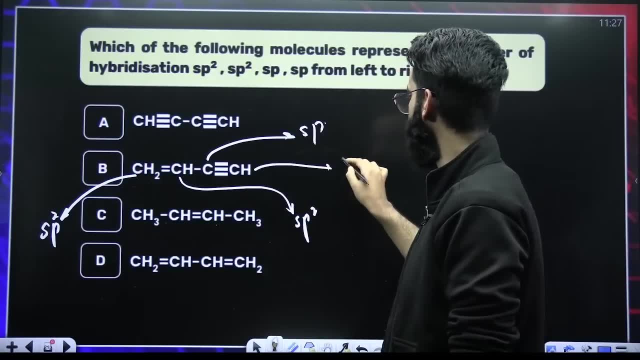 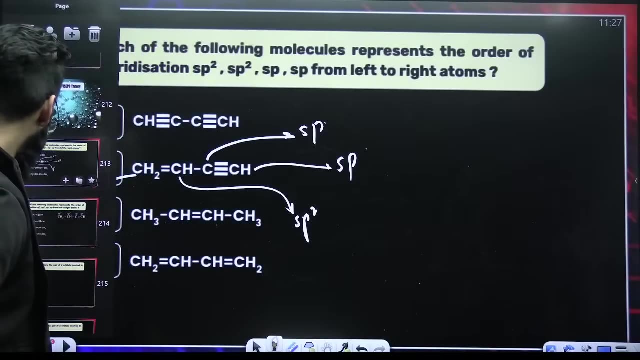 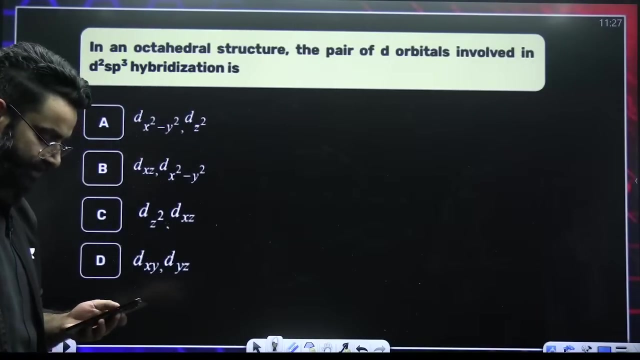 3 sigma bonds: zero loan per sp2. three sigma bonds: sp2. two sigma bonds: sp. two sigma bonds: sp. done, done people this: in the yesterday session i've told you which type of d orbitals are involved in sp3d2 hybridization. quickly. 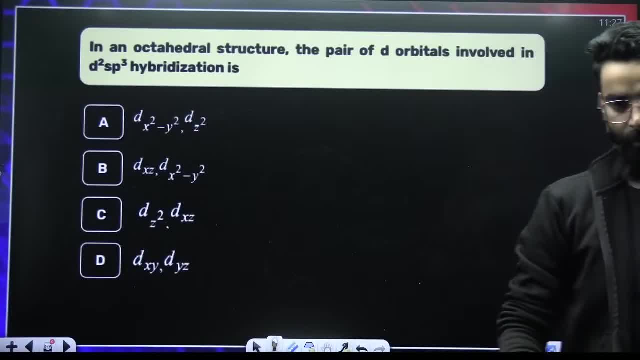 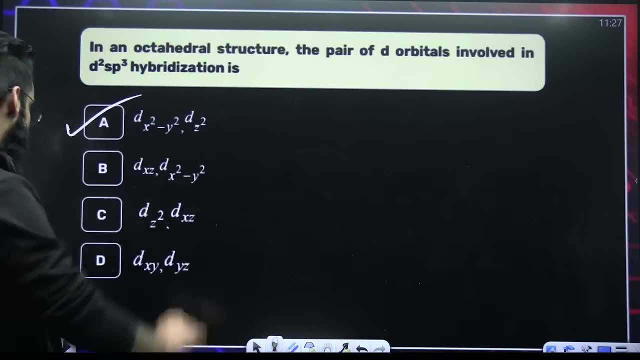 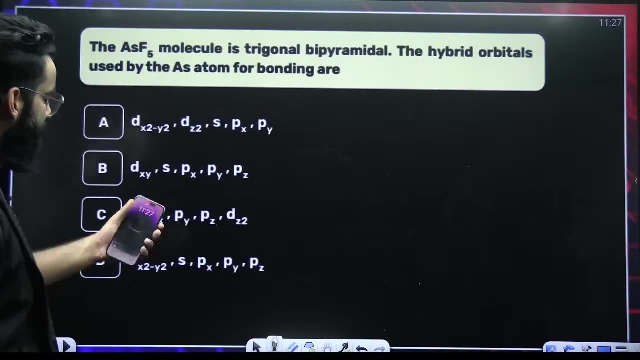 quickly people, which type of d orbitals are involved in the intermixing? yesterday i've told you in detail: it's d z square and d x square minus y square, right, yes, perfect, tell me this one. tell me about this one. asf5 molecule is trigonal bipyramidal. the hybrid orbitals used for as: first of all, if you look at the molecule asf5 we have, asf5 is a trigonal bipyramidal f5. we have right. the type of the molecule is ab5l0. hybridization is sp 3d. it is s plus px plus py plus. 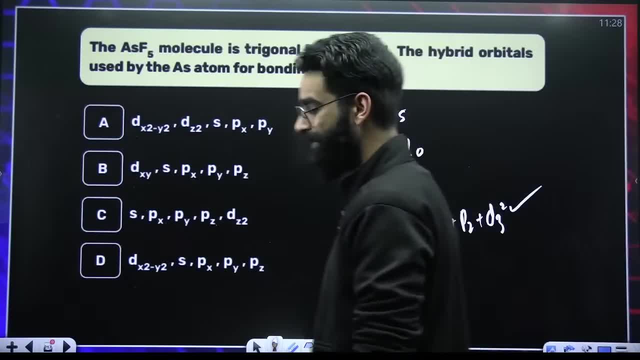 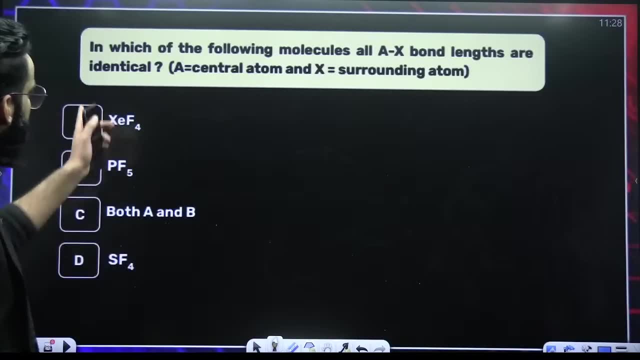 e z plus dz square in discussed in detail yesterday. yes, perfectly done. in which of the following molecule: a x bond length is identical, where a is the central atom, x is the surrounding atom. in which of the following? in which of the following: in which of the following all the? 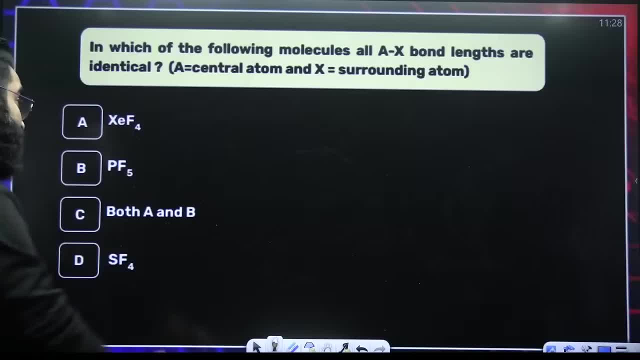 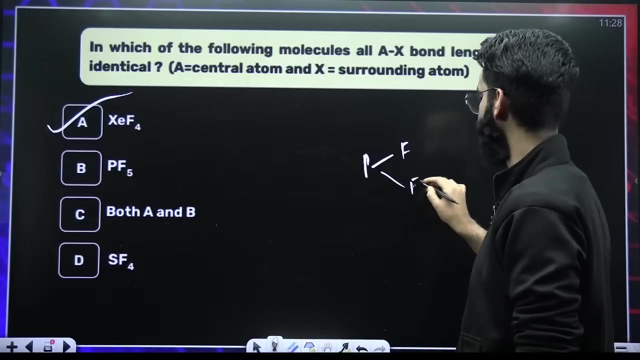 bond lines are equal, remember, in square planar one, if all the atoms are same, right, okay. okay, guys, moving on. okay, a lot of students are saying option c. why do you think option c? well, if you talk about pf5, if you talk about pf5, for example, or pcl5, if i talk about a molecule like this, 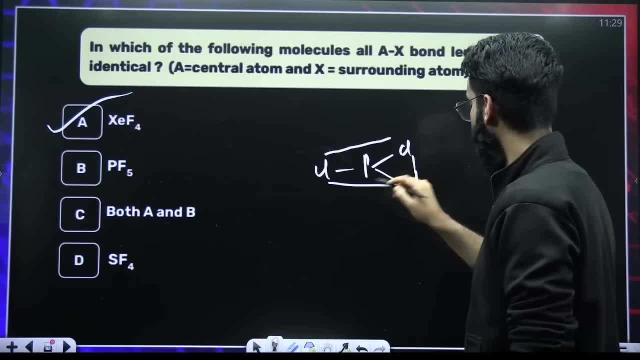 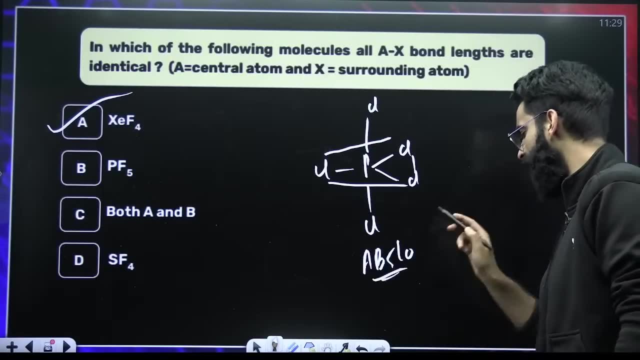 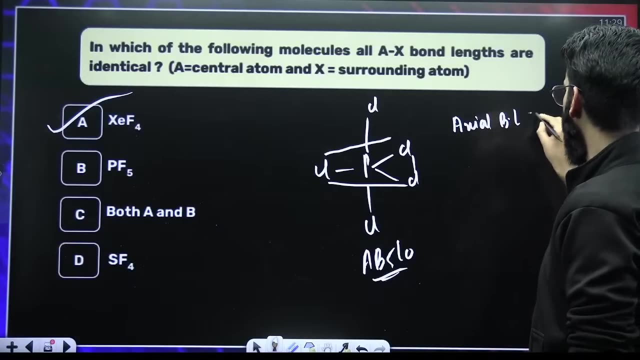 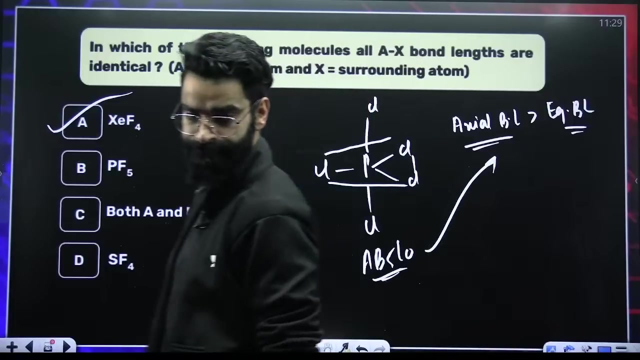 perfect. these are the equatorial bonds. this is axial. this is axial in case of your ab5l0 molecule: axial bond lines. axial bond lines are greater than that of equatorial bond lines in case of this particular category. remember this, okay, remember this carefully. remember from now. 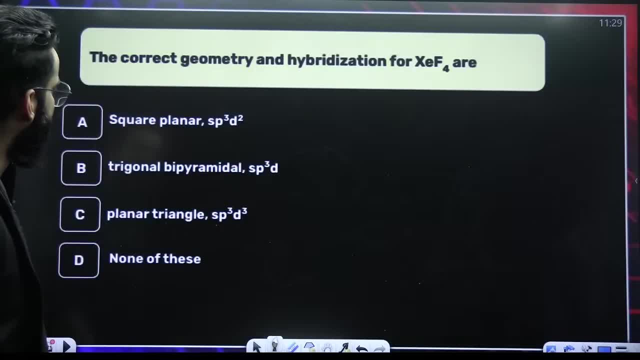 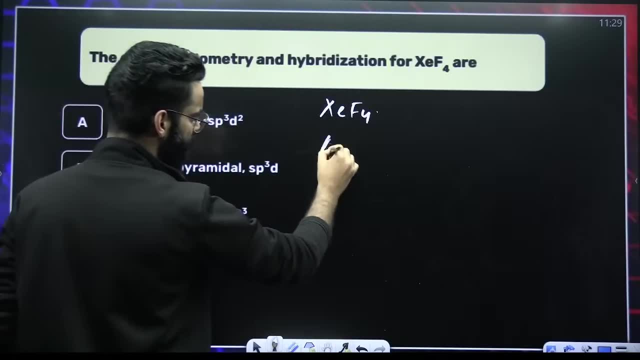 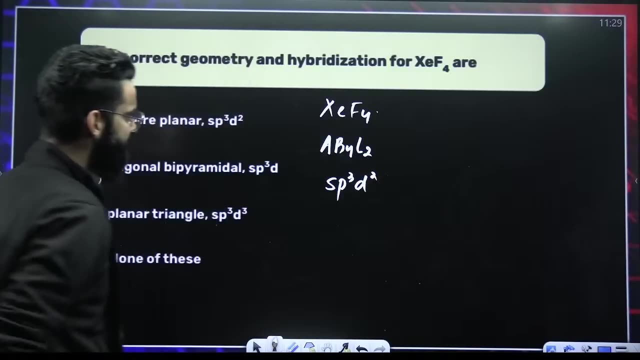 onwards quickly. the correct geometry and hybridization involved in xef4. how do you do that xef4, xef4: the type of the molecule is ab4l2 right- ab4l2. hybridization involved is sp3d2 right- sp3d2. perfect the geometry. 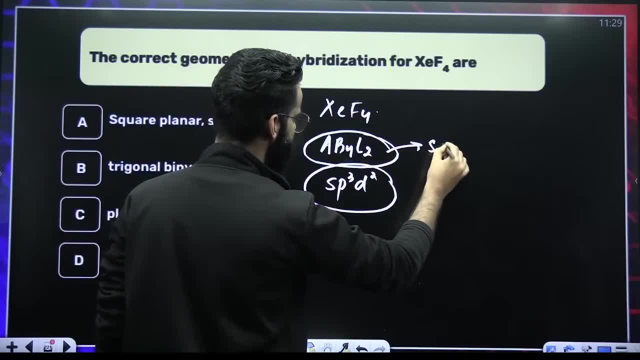 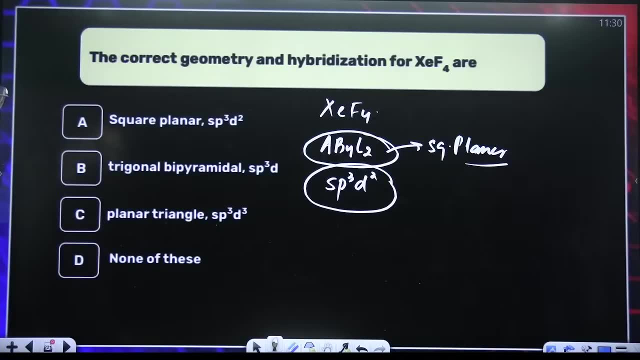 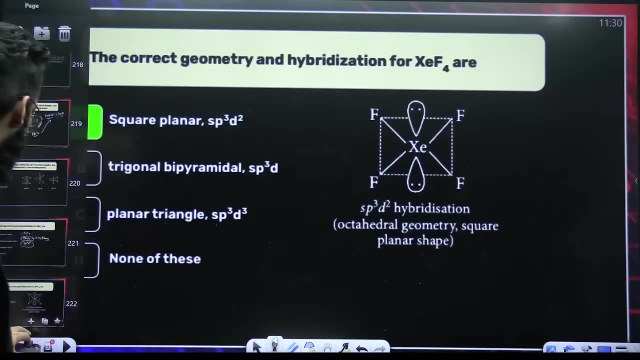 if you talk about this, sp3d2, ab4, l2, the shape of the molecule is square, planar, right? all those things we have discussed, all those things we have discussed, right, all those things we have discussed, perfect. so it's option, it's the correct answer of this particular equation. 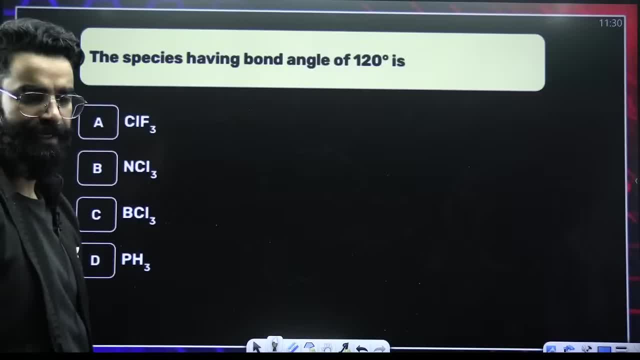 i'm moving ahead. the species having bond angle of 120, 120. the species having born angle of 120. so it has to be sp2, hybridized trigonal planar, right, okay, remember all the various possibilities here. if we did that, okay, the answer should be exactly the same. we will not be asking you all if you are. confused, if i can figure out how to solve this. in course of the image we are going to react to an au 4000 TV, but we will explain the protocol here, also what we are going to talk about when i put the some things. we do it and explain we did. 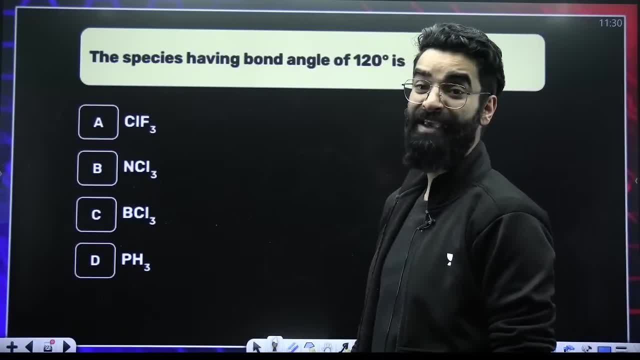 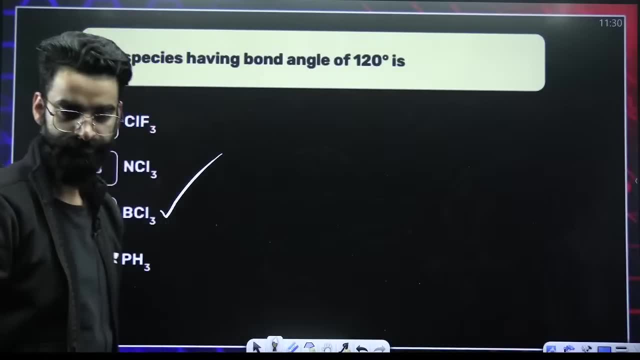 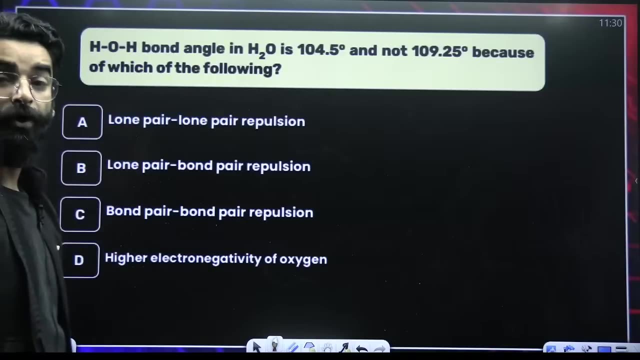 it has to be sp2 hybridized. the type of the molecule has to be ab2l0 or ab3l0. which one is ab3l0? this is ab3l0. that understood, yeah, perfect. in case of water. in case of water, my dear students, in case of water, the bond angle is 104 degree, 5 minutes. it has to be. 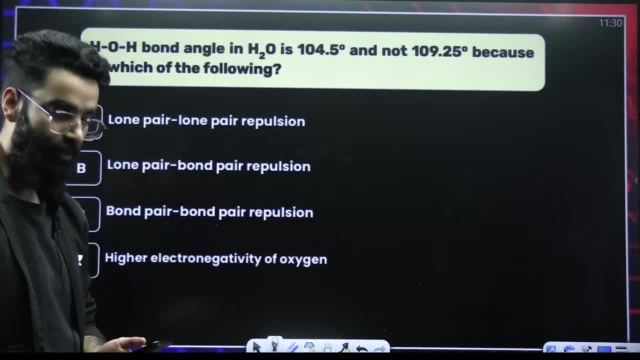 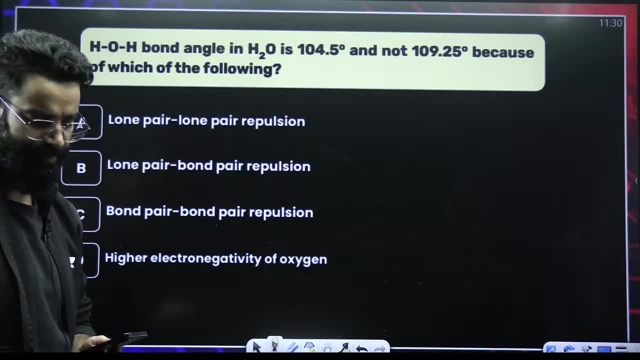 109 degree 28 minutes. what is the reason for that? what is the reason for that? quickly, let me know. in the chats in water the bond angle is 104 degree 5 minutes, but it should be 109 degree 25 minutes, right. what is the reason for the decrease in bond angle? it is: 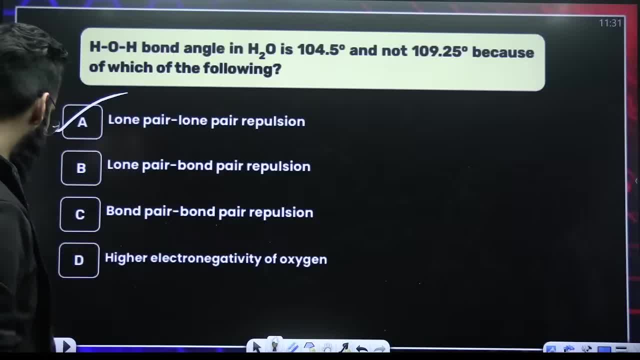 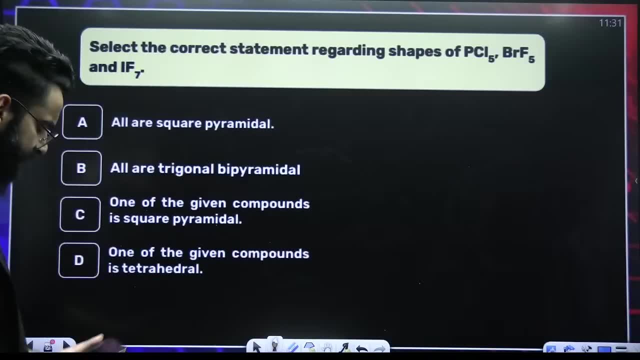 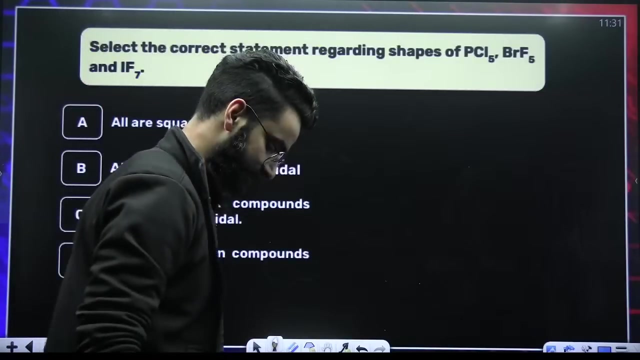 the lone pair, lone pair repulsions which happen there in case of water. okay, what do you think about this one? quickly in the chats. i'm looking at your chats only. i am looking at your chats only quickly, quickly, people, everyone, this is simple, this is simple. it's pretty, pretty much simple. 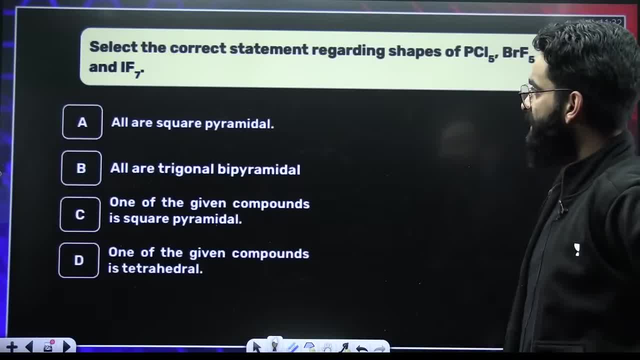 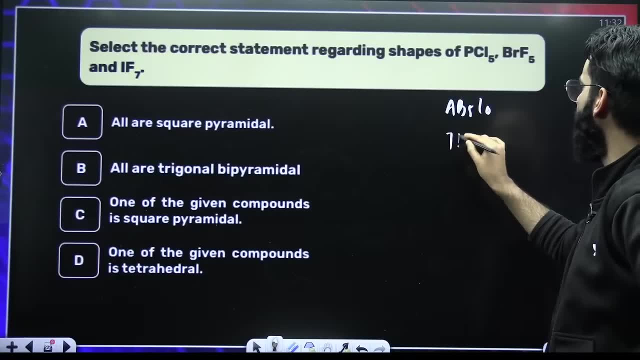 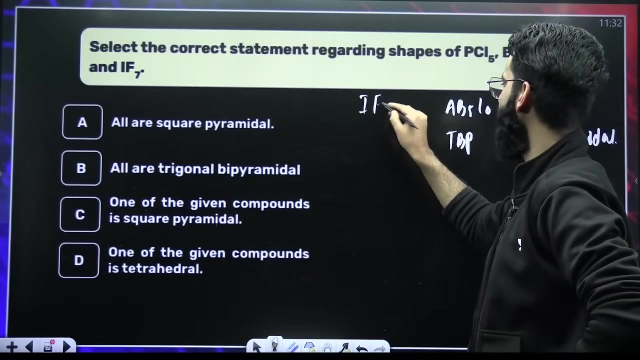 select the correct statements regarding the shape of pcl5. shape of pcl5. pcl5 is ab5l0, trigonal bipyramidal right brf5. it is ab5l1. it is square pyramidal. it is square pyramidal. one more is if7. if7 is the type is ab7l0. it is pentagonal bipyramidal. 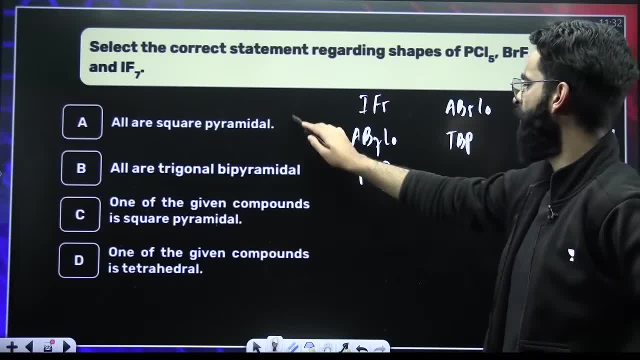 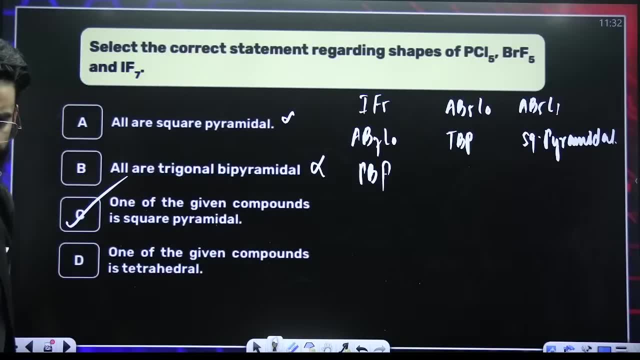 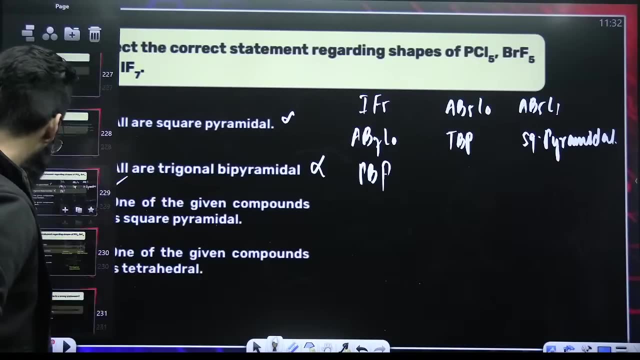 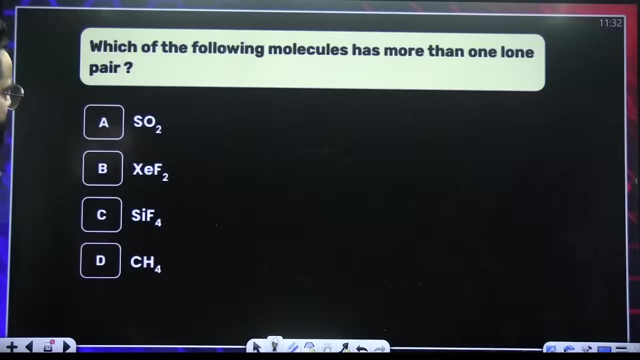 now select the answers. select the correct statement. all are square pyramidal? no, all are trigonal bipyramidal. no one of the given compound is square pyramidal. yes, right, done people, all right, all right, perfect, perfect. which of the following molecules has more than one lone pair? 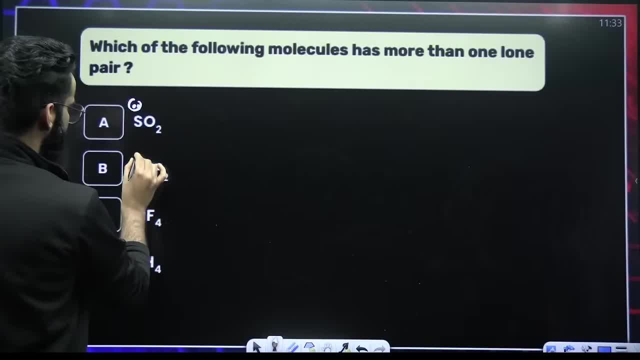 more than one lone pair. sulfur has got one lone pair. over here, xcf2 xenon has got three lone pairs. silicon: no lone pair. carbon: no lone pair. right, which of the following pairs has more than one lone pair? it is option b, which is the correct one. 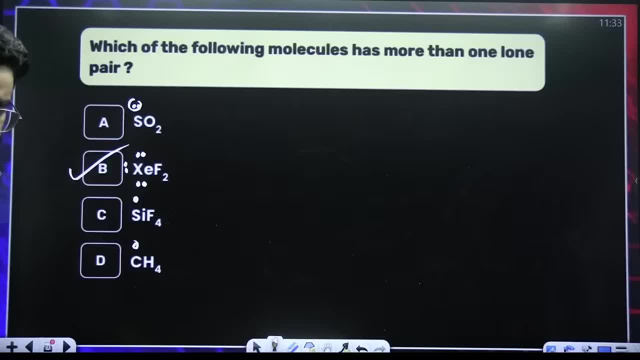 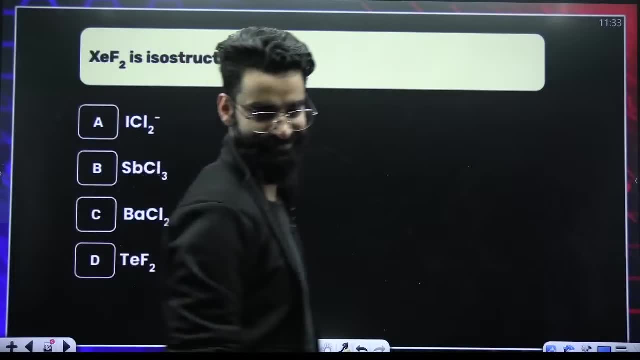 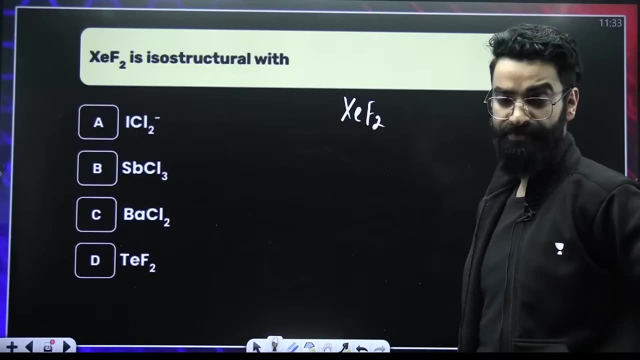 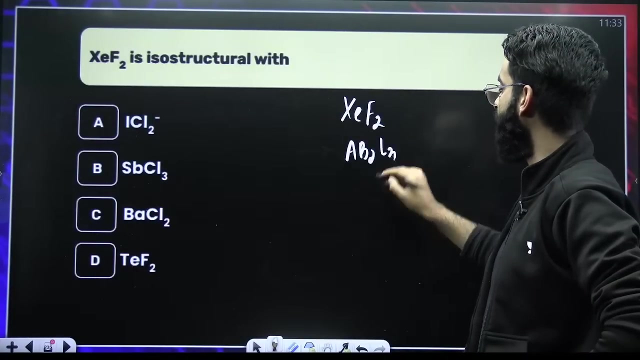 correct. absolutely, guys, all of you are perfectly right. that means you have understood the chapter. that means you have understood the chapter. that's great. that is great. xef2 is isostructural width, xef2. xef2 is isostructural width, xef2. type of the molecule is ab2l3. right hybridization is sp3d. 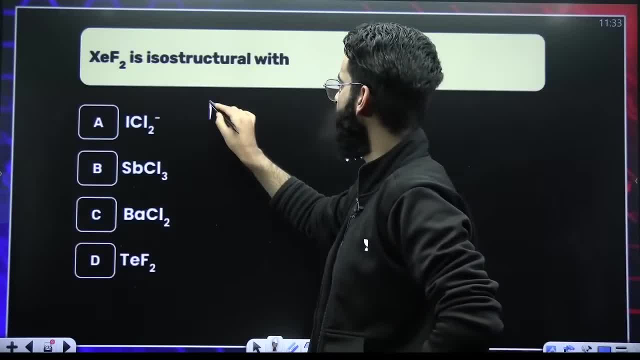 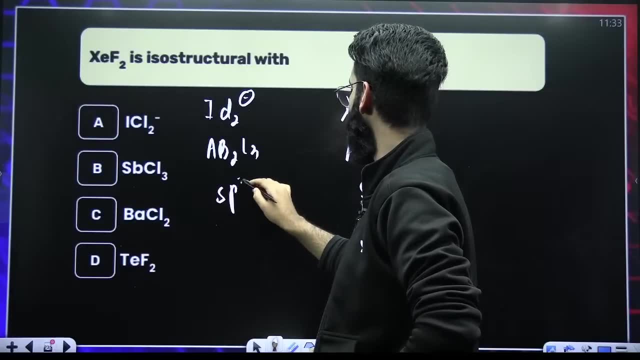 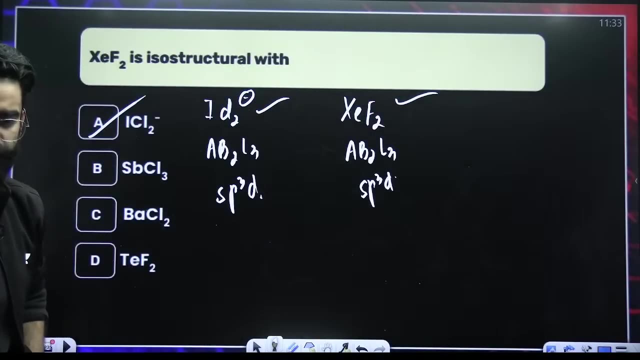 hybridization is sp3d. look at icl- negative. Look at ICl2 negative Type of this molecule is also what AB2L3.. Hybridation here also is sp3d- Perfect. So they must be isostructural, They must be isostructural. They must be isostructural, Yes, they must be. 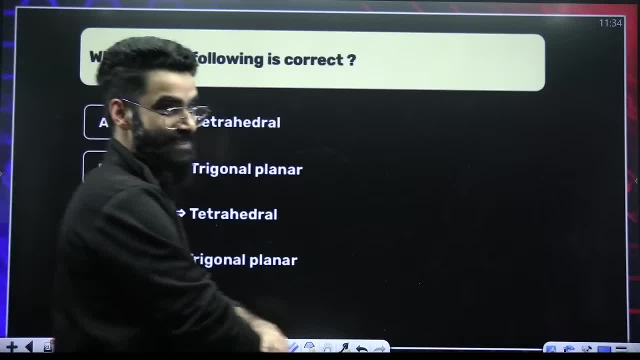 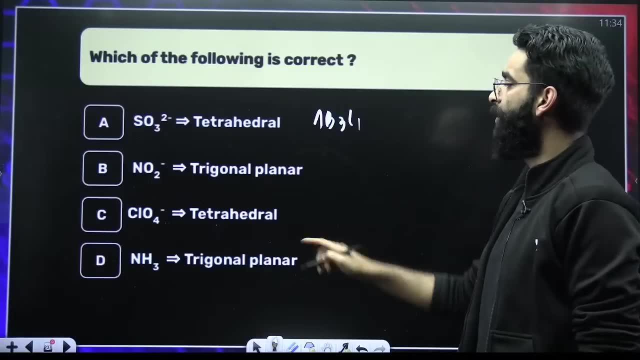 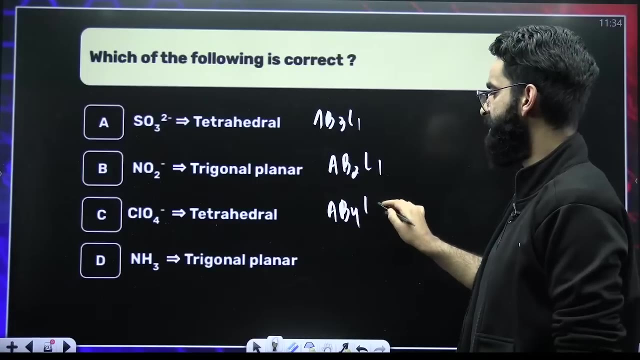 isostructural. Which of the following is correct: SO3 di negative, SO3 di negative. Let's write the type of the molecule. Type of the molecule is AB3L1. Right NO2 negative. NO2 negative- AB2L1.. CLO4: negative. AB4L0. NH3. AB3L1.. 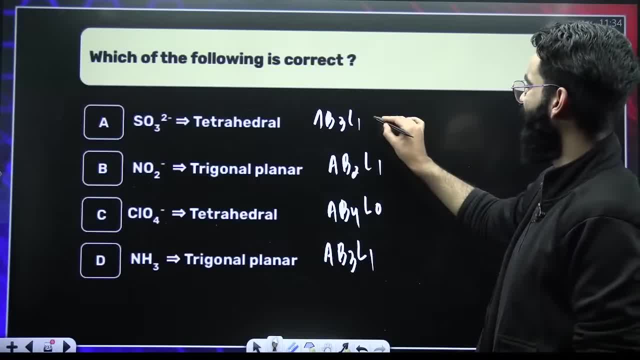 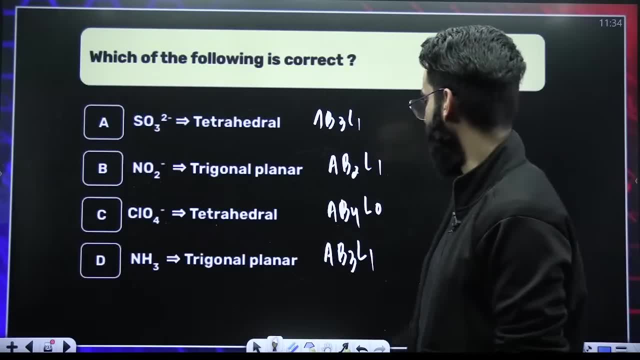 Which of the following is correct? Well, AB3L1.. First of all, SO3 di negative. AB3L1.. Is this going to be tetrahedral? Which one is going to be tetrahedral? AB4L0 is tetrahedral, So CLO4 negative is tetrahedral here. Yes, 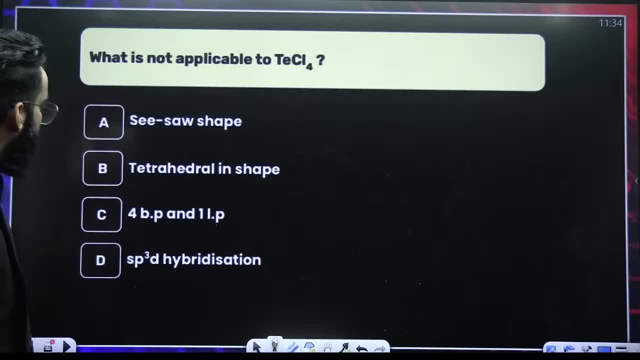 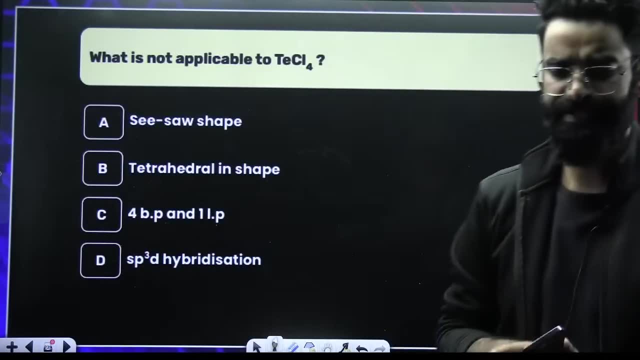 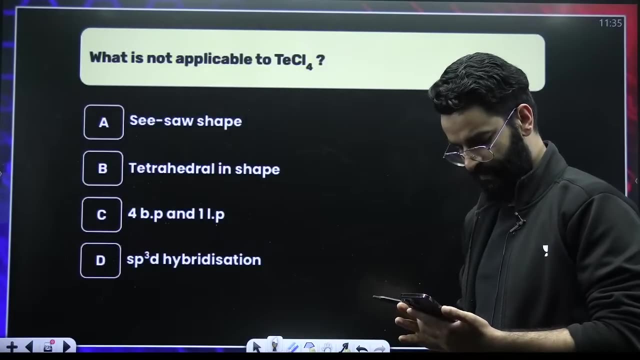 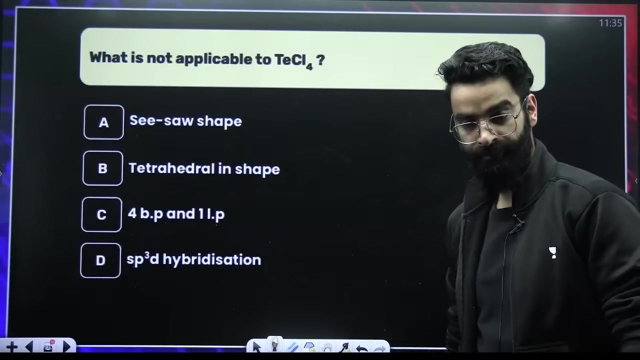 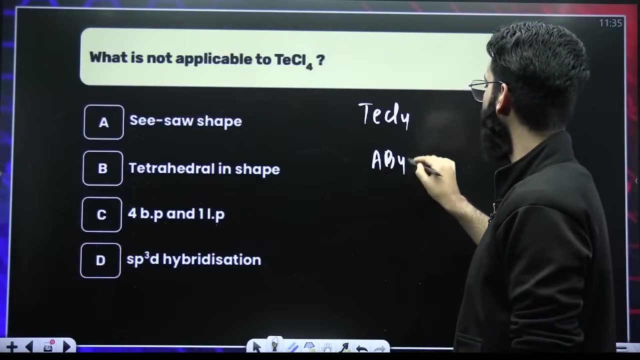 Perfect, Which is not applicable to TECL4?. TE is your group 16 element. TE is your group 16 element? Quick, Quick people, Quickly in the charts. Done TECL4.. The type of the molecule is AB4L1.. Is it going to be tetrahedral, Is it? 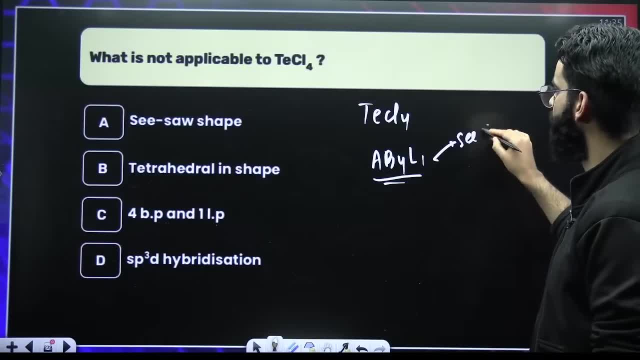 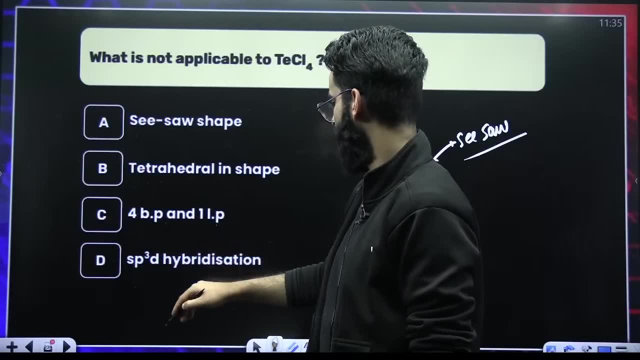 going to be tetrahedral AB4L1?? It is seesaw shaped. It is seesaw shaped Right, So which is not applicable. Not applicable means tetrahedral in shape. Option B is the one. I hope it's. 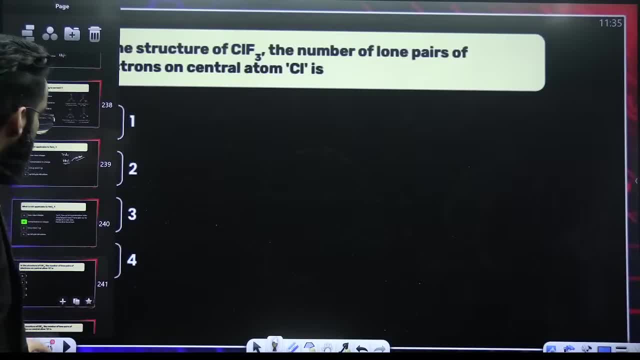 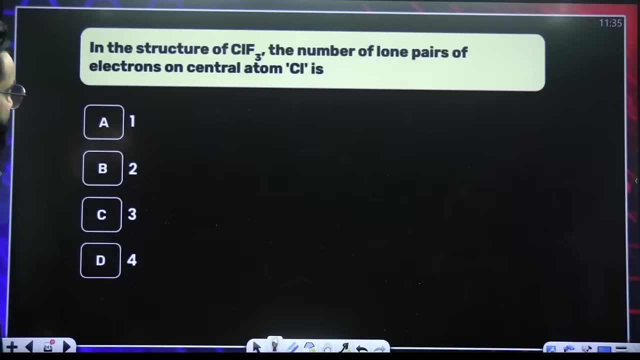 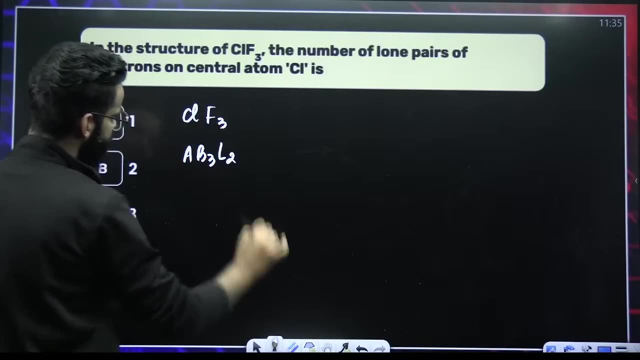 clear. I hope it's clear. What about this one In the structure of CLF3, the number of lone pairs of electrons on central atom? In case of CLF3, CLF3,, the type of the molecule is AB3L2.. Right, AB3L2.. So there? 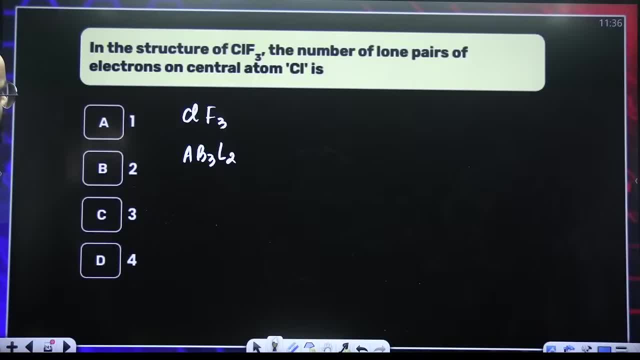 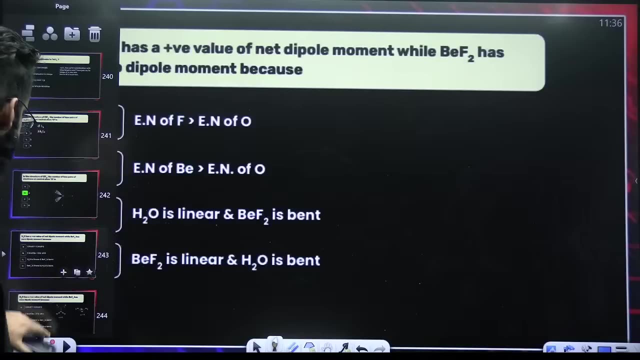 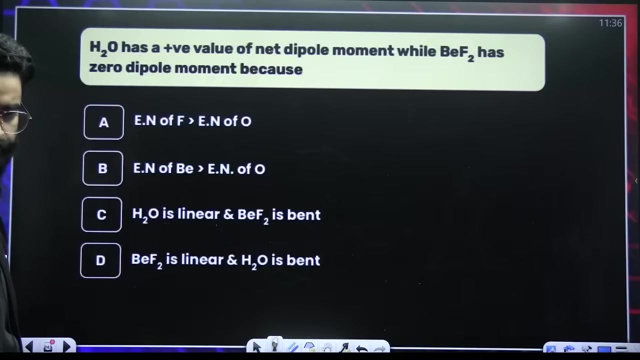 are two lone pairs. There are two lone pairs on the central atom. Yes, There are two lone pairs on the central atom. Perfect, Perfect, Perfect, Alright. What about this one? What about this one? What do you think about this one? 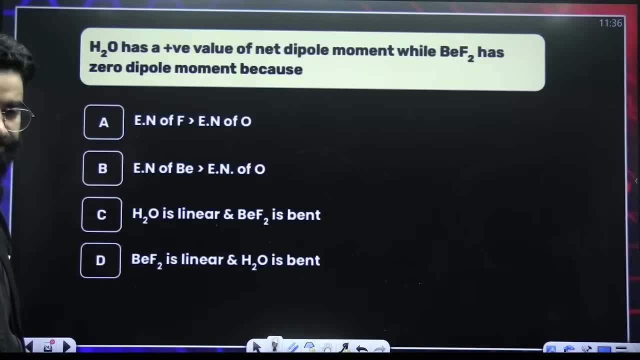 Water has positive value of net dipole moment, BEF2 has zero. Why is that? Why is that? Because BEF2 is linear, Water is bent Right. BEF2 is linear and water is bent Correct: BEF2 is linear and water is bent. 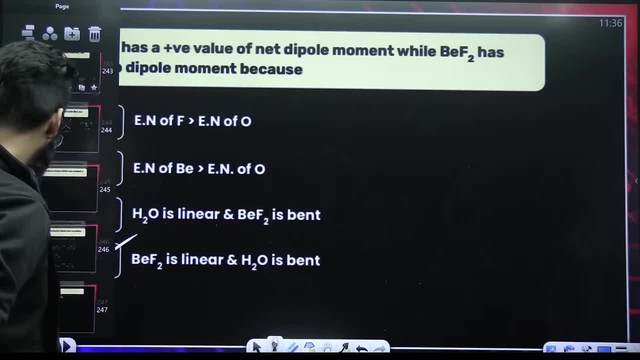 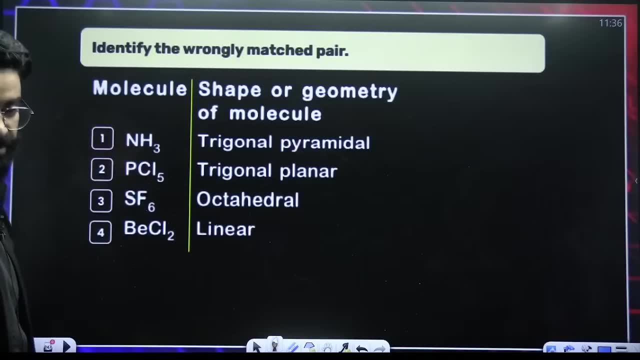 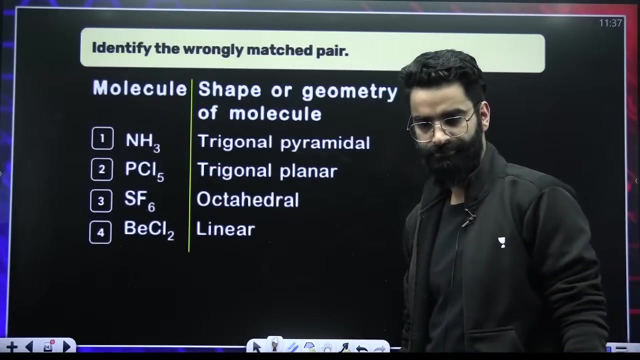 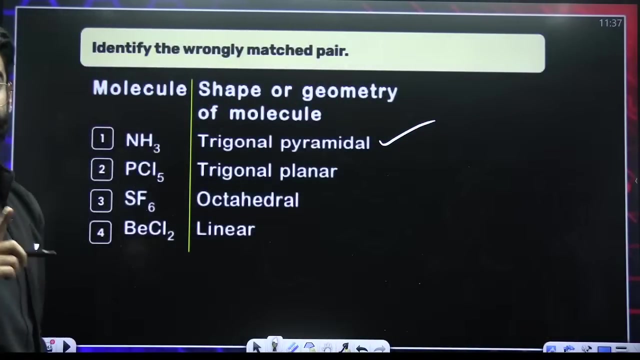 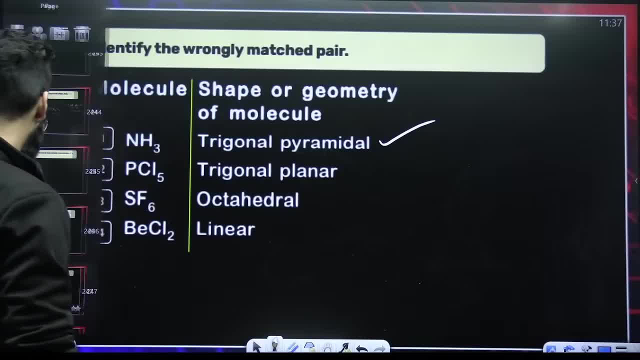 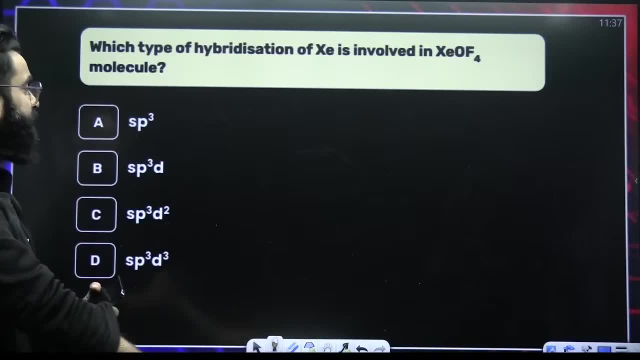 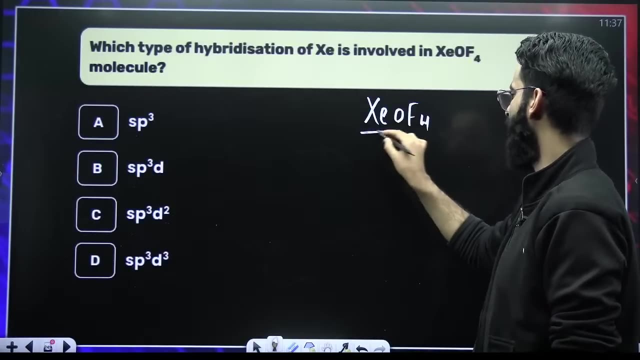 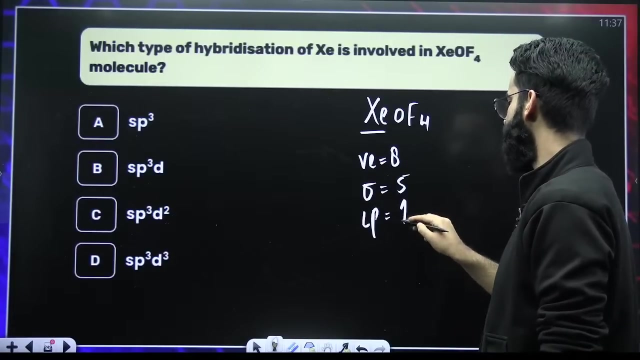 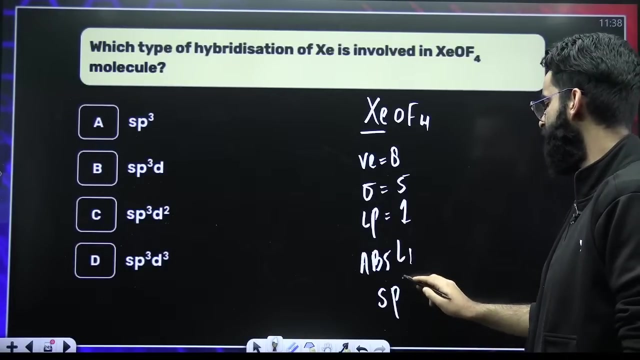 it's pyramidal. yeah, it's pyramidal, it's pyramidal. Which type of hybridization of xenon is involved in XeOF4 molecule XeOF4, XeOF4, valence electrons: 8, sigma bonds: 4 plus 1, 5, lone pairs: 1, right type of the molecule AB5L1, hybridization. 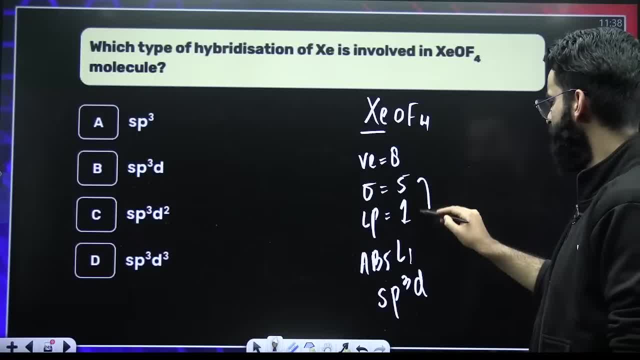 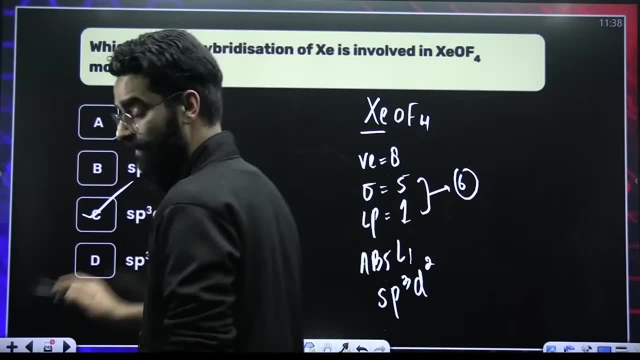 sp3, okay. steric number is. steric number is 6, hybridization is sp3, okay. So there is a type of compound, XeOF4, in the H3N1,, H3N2, H3B2.. 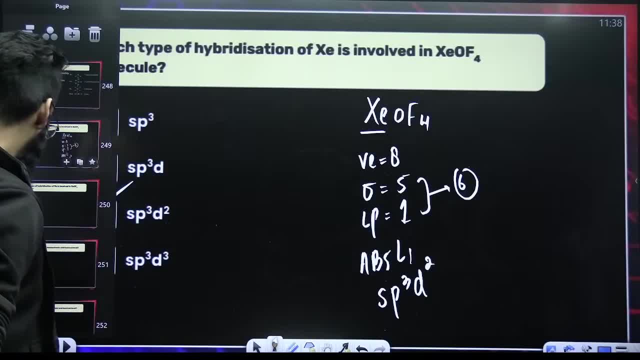 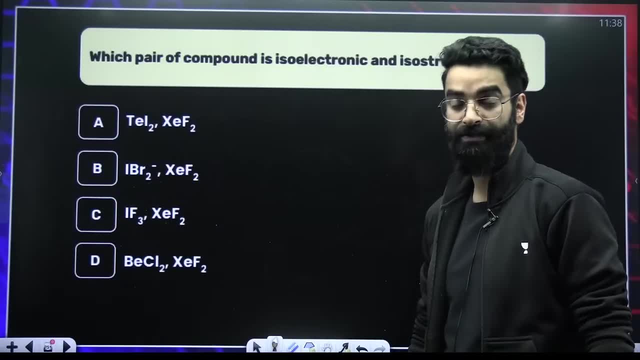 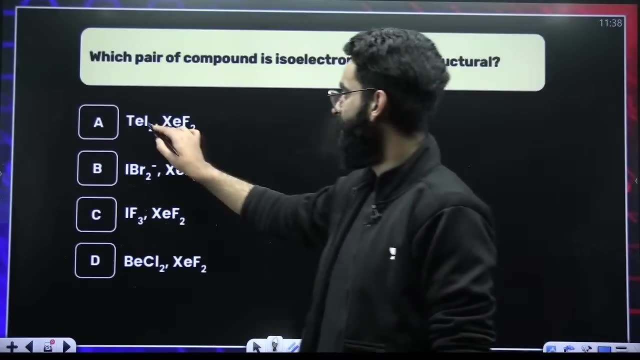 Okay, done, done. people. Which pair of compounds is isoelectronic and isostructural? Isoelectronic, isostructural, isoelectronic? get the type of every molecule. get the type of every molecule. if you look at this particular one, it is type: is AB2L2.. 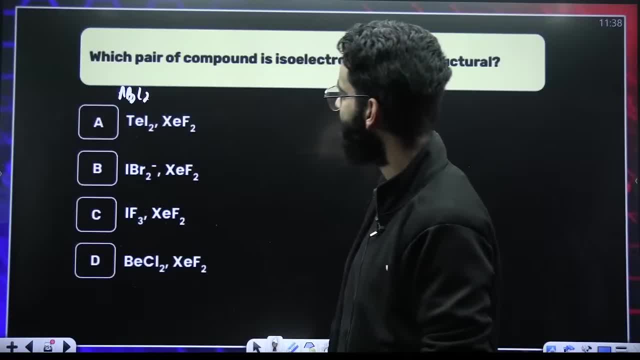 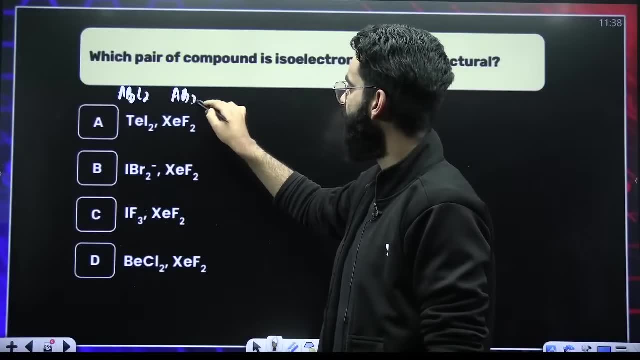 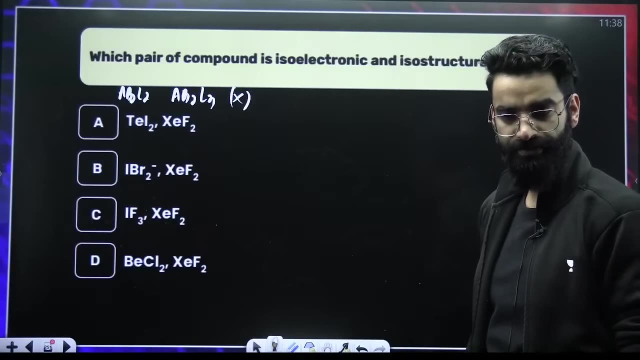 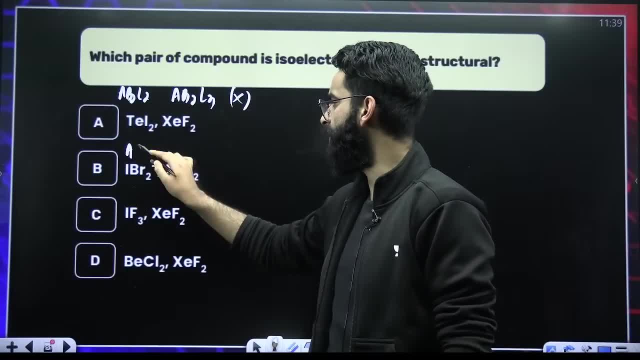 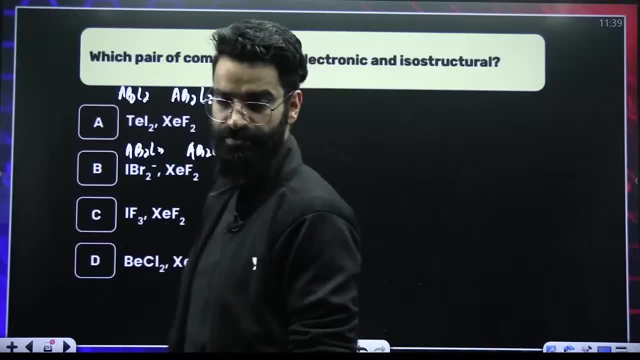 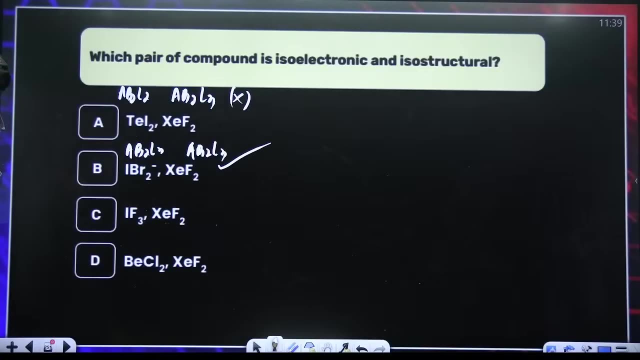 IBR2-2. IBR2-2- it is AB2L3 type. this one is also AB2L3 type, so type is same. so they are supposed to be iso-structural. they are supposed to be iso-structural. yes, guys, I want you guys. 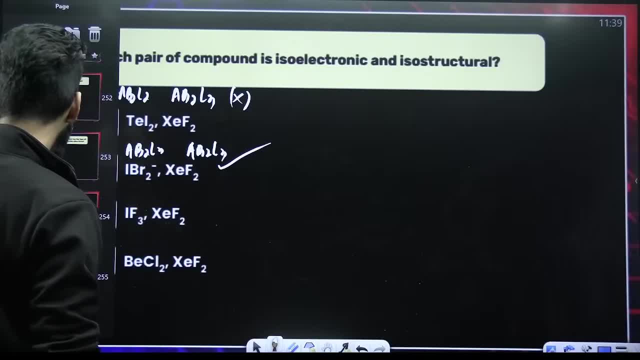 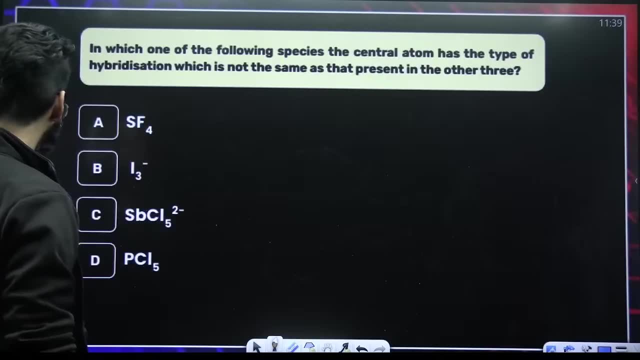 to be ec2 in the chats. by the way, I want you all to be ec2 in the chats. what do you think about this one? what do you think about this one in which, of the following species, the central atom has the type of hybridization which is not the same as present in other? 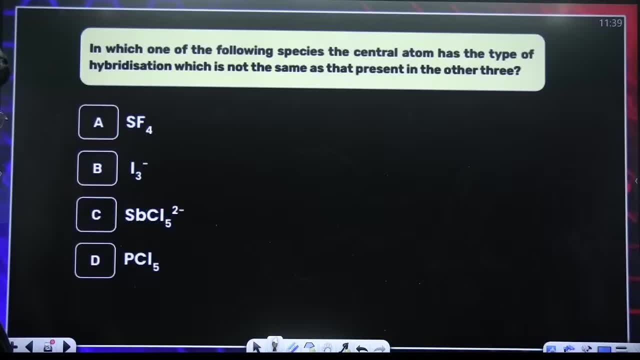 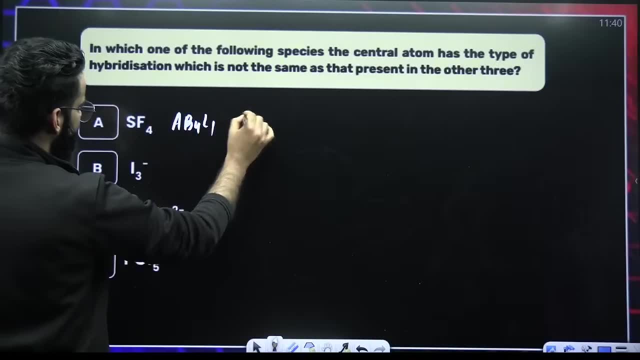 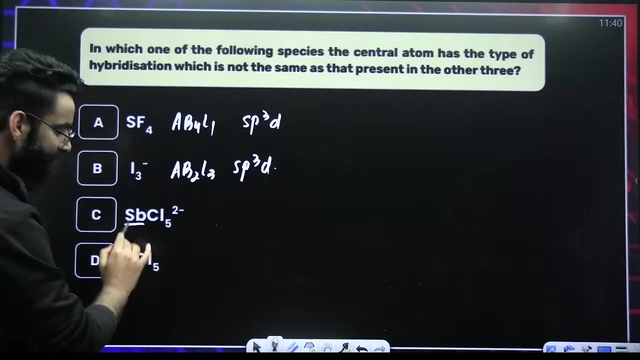 three, which is not the same as present in other three. first of all, get the type. type of this molecule is AB4L1. steric number is four plus one, five. let's speed 3d. this is AB2L3 type, SB3D. what is what is SB? what is SB? what is SB? it's antimony, right. 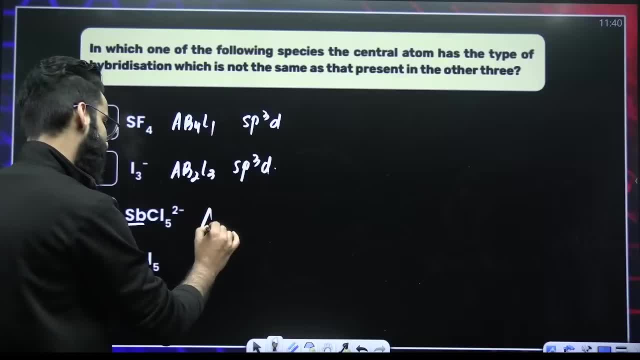 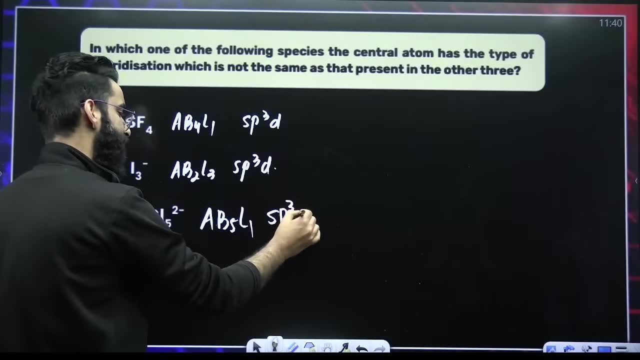 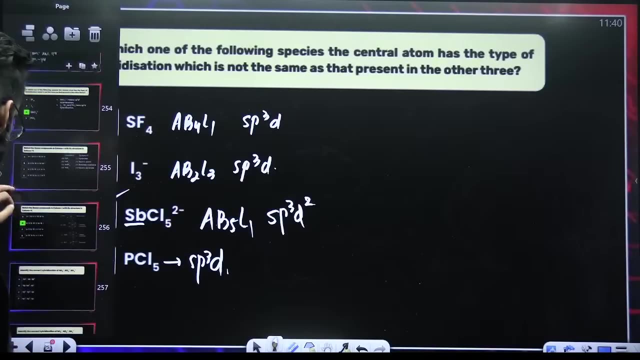 it is antimony, perfect. the type of the molecule will be AB5L1, AB5L1 and, you know, AB5L1. the hybridization will be D2.. This will be SP3D. Kill it, Kill them, Yeah, Quickly. This is the. 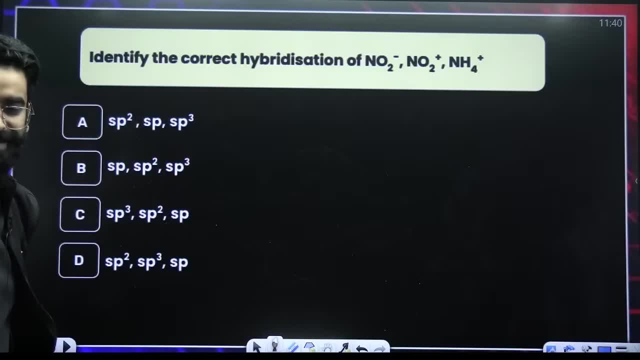 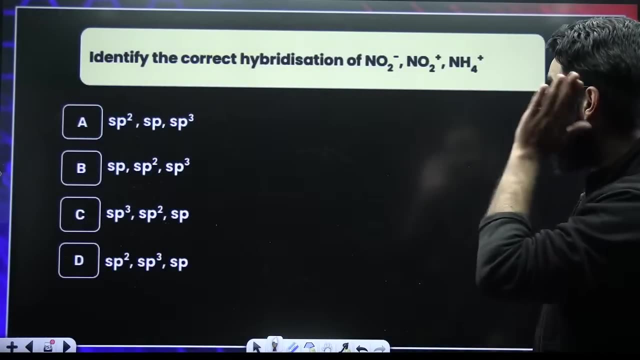 recent J-Mains question. This is the recent J-Mains question. Kill it. Identify the correct hybridization of NO2-2, NO2+, NH4+. What do you think? What do you think about this one? Again, you should be in a position to solve this question. 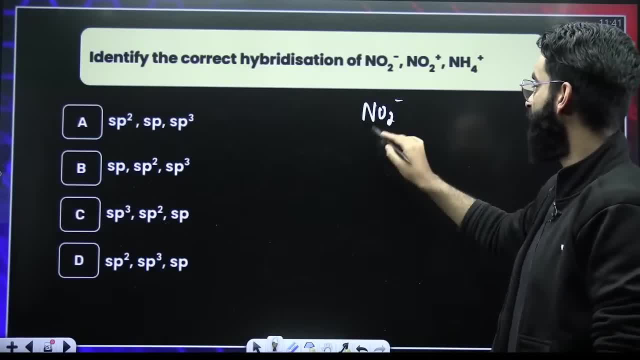 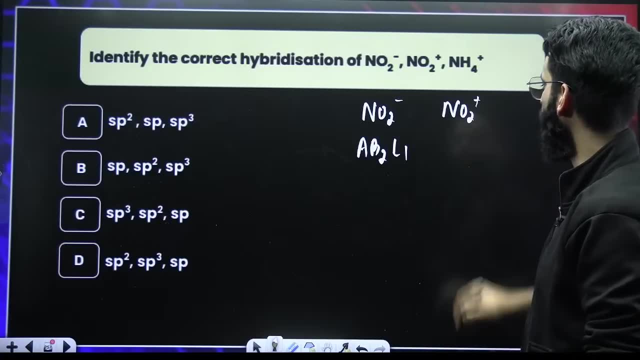 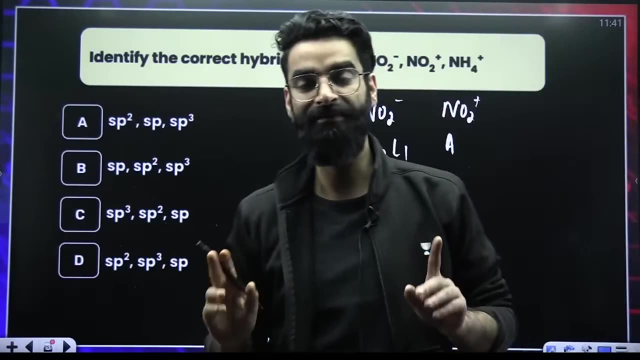 If you talk about NO2-2,, get its type. The type of this one is AB2.. AB2L1. NO2+: Get the type of the molecule And you know how do we get the type. Do you remember? how do we get the type of the molecule? 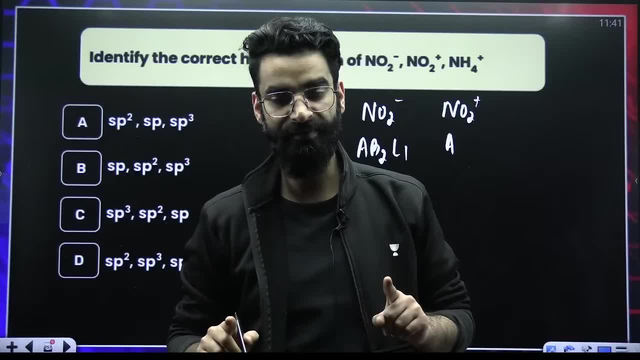 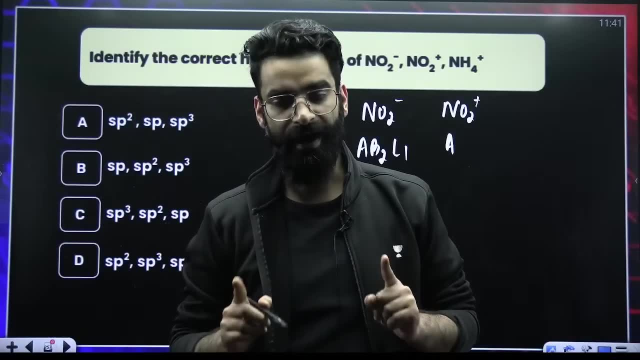 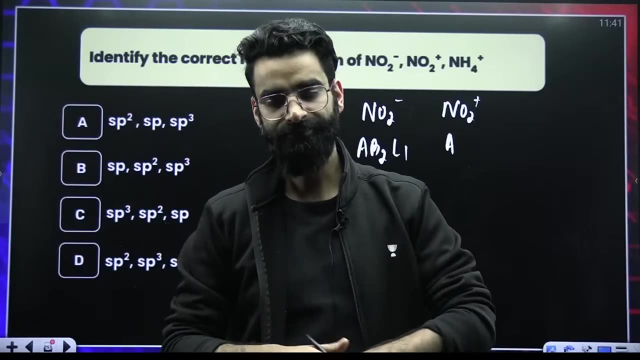 Just tell me that first. Do you remember that? How do we get the type of the molecule? Do you remember? how do we get the type of the molecule, the molecule? I'm asking you quickly Say it. Do you remember? how do we get the type? 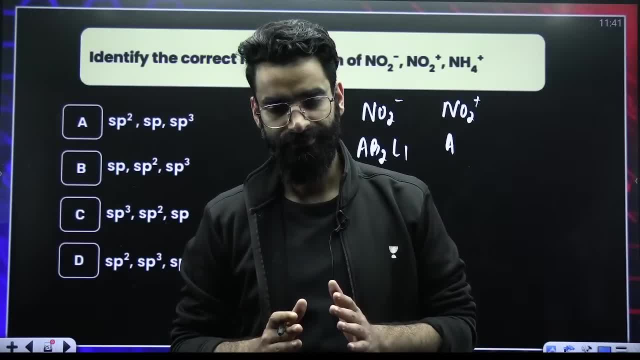 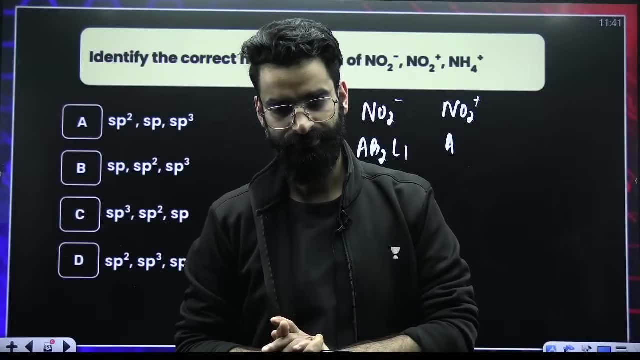 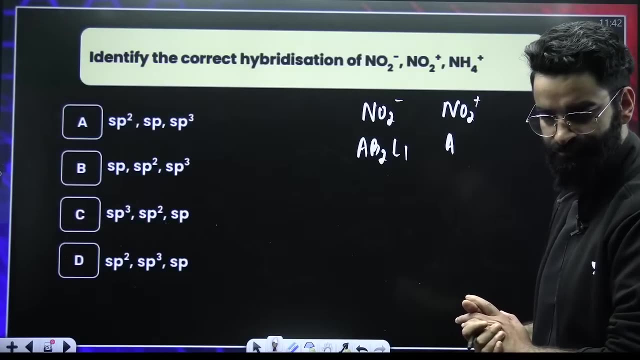 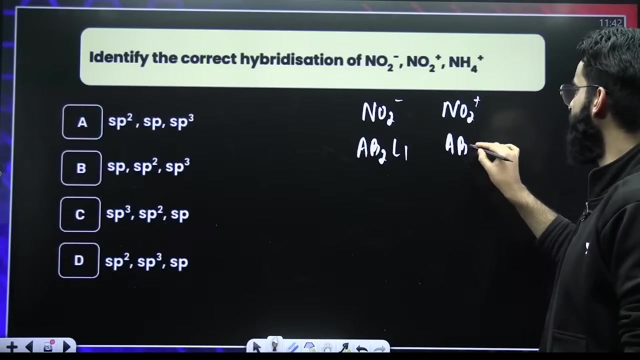 of the molecule. Someone is asking me how to find the lone pair. Watch the yesterday's session, You'll get to know. Look at this one. This is AB2L0.. NH4 positive: This is AB4L0.. Hybridization 2 sigma 1 lone. 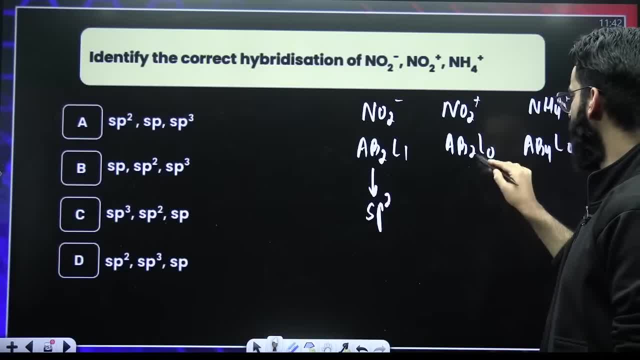 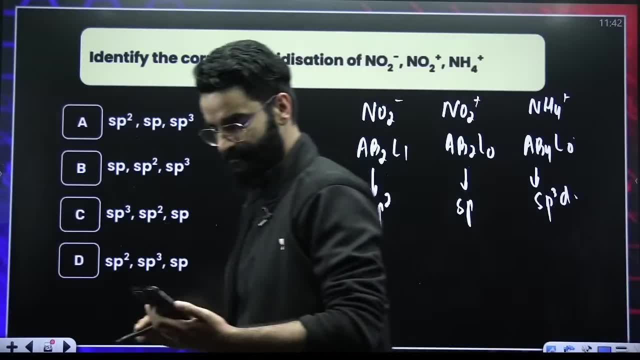 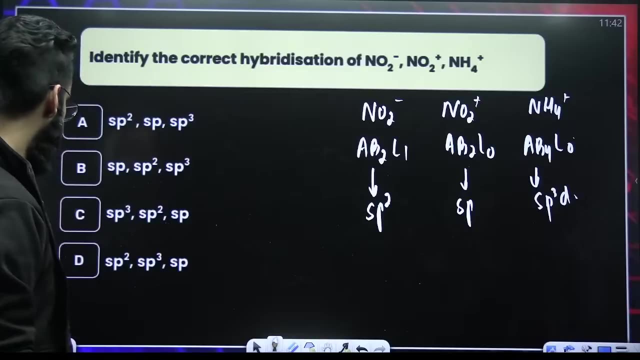 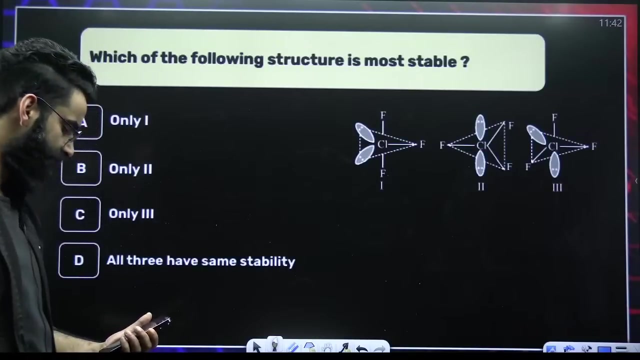 pair: 2 plus 1,, 3.. SP2.. 2 plus 0, 2. SP, Right, And this is SP3D. Now, what is the answer? You can easily check it. Yeah, Perfect. What about this one? What about this one? What about this one? Which of the following? 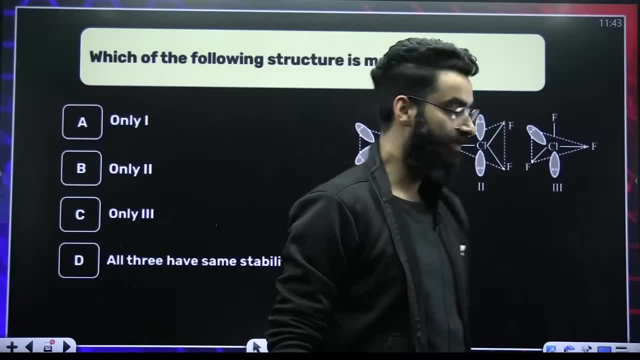 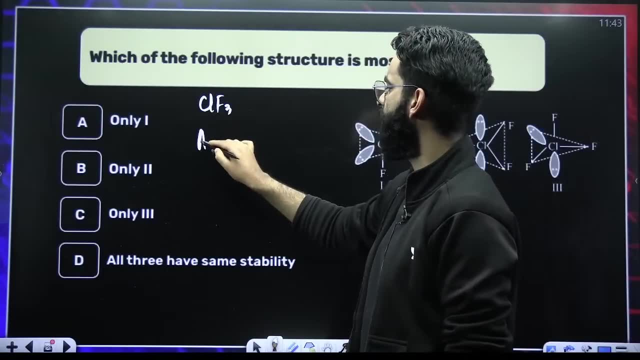 structure is more stable, More stable. We are basically given with CLP. We are given with CLF3 molecule. Right, We are given with CLF3 molecule. If you look at the CLF3 molecule, the structure, the type will be AB3L2 and it has to be T-shaped It. 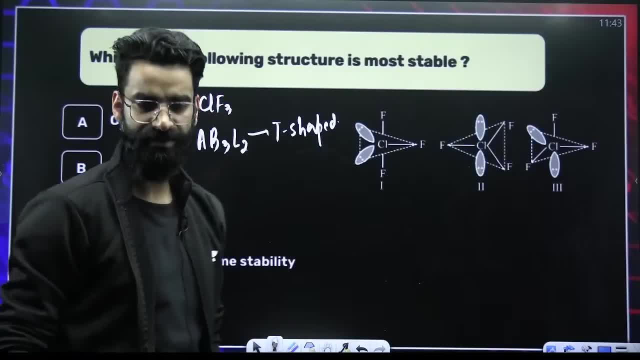 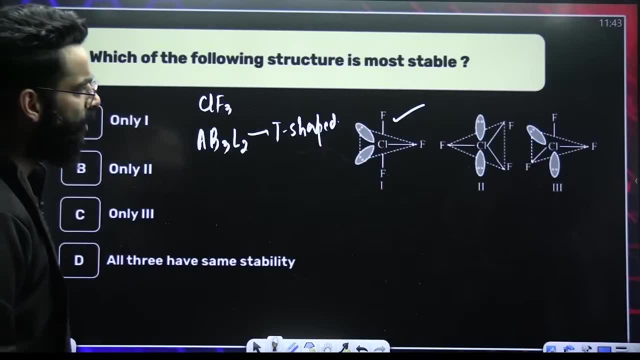 has to be T-shaped. Discussed yesterday. It has to be T-shaped. Discussed in yesterday's marathon. Which one is T-shaped? It's option A, Right, It is option A, Perfect, It has to be T-shaped. 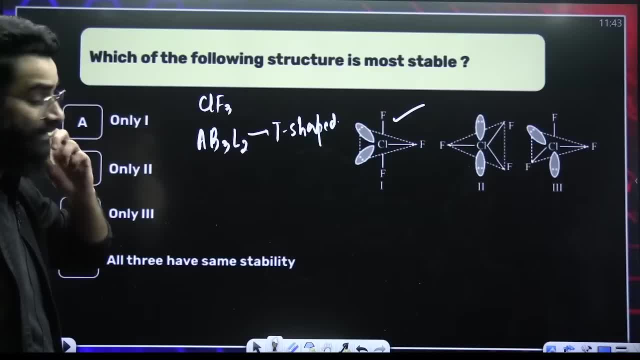 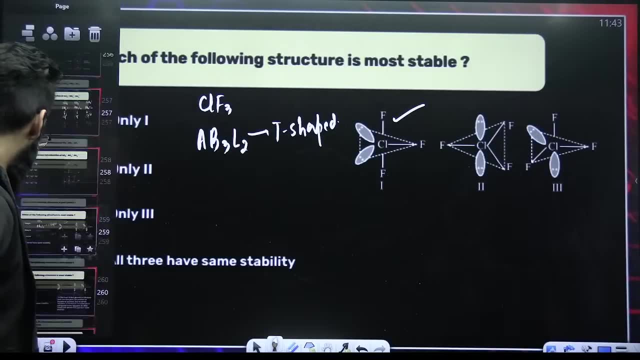 CLF3.. 3 sigma 1, 2 lone pairs. Right 3 sigma 1, 2 lone pairs. It has to be T-shaped. T-shaped structure is the one wherein it has got minimum repulsions and maximum stability. Only one. 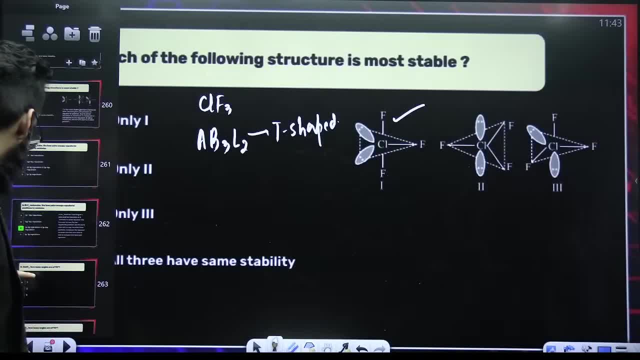 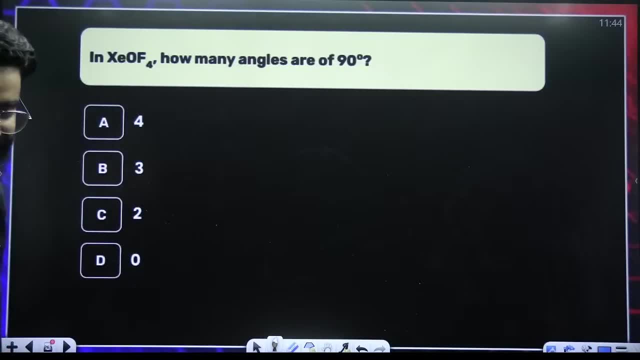 Only one. This question is tricky. Can you let me know the answer of this one? Give it a try, Let me see what you will think about this one. Quick, This is Quickly. What do you think? What do you think? 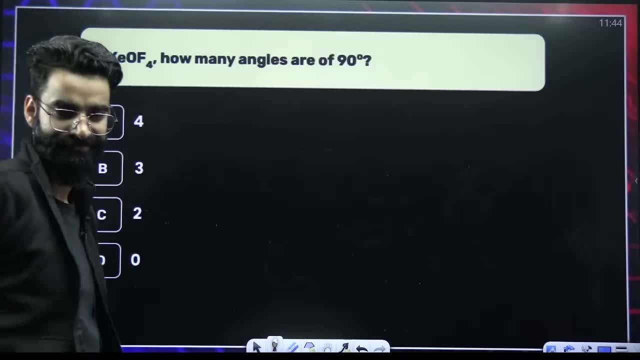 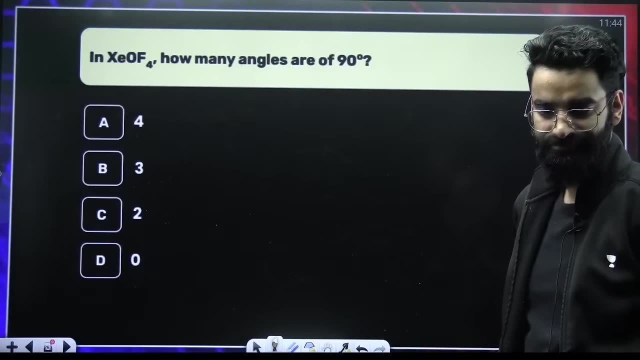 First of all, what do you think about something like this? Well, what do you think? The answer is YES, ZERO. Right, Mrый question was what you think, not what you think. YEE worry, See, guys, This is XEOF4.. First of all, let me tell you: answer is zero. Why? Have a look. 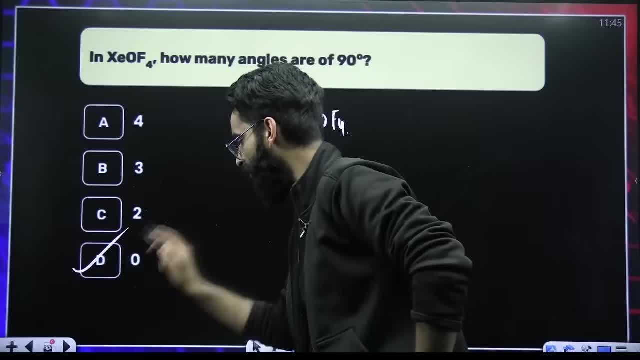 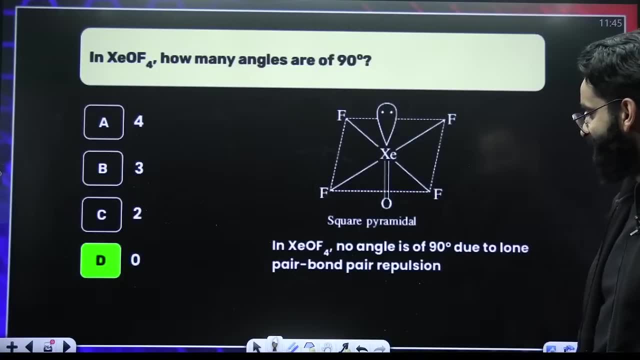 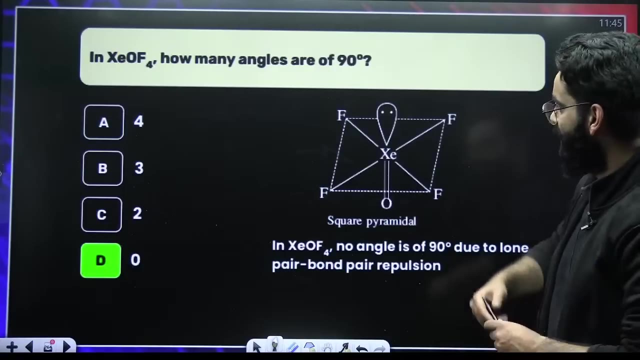 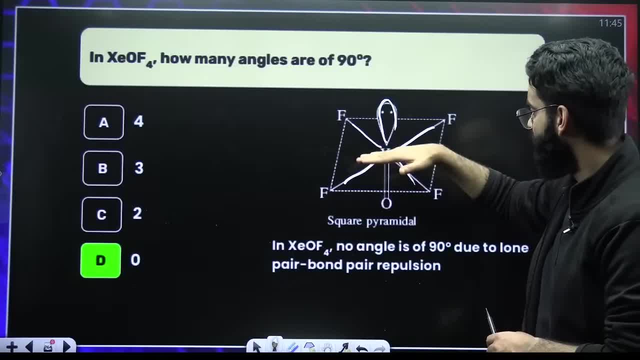 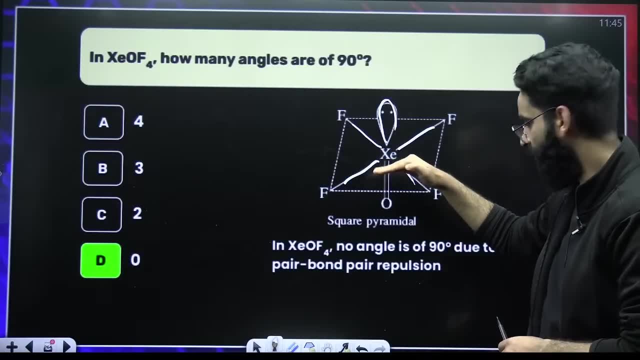 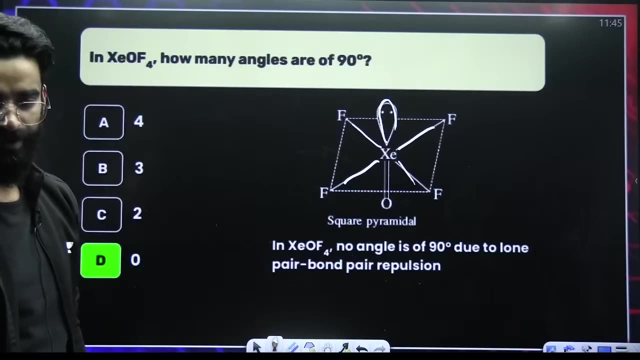 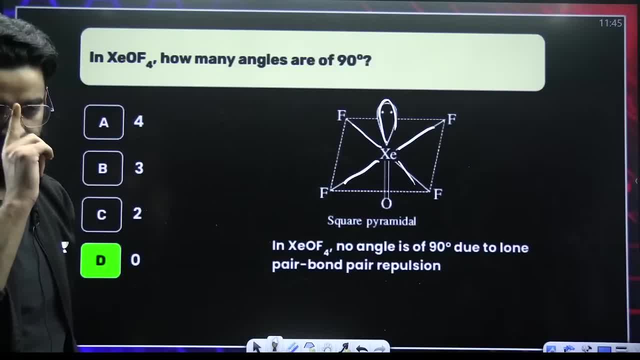 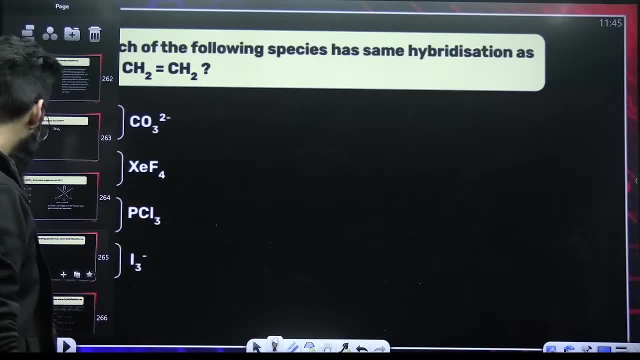 bond pair and loan pair. there will be no angle, which should be 90 degree here. Remember this particular case. it's a special case. okay, remember it Quick. what do you think about this one? What do you think about this one? Which of the following species have same hybridization, same hybridization as that of carbon in CH2CH2?? In CH2CH2, carbon has got sp2 hybridization. Now, where do you see sp2 hybridization? Where do you see sp2 hybridization? 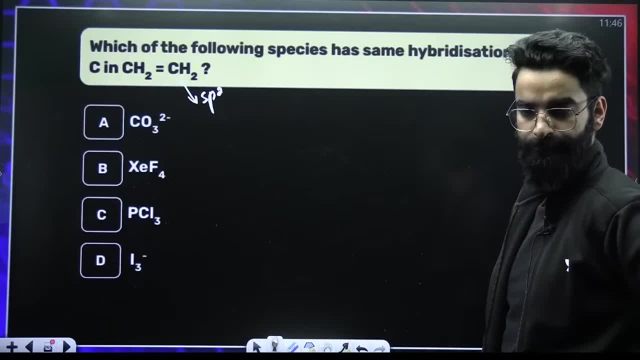 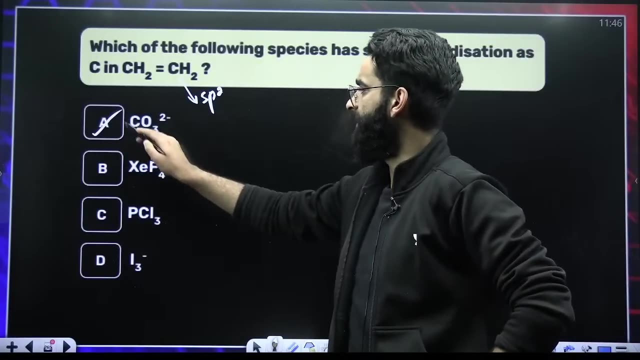 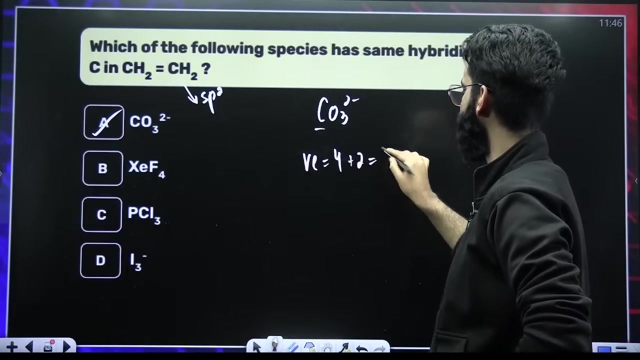 Where do you see sp2 hybridization Quickly? If you talk about the first one, let me show you over here. CO3 di-negative right valence electrons of carbon are 4, there is a negative charge, 4 plus 2, 6, sigma bonds are 3, sigma. 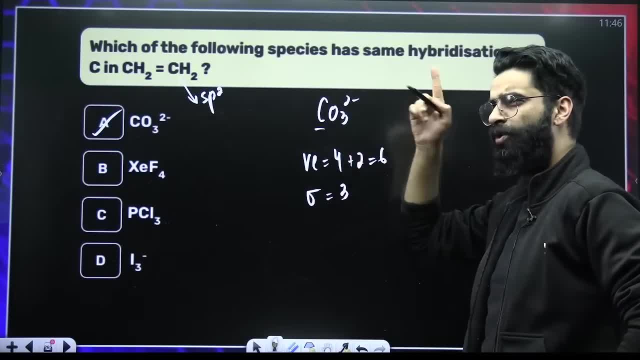 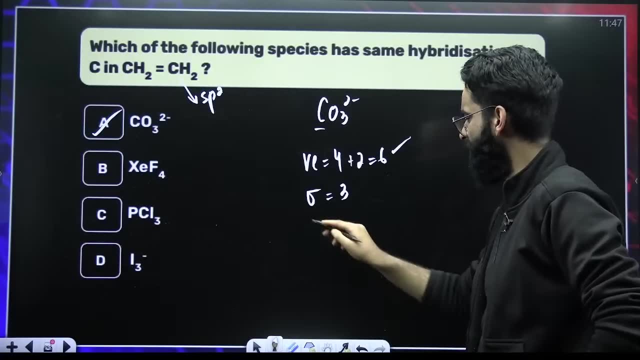 bonds are 3.. Now is there any loan pair? oxygen is di-valent, so consider two bonds. so 3,, 2's are 6,, 6, 6 bonds. So all the 6 valence electrons have been. understand it, they have been used, so loan. 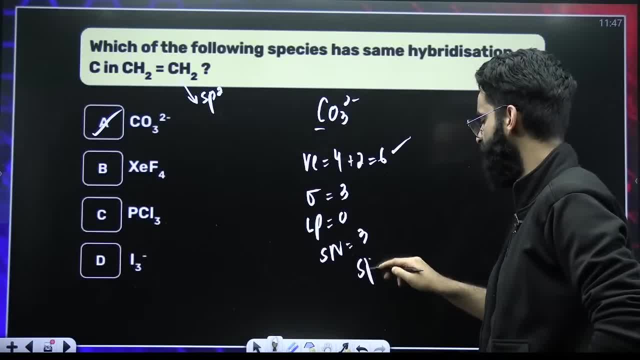 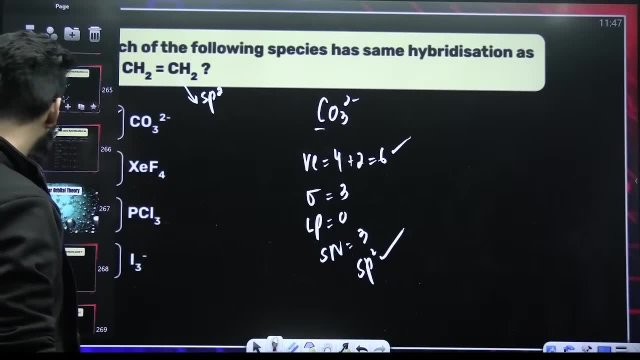 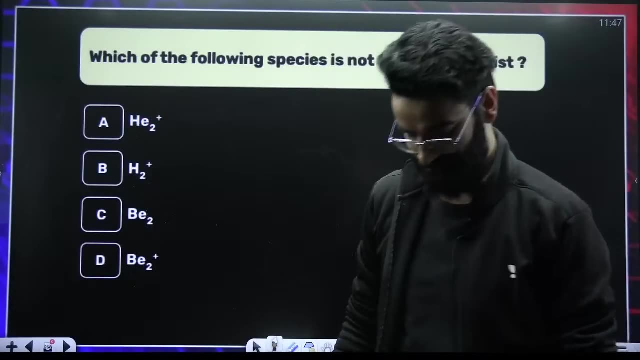 pair 0, steric number 3 plus 0 is 3, hybridization is sp2,. yeah, hybridization is sp2.. Which of the following species is not expected to exist does not exist? Which species does not exist? 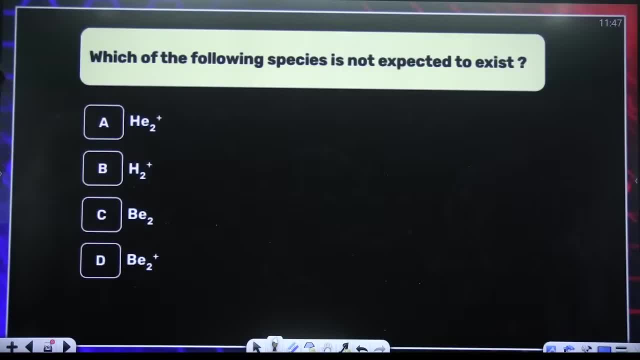 The one Which species does not exist? The one? The one whose bond order will be less or equal to 0,. the one whose bond order will be less or equal to 0,. less or equal to 0, which one is that? 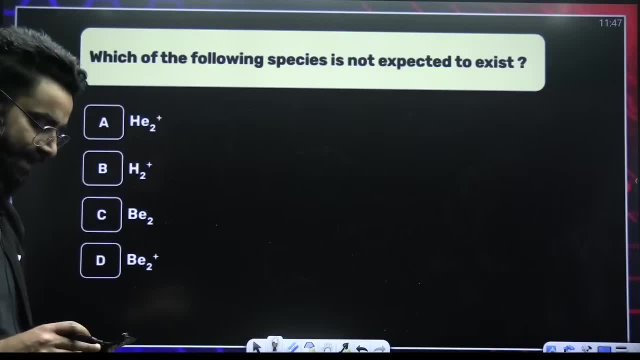 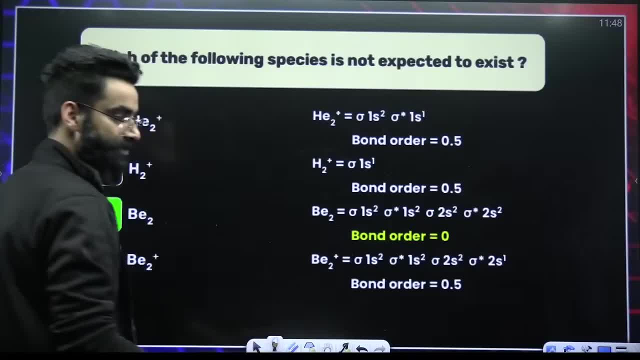 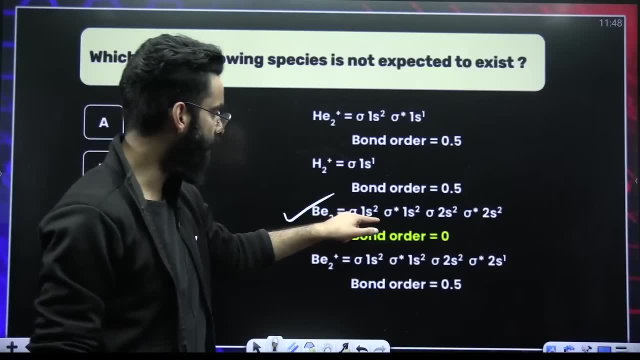 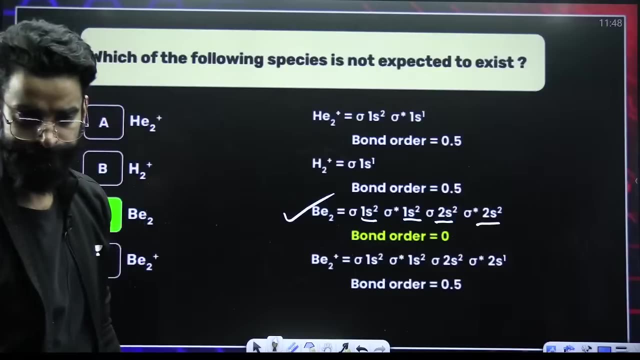 And look at the configurations. If you write the molecular orbital configurations the way I showed you in yesterday's marathon, If you write the molecular orbital configurations, B2 has got 4 bonding electrons and 4 anti-bonding electrons. If you write the molecular orbital configuration minus 4 divided by 2 comes out to be 0, yes, 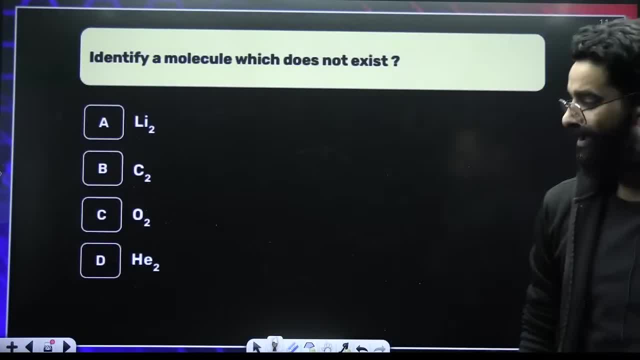 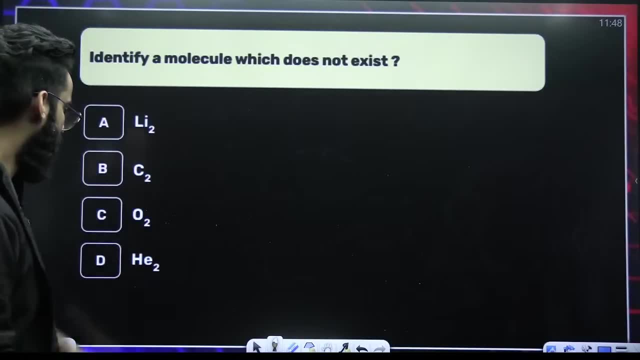 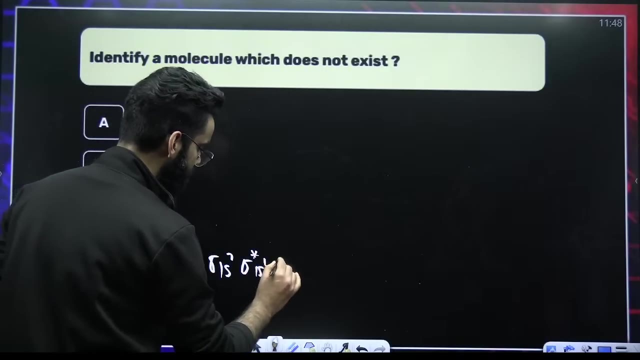 Which of the following does not exist? Again, the similar type of question. Again, you will be writing the molecular orbital configuration. Again, you will be writing the molecular orbital configuration. If you talk about He2, there are total 4 electrons. Its molecular orbital configuration is sigma 1s2, sigma star 1s2, sigma 2s2, sigma star. 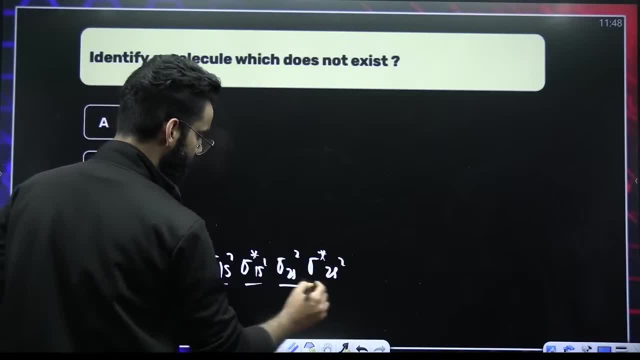 2s2.. Right, So how many bonding electrons are there? 4 bonding, 4 anti-bonding, 4 bonding, 4 anti-bonding. Bond order will be 0.. Bond order will be 0.. 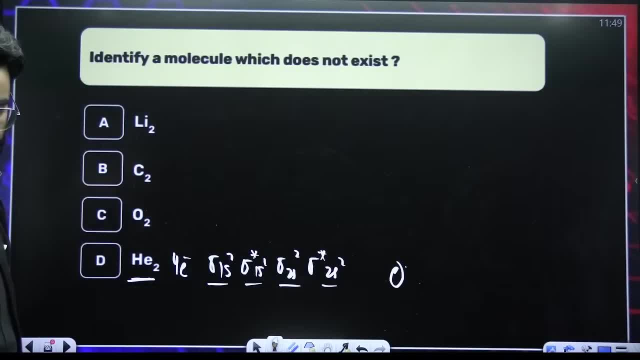 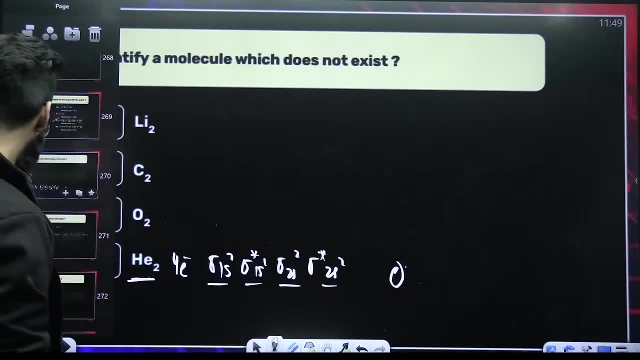 4 bonding, 4 anti-bonding, Bond order will be 0.. Right, Yeah, Perfect. So bond order is 0. in the fourth case, Which of the following is paramagnetic? This sort of a question I told you yesterday. 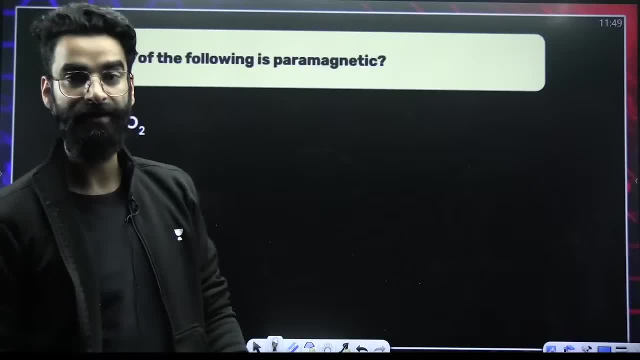 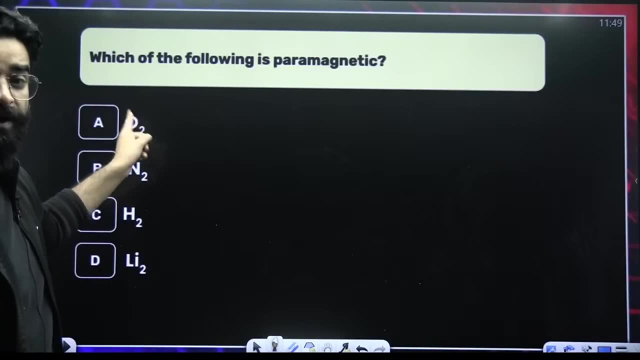 If you remember How do we check whether the species is paramagnetic or diamagnetic? Write the molecular orbital configuration. If there is unpaired electron, If there is unpaired electron. If there is unpaired electron it's paramagnetic. If you write the molecular orbital configuration of O2, there will be two unpaired electrons. 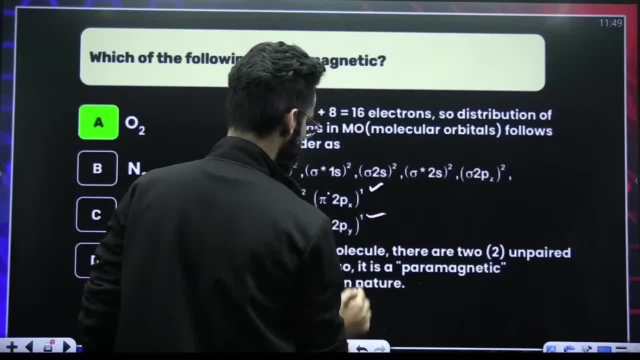 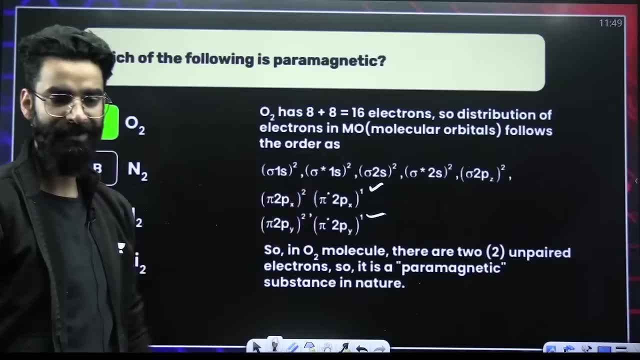 There will be two unpaired electrons. Have a look, These are the two unpaired electrons: One in this and one in this Right, One in pi star 2px and one in pi star 2py. So there are two unpaired electrons. 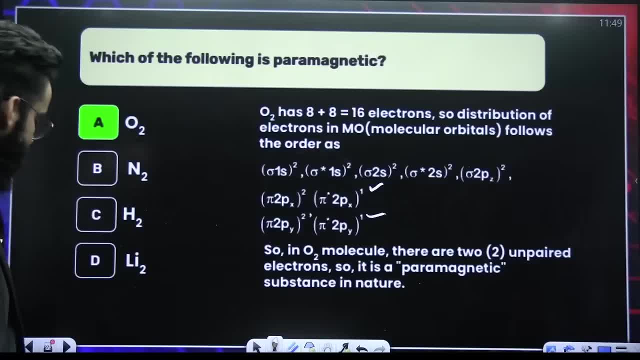 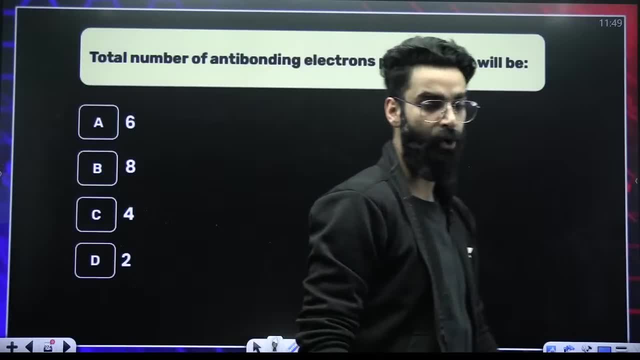 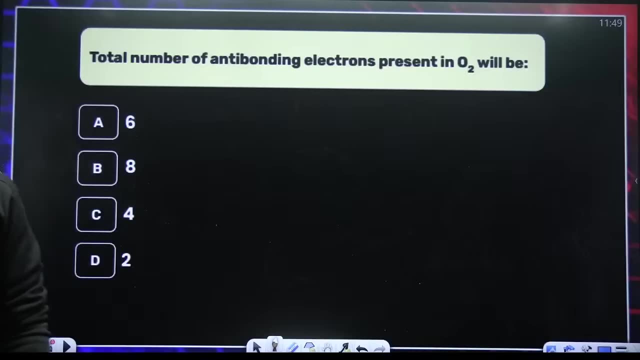 So it has to be paramagnetic. It has to be paramagnetic, Right, It has to be paramagnetic. Total number of anti-bonding electrons present in O2 will be. Total number of anti-bonding electrons present in O2 will be. 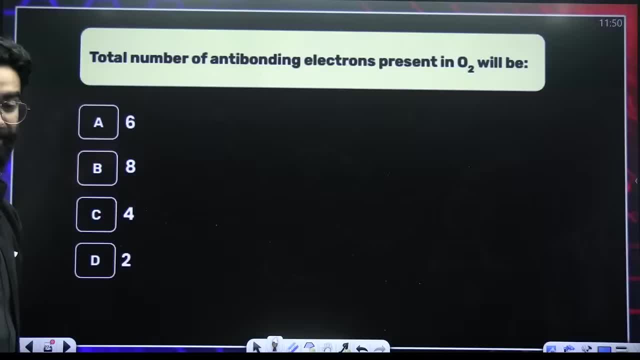 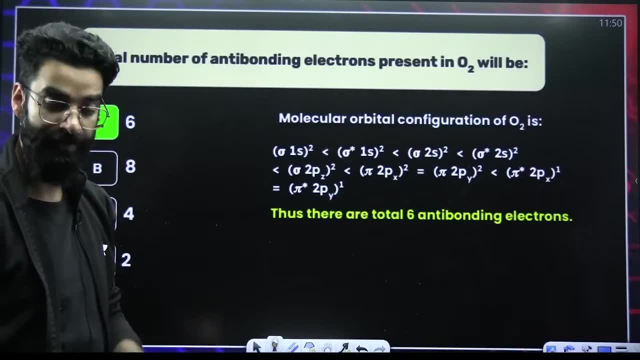 Total number of anti-bonding electrons present in O2 will be: Again, you will have to write the molecular orbital configuration. After writing the molecular orbital configuration, now you have to calculate the anti-bonding electrons Two, four, five and six. 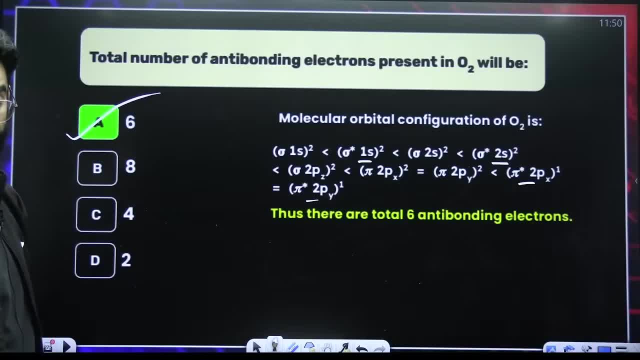 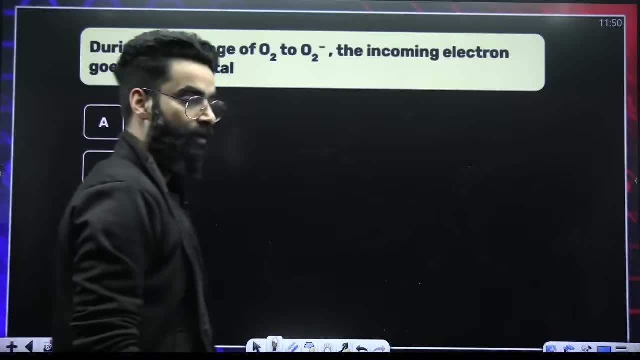 So there are six anti-bonding electrons Total Six total anti-bonding electrons present in O2.. Right Now, the other thing that you do is you ask now what represents an O2.. I believe it is clear. When you convert O2 into O2 negative, how do you convert O2 into O2 negative? 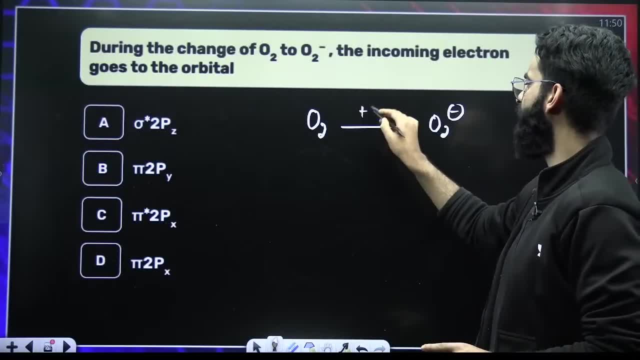 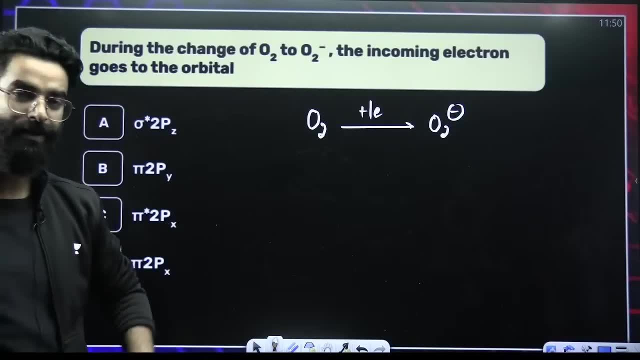 How do you do that? You give one electron to O2.. You give one electron to O2, it gets converted to O2 negative. It gets converted into O2 negative. Now, where that electron goes, in which molecular orbital that electron goes, that electron goes. 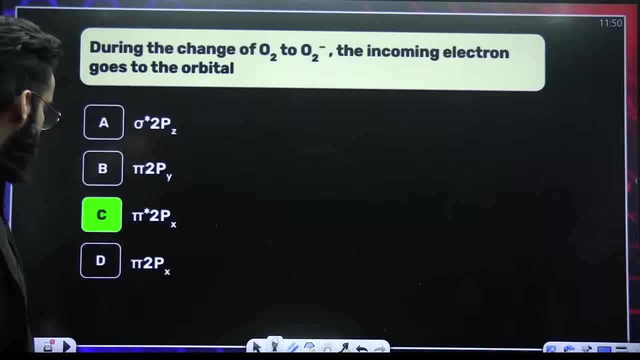 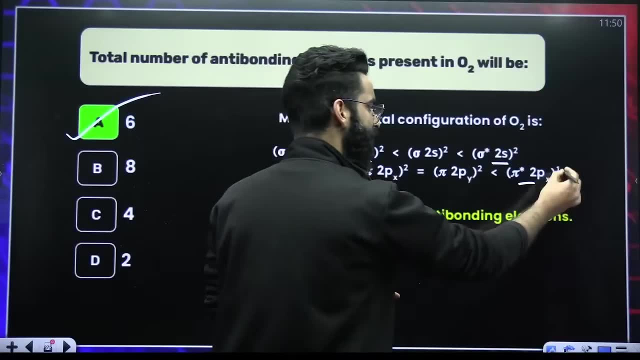 to pi star 2 px molecular orbital. Right, That goes to pi star 2p x molecular orbital. This is the molecular orbital configuration of O2.. Now the extra electron. one more electron will go here, Then one more electron will go here. 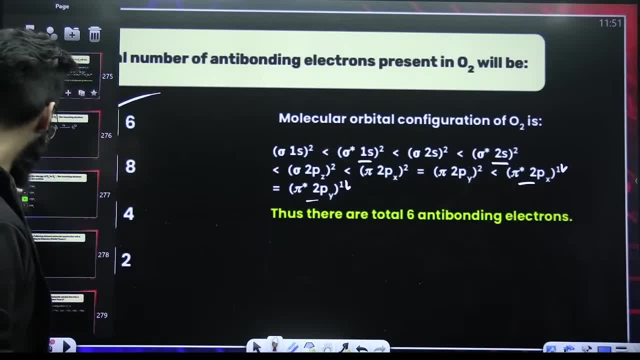 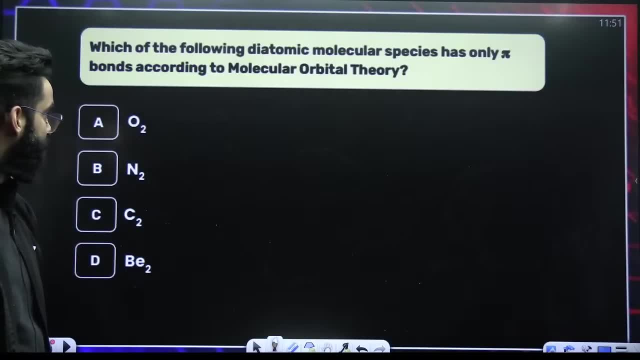 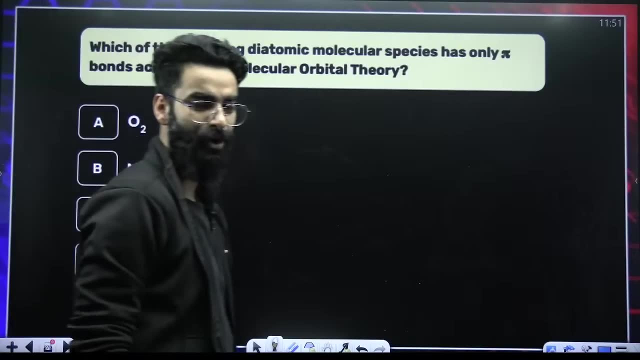 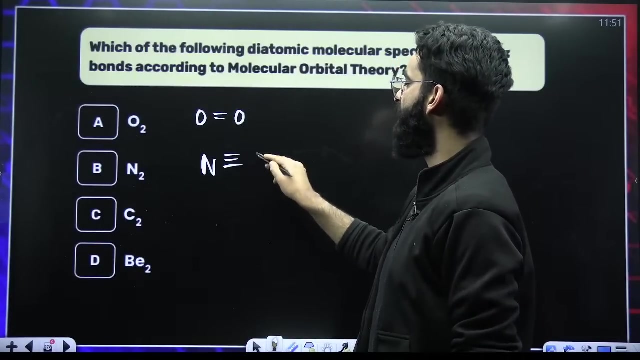 Got it Perfect. I hope it's clear. I hope it's clear This question. yesterday I have told you which of the following, which of the following diatomic molecule species has only pi bonds, Only pi bonds. This is discussed yesterday. O2, 1sigma 1pi, 1sigma 2pi. both are pi here. both are pi. 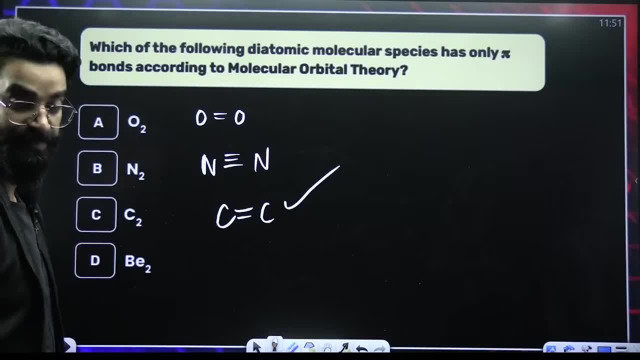 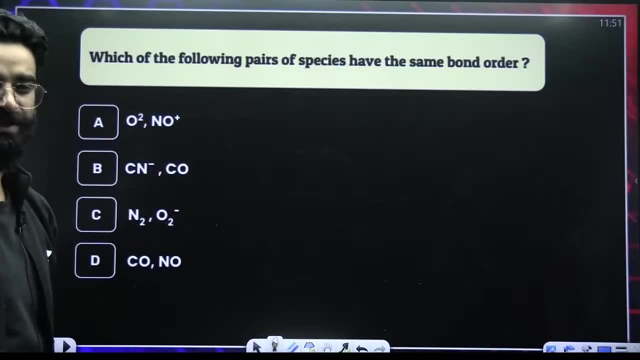 here in C2, right? This was explained by MOT. if you remember Which of the following pair of species have same bond order. Iso-electronic species have got same bond order. Iso-electronic species: Carbon: 6 electrons, 7 electrons. 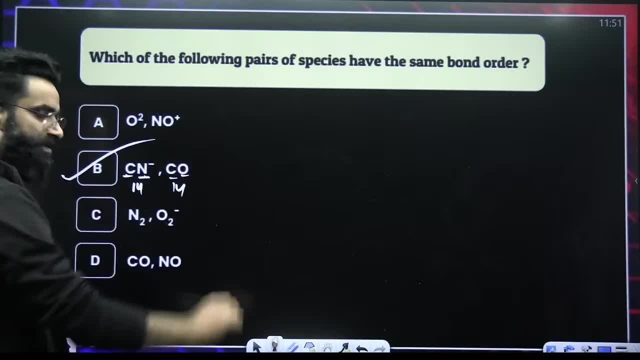 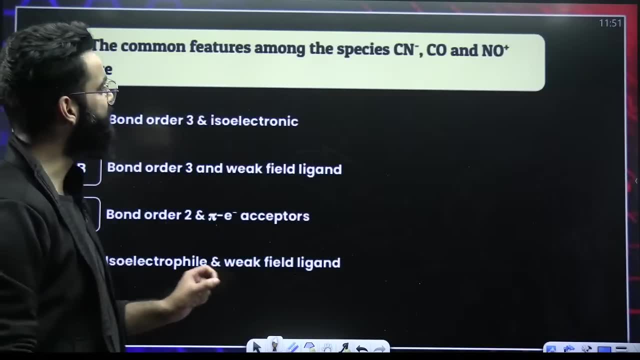 6 plus 6 plus 1, 14.. So 8 plus 6, 14,. isoelectronic species- bond order: same. Iso-electronic species- bond order: same. The common features: the common features among the following species: Cn- Cono+. what do? 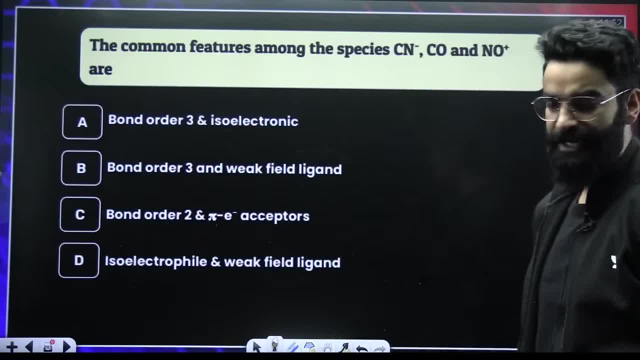 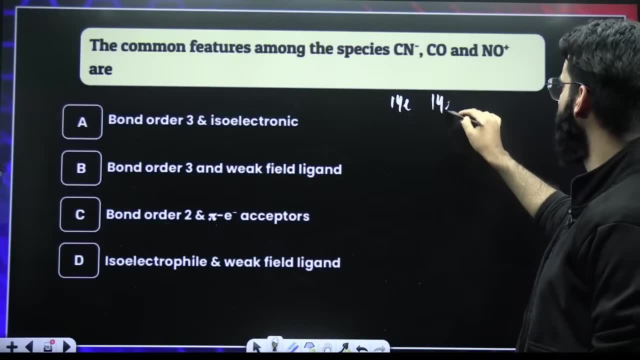 you think? What do you think? Cn- Cono+ Cn- Cn- 7 plus 6 is 13 plus 1.. This is a 14 electron species. this is a 14 electron species. this is a 14 electron species. 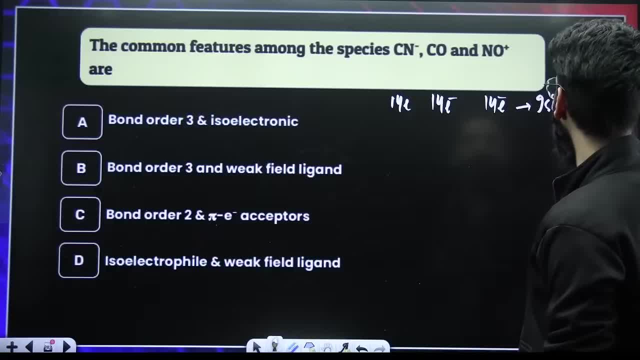 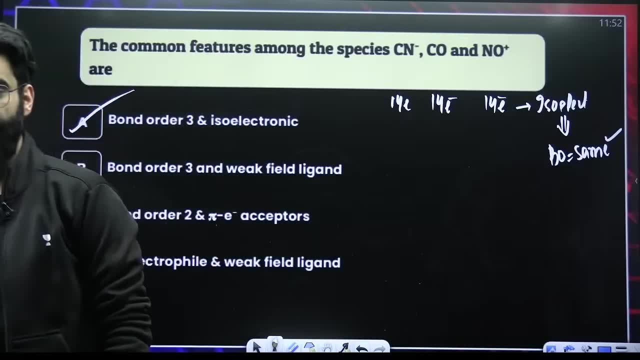 So first of all they are isoelectronic, And isoelectronic species have got same bond order. Iso-electronic species have got same bond order And you know 14 electron species. they have got the bond order of 3.. 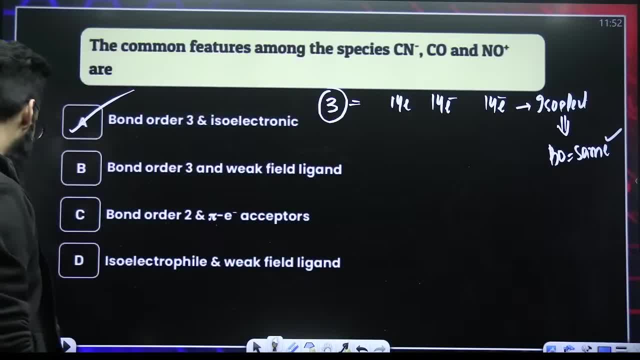 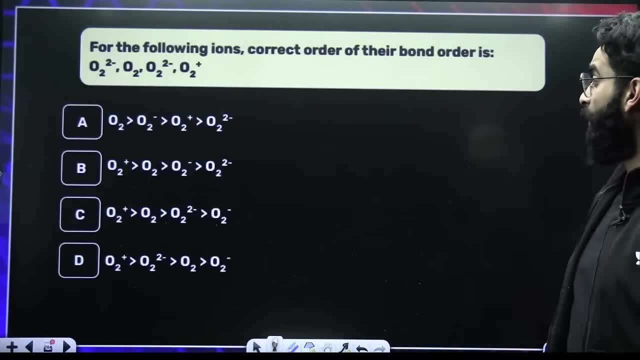 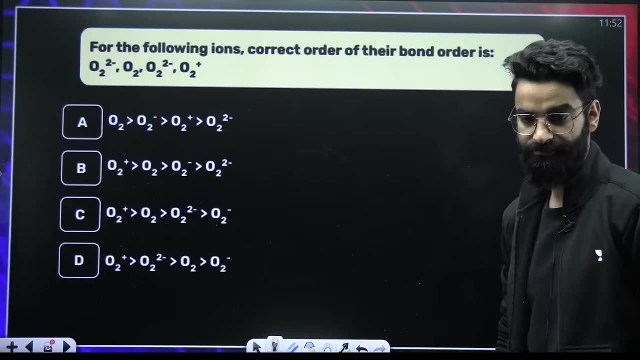 14 electron species, all the 14 electron species. they will be having bond order of 3.. Right You are given with following species: correct order of their bond order. Correct order of their bond order. One trick I gave you yesterday, if you remember. 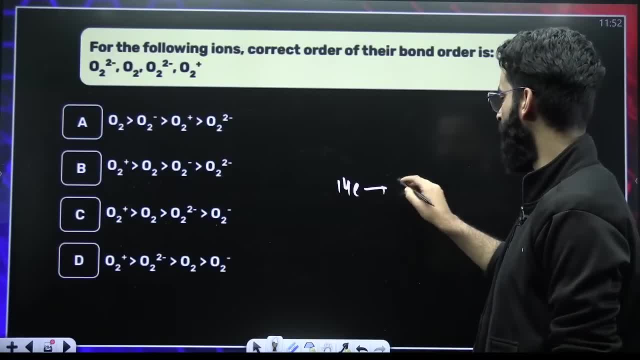 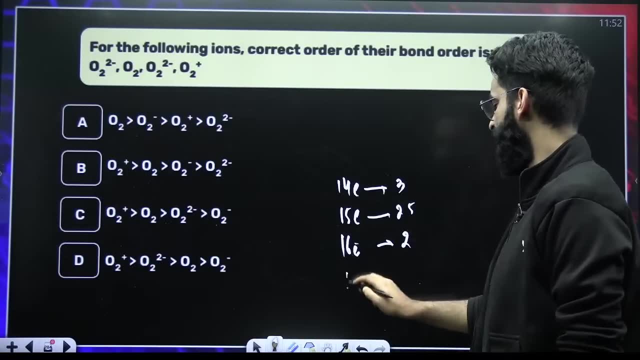 One trick: I gave you yesterday 14 electron species. they have got bond order of 3, 15 electron species, 2.5, 16 electron species, 2, 17 electron species- what? 1.5, 18 electron? 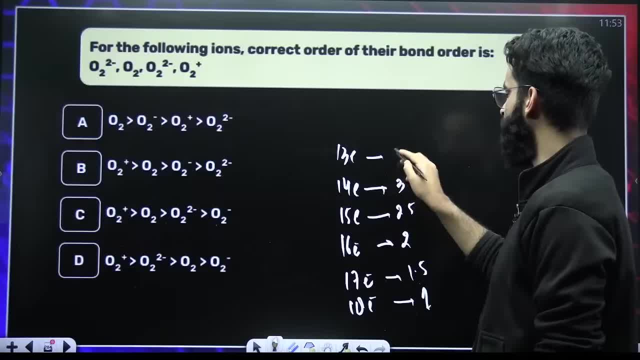 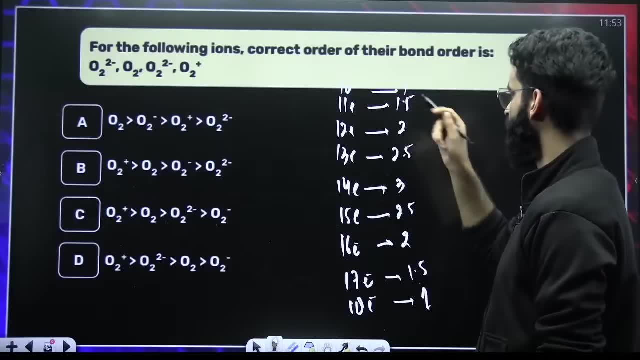 species? what? 1.. 13 electron species 2.5,. 12 electron species 2, 11 electron species 1.5,. 10 electron species 1. Right, That is the thing I have given you yesterday. 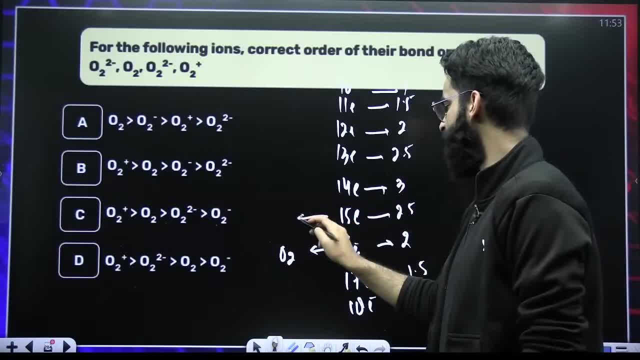 Are you isoelectronic right? So all of this is going in the same, But right now I am adjusting the way. So in this reading you will see thatDEV A cute right. See him, says he. he says O2 is 16 electron species. 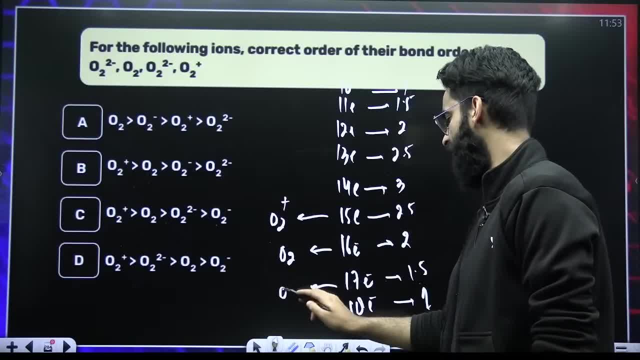 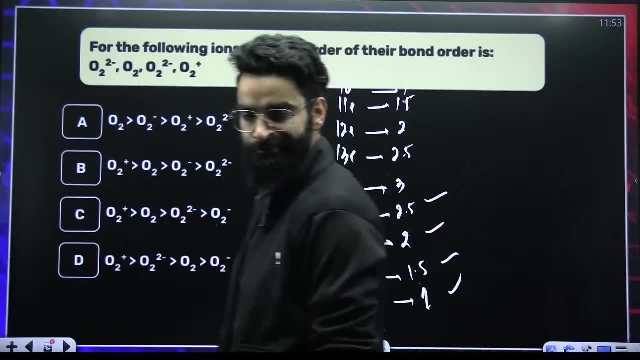 O2 is 16 electron species, O2 positive is 15 electron species right. O2 negative is 17 electron species And O2 di negative is 18 electron species. Now arrange them on the basis of their bond orders Done. 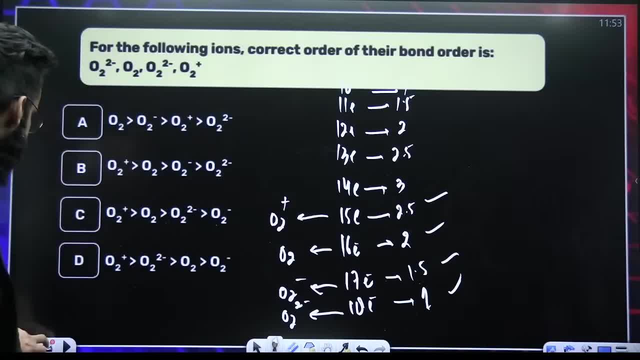 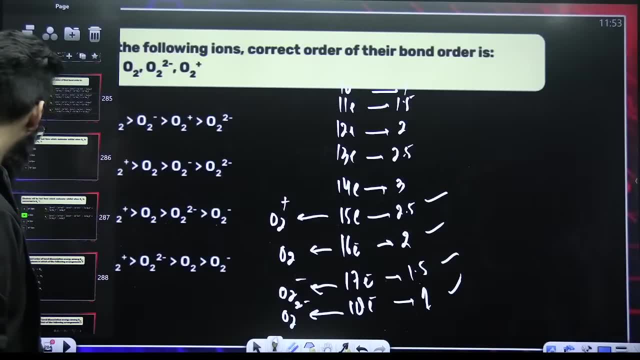 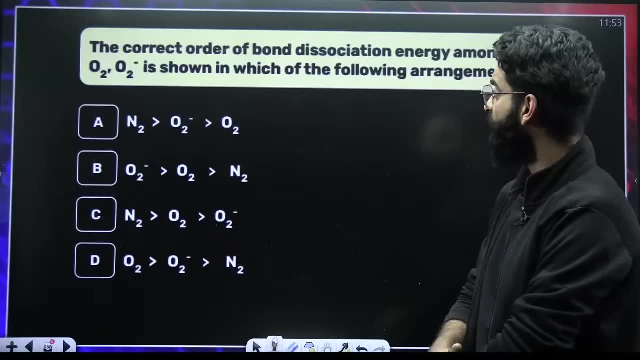 Simple: Arrange them on the basis of their bond orders. We are done here. OK, We are done here. We have to write the order of what We have to write: the order of bond dissociation energy. We know bond order is strictly proportional to bond dissociation energy. 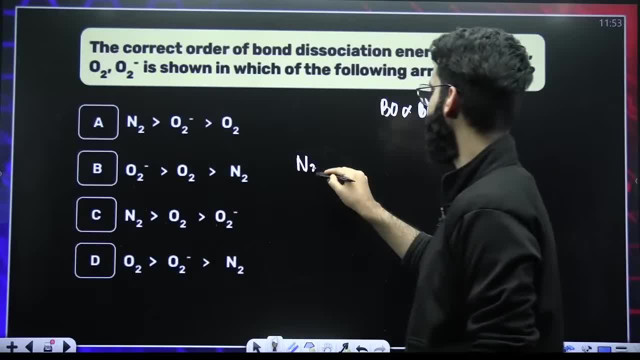 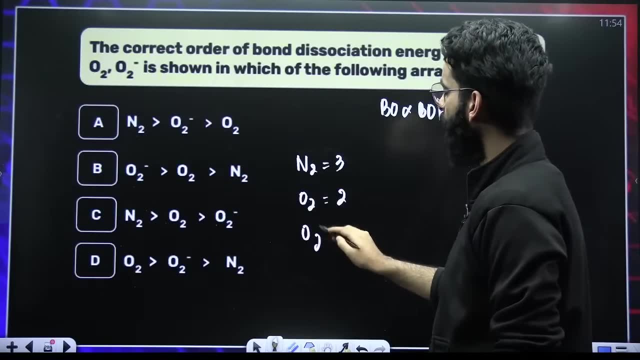 So calculate their bond orders. Bond order of N2 is 3.. Bond order of N2 is 3.. Bond order of O2 is 2.. Bond order of O2 negative. Bond order of O2 negative will be 1.5.. 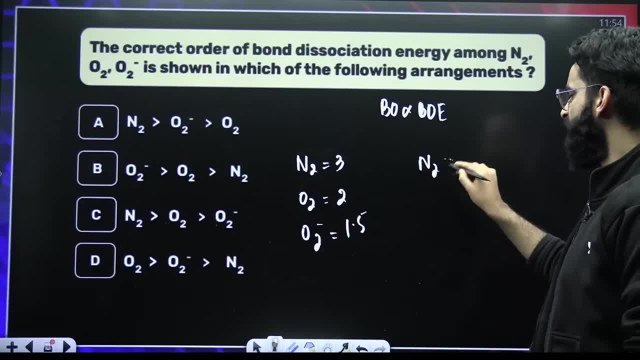 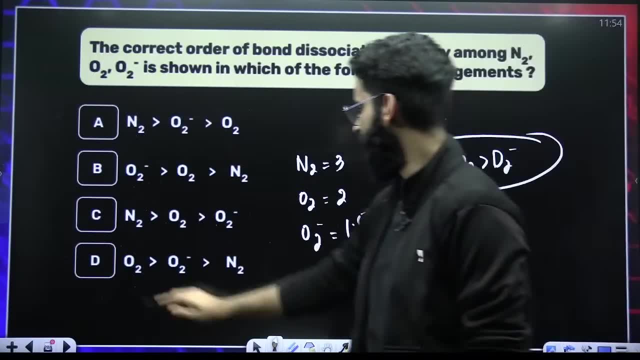 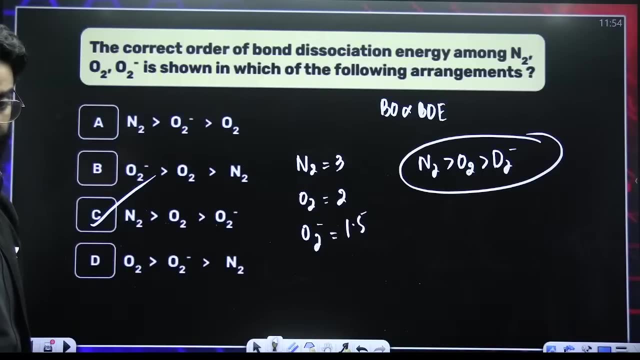 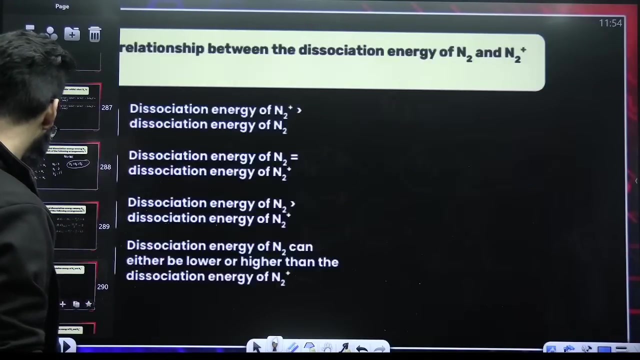 Perfect. Whatever is the order of bond order, same as the order of the bond dissociation energy. Perfect This. N2 greater than O2 greater than O2 negative. Perfect Guys, I want you to be active in the chats. You have to solve the questions in very lesser time, by the way. 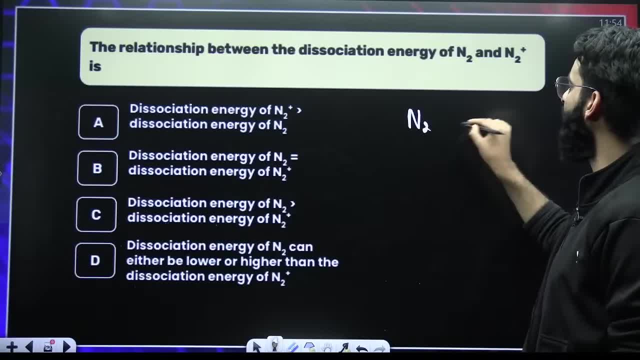 Relationship between the bond dissociation energy and bond dissociation energy. The bond dissociation energy, The bond dissociation energy, is the energy of N2 and N2 positive N2 and N2 positive Right. Here the bond order is 3 and here the bond order is 2.5. 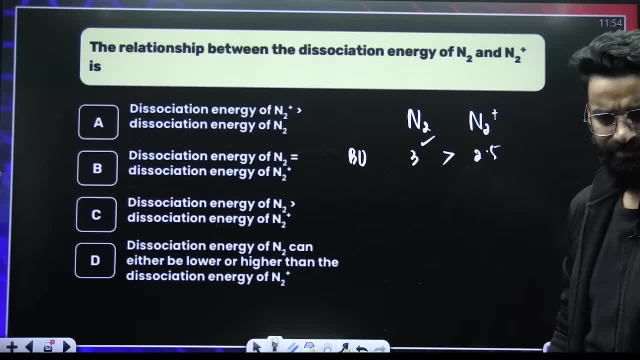 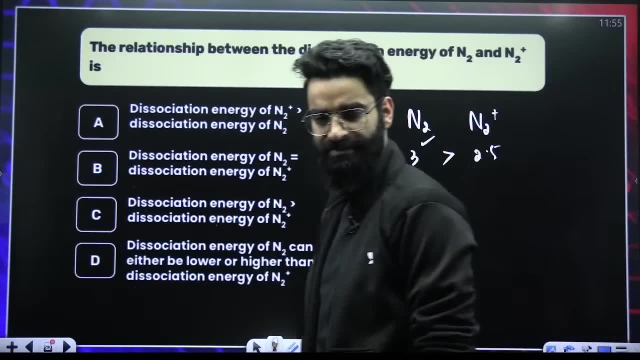 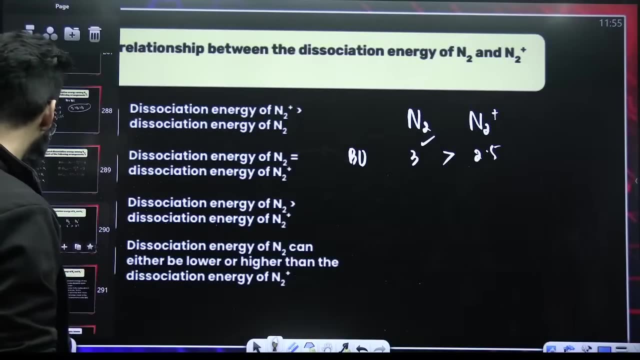 Bond dissociation energy. here it will be more Simple: More the bond order, more the bond dissociation energy. That's all. Yeah, That's all, That's all, Okay, Done, Okay, Alright, Alright, Okay. 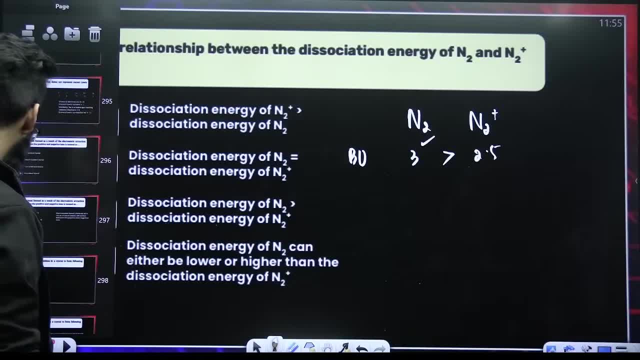 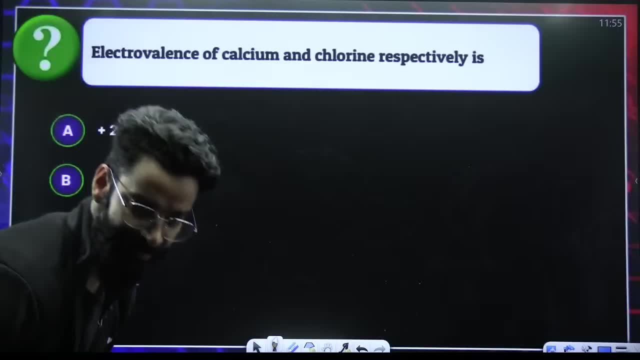 Just a second. These are the repeated questions here. Just a second, Okay. Electrovalence of calcium, Electrovalence of calcium and chlorine. One simple and basic question which all of you can solve easily: Electrovalence of calcium and chlorine. 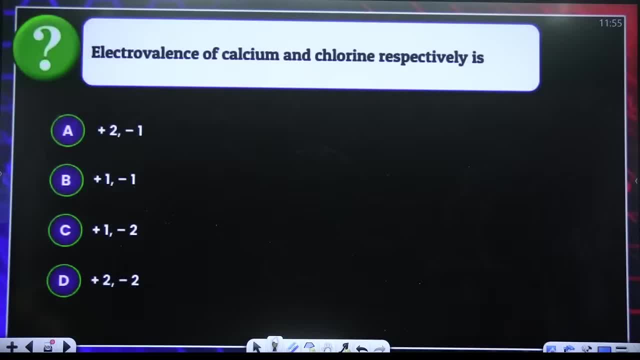 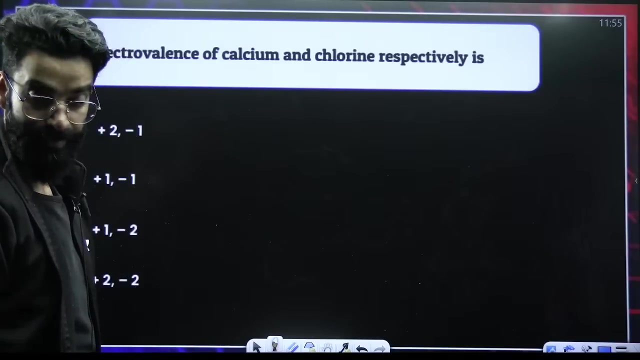 What do you think? Calcium: It belongs to group 2. So 2 electrons in the outermost shell, Right Chlorine, Group 17. 7 electrons in its outermost shell. Electrovalence of calcium and chlorine are: 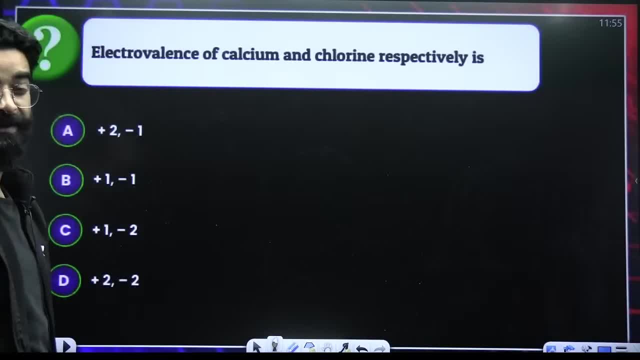 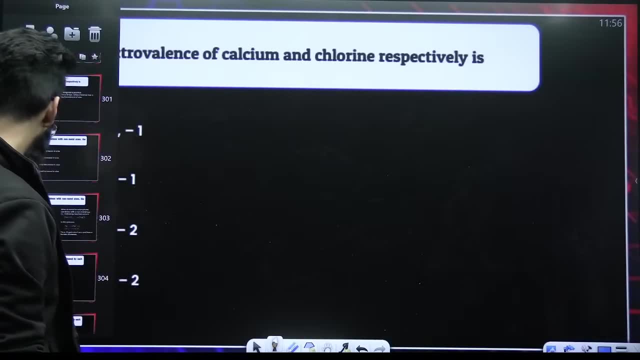 Calcium is group 2. So it will show plus 2.. Fluorine, I mean chlorine, is group 17.. It will show minus 1.. So plus 2 minus 1 is the answer. Plus 2 minus 1 is the answer. 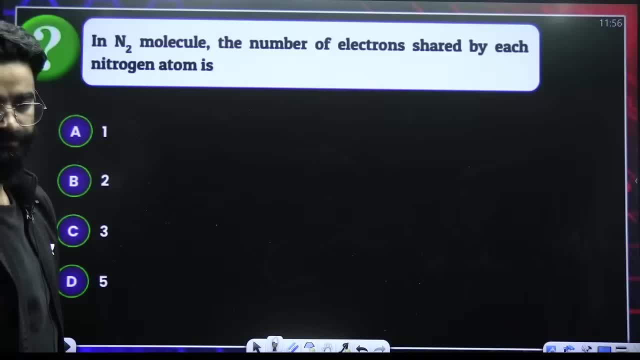 In N2 molecules, the number of electrons shared by each nitrogen atom. Guys, we will complete this session in very lesser time. okay, You know what kind of speed we are having to solve the equations. I think till now we have solved almost like 80-90 equations in less than an hour. 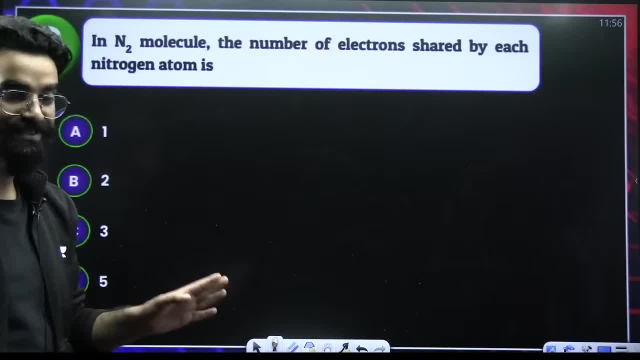 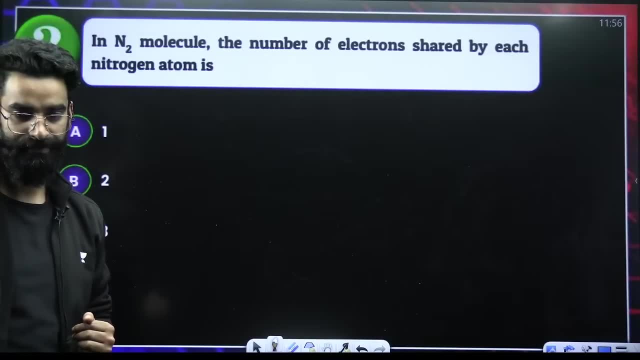 Perfect Right. So don't worry, I am not going to exceed the session. I will finish it quickly, as soon as possible, But I want your support in the chats continuously. So let's keep this session short and crisp. only Let's complete. 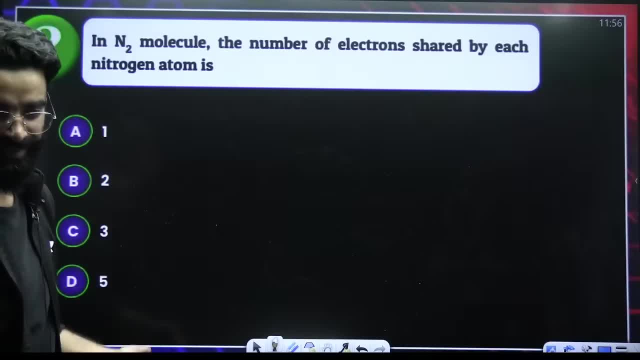 Because whatever. See, I don't need to explain anything here, Because all the things are explained in the yesterday's session. Why would I explain the same things again? Yeah, So let's be quick, Let's be very fast, Let's try to solve the equations in less than 10 seconds. 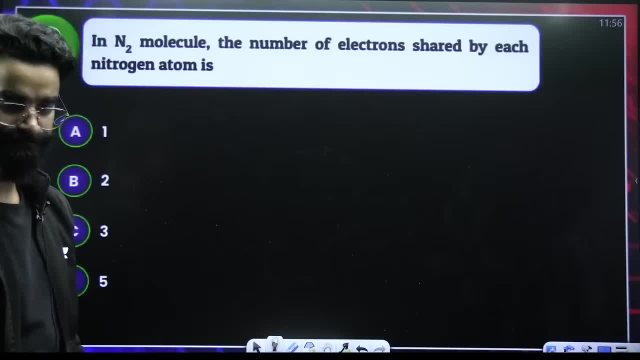 Okay. In N2 molecules, the number of electrons shared by each nitrogen atom. 3. Right Discussed Among the following: The electron deficient compound- Electron deficient- Electron deficient. The electron deficient compound- Electron deficient- Electron deficient. 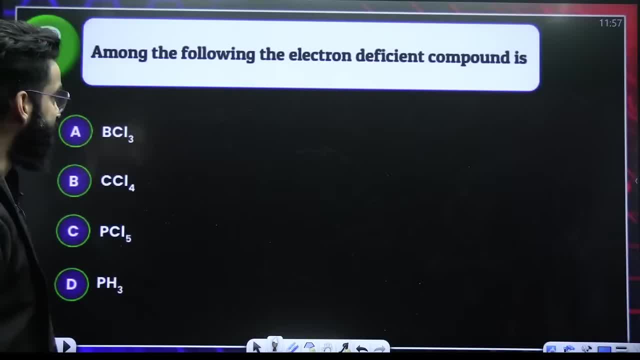 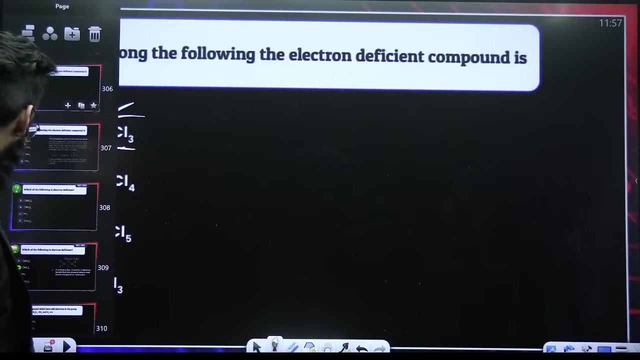 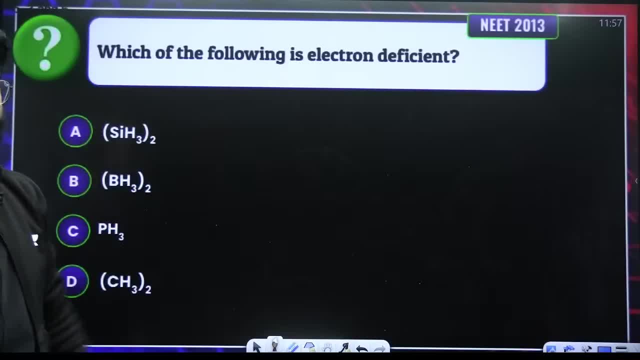 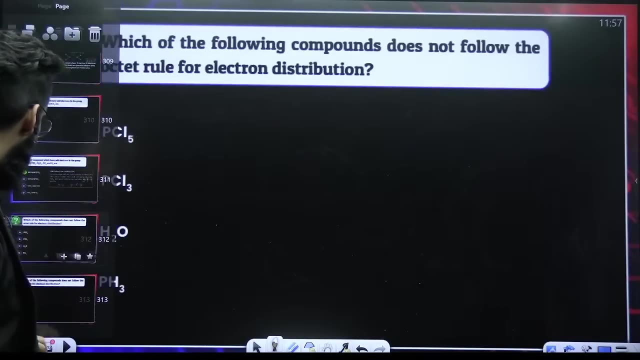 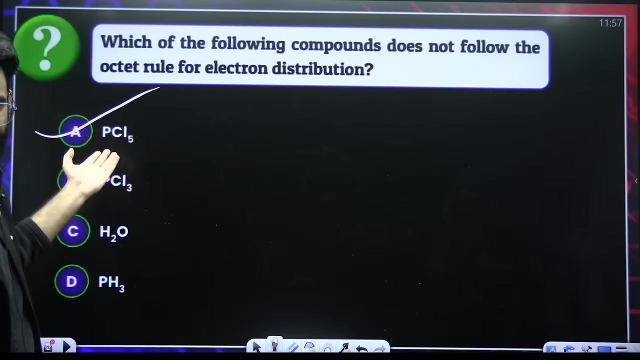 you which of the following is electron deficient? I told you right now, few minutes back: bh3- right, so this is electron deficient. need 2013: okay. which of the following does not follow the octet rule? pcl-5- pcl-5. so it has got 10 electrons in its outermost shell- right, the octet rule is failed, it you? 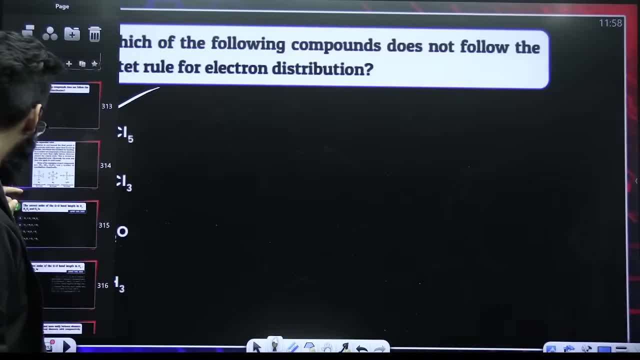 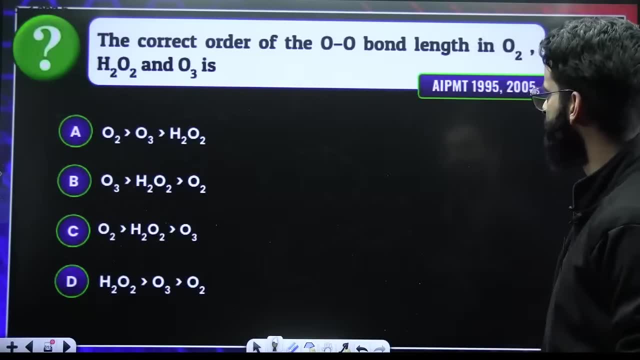 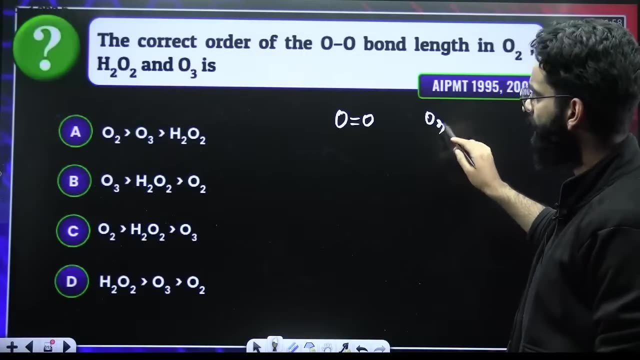 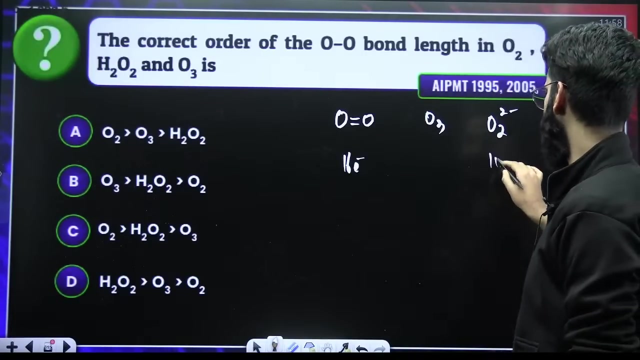 should have eight done. this question has been asked two times. you are given two species, three species, sorry. you hold two O2, then you have got O3, then you have got H2O2. H2O2 means O2 di negative right. O2 is a 16 electron specie. this is a 18 electron specie. 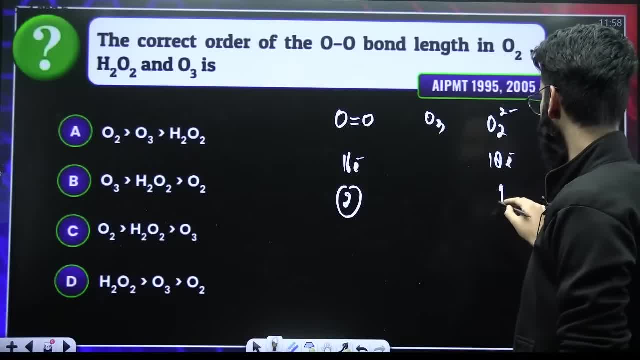 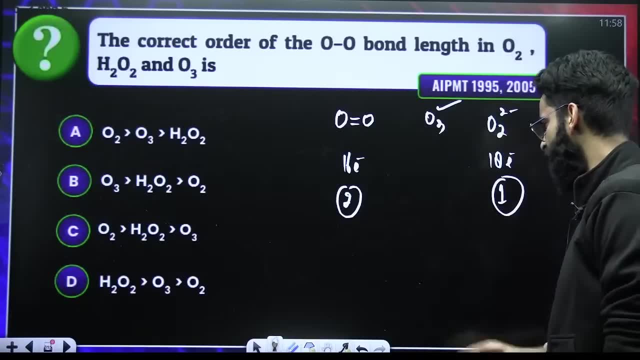 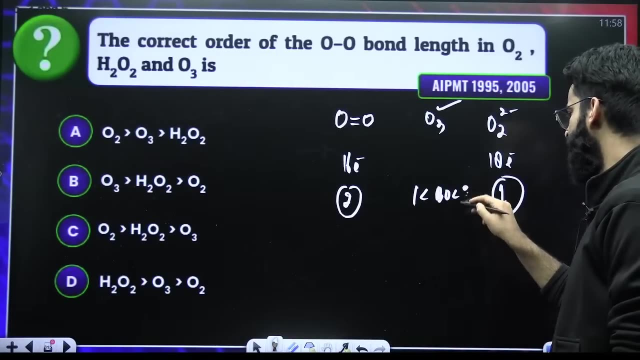 16 electrons specie. its bond order is 2: 18 electrons specie. its bond order is 1, right. its bond order is 1, perfect. and its bond order in O3- there will be resonance bond order lies between 1 & 2. it lies between 1 and 2, perfect. so you know, bond order is inversely proportional to bond. 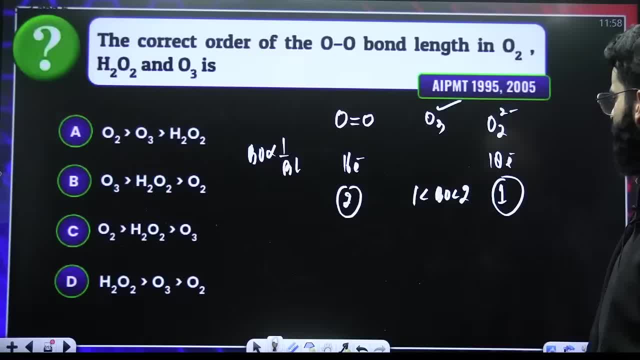 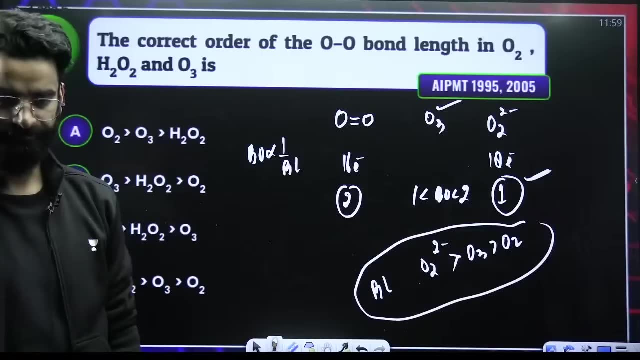 length right. so which one has got least bond order? this has got least bond order, so maximum bond length. so O2 di negative will have maximum bond length, followed by O3, followed by O2. this is the bond length order, right? this is the bond length order, is it done? 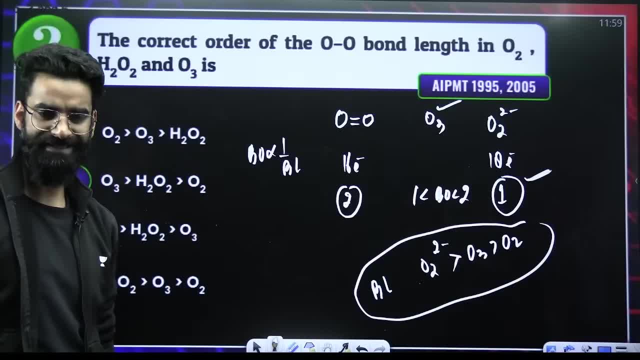 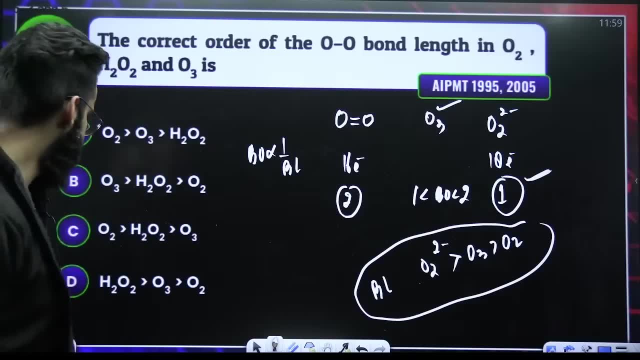 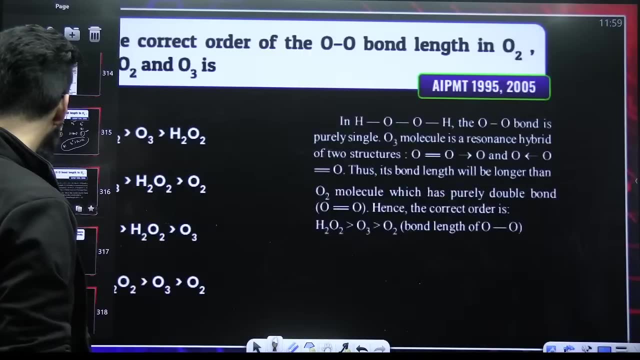 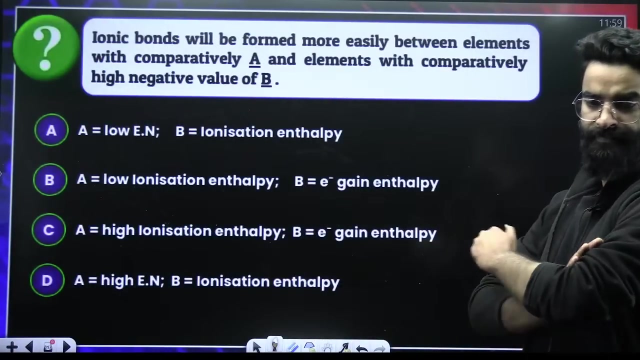 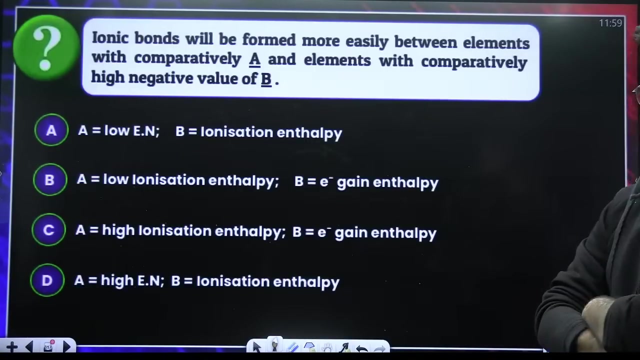 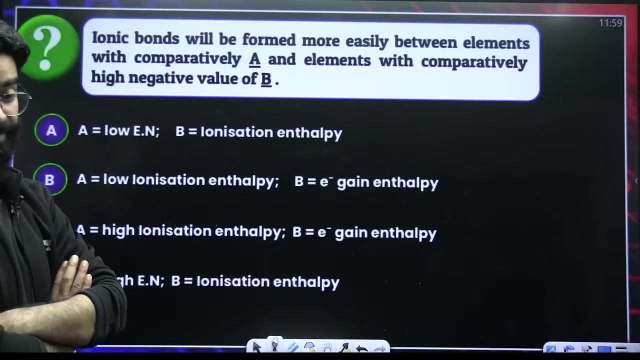 is it done, guys? is it done? I believe it is okay. I'm going ahead. what about this question? look at the question carefully. look at the question carefully. ionic bonds will be formed more easily if metal has low ionization energy and non-metal has high electron affinity or electron gain enthalpy. yesterday, I've told you yesterday. 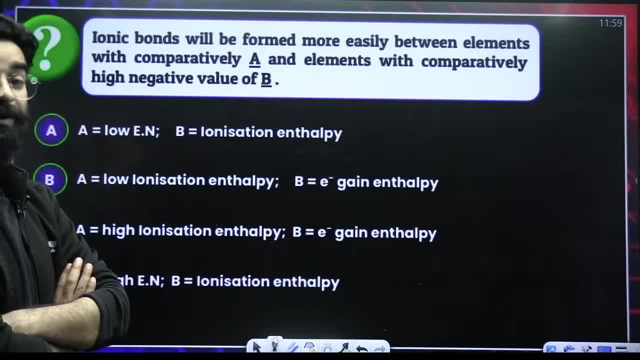 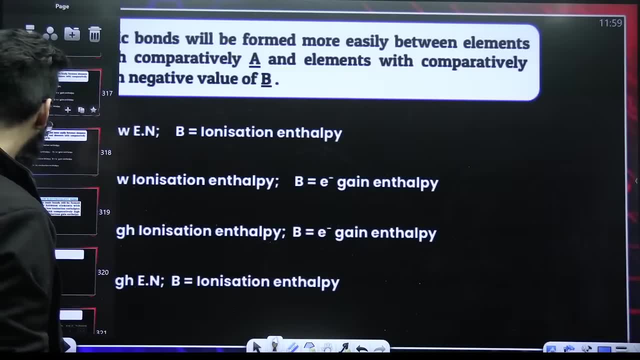 I've told you that. so what is the answer? metal should have low ionization energy and non-metal should have high electron affinity. perfect, so it's option b. with the answer, tell me the isoelectronic set of species among all isoelectronic set which have got same. 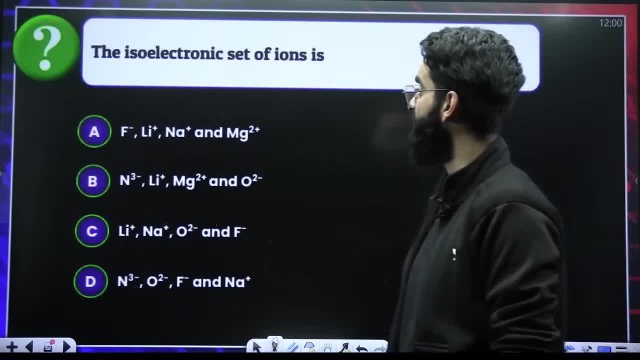 number of electrons, same number of electrons, same number of electrons, n trine gate to 7 plus 3, 10, 8 plus 3, 10, 9 plus 1, 10, 11 minus 1, 10. so these are isoelectronic species. 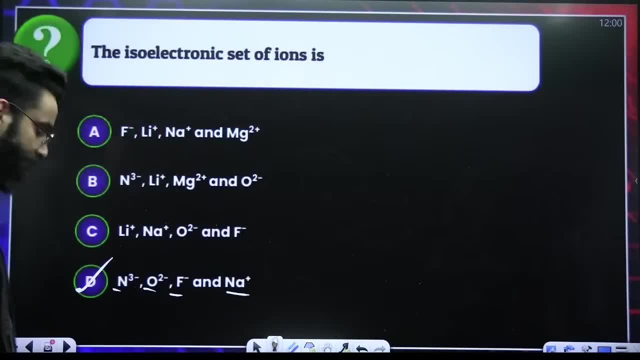 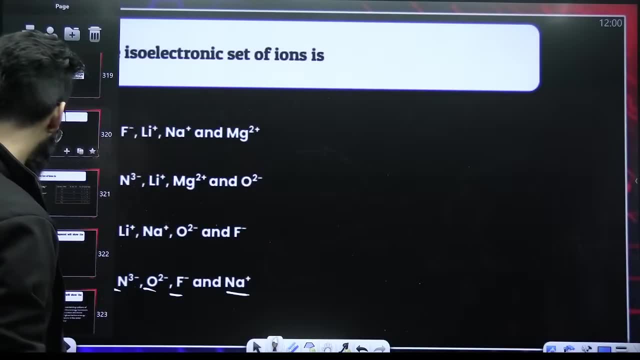 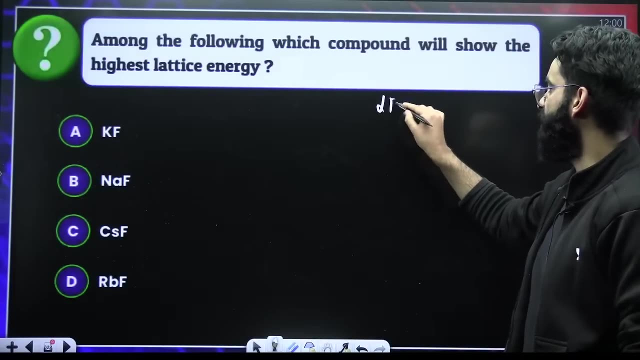 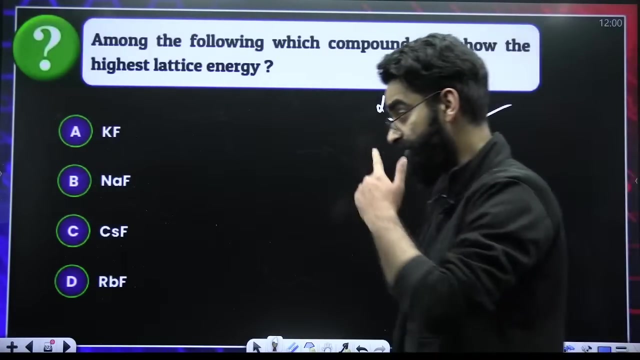 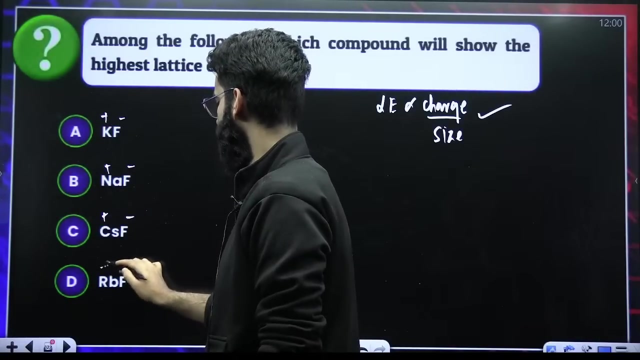 these are isoelectronic species. which of the following has highest lattice energy? lattice energy, if you remember, yesterday I've told you: directly proportional to charge. inversely proportional to size. directly proportional to charge. inversely proportional to size charge. charge everywhere is same. F-K-N-A charge everywhere is same. charge everywhere is same. now decide on the size. 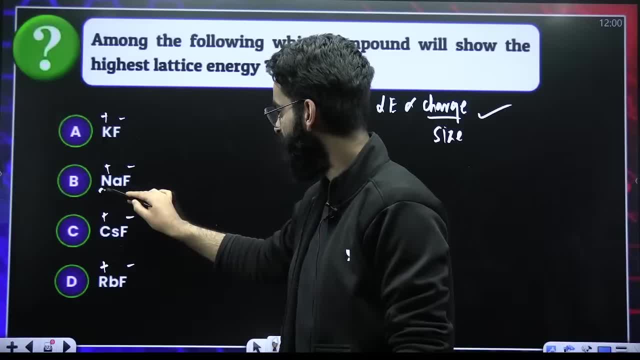 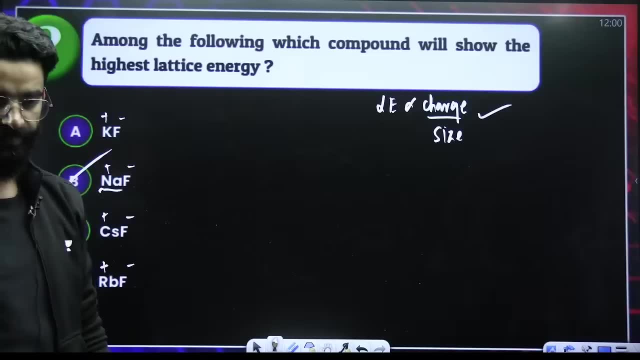 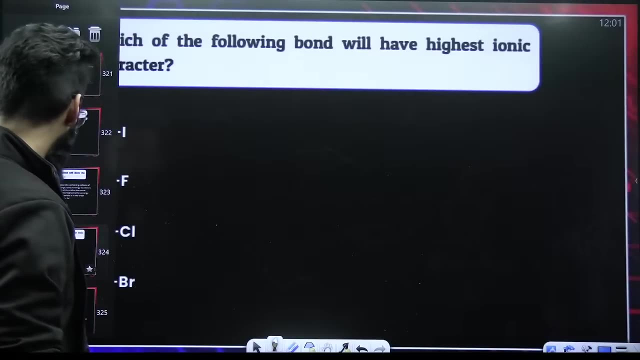 lesser the size of cation, more the lattice energy Na positive has got lesser size among all these cations. so maximum lattice energy, maximum lattice energy. maximum lattice energy. what about this one which of the following bonds have got highest ionic character: H-I-H-F-H-C-L-H-B-R. 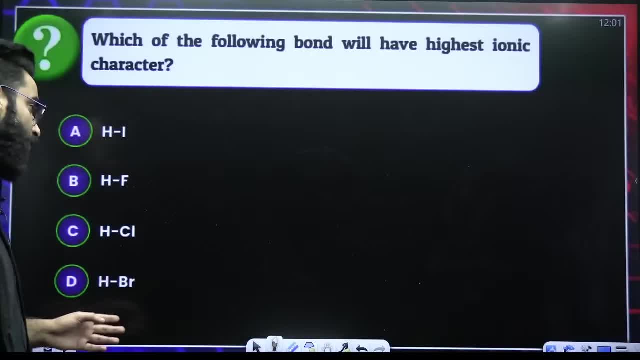 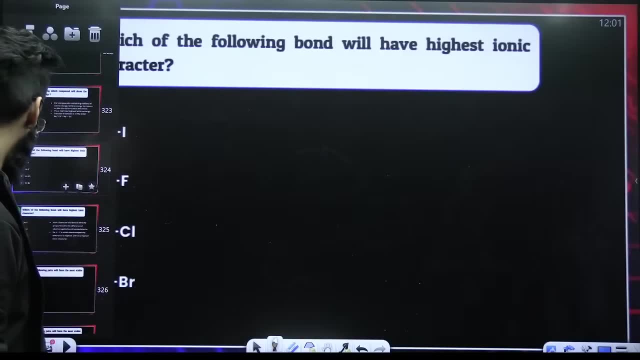 Look at the electronegativity difference. Where is the electronegativity difference? more In the second one. More the electronegativity difference, more the polar nature, More the covalent character, Sorry, more the ionic character. 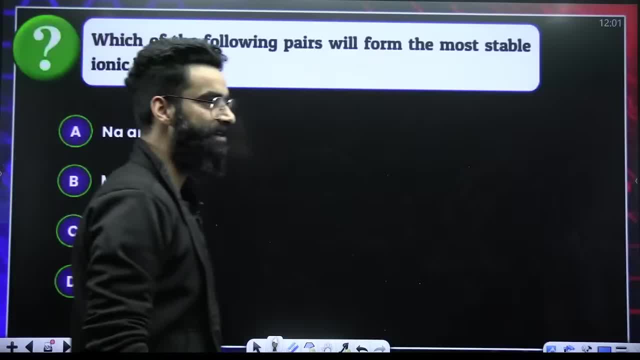 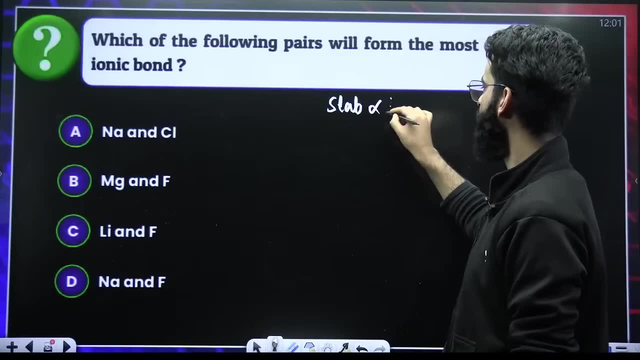 Right More the ionic character. Which of the following pairs will form most stable ionic compound? Stability of ionic compound depends on lattice energy. Stability of ionic compound depends on lattice energy, And lattice energy depends on charge and size. Charge and size. 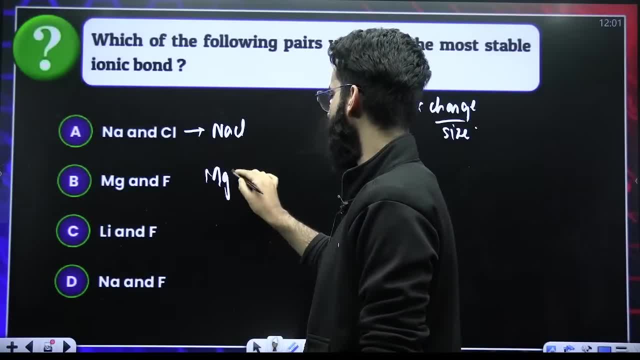 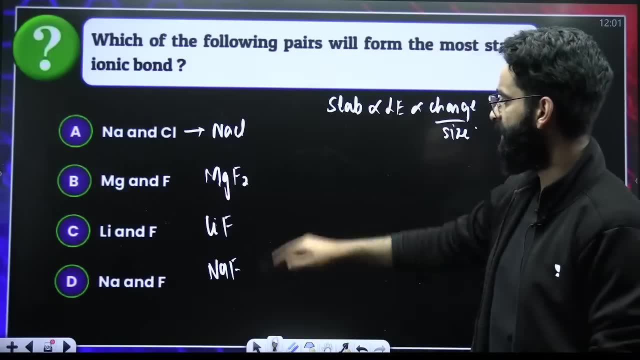 If Na and Cl mixes, it forms NaCl, This forms MgF2.. This forms LiF. This forms NaF. Right Now, which one has got maximum lattice energy? Look at the charge: Plus 1.. Plus 2.. 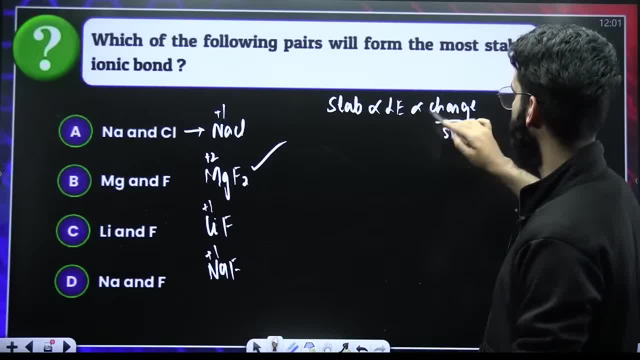 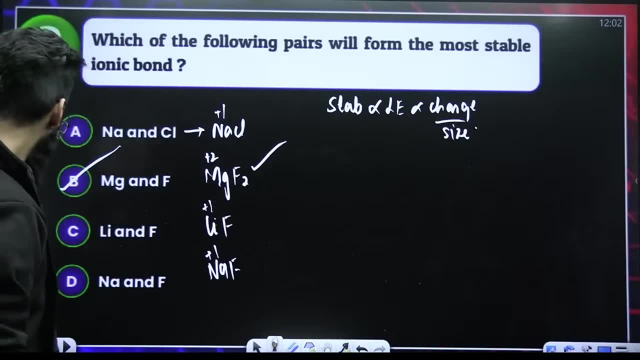 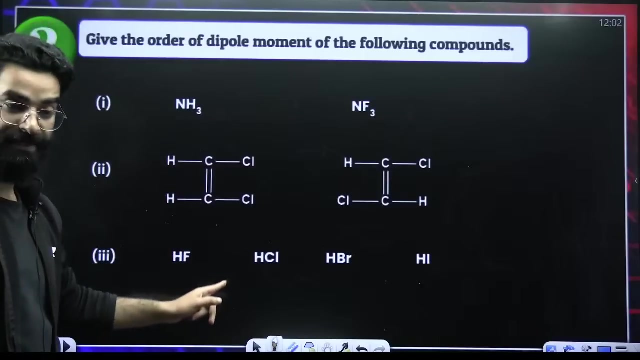 Plus 1.. Plus 1. This has got maximum lattice energy. Maximum lattice energy means maximum stability. So MgF2.. Right MgF2.. I believe I am clear. I believe I am clear. Well, these questions we have solved yesterday. 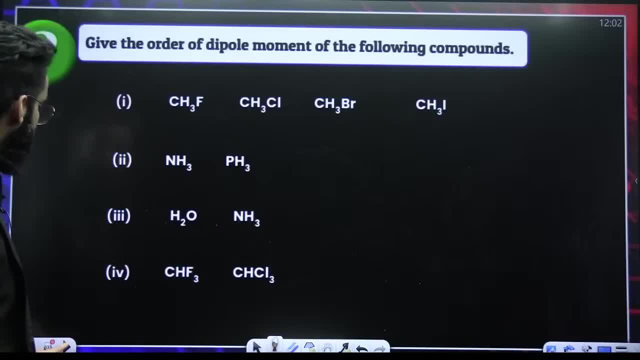 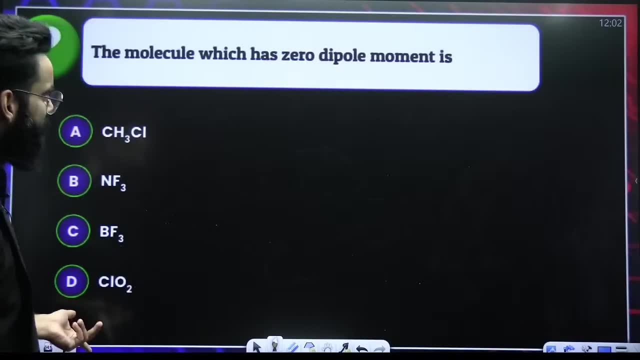 If you remember, I am not going to solve them again- These questions we have solved. These set of questions also we have solved yesterday. What about this one? This you already know: The molecule which has zero dipole moment is BF3.. 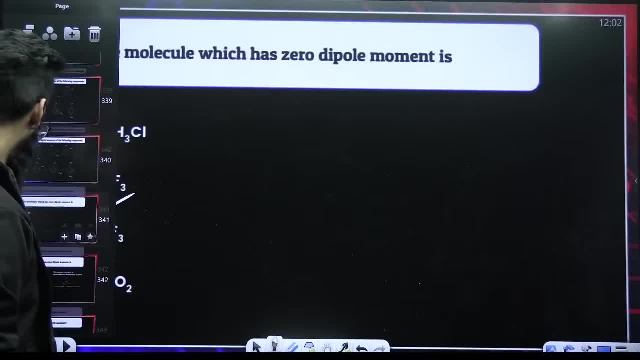 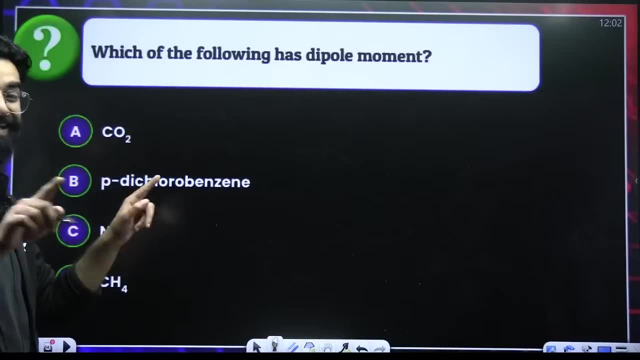 Right. The molecule which has zero dipole moment is BF3.. The molecule which has dipole moment- carbon dioxide- linear- no dipole moment. p-dichlorobenzene: no dipole moment. CH4: no dipole moment. only NH3 is the one which has got the dipole moment. 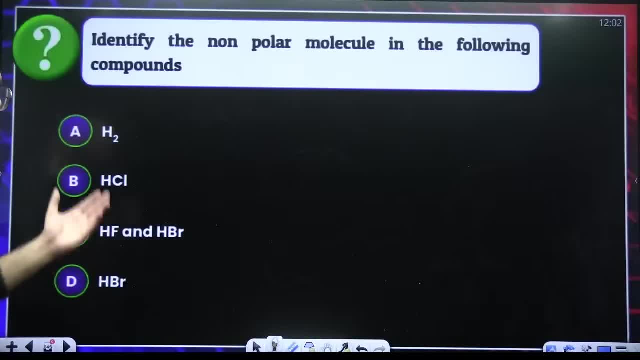 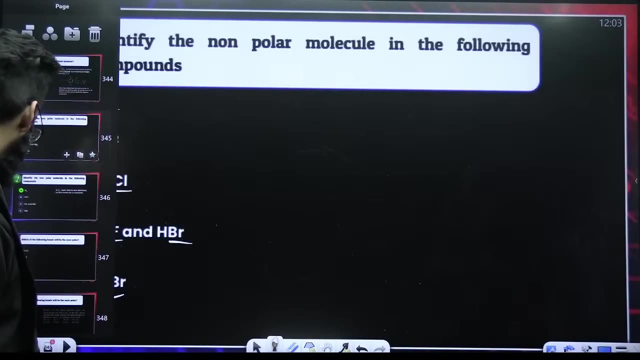 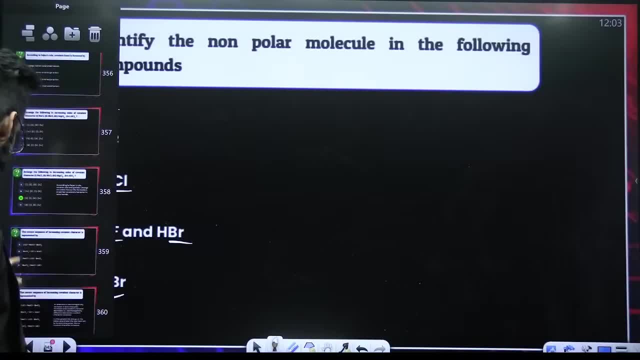 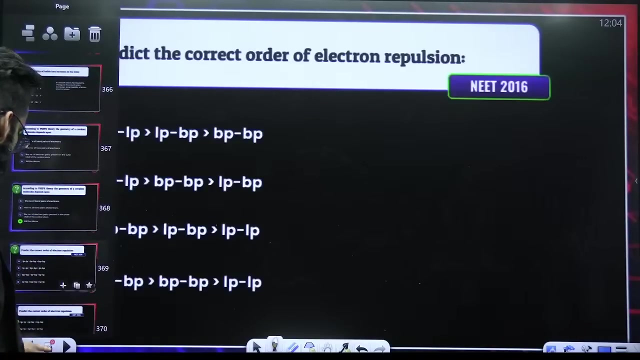 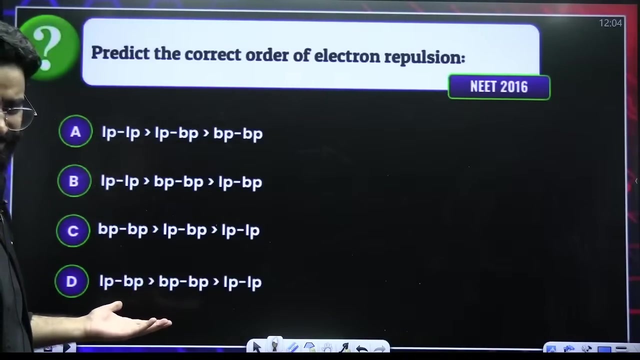 Just a second, guys. these are some repeated questions which I have solved already. Subtitles by the Amaraorg community. This you should be able to answer quickly. This you have to be. you have to. I mean you know it already right yesterday. I have told 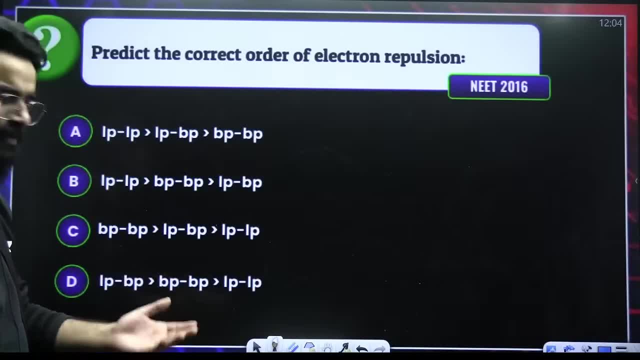 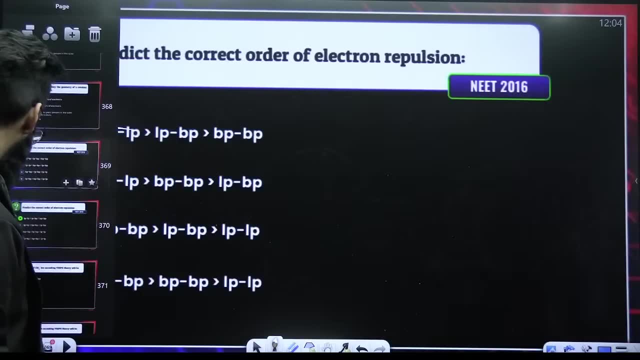 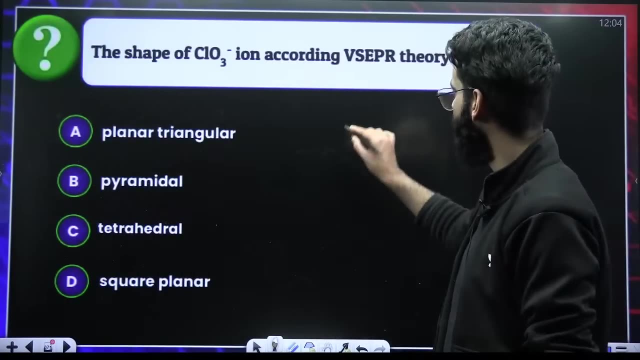 you in detail: Loan pair- loan pair repulsions are maximum, followed by loan pair- bond pair, followed by bond pair bond pair right. perfect. The shape of ClO3 negate to iron. shape of ClO3 negate to iron quick. 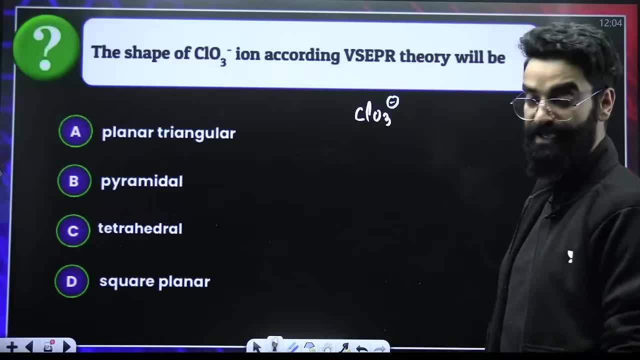 The shape of ClO3 negate to iron. The shape of ClO3 negate to iron. The shape of ClO3 negate to iron, As per VSCPR, is: Quick guys, be very quick, be very quick, Be very quick. 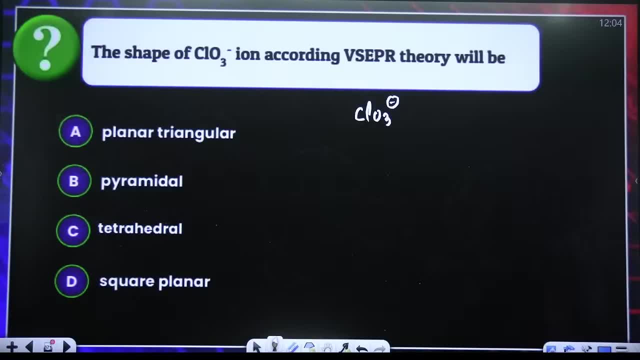 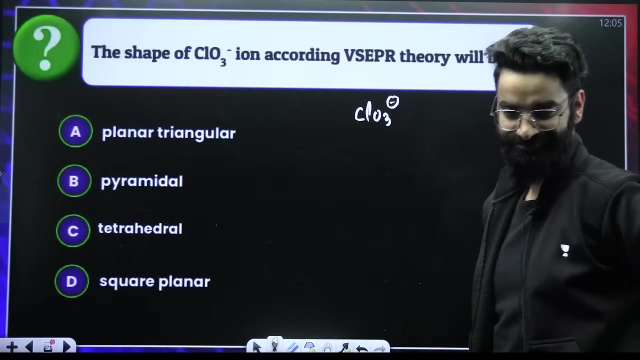 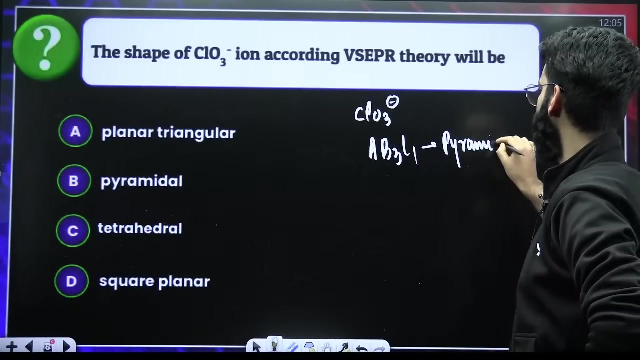 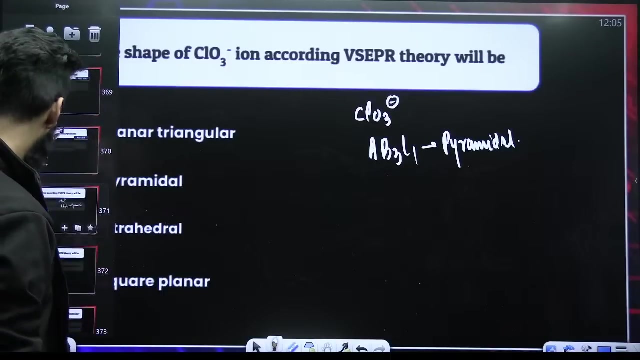 The shape of ClO3 negate to iron? It is which one is it? The type of the molecule is AB3L1, which has to be pyramidal, right, Which has to be pyramidal. So option B is the one which is correct. 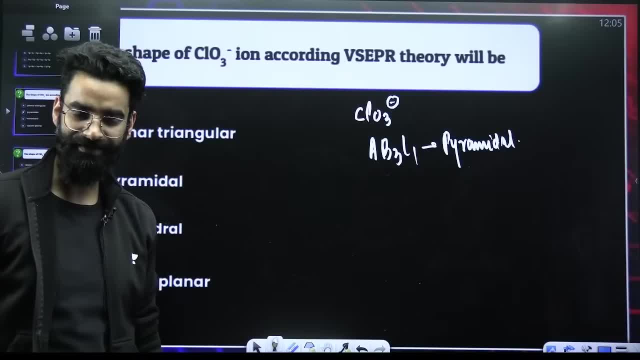 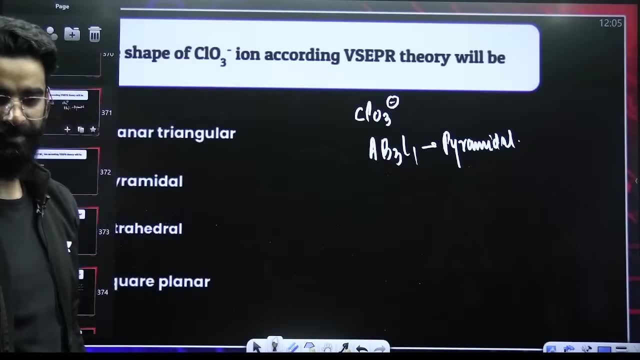 Guys, am I going very fast or it's fine? Just tell me in the chats: Am I going very fast or you are liking it? See all these things we have discussed yesterday. right, All these, all these things we have discussed yesterday. 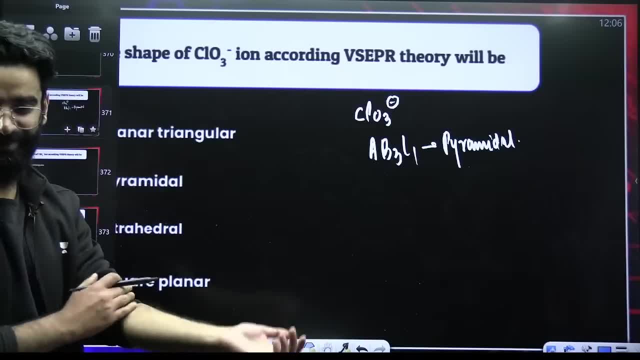 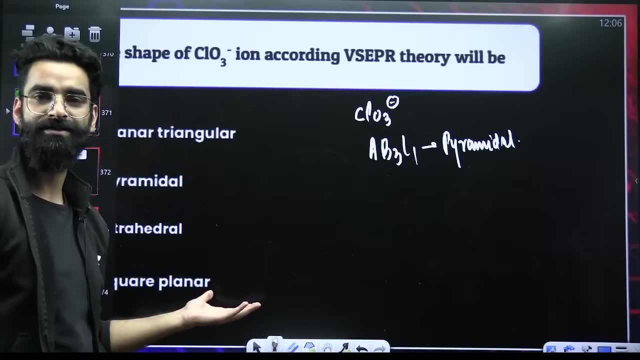 I'm not explaining things. we are trying to solve the questions in lesser time, right? Because if it was physical chemistry, then I don't know in order to? I think till now we have solved some hundred questions. If it was hundred questions of physical chemistry, then it would have taken like four hours. 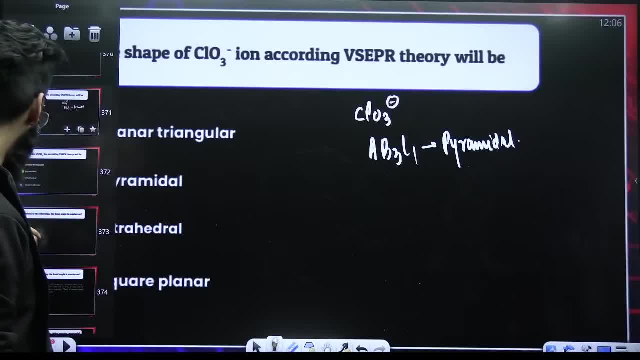 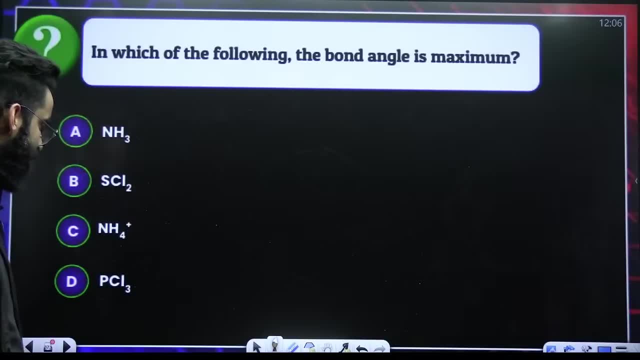 You know it: Perfect Chalo. you are loving it. That's great. Quickly, Which of the following Bond angle is maximum? Bond angle is maximum quickly. Bond angle is maximum quick, Quick, Quick, quick, quick, quick. Quickly, It is option C: SP3 geometry, SP3 tetrahedral 10928.. 10928, right. In all the others, it will be less than that. In all the others, it will be less than that. 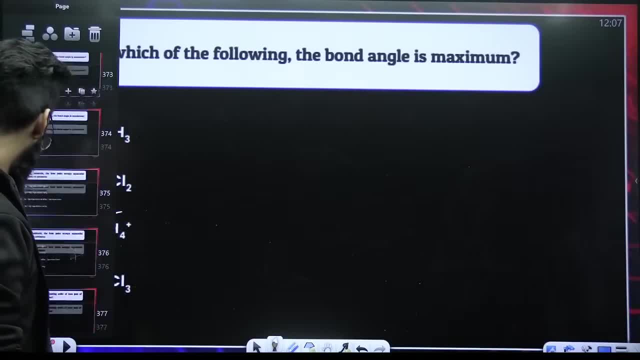 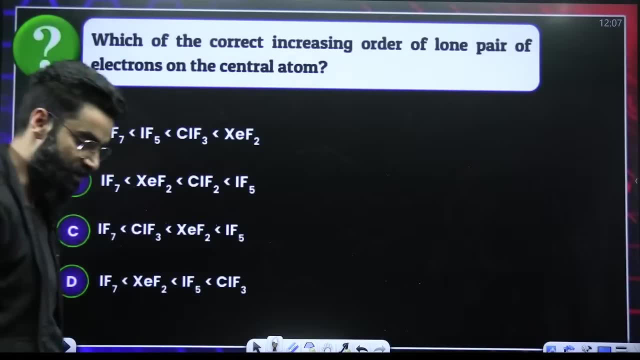 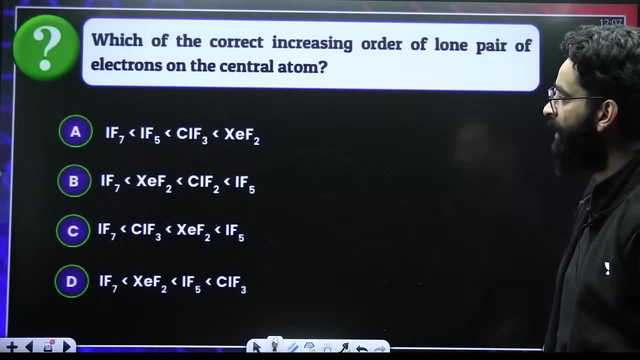 Because of the presence of the lone pairs. Because of the presence of the lone pairs. Order of the lone pairs. Order of the lone pairs on the central atom: Quick X, E, F2.. Xenon has got three lone pairs. 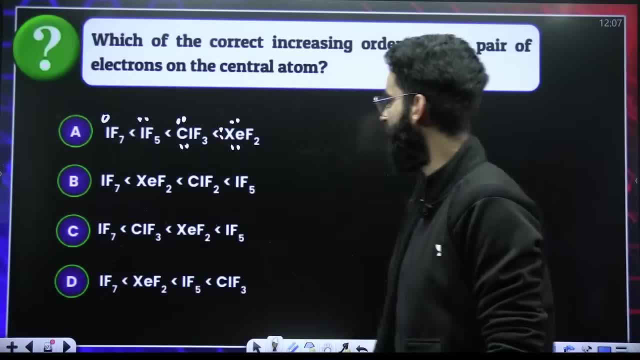 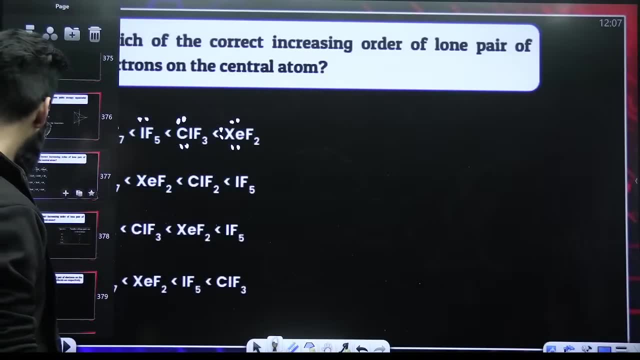 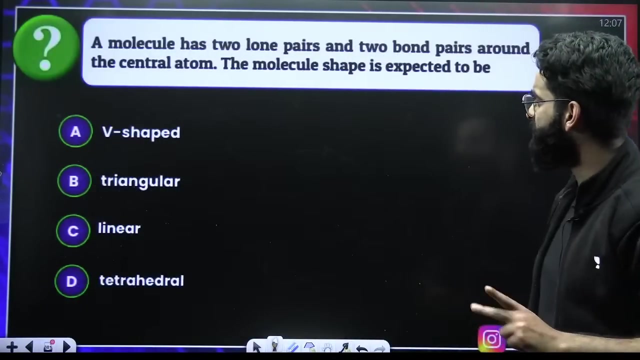 Chlorine has got two lone pairs. Iodine has got one lone pair, Zero lone pair. Right Done, Done people. Yeah, A molecule has two lone pairs. A molecule has two lone pairs and two bond pairs around central atom. 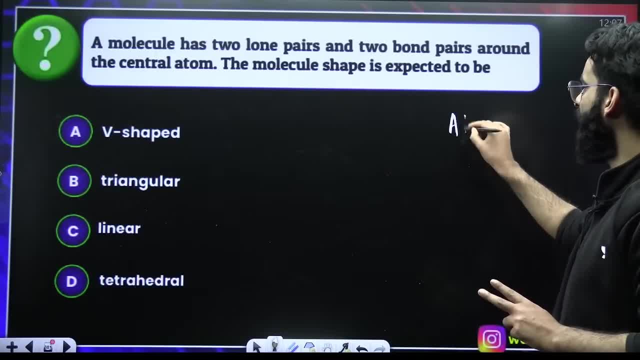 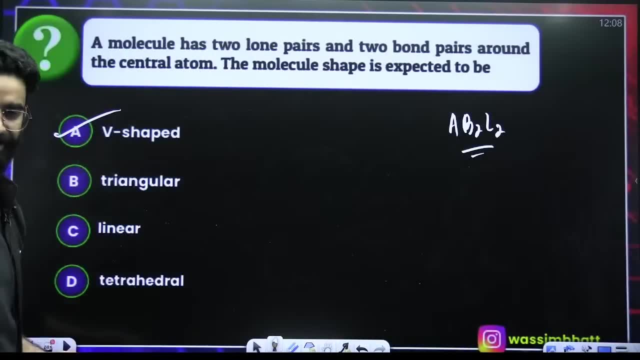 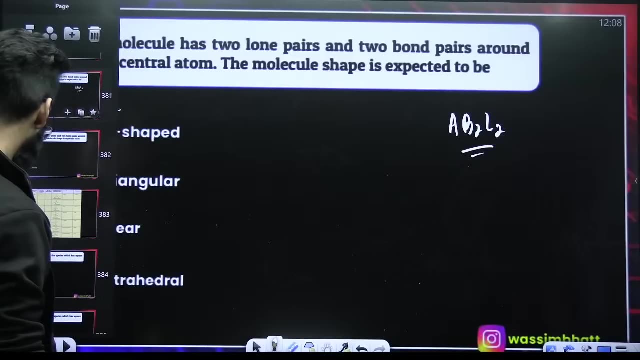 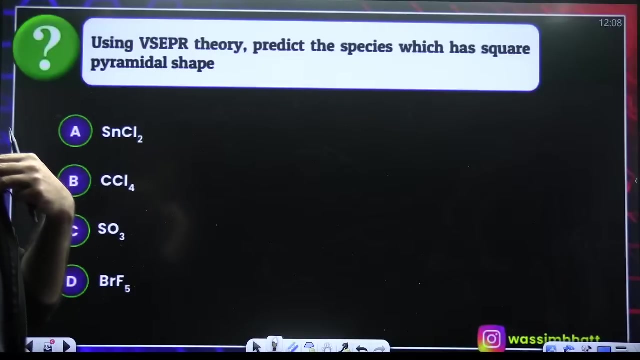 Right Around central atom. The molecule shape is: It is AB2L2.. AB2L2.. AB2L2. V is CPR, V shaped, Right Yeah, What about this one? Last one? Wait guys. Wait guys. Square pyramidal shape, Square pyramidal, Square pyramidal means: AB5L1.. AB5L1.. AB5L1.. Yes, Dusted, Dusted, CLF3.. Number of lone pairs on central. 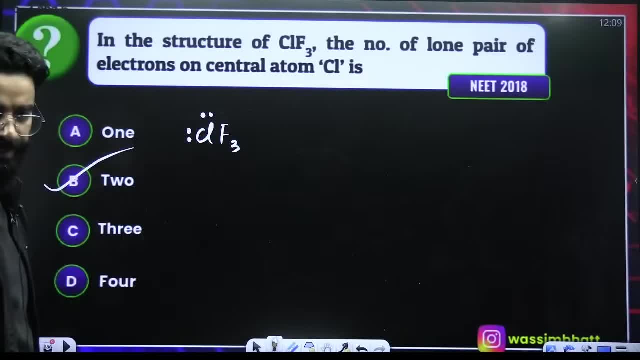 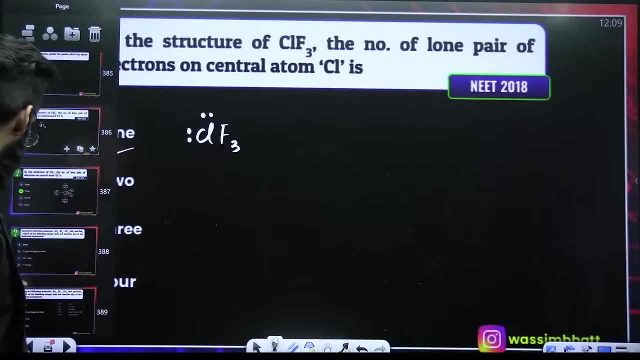 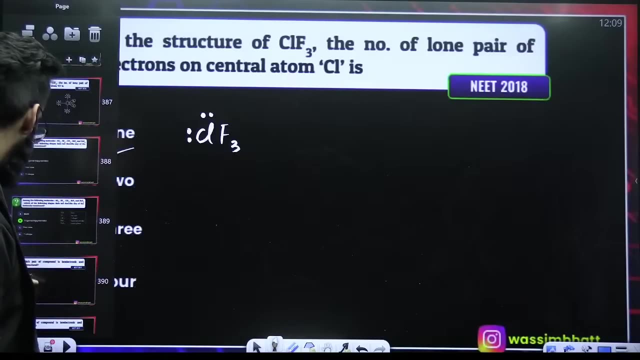 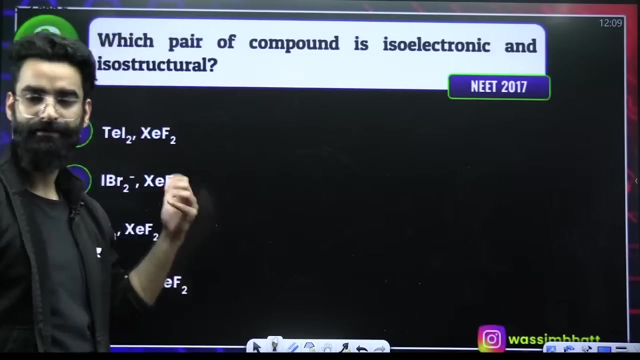 CLF3.. Two lone pairs on chlorine Right. Two lone pairs on chlorine Need 2017.. I think we have solved this question already Today. only we have solved Option was two Right: AB2L3.. AB2L3.. 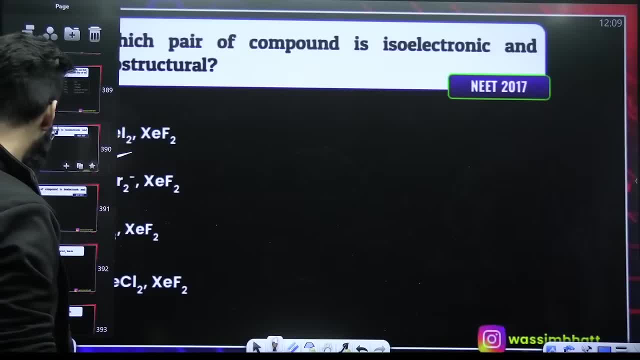 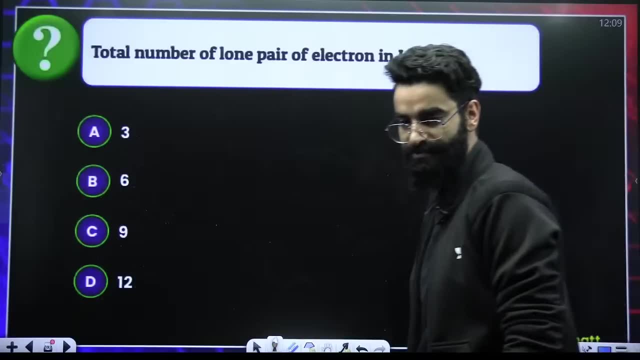 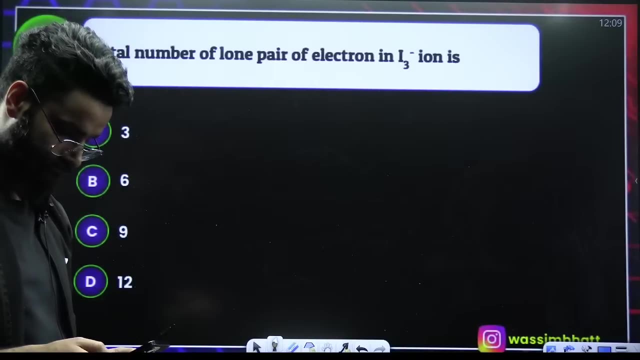 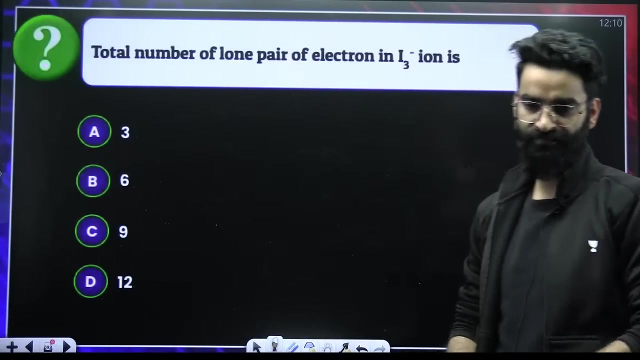 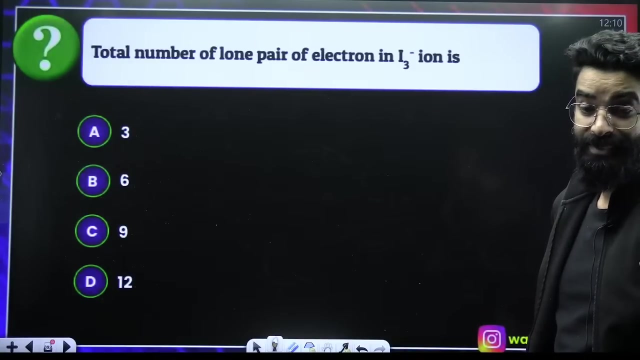 We have solved this question already. okay, I believe a lot of students will mark this question incorrectly. why do I feel so? why do I feel so? that's why I told you a lot of students will mark it incorrectly. he's not asking about the loan pairs on central atom. he's asking about the total number of loan. 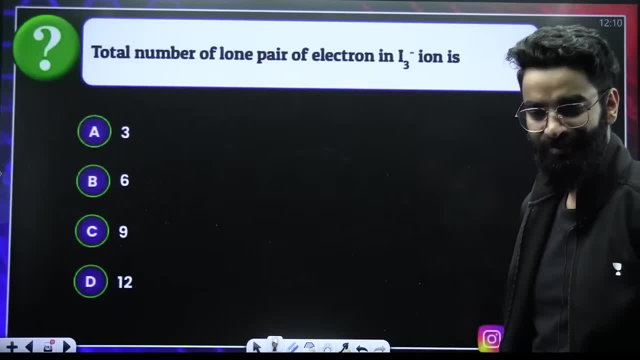 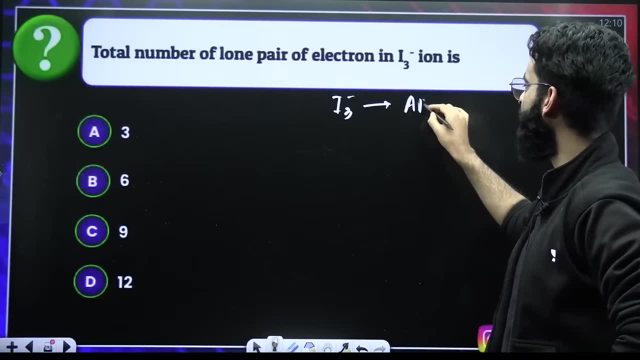 pairs. he's asking about the total number of loan pairs. see, we already know in case of i3 negative, we already know in case of i3 negative, it is of the type AB2L3. I hope you remember this. for example, iodine: right there's a lone pair of. 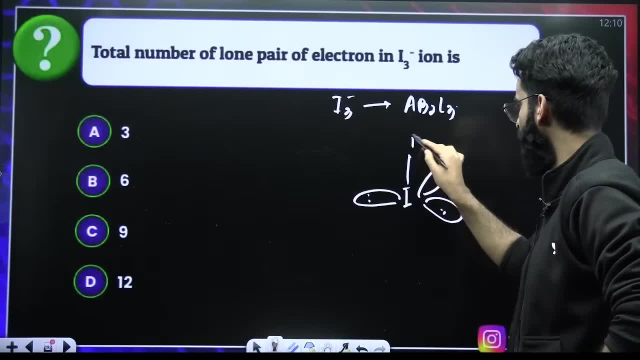 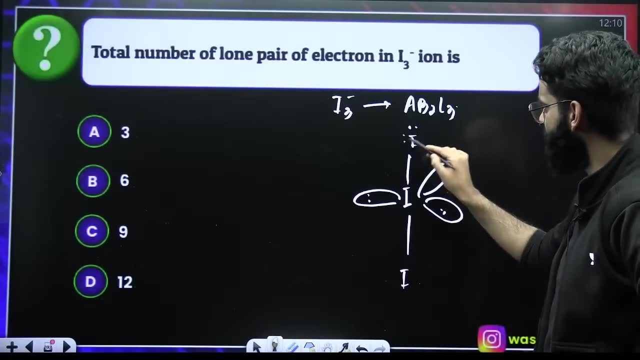 the central iodine lone pair of the central iodine lone pair of the central iodine. there's one more iodine here. this is one more iodine here. right, perfect, this is the structure. no, no, this particular iodine has got three loan pairs. this also has three loan pairs. this also has three loan pairs. 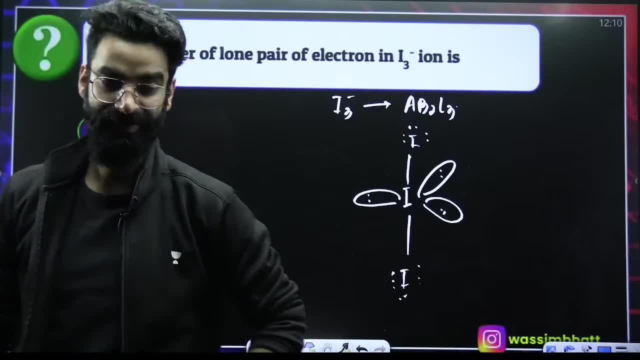 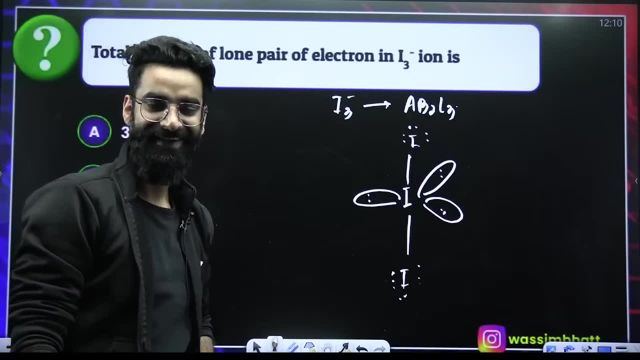 so in total, how many? 3, 3, 9, 3, 3, 3, 6, 3, 9 in total there are nine loan pairs in the molecule. if he had asked about you, the total lone pairs in the central atom, if he had asked about the total lone pairs on the, 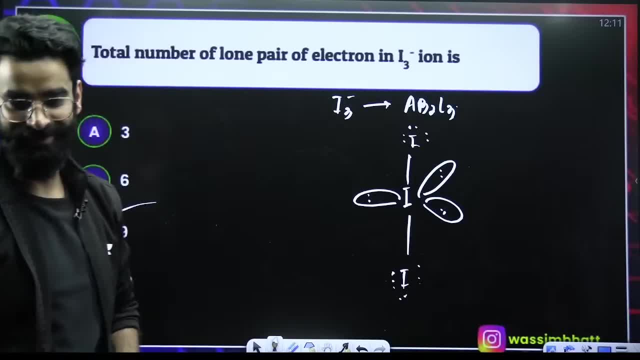 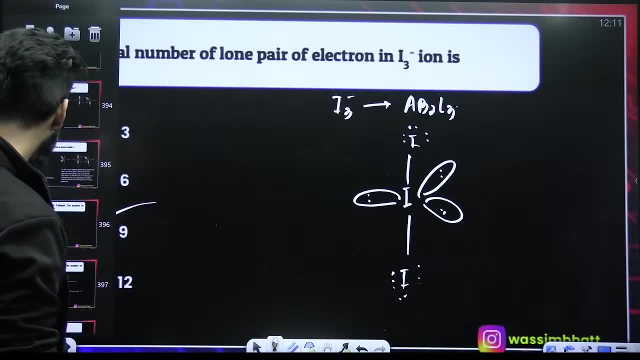 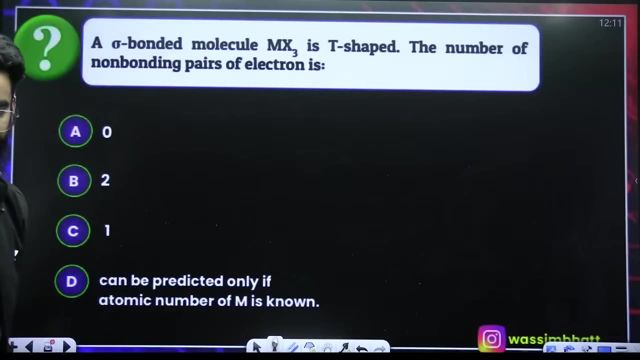 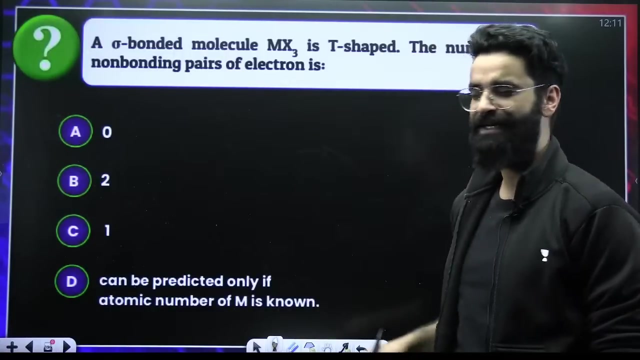 central atom, then the answer was three. he's asking only about the total loan pairs. they see how? how do they play with you with small kids? not good, right. okay, quick right. a sigma-bonded molecule, MX3. MX3 is t-shaped, E shaped, just understand, T shaped has to be. 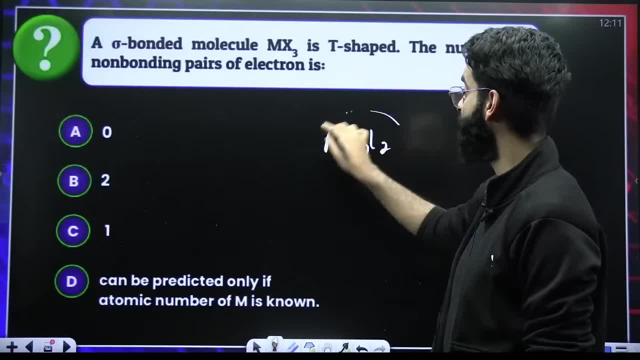 the type has to be what a sigma-bonded molecule, MX3. MX3 is t-shaped. I just understand t-shaped has to be. the type has to be what? what p shape? the type has to be ab3, l2, ab3, l2, the non-bonding electrons. non-bonding means lone. 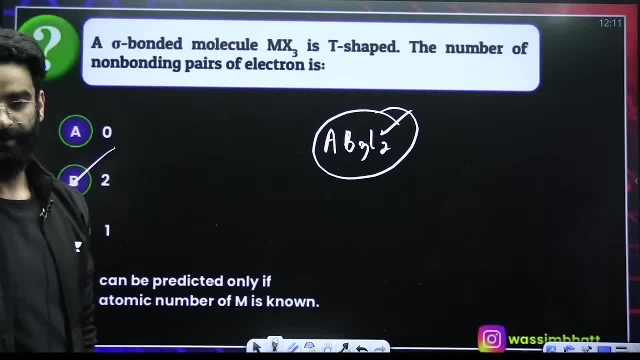 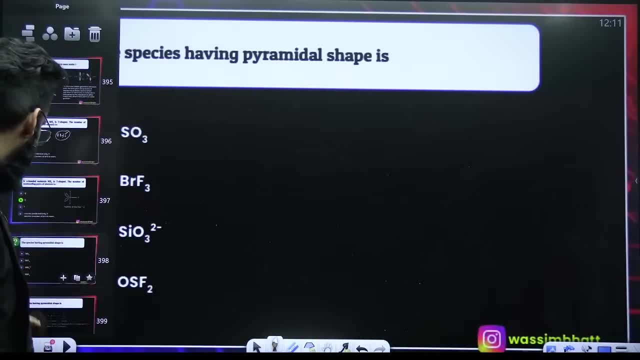 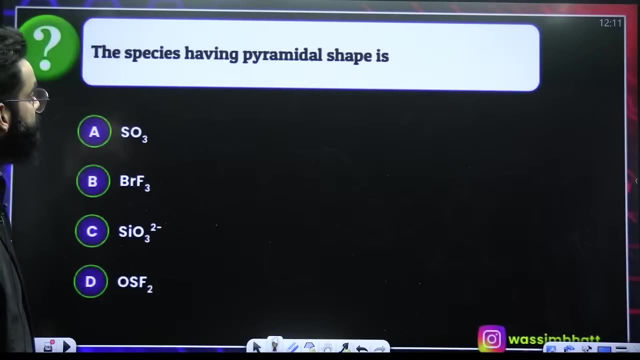 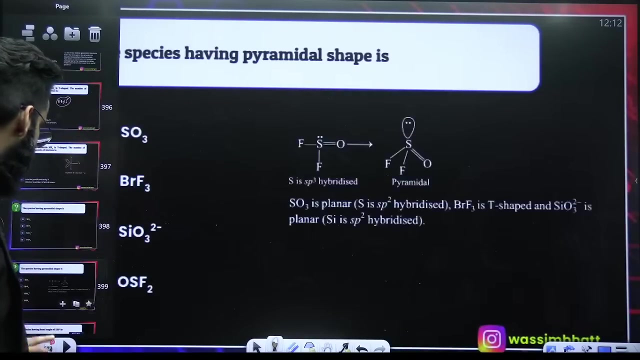 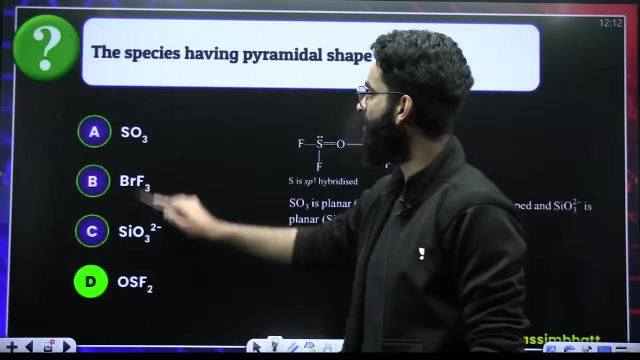 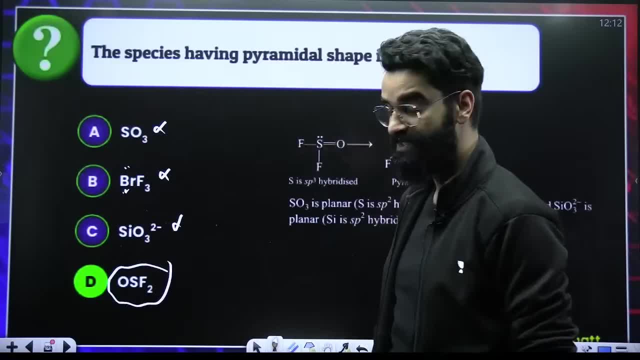 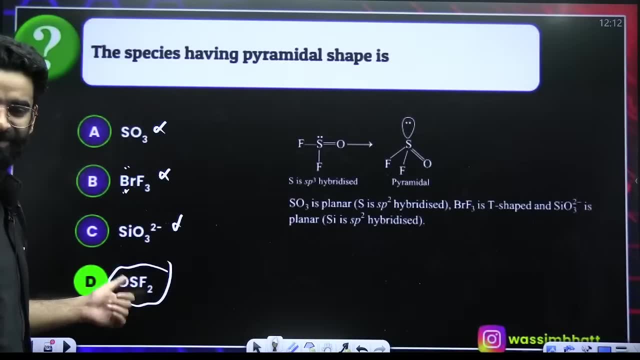 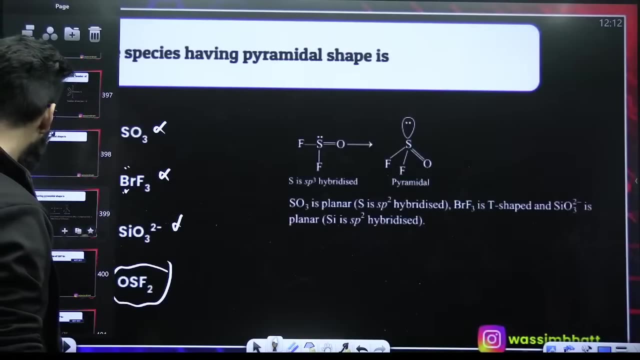 when this is not pyramidal. it is osf2, basically, here, which is pyramidal among all. okay, this is not osmium. okay, It's not osmium. O stands for oxygen, S stands for sulphur. Right, Perfect Shape of methane molecule is, you know, tetrahedral. 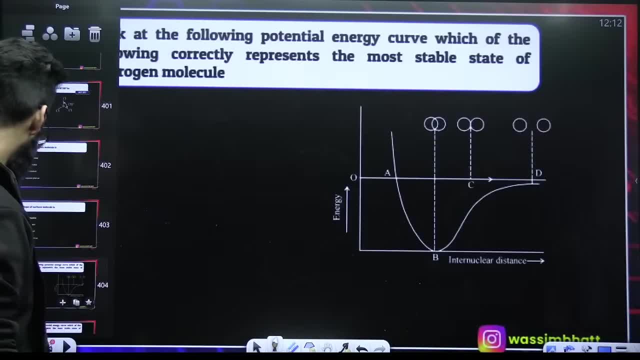 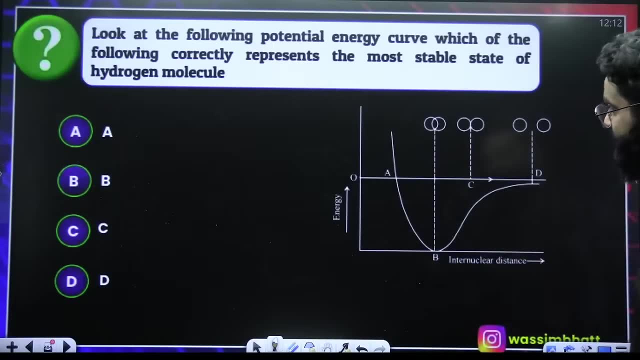 Believe it. Can you see the graph: Energy versus internuclear distance? this graph we have seen. Look at the following curve. Which of the following correctly represents the most stable state of hydrogen molecule? Most stable state: Most stable state: Quick. 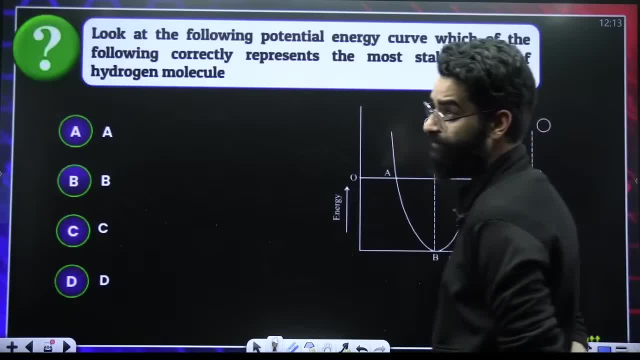 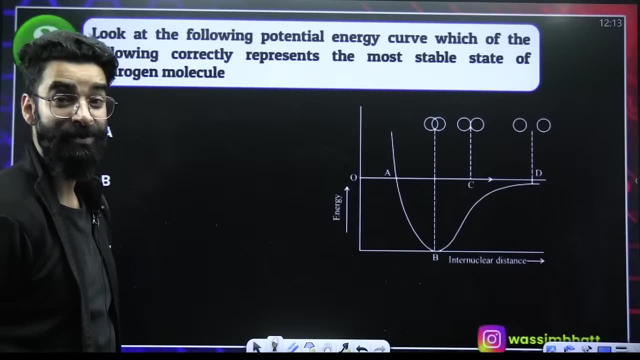 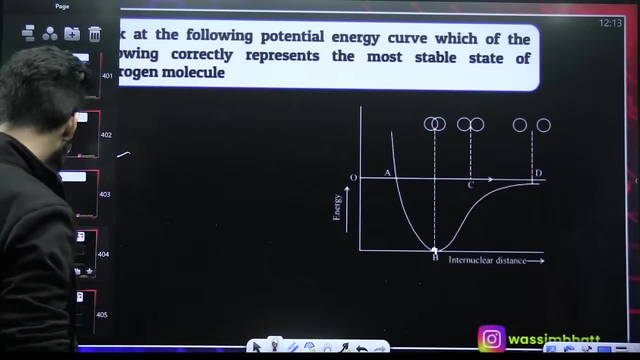 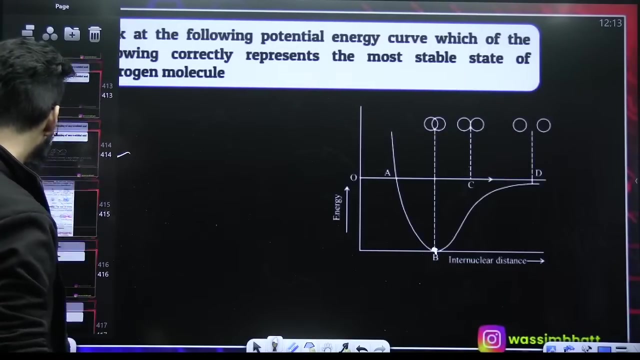 Most stable state. Where is the most stable state? Most stable state: Potential energy: minimum Potential energy: minimum Stability: maximum Right du by dr is equal to 0.. Yesterday we have discussed at this point Perfect. Where do I get more questions from bonding? 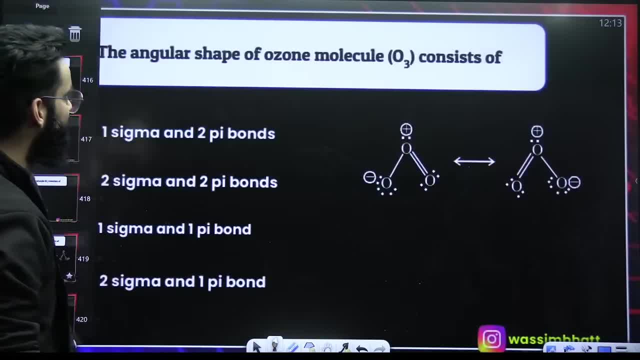 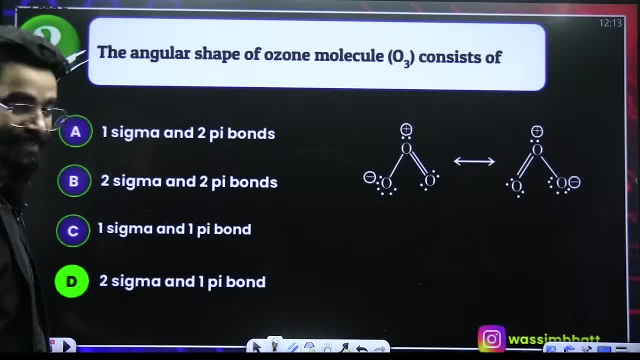 I think bonding is all about it. Right, I'll say one more O3 molecule: the number of sigma and pi. This has been frequently asked, this question. Okay, In case of O3 molecule, How many sigmas are there? 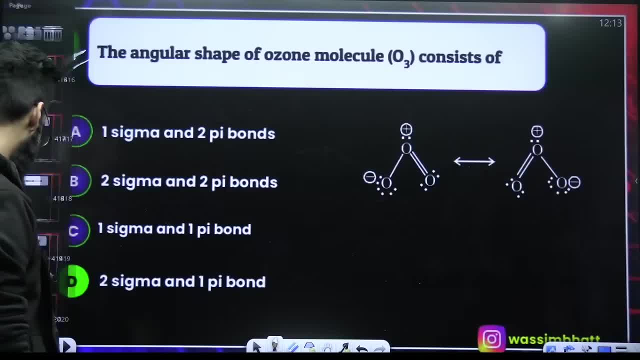 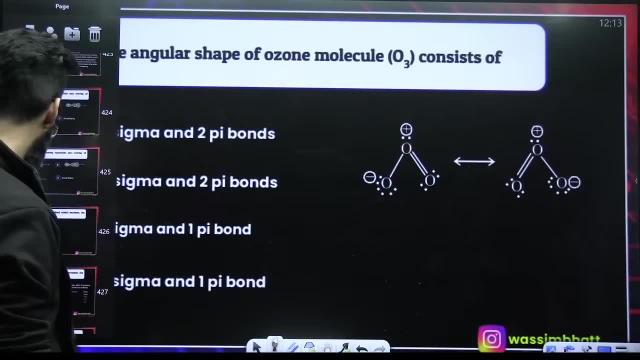 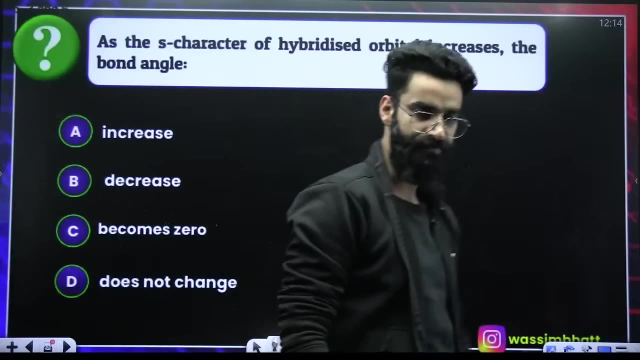 How many pi are there? Remember this one: There are two sigma and one pi bond in O3.. Let me see some assertion based questions. Okay, One question. One question Which is for everyone. This I would have taught you in GOC. 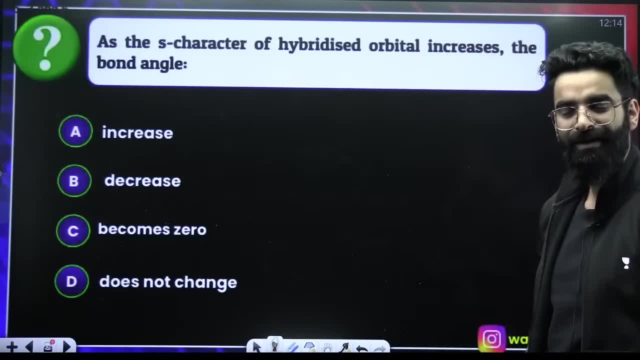 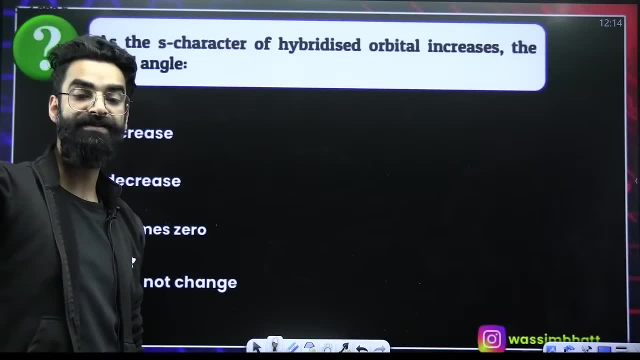 If you have seen my GOC lecture long back, As the S-corrector of the hybrid orbital increased, The bond angle. Bond angle is directly proportional to electron negativity. Electron negativity is directly proportional to percentage of S-corrector. It increases. 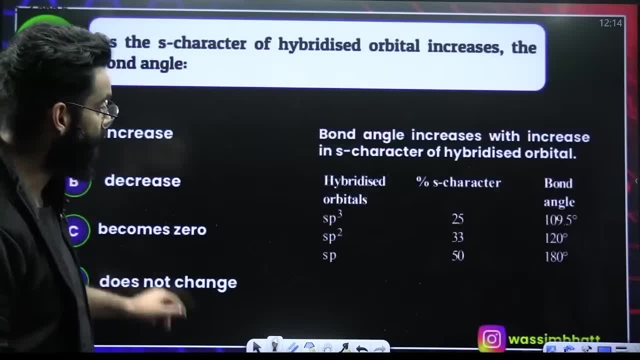 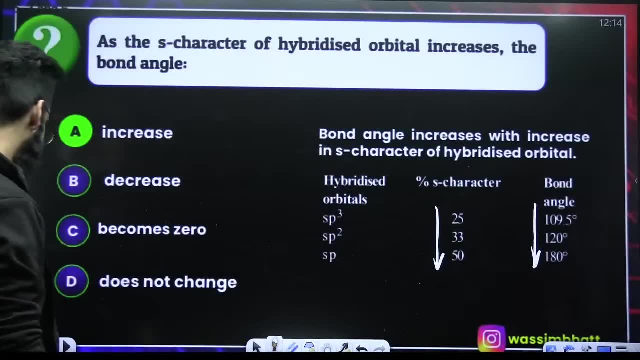 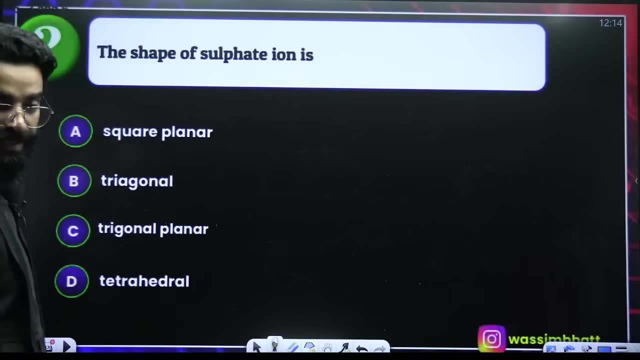 Right, Perfect, I hope you remember this. As the bond angle, Bond angle increases, S-corrector also increases, Electron negativity also increases. Okay, What is the shape of sulfate ion SO4 di-negative? Shape of sulfate SO4 di-negative. 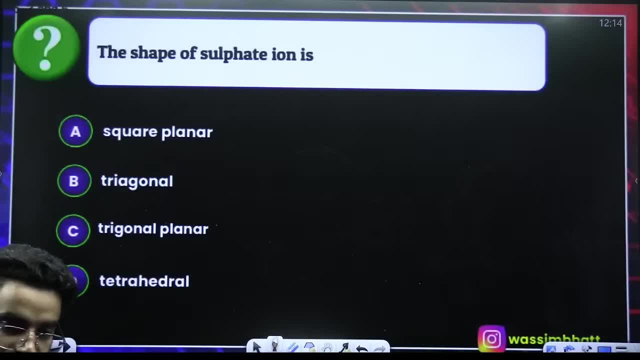 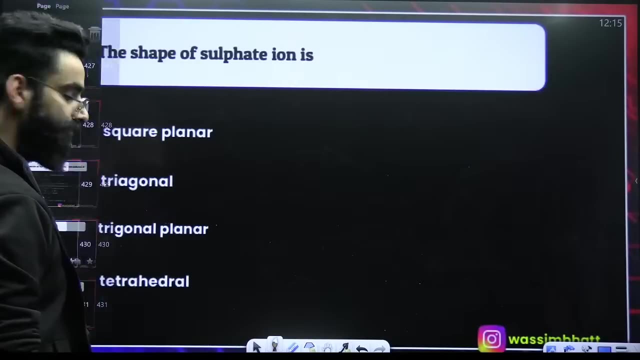 Quick Shape of sulfate SO4 di-negative Everyone. Shape of sulfate SO4 di-negative. Quick SO4 di-negative. SO4 di-negative- It is SO4 di-negative, Wait guys. SO4 di-negative Right. 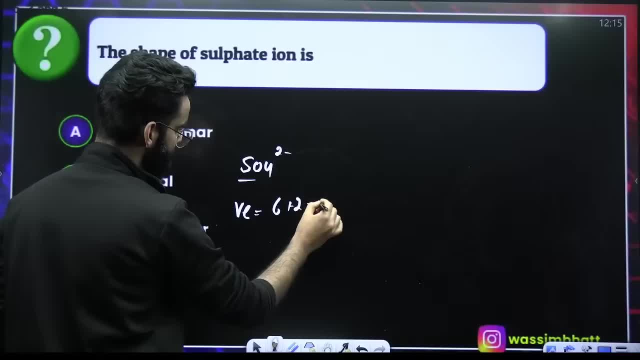 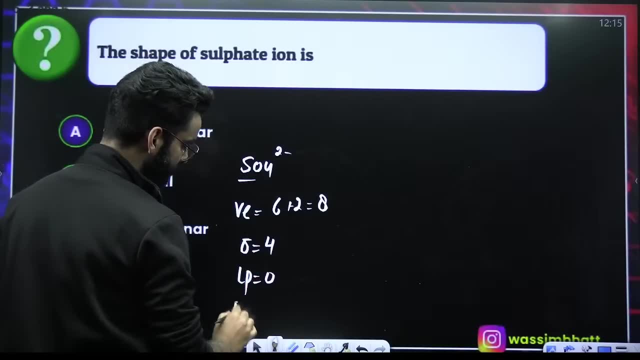 Violence. electrons of sulfur: R6 plus 2 makes it 8.. Right Sigma bonds: R4.. Sigma bonds: R4.. Lone pairs: R0.. Type AB4L0.. AB4L0. Tetrahedral. 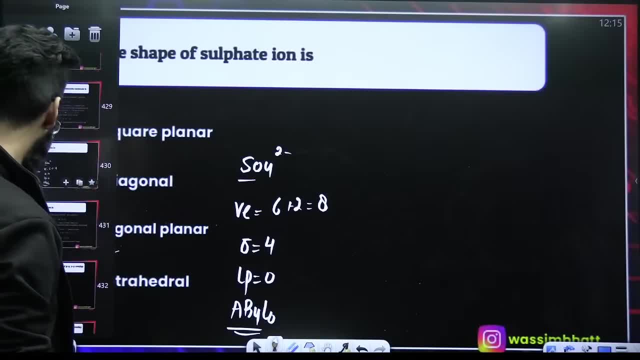 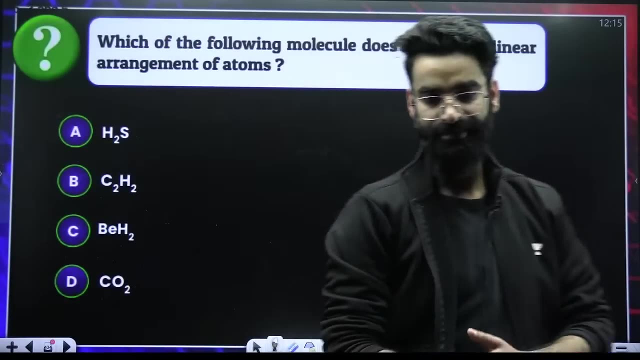 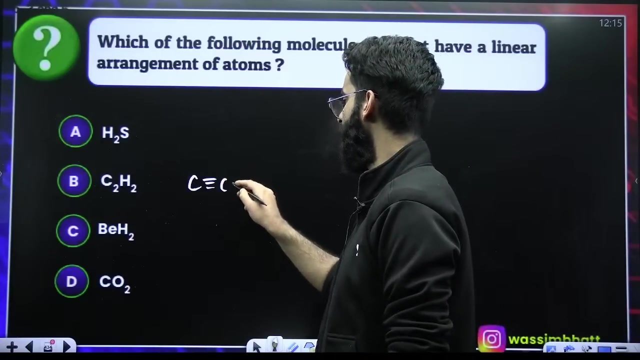 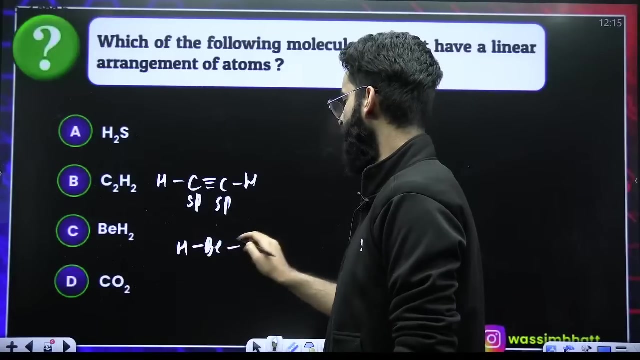 Correct: AB4L0.. Tetrahedral sp3. I think you have already seen the answer here. I think you have already seen the answer. which of the following molecule does not have the linear arrangement of atoms? c2h2, c2h2 sp, sp linear beh2, beh2 sp. hybridized linear carbon. 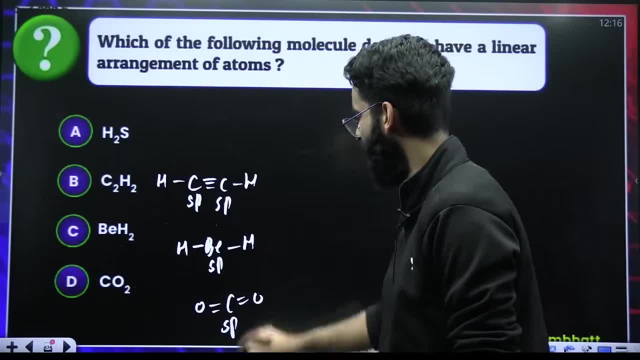 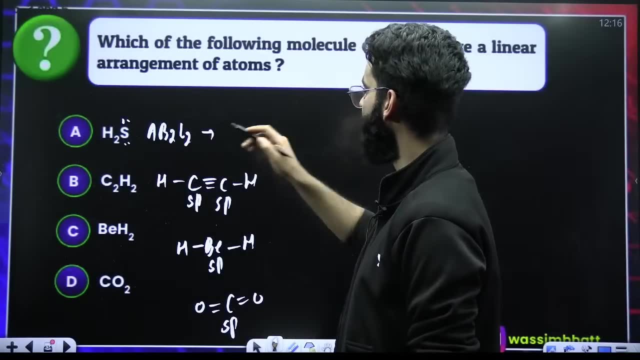 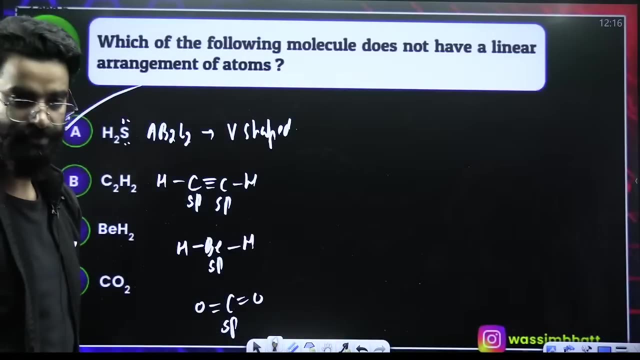 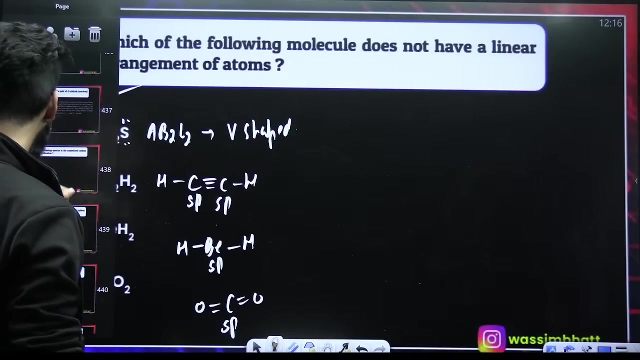 dioxide, carbon sp. hybridized linear. so all these are linear h2s. type of the molecule is ab2l2. ab2l2 means it is v-shaped. it is v-shaped, correct. it is v-shaped, it is v-shaped. tell me the answer of this question very quick. 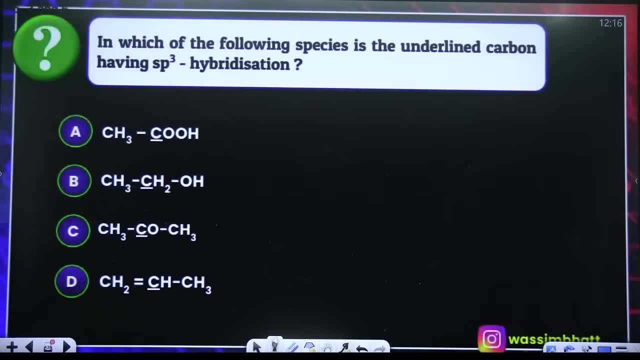 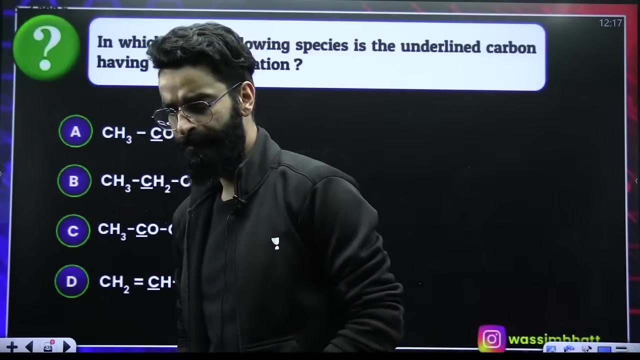 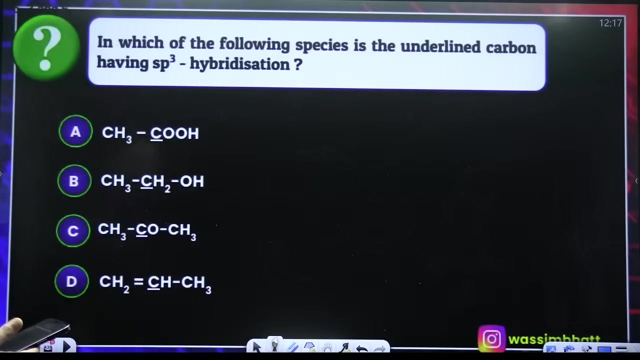 tell me the answer of this particular question very, very, very quick, quickly, guys, quickly, quickly quickly. sp3, Sp three, sp 3 equation is saying in which of the following species is the underlying carbon having sp3 hybridization? right quickly, I would want the answers in the chats everyone. 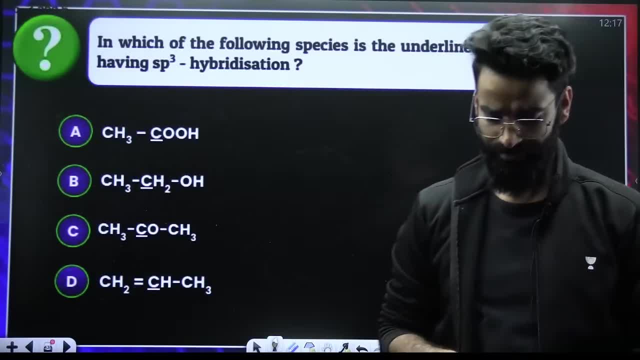 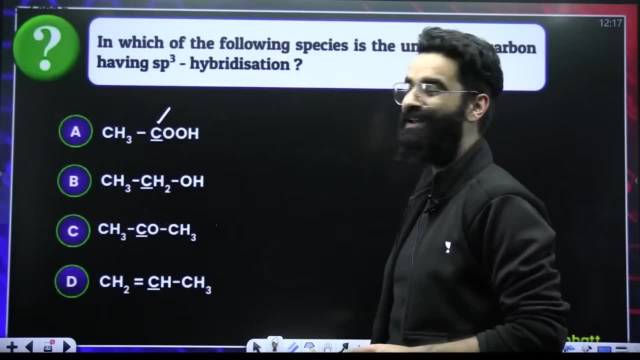 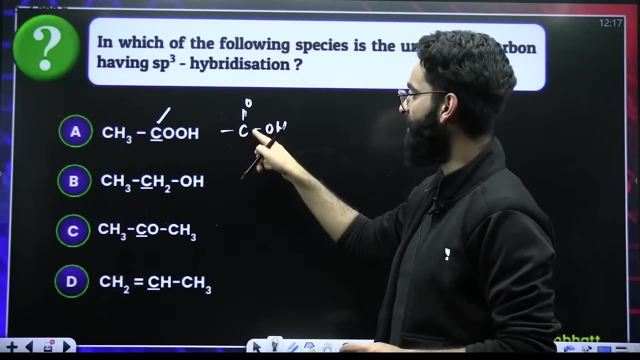 it is a very simple and basic equation, right, it is a very simple and basic equation, my dear students over here, if you look at this particular underlying carbon atom, it is basically C double bond OOH. right, It is basically C double bond OOH. So how many sigma it's forming? 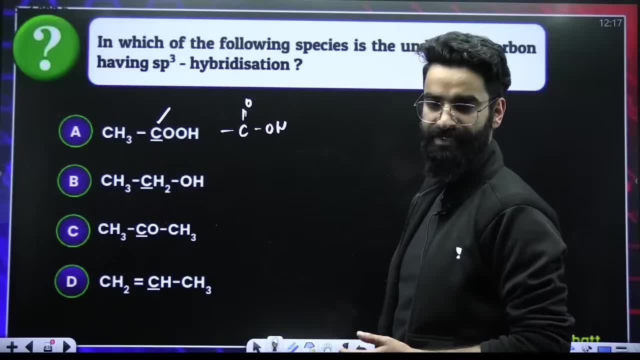 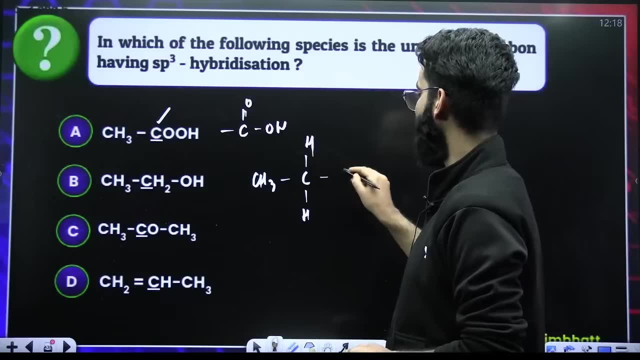 3 sigma, 3 sigma and 1 pi, So it cannot be SP3.. Look at this particular one: It is CH3, this is CHH, right, And this is OH. This is forming 4 sigma bonds, so it's definitely SP3. It is definitely. 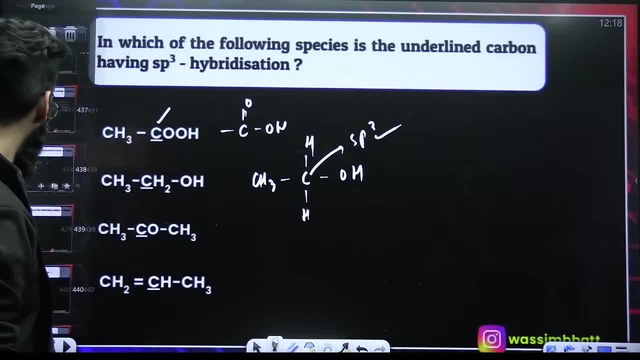 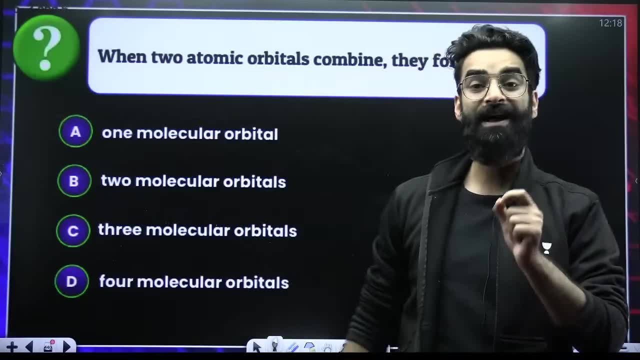 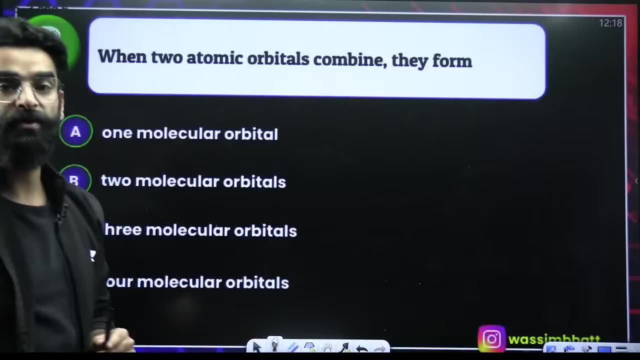 SP3, right. So the correct answer of this particular equation has to be option B. Look at this one. As I told you in the last session, the number of atomic orbitals combined is always equal to the number of hybrid orbitals formed. right Is always equal to the number of. 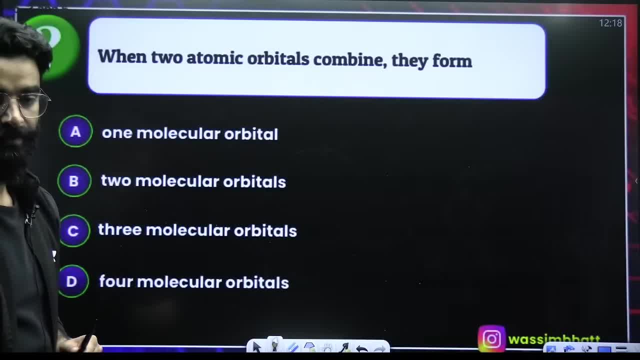 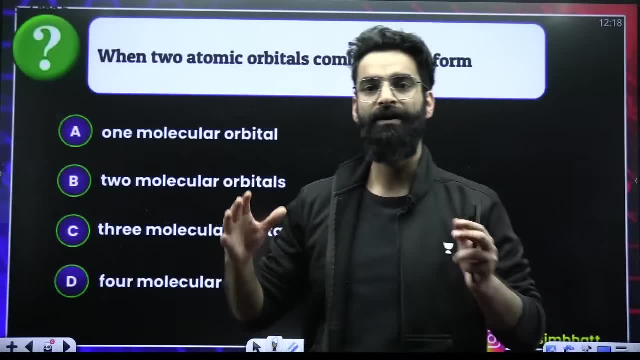 hybrid orbitals formed right. But over here the answer is not in terms of hybrid orbitals, it's in terms of molecular orbitals. Again, I told you in the last session, as the number of atomic orbitals combining is equal to the number of molecular orbitals formed, out of which few. 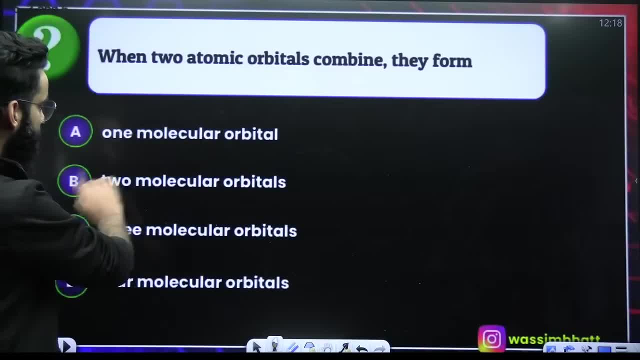 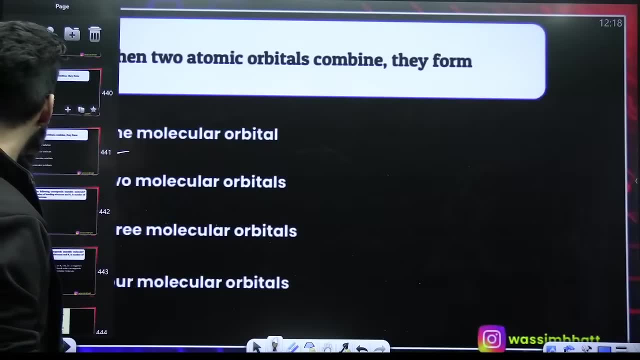 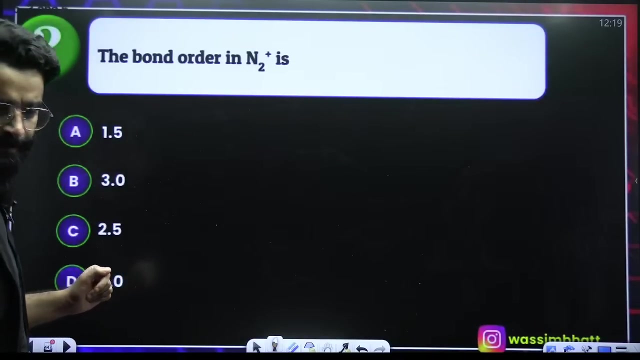 are bonding and few are anti-bonding. right, The two molecular orbitals are formed there. Perfect, The bond order of N2 positive. N2 positive is a 13 electron species. its bond order has to be 2.5, right, Its bond order has to be 2.5.. 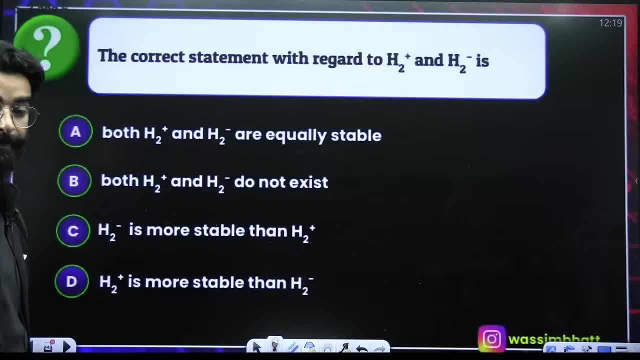 H2 positive and H2 negative. H2 positive and H2 negative. H2 positive and H2 negative. Quick, Quick guys. H2 positive and H2 negative. Which one is more stable? What do you need to do? 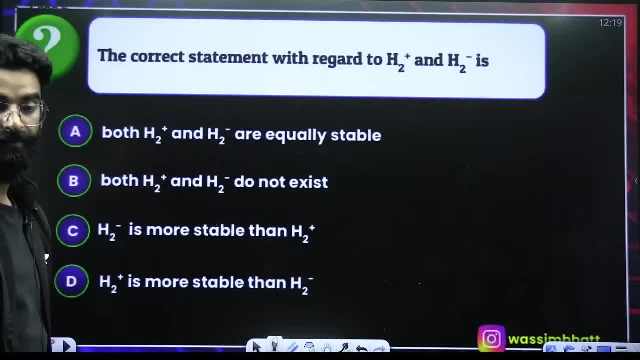 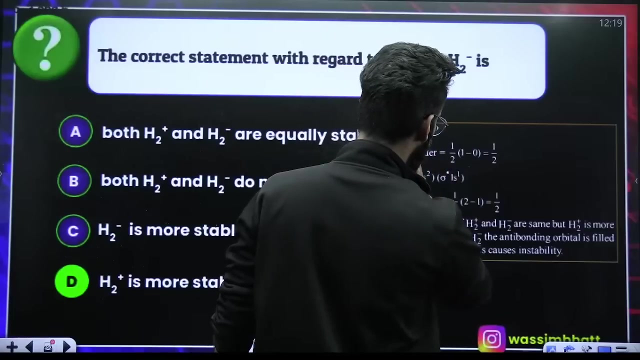 You need to write the molecular orbital configuration. You need to write the molecular orbital configuration. Yeah, Majority is saying option C. It is option D, It's option D. If you calculate the bond order of H2 positive, it comes out to be 1 by 2.. 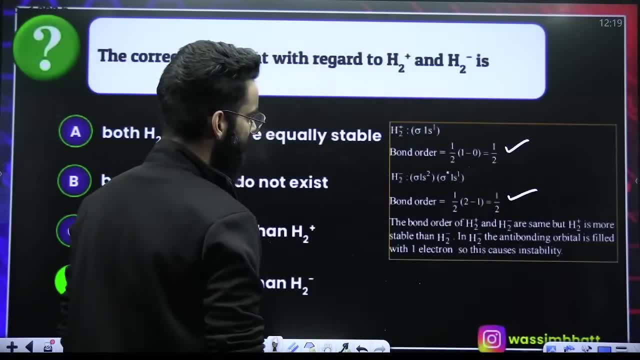 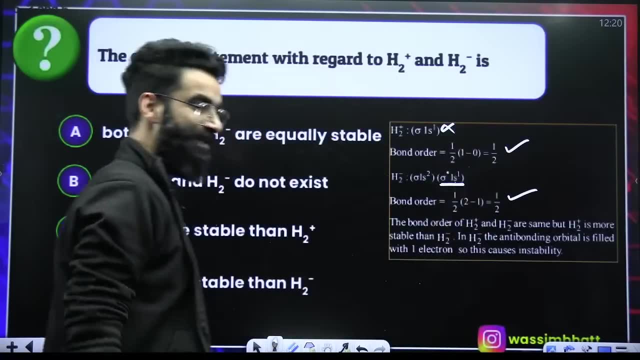 Bond order of H2 negative is also coming out to be 1 by 2.. But in case of H2 negative there is anti-bonding electron. Here you do not have any anti-bonding electron. More anti-bonding electrons means lesser the stability. 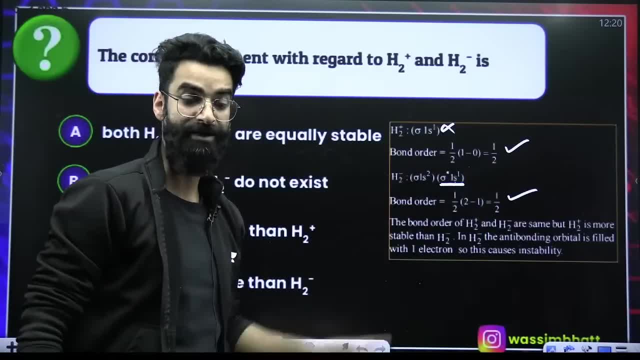 So H2 negative, H2 negative, is less stable than H2 positive, So H2 positive is more stable, H2 positive is more stable. right, Perfect, I have two more. I have told you in the last session, if you remember. 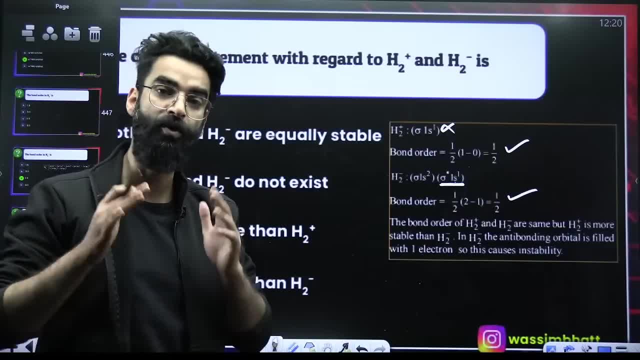 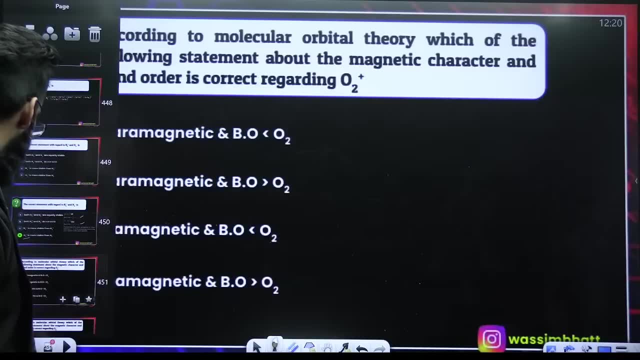 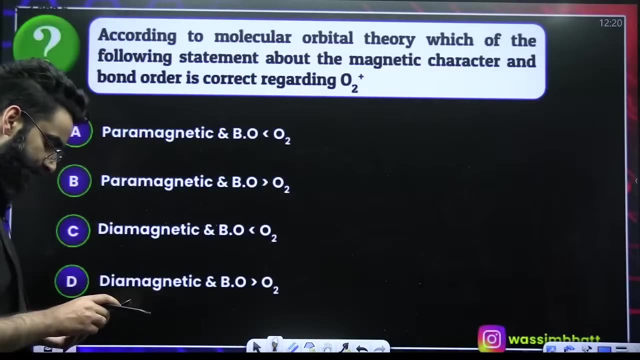 if bond order of two species is same, then look at the anti-bonding electrons. More the anti-bonding electrons, lesser the stability- Yeah, What about this one? What about this one Quick? What about this particular equation? 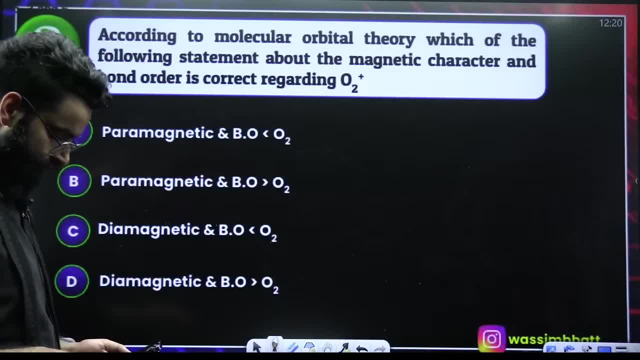 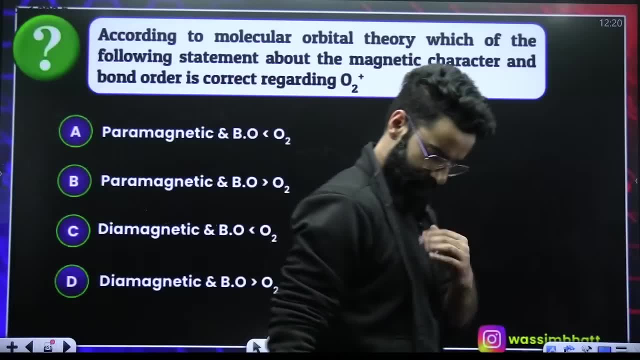 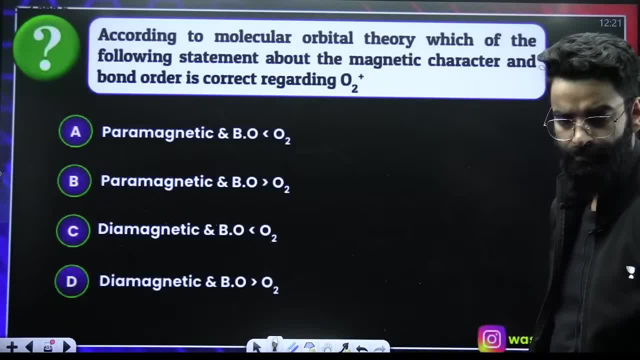 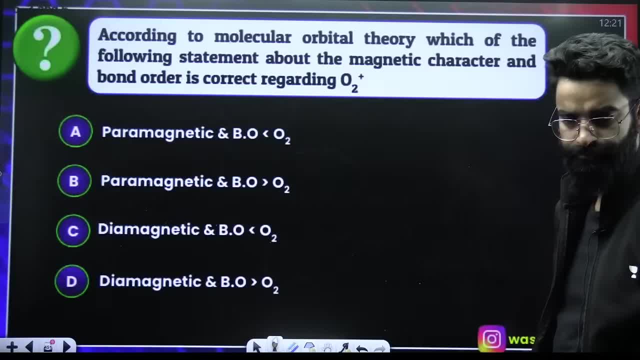 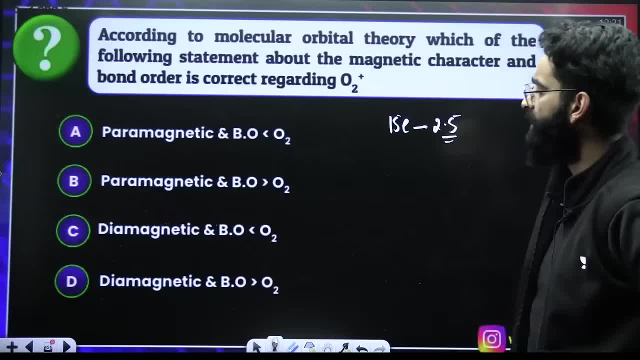 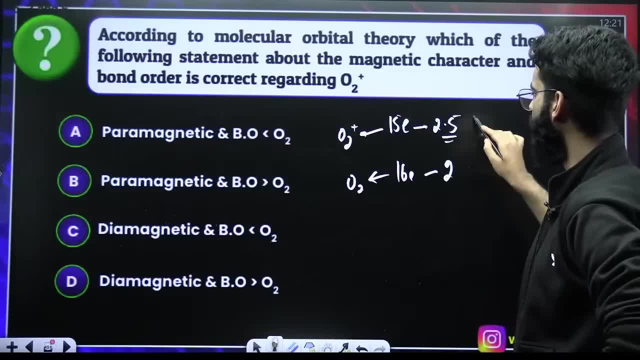 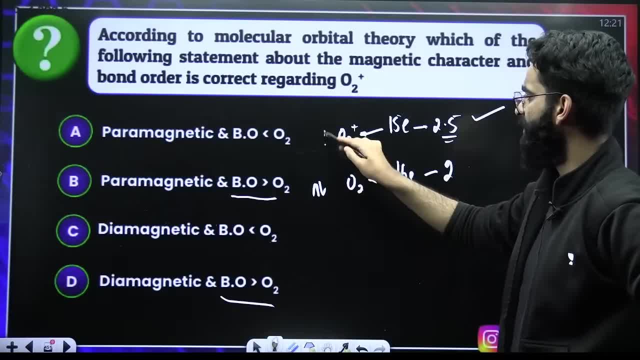 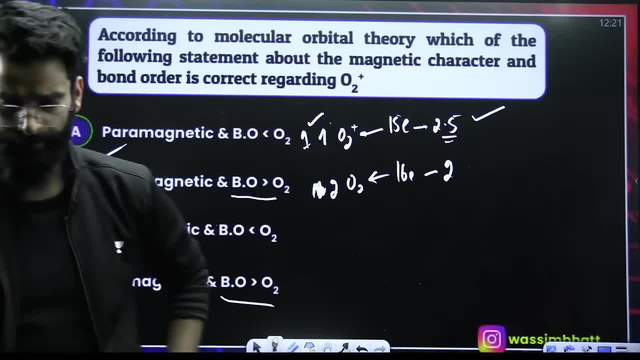 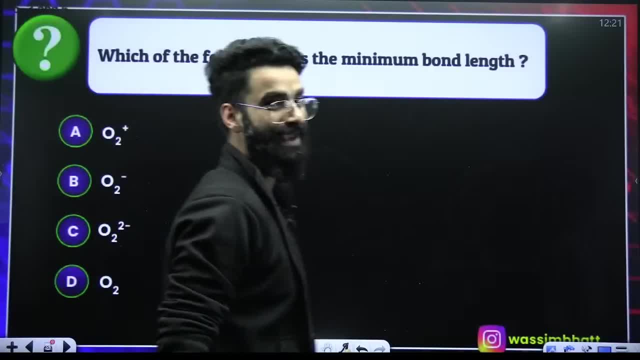 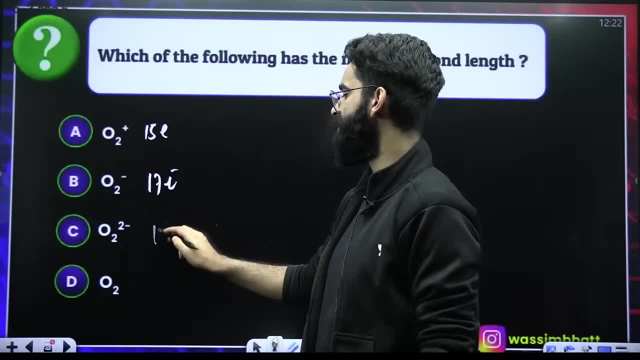 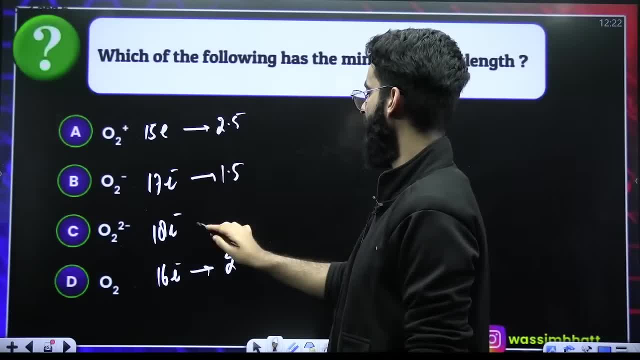 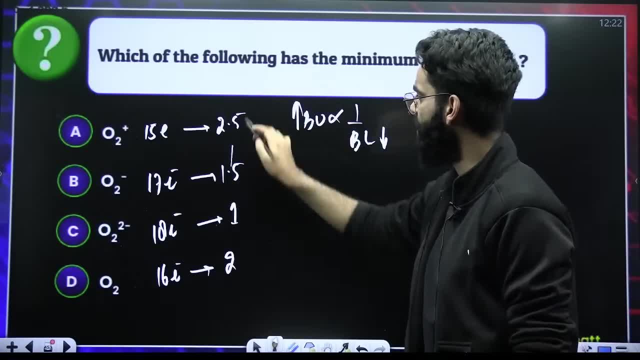 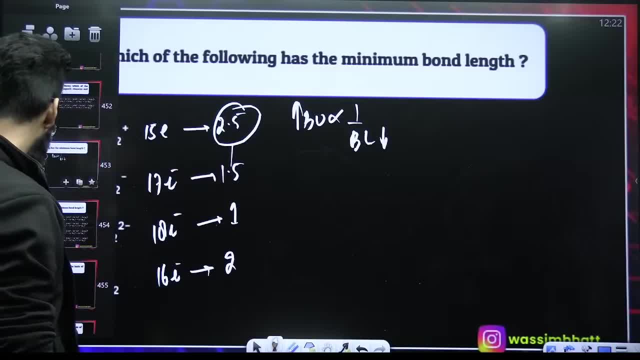 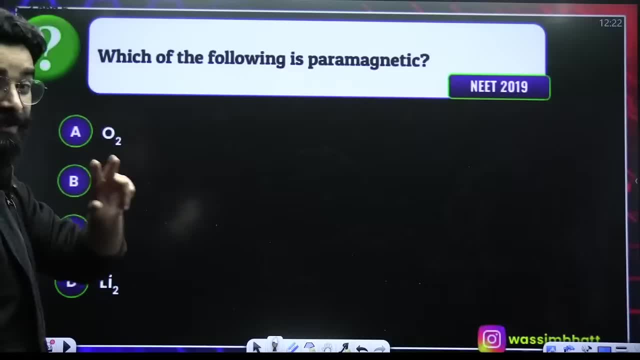 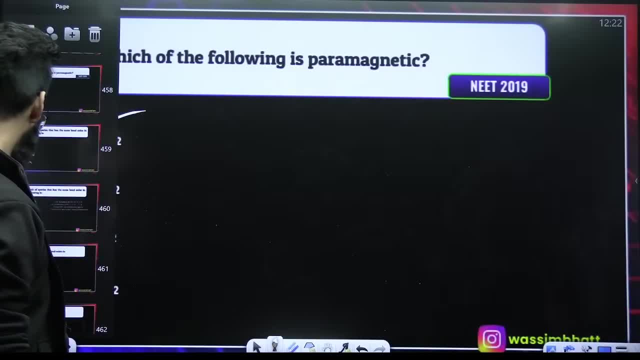 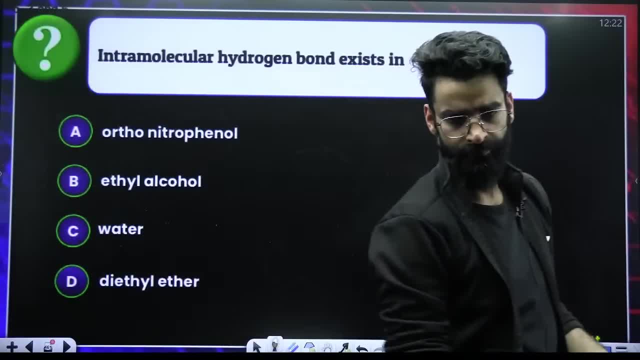 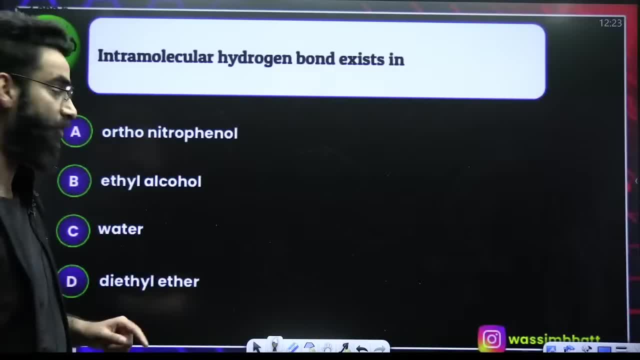 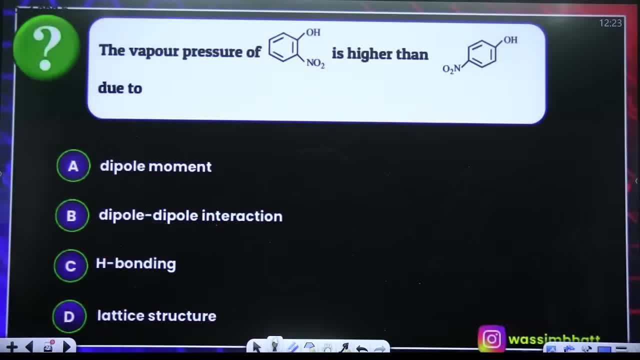 what do you think about this one? can you look at the question? the vapor pressure of this is higher than this. due to vapor pressure of first one is higher than the vapor pressure of second one. what is the logic? what is the logic? what is the reason? I can see majority is coming up with option c and you are absolutely right. it's option. 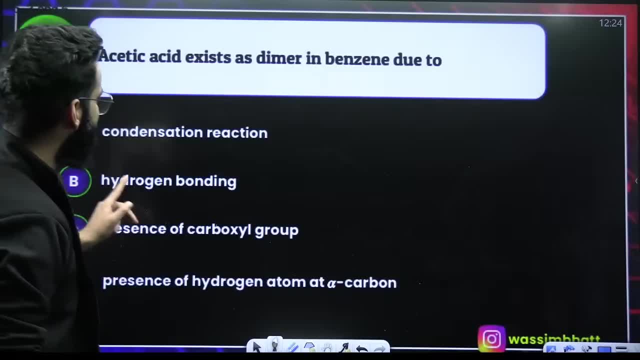 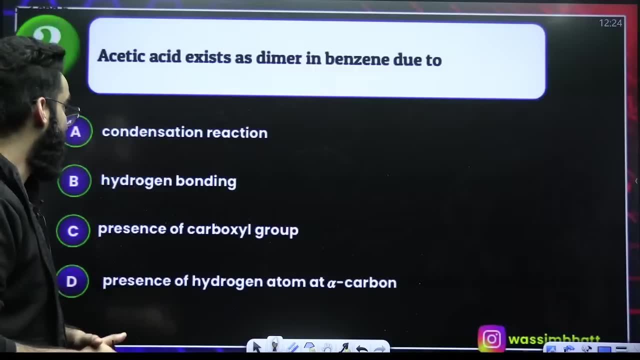 c. one more acidic acid exists as a dimer. that means two acidic acid molecules. they are forming one right, okay, acidic acids. acidic acid exists as dimer in benzene. why is that? why is that? why is that? because of hydrogen bonding? because of hydrogen bonding, yes, because of hydrogen bonding. 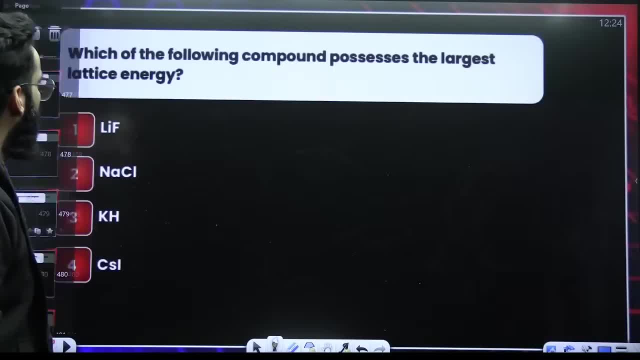 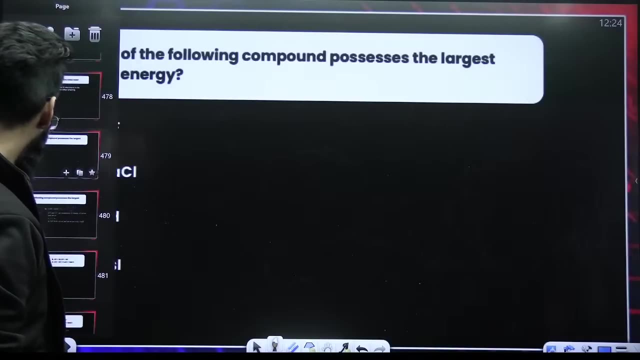 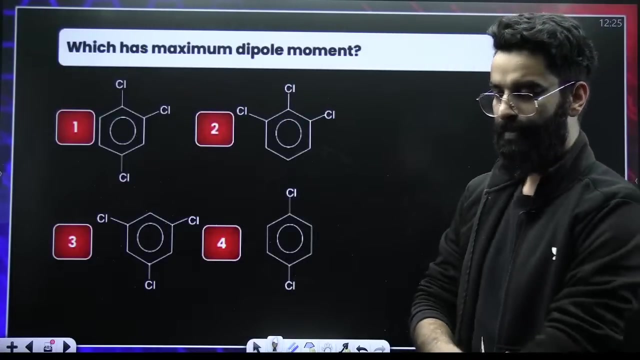 which of the following compound possesses the highest lattice energy charge? everywhere is same talk in terms of size: lesser the size, more the lattice energy. la positive has got least size among all these ketones. maximum lattice energy option: one option, one option. one which of the following has got maximum dipole moment? maximum dipole moment? this sort of 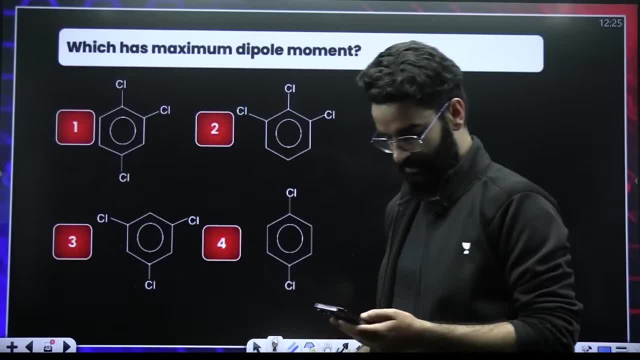 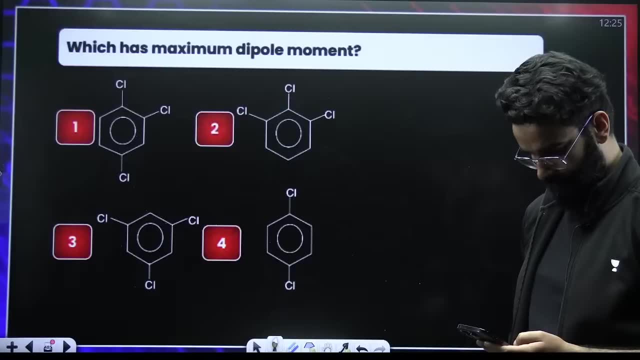 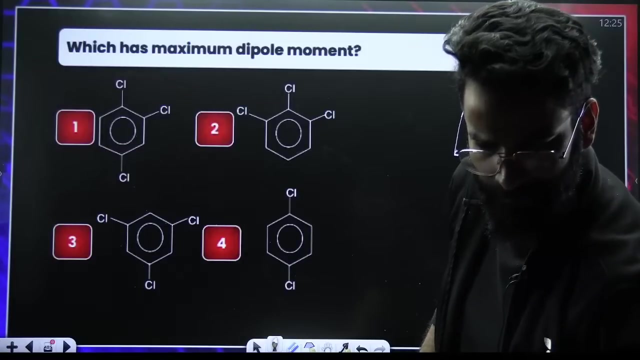 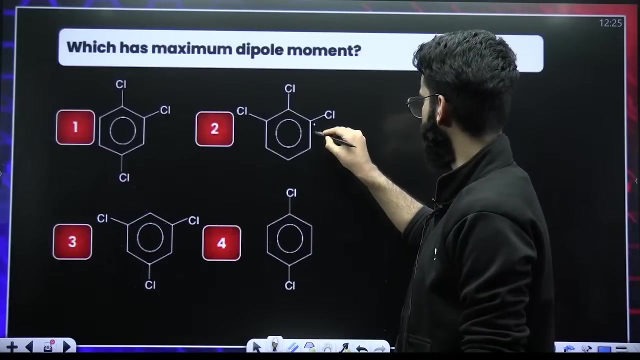 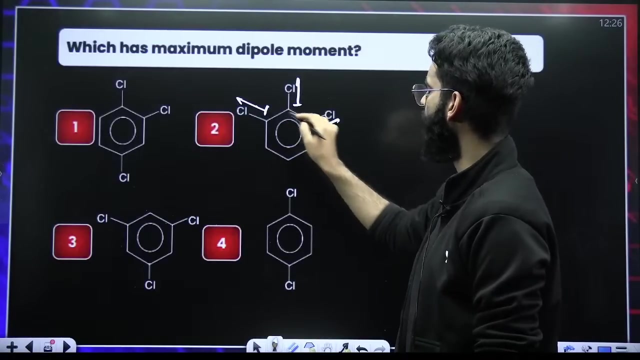 equation yesterday we have solved. I want you guys to give it a try and let me know in the chats quickly, quickly, maximum see. first of all, this is: this is sales, sales, sales, sales, sales, sales, electron withdrawing. so negative, positive, this direction, this is the direction. this is the direction these two, they are at an angle of what? 120 if. 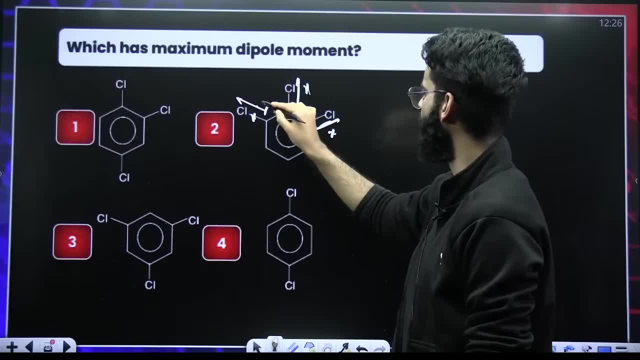 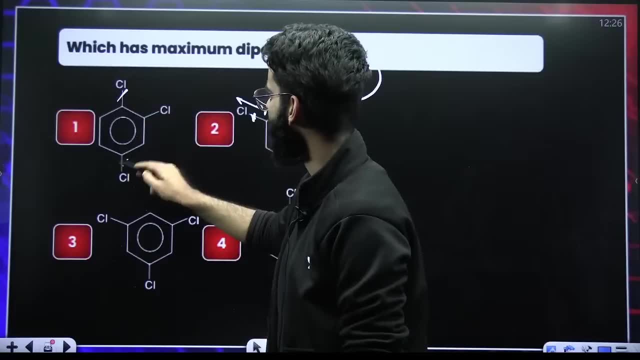 this is X, this is X, this is X. now, this one and this one. they are at an angle of 120, so the resultant will go in this direction, that will be X, X plus X makes it to X. right, this one, this one, cancelled out only X. perfect, the. 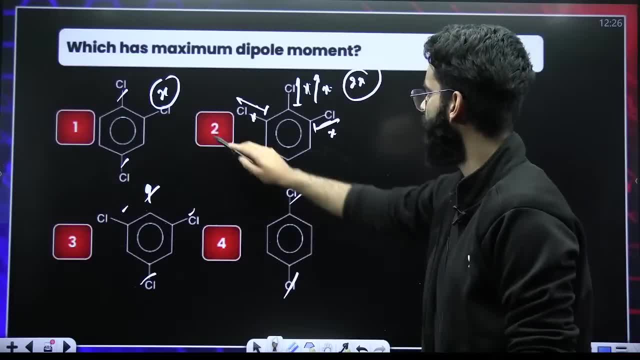 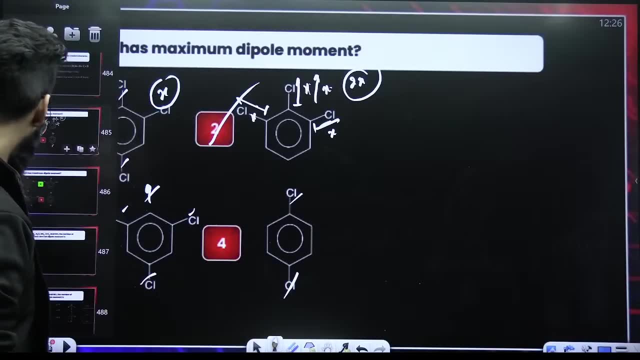 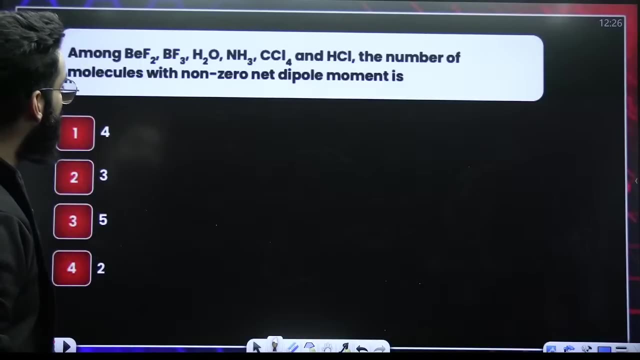 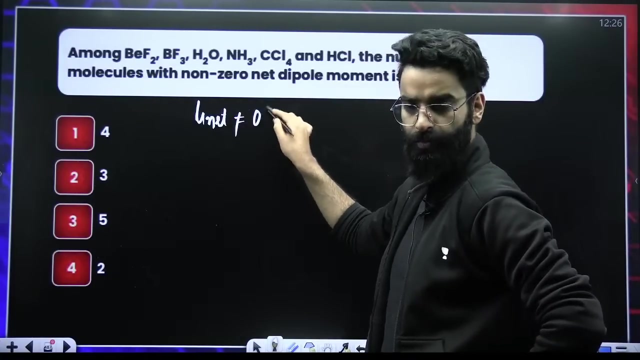 resultant of these two will be in this direction: net is zero, net is zero. option two: yeah, option two, option two: we have discussed all the stuff yesterday: the number of molecules with non-zero net dipole moment. how many species are there which have got net dipole moment to non-zero? non-zero. 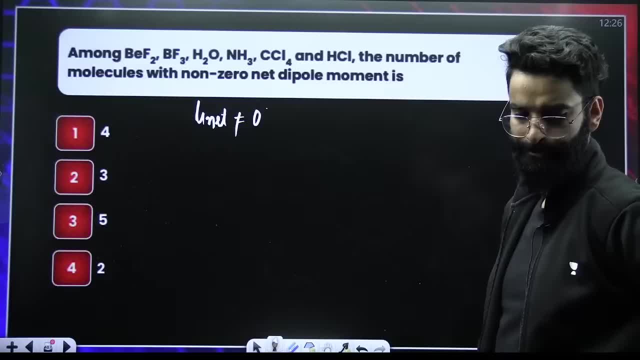 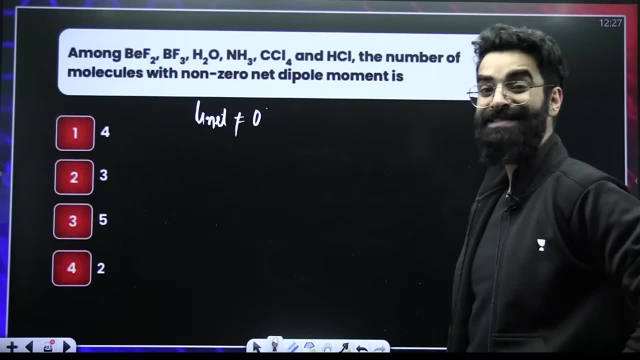 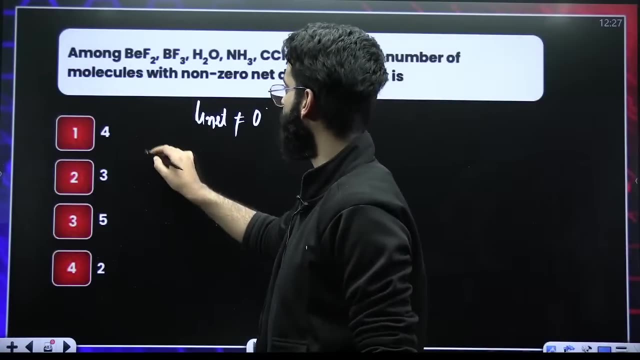 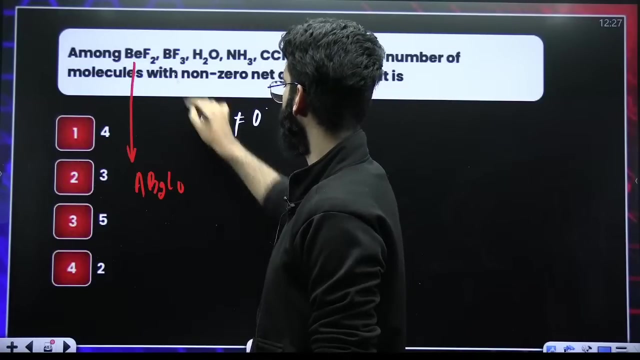 wake. I'll told you already the set of molecules which好 гар Zero dipole man right: AB 2 l 0. AB 3 l zero. v for l 0, v 5 l 0. let's check it out: bf2- if i talk about bf2, if i talk about BF to, it is a b2l 0. this is a bit real. 0. 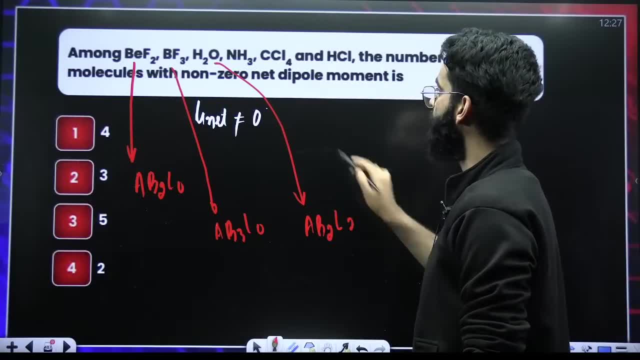 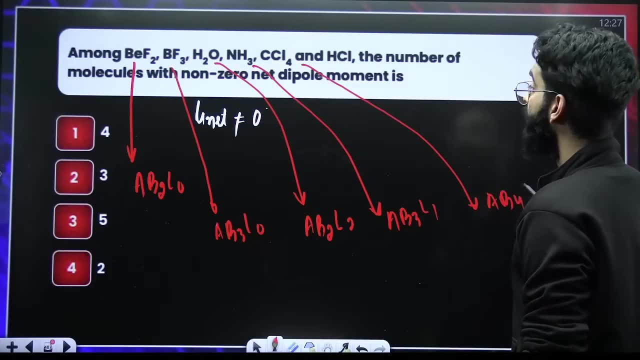 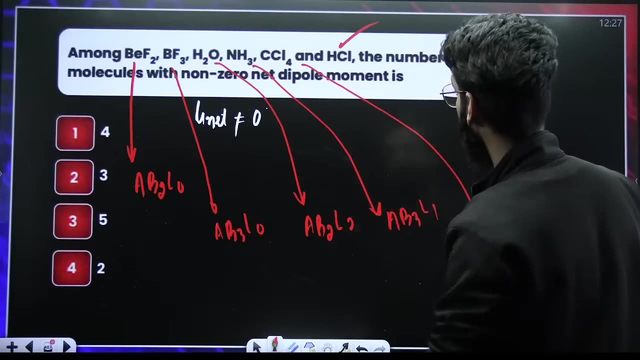 this is AB2L2,, this is AB3L1,, this is AB4L0, and HCl. we know it is already polar. What do we have to see? The number of molecules with non-zero. this is the molecule with non-zero. this is the. 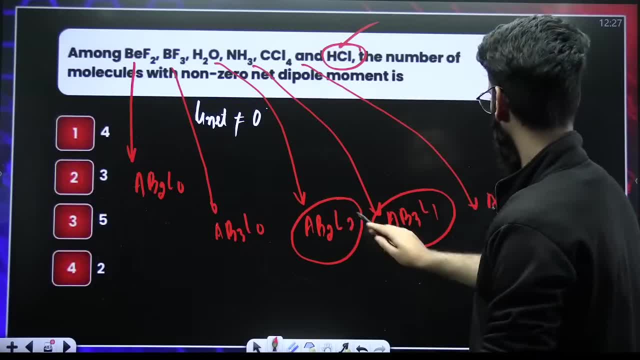 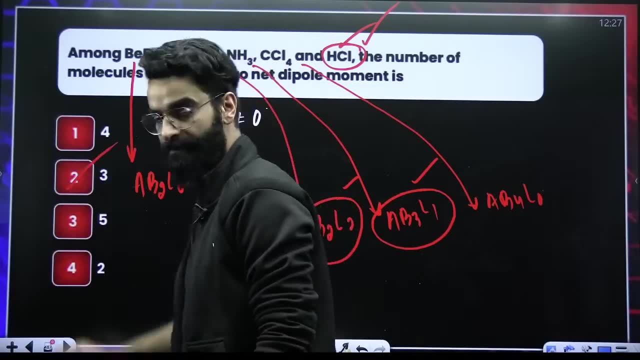 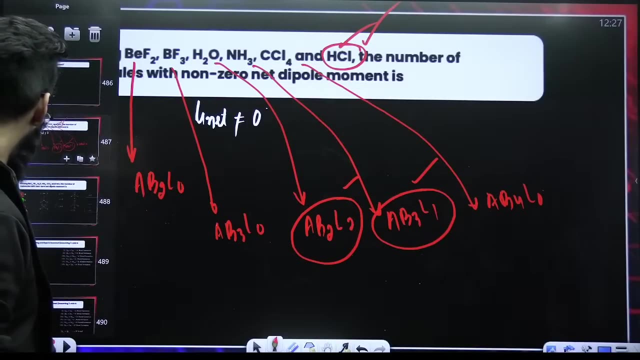 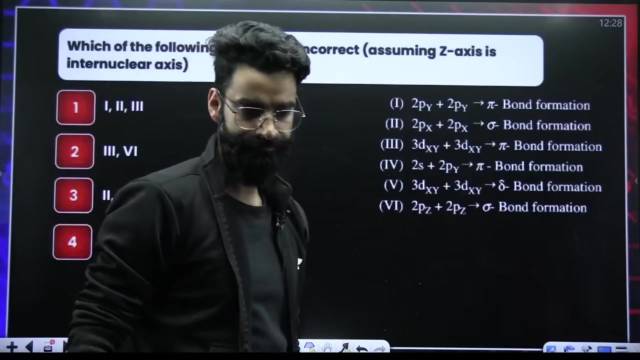 molecule with non-zero. this is the molecule with non-zero. so 1,, 2 and 3, there are 3 molecules which show non-zero. Perfect, I believe it's all clear to everyone. tell me the answer of this question. which of the 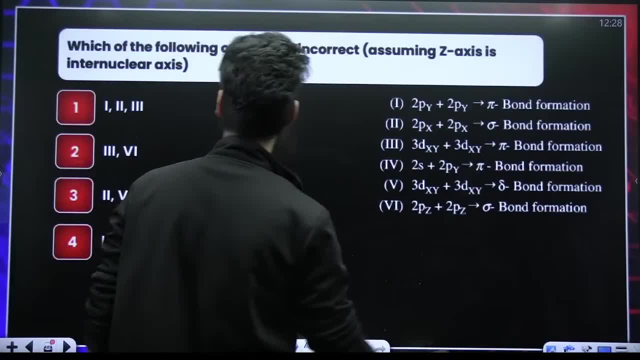 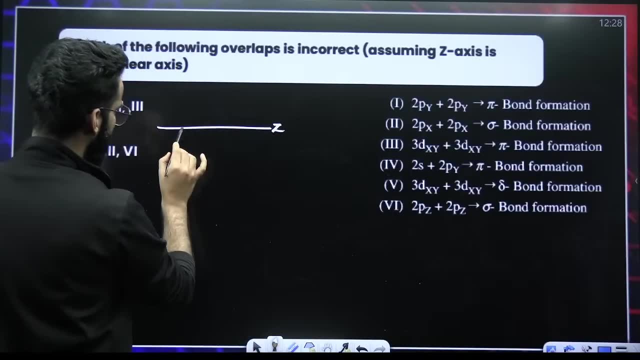 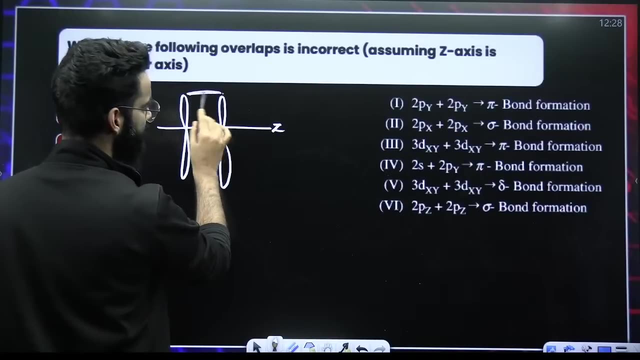 following overlap is incorrect, incorrect, incorrect. if Z is the internuclear axis, this is Z, for example. which is the internuclear axis? right, this is Z. now Py and Py. this is, for example, your Py. if this is Z axis, then let's call this as Py, Py and Py they. 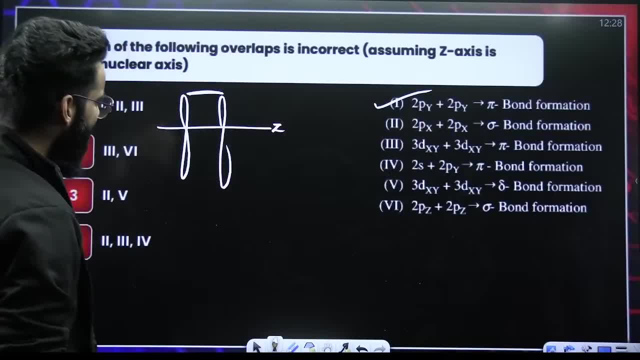 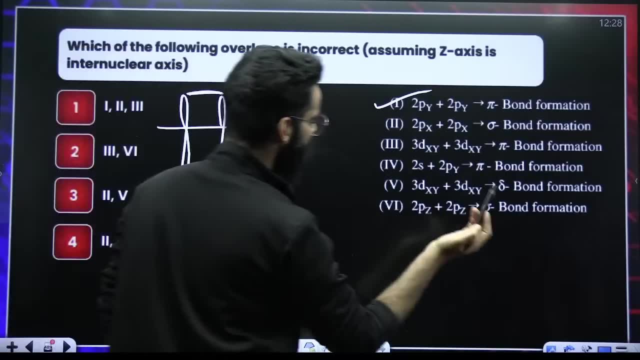 are going to form Py bond, so 1 is correct: X and X. if this is Z, this will be X and this will be X, X and X. what do they do? They do parallel overlapping right. parallel overlapping means Py bond, so this is incorrect. 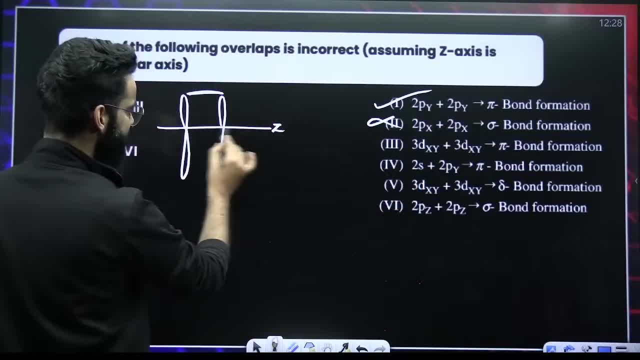 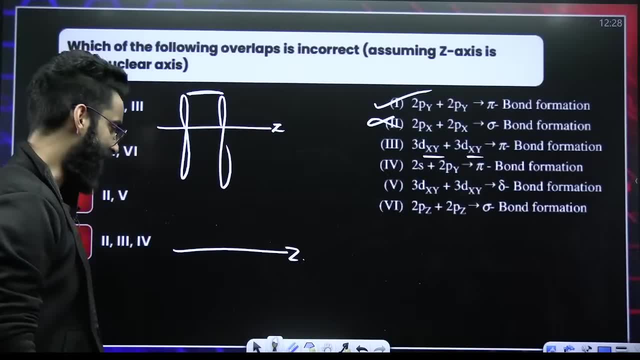 perfect. If this is, if Z is the internuclear axis, Z is internuclear axis. we have got Z as the internuclear axis. Now: 3DXY, 3DXY, 3DXY, 3DXY. right, if this is Z. if this is Z, then XY plane is this: 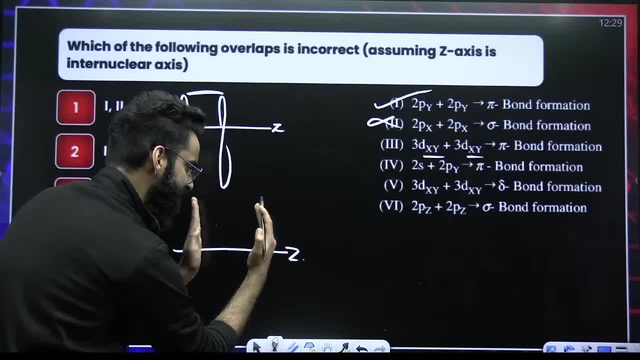 my hand is XY plane, this XY plane, so 3DXY, 3DXY. there will be 2 lobe interaction or 4 lobe interaction. see, this is 2 lobe interaction. this is 4 lobe interaction, 4 lobe interaction. 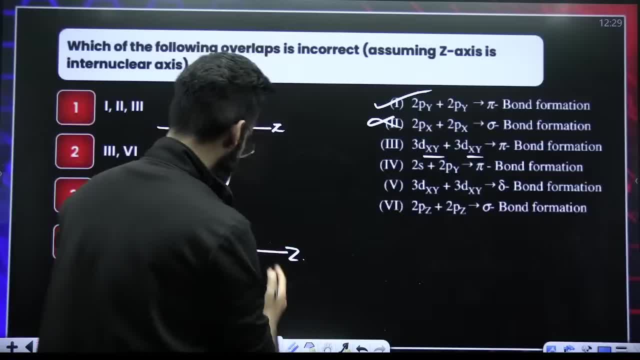 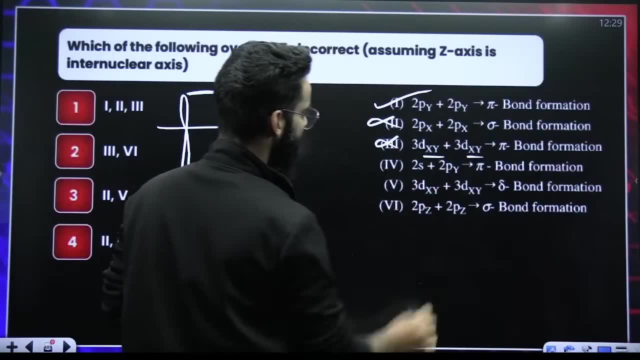 means delta bond. 2 lobe interaction means Py bond, right. so over here 3DXY. 3DXY will show 4 lobe interaction. they will form delta bond. so this is wrong. 2S, 2P. 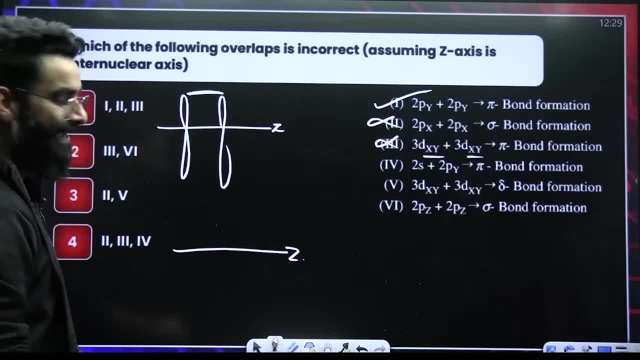 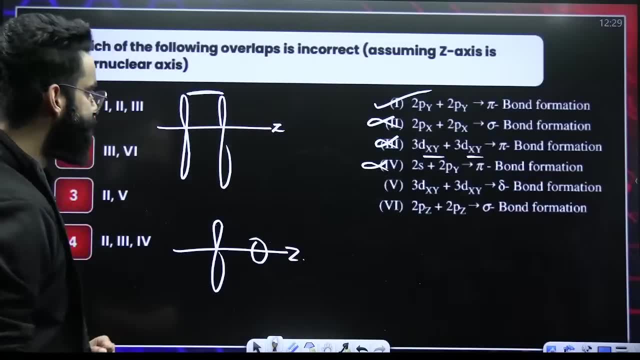 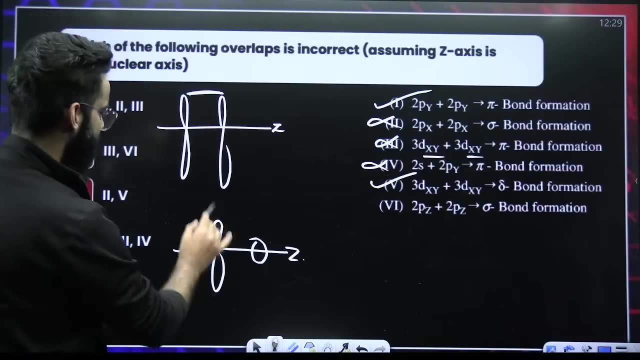 2S, 2P, 2S. this is S and this is P. what will happen? bond formation no 3DXY- 3DXY. they are going to form delta bond: 2PZ- 2PZ. if this is Z axis. if this is Z axis, this is your 2PZ. 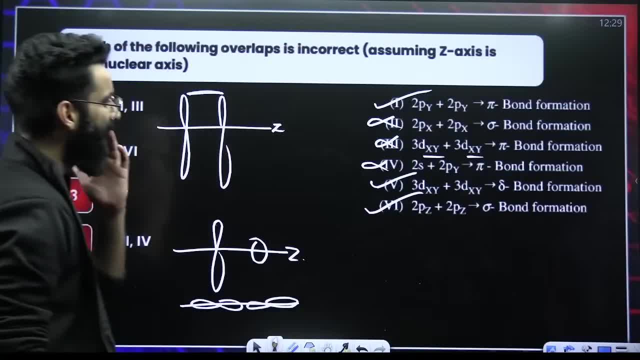 this is 2PZ. it is head on overlap sigma, so this is right, right. so how many are wrong? 2, 3, 4,. 2, 3, 4 is the answer right. 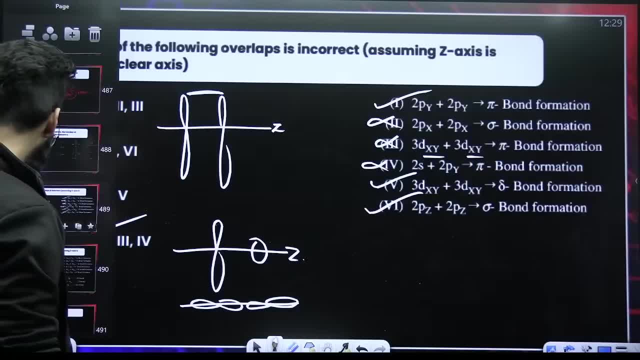 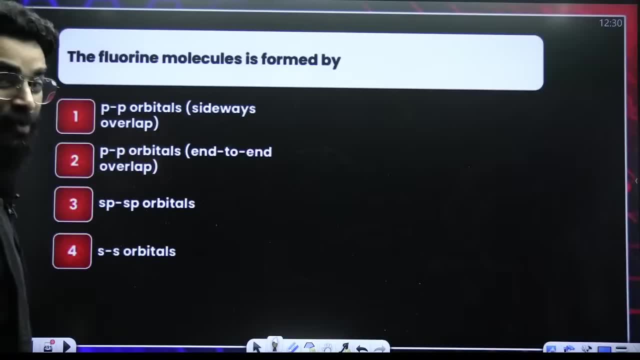 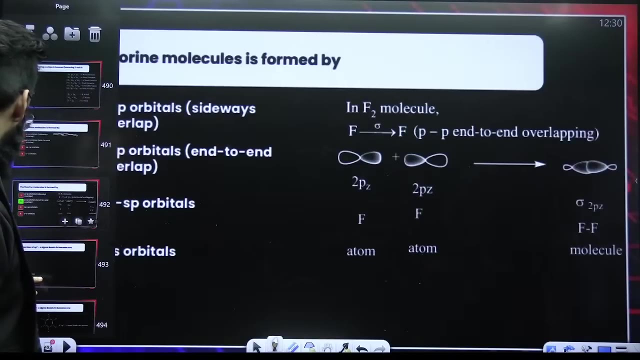 I believe I am all clear. okay, fluorine molecule is formed by yesterday. we have seen in VBT this is the form of PP overlap: PP head on overlap. PP end to end overlap right PP end to end overlap. this is discussed already. 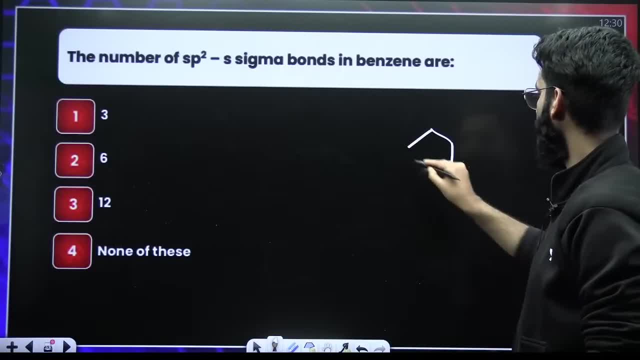 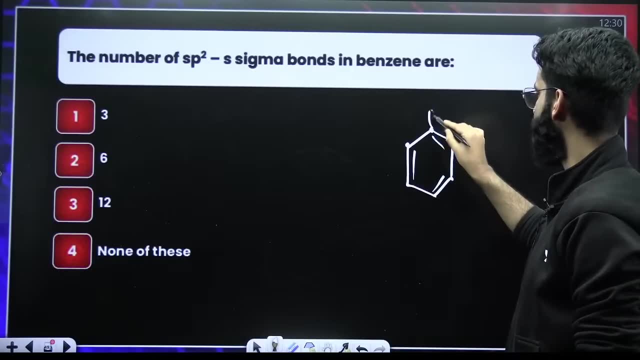 The sp2s sigma bond, the sp2 s sigma bond in benzine. in benzine, all of the carbon atoms are sp2, so sp2, hybridized sp2, sp2,, sp2, sp2, sp2, there is an hybrid orbital here. 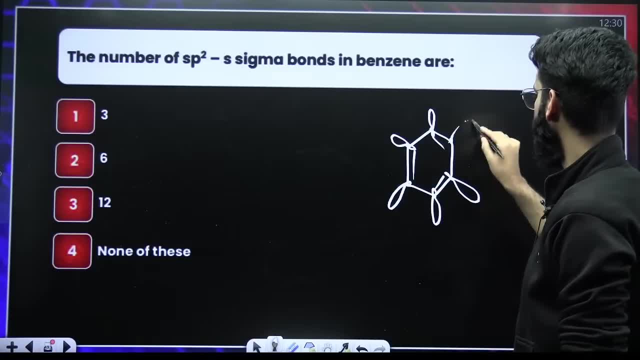 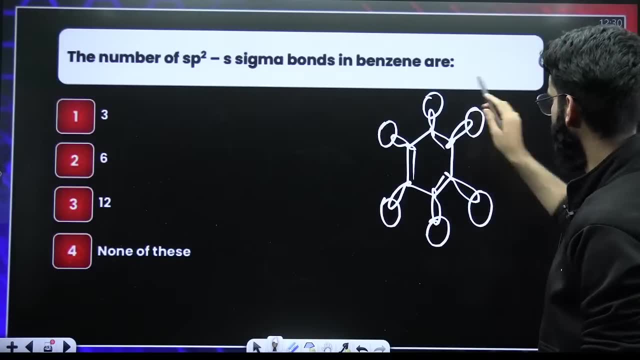 hybrid orbital, hybrid orbital here, hybrid orbital, hybrid, hybrid orbital, as well as hybrid orbital. right now, one of the hydrogen will come from this side right, one from this side, one from this side, one from this side, so this overlap is sp2s, sp2s, sp2- hybrid orbital of benzene. i mean sp2- hybrid orbital of carbon. 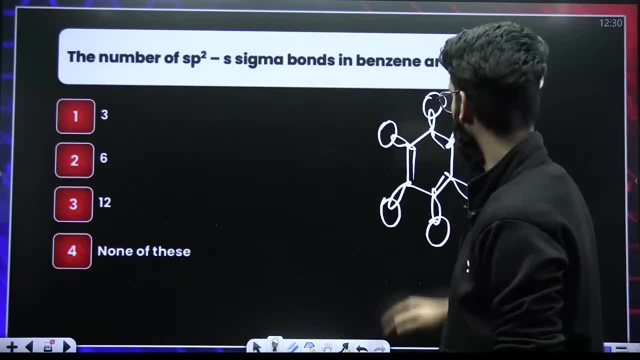 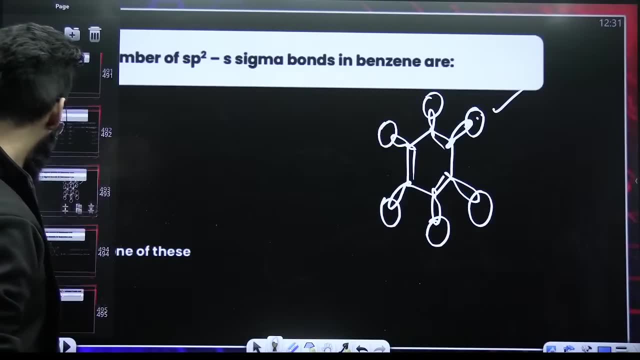 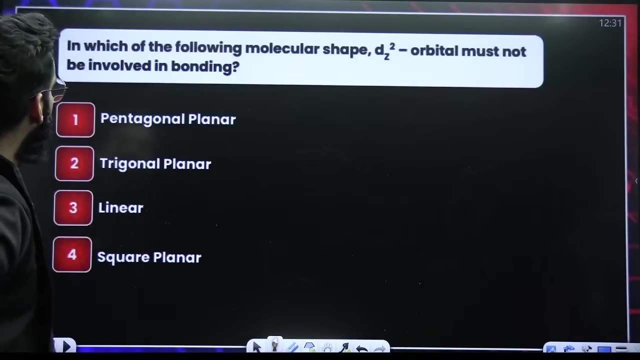 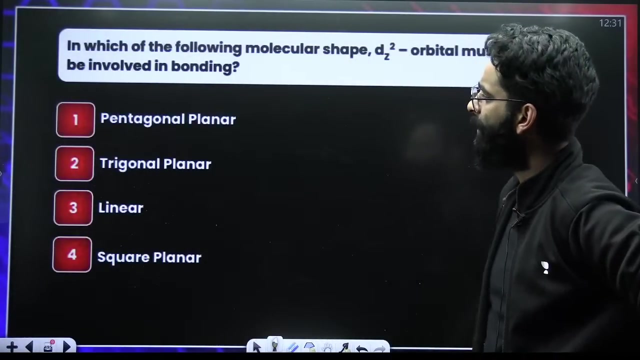 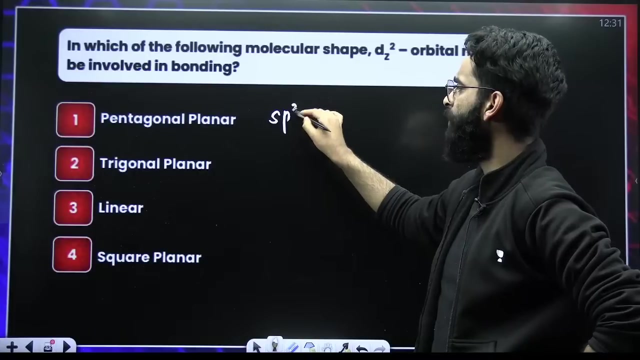 and s orbital pure s orbital of hydrogen. so this is sp2s. so how many? one, two, three, four, five, six. so six sp2s. okay, six sp2s. in which of the following molecule: dz square orbital must not be involved in bonding dz square. dz square in pentagonal planar. pentagonal planar hybridization will be, anyways. what? 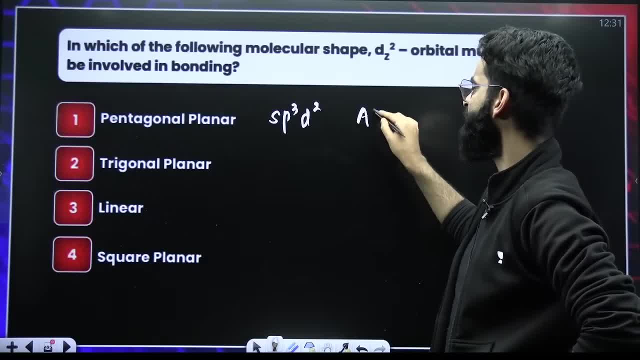 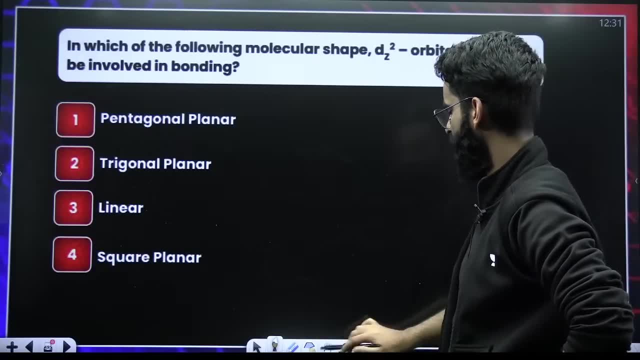 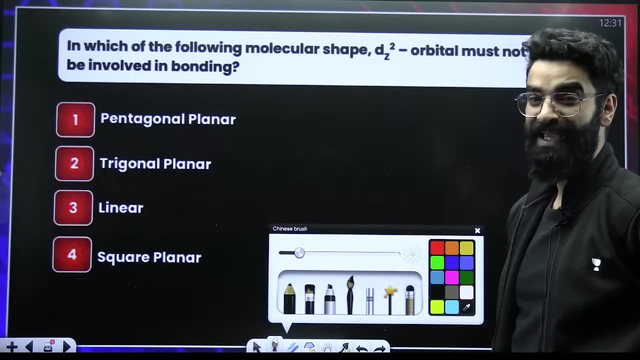 pentagonal planar: sp3d2. pentagonal planar means a b pentagonal planar. okay, wait just a second. what is going to be pentagonal planar? like your square planar, it is a- b5 l2 a, b5 l2 a. 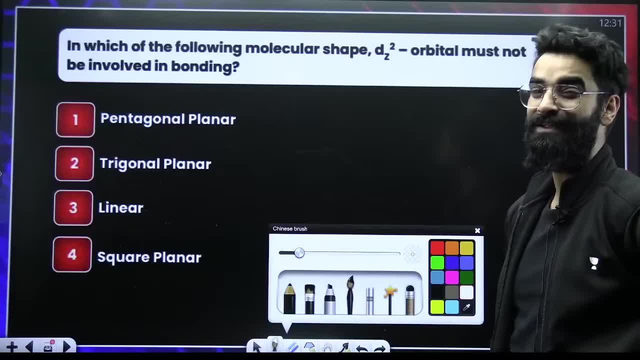 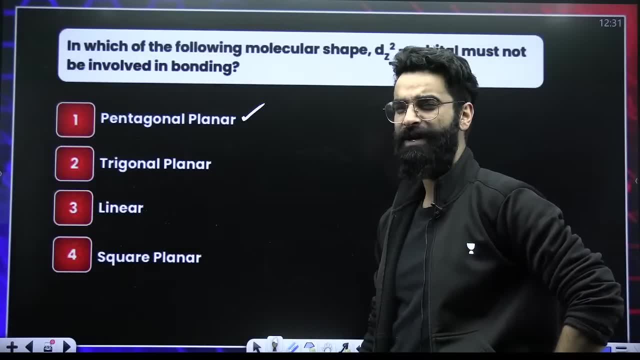 b5 l2, 5 plus 2, 7 straight number, 7, sp3, d3. dz square is involved there. dz square is involved there. in case of linear is dz square involved. linear it can be a b2 l3. a b2 l3 is linear. 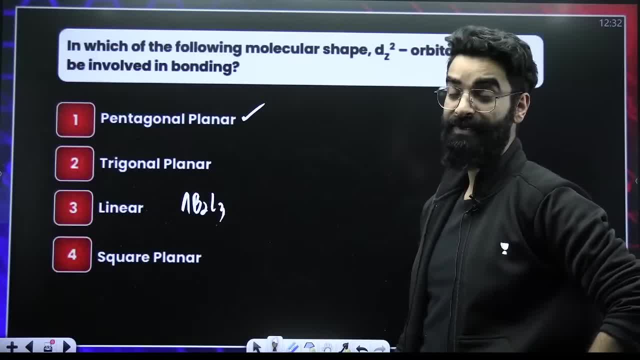 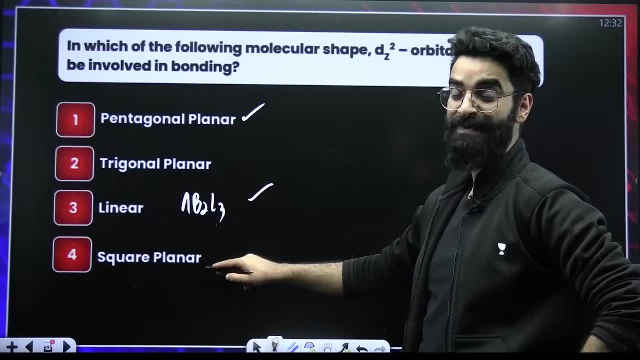 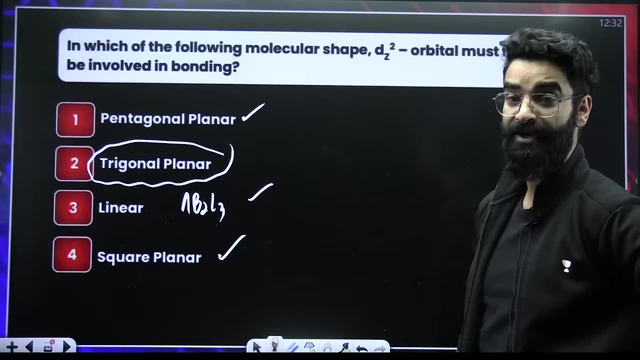 right. a b2 l3 is linear. be careful with this. a b2 l3 is linear. perfect hybridization. sp3d dz square is involved: square planar. sp3d2 dz square is involved only trigonal pyramidal. is there right trigonal pyramidal? is there a b3 l1? a b3 l1 hybridization? 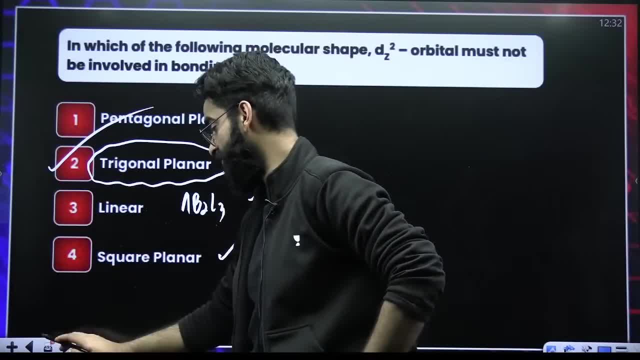 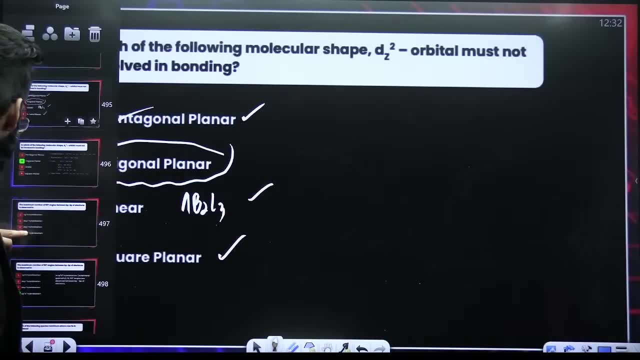 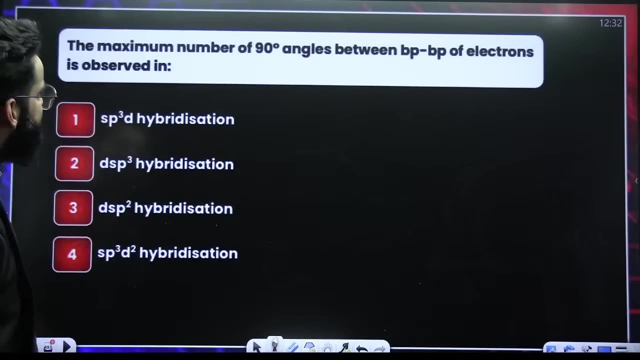 is sp3. that is the only one wherein dz square is not involved. so option two is the one that's correct. option two is the one which is correct. the maximum number of 90 degree angles between bond pair bond pair of electrons is maximum number of 90 degrees. this question also i have told you yesterday: maximum 90 degrees. 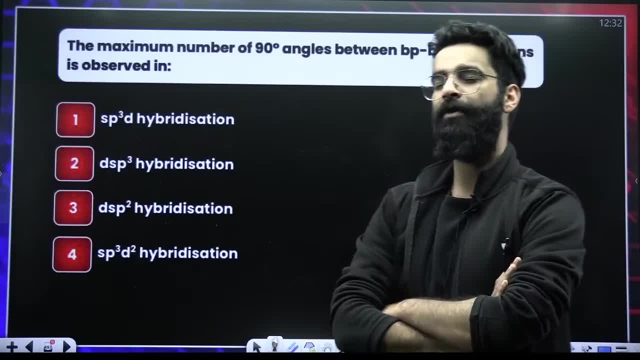 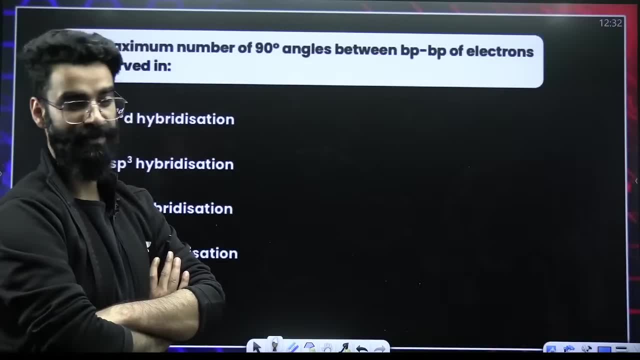 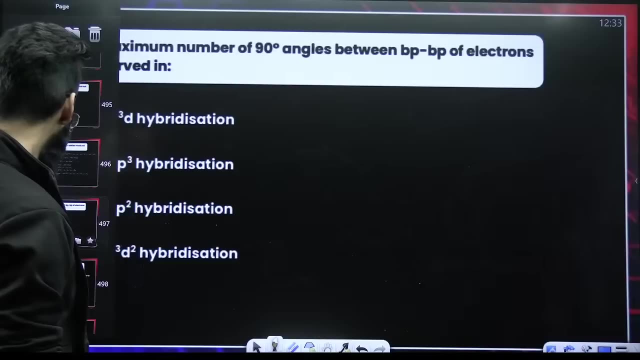 between bond pair, bond pair. it has to be what? between bond pair, bond pair? it has to be sp3 d2, right octahedral, wherein there are 490 degrees between bond pair, bond pairs, right here, right octahedral, and you have to be down, it has to be in the center of the matrix. 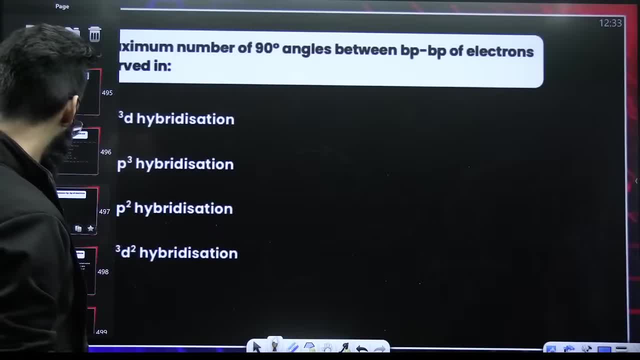 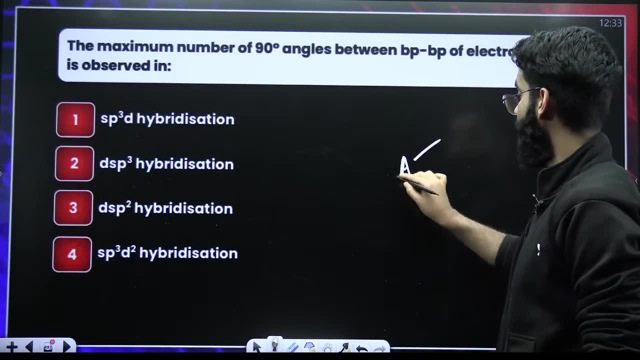 right here. right, and thisiels is not working here. the spectrograph is working here and this is how long it is. sp3d dz square is involved, right, and you have to be down. it has to be right. so when you have this 10 to 20 degrees between bond pair, bond pair, it has to be in. 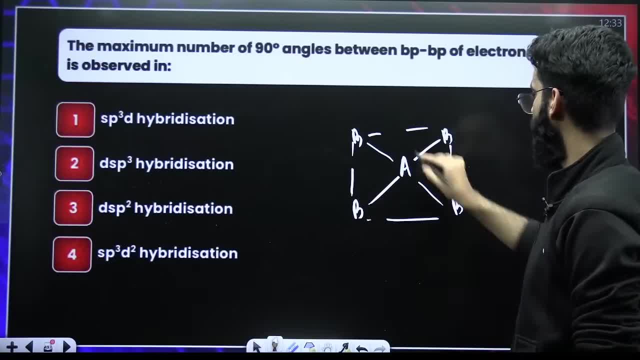 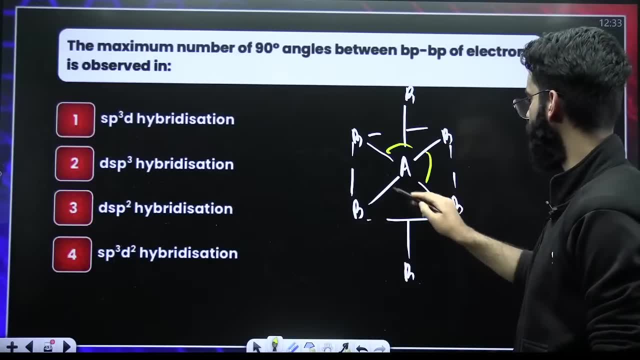 the center of the matrix. sorry i was. this is like this. just a second. i don't know what Perfect. this is B. this is B In this equatorial plane. how many 90 degrees are there? This is 1,, 2,, 3,, 4, right. 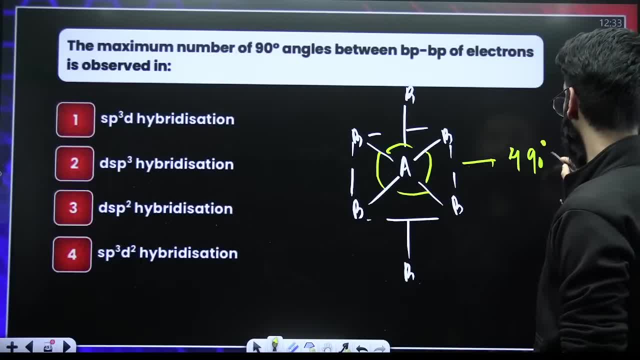 In the equatorial plane there are 4, 90 degrees. perfect. This is forming. this bond is forming 4, 90 degrees from top. this bond is forming 4, 90 degrees from bottom. So in total there are 12 90 degrees right. 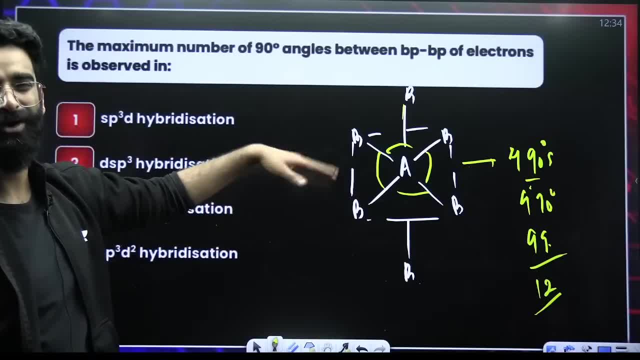 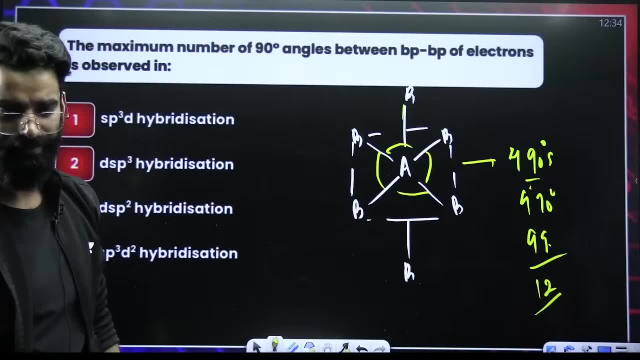 So perfect. they are not asking about axial-axial-axial or axial-equatorial or equatorial-equatorial, they are asking about general bond, pair-bond, pair. right, It is 90 degree. perfect, It is 12, 90 degrees basically. 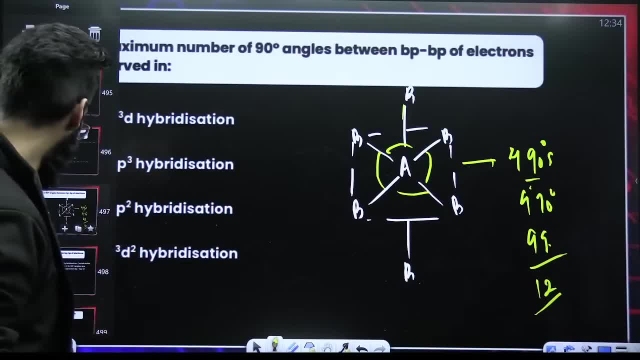 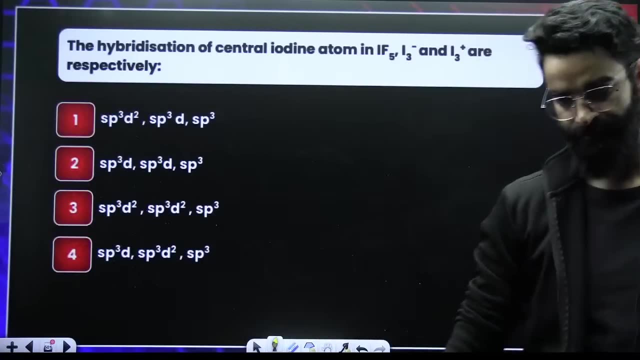 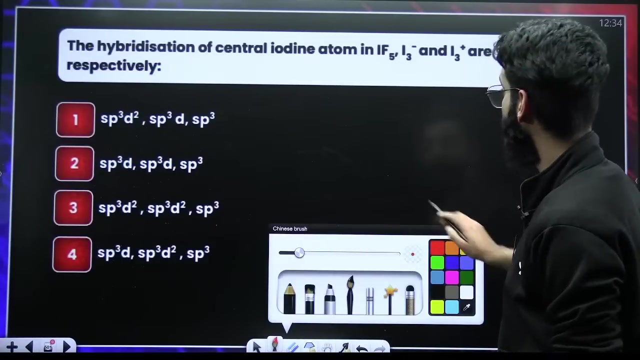 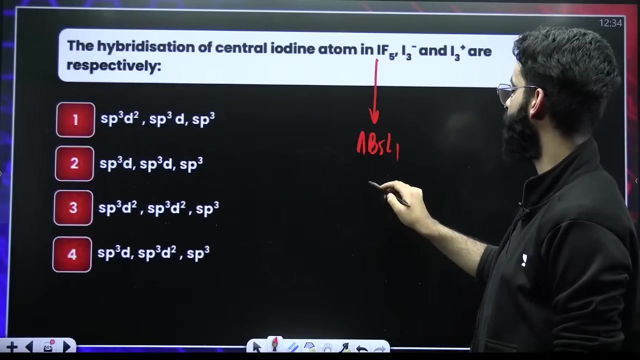 If you remember, yesterday, I have told you the same thing, right? We discussed all this in detail yesterday. quick, Okay, guys. hybridization of the central iodine in IF5, in IF5, in IF5, AB5L1,, SP3D2, AB2L3,. 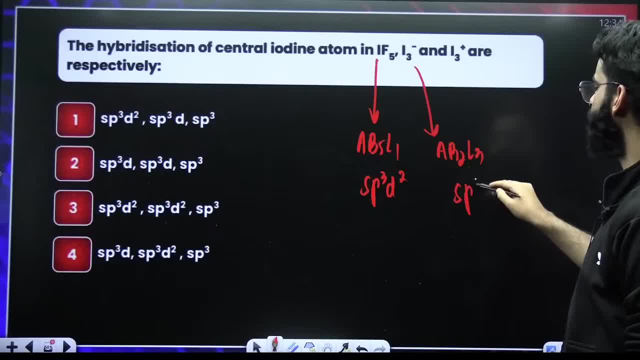 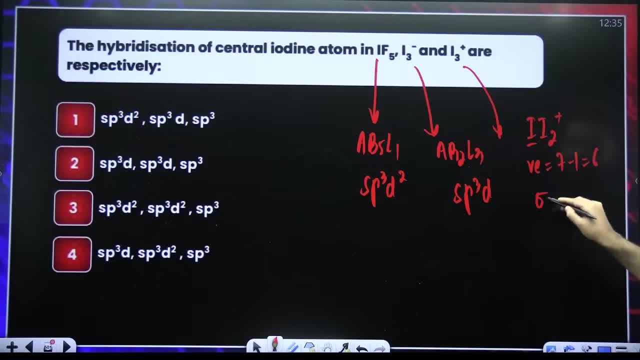 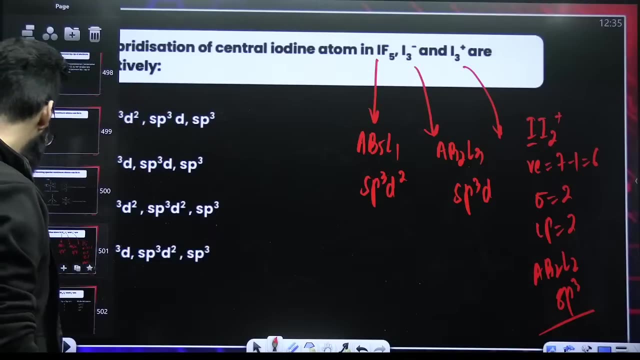 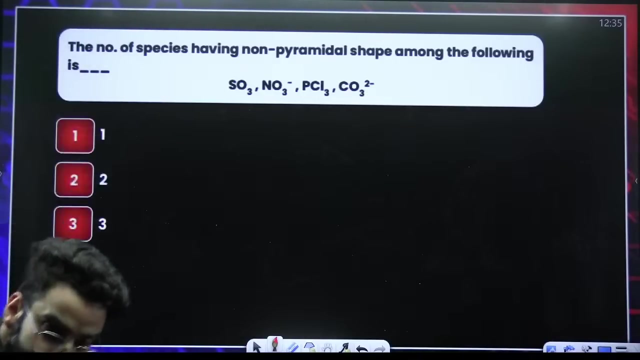 Correct, Done. These are here the similar type of questions. just a second. what is the answer of this question? what is the answer of this question? you know, till now, we have solved 200 questions. by the way, till now we have solved 200 questions. 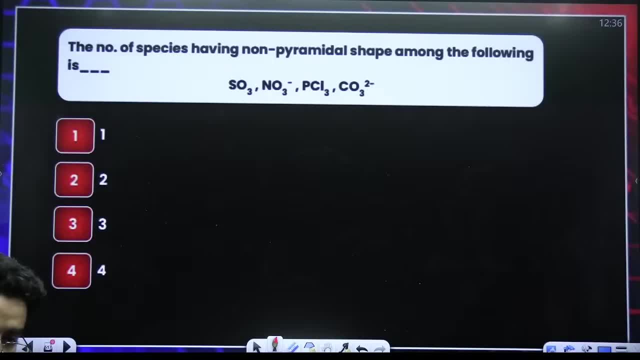 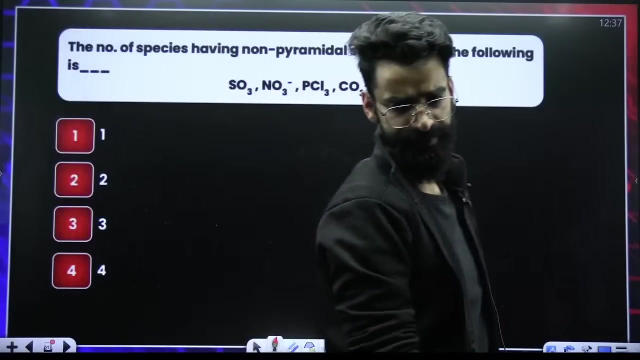 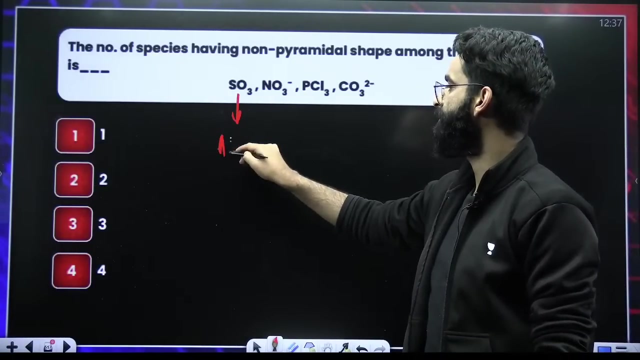 you know, till now, we have solved 200 questions. by the way, what is the answer of this one? quick guys, quick, quick quick. is it done? non-pyramidal: the ones which are not pyramidal: ab3l0, it is pyramidal no3, negative. 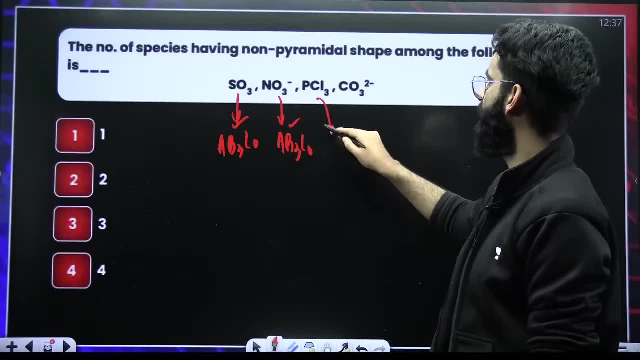 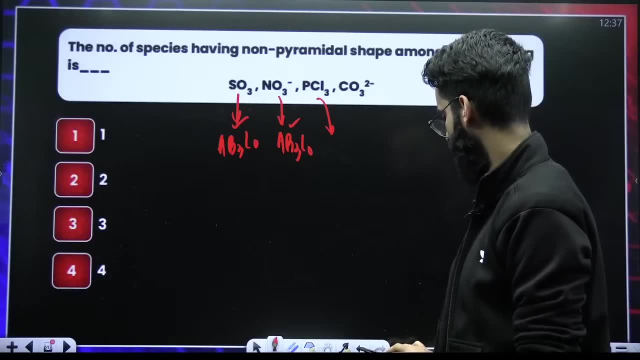 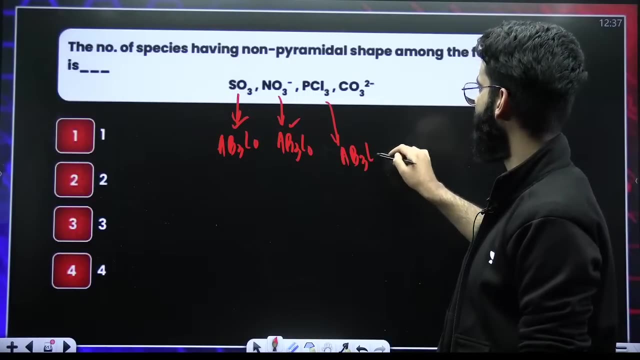 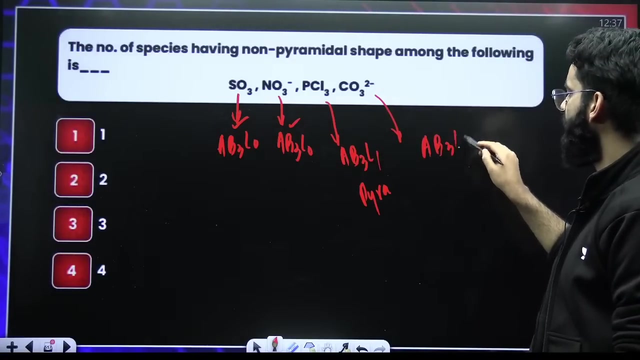 ab3l0. it is pyramidal, non-pyramidal. i mean non-pyramidal, this is non-pyramidal. this is ab3l1, this is pyramidal and this is ab3l0, non-pyramidal. 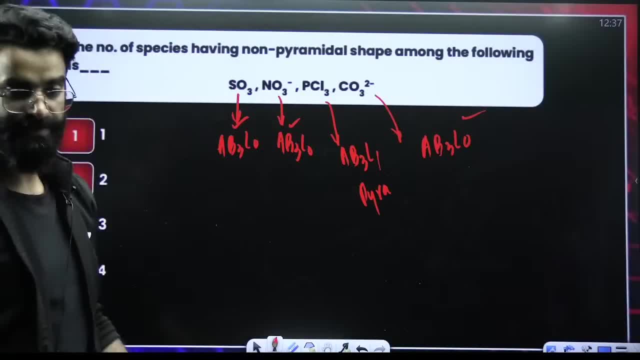 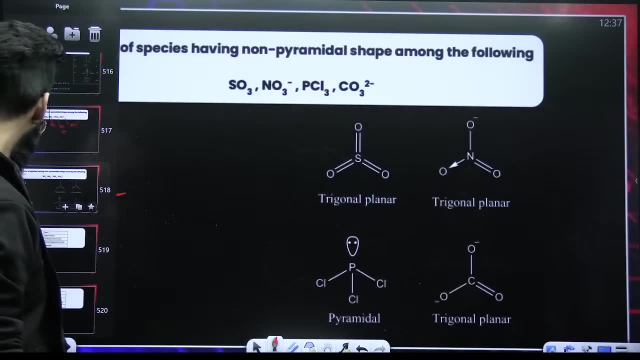 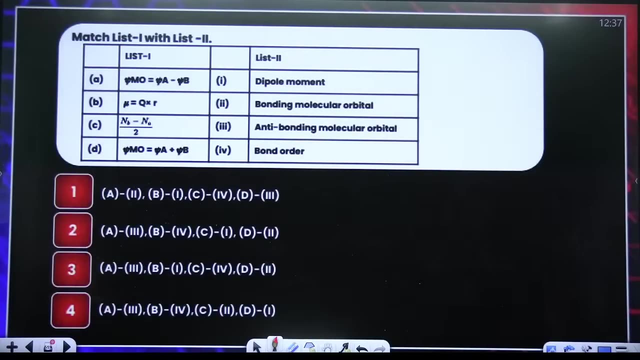 so there are three species which are non-pyramid. basically, there are three species which are not pyramidal. basically, ok, what do you think should be the answer of this question? what do you think is the answer of this question? quick, quick, first of all, psi a plus psi b. psi plus psi b, that means constructive units. 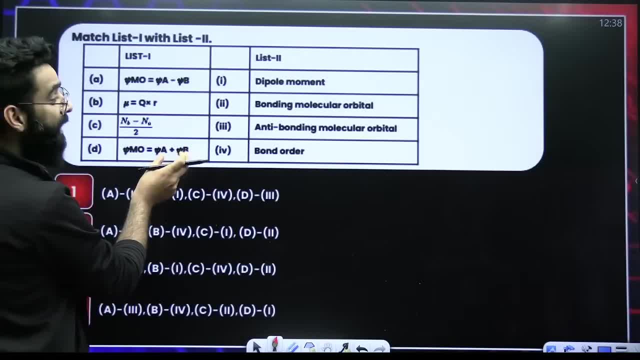 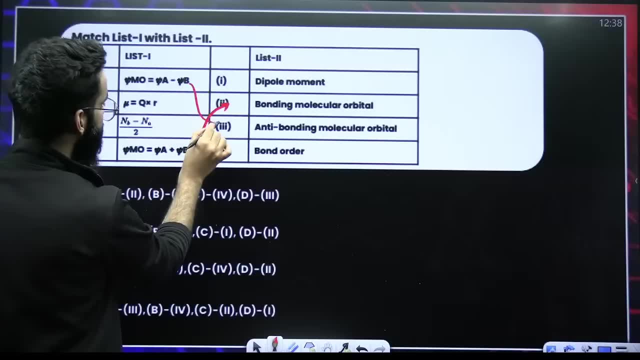 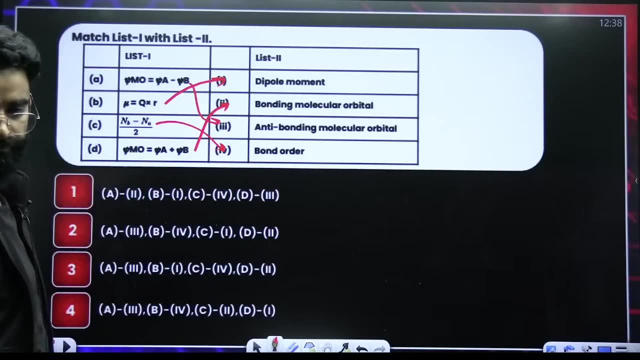 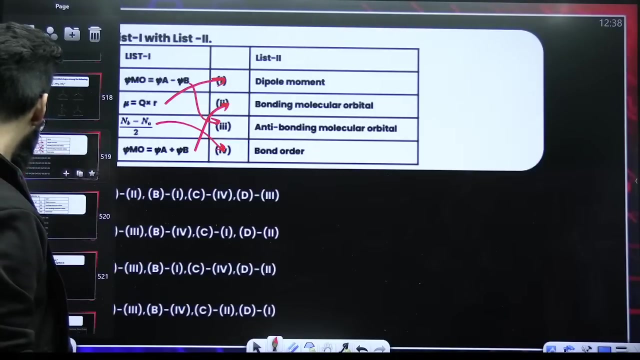 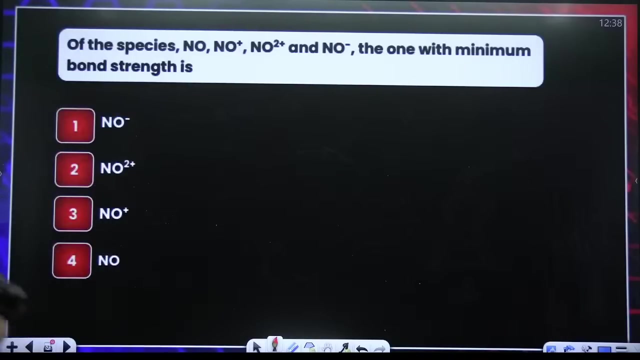 así rằng: constructive interference bonding: molecular orbital constructive interference bonding psi A minus psi B, destructive interference, anti-bonding: perfect Q multiplied by R. dipole moment bond order NB minus NA by 2. yeah, perfect. tell me the answer of this. one of the following species: no, no, positive, no 2 die, positive or negative the one? 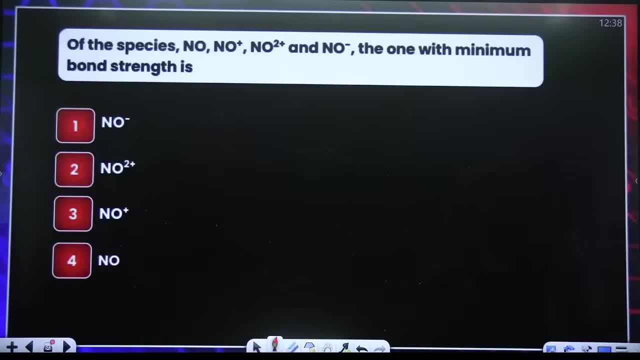 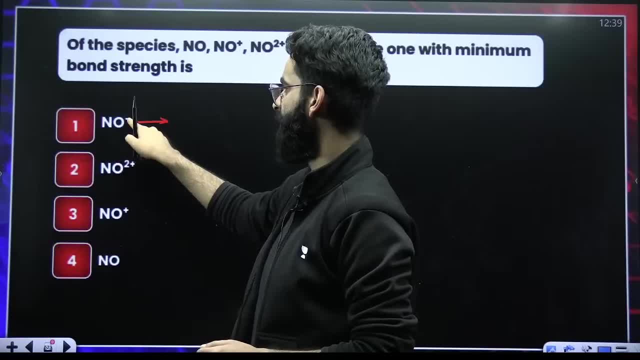 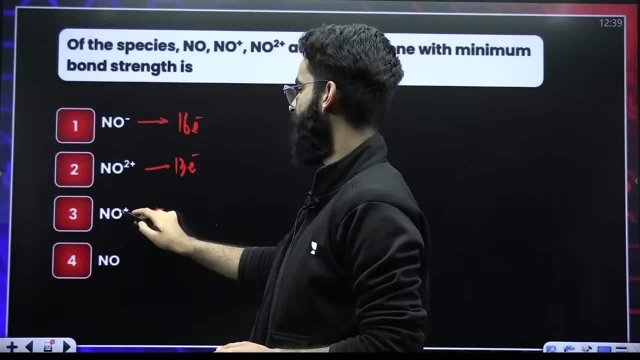 8 plus 7., 15.. 51,, 16.. 16 electrons spacing: 8 plus 7.. 15, 15 minus 2.. 13 electrons spacing: 8 plus 7. 15 minus 1.. 14 electrons spacing: 8 plus 7.. 15 electrons spacing Right. Bond order 2. Bond order 2.5.. Bond order 3. Bond order 2.5.. These two, Which of the following has got minimum bond strength? Minimum bond strength means minimum bond order. Minimum bond order is N O 2 negative, So it's N O negative here, Right. It is N O negative here, Perfect. It is N O negative here. Just a second, guys. Let me check the other new questions. 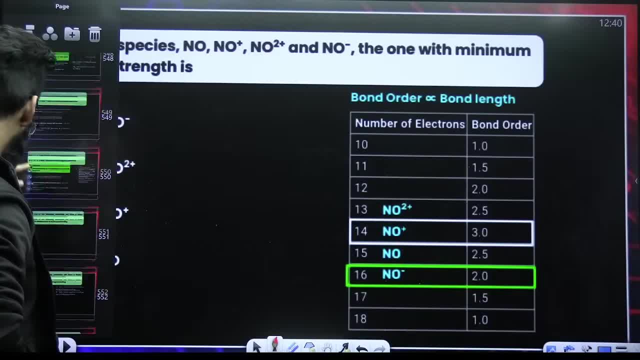 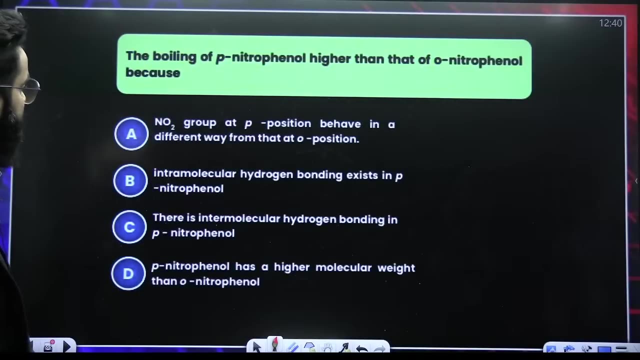 Because these are all repeated. These are all repeated ones. What is the answer of this one? The boiling of para-nitrophenol is higher than that of ortho-nitrophenol. Because, Because, Because of what? Because of what? 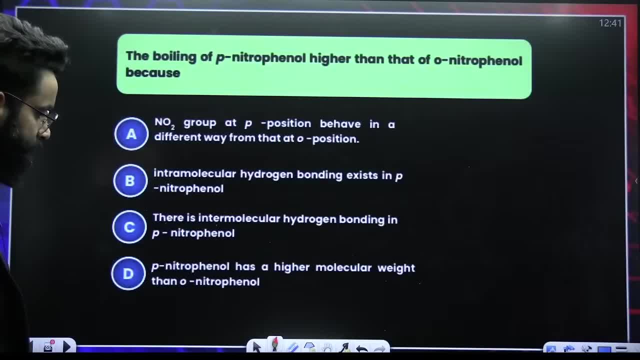 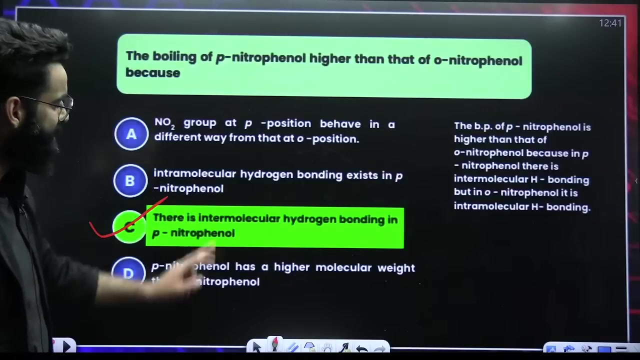 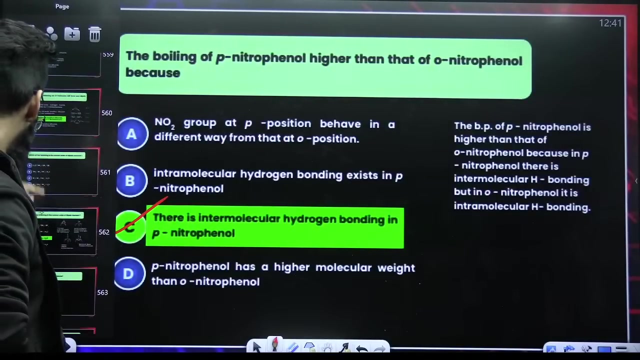 Because of what? Absolutely All of you are right. It's option C. There is intermolecular hydrogen bonding In para-nitrophenol In para-nitrophenol In para-nitrophenol. All these questions we are done with. 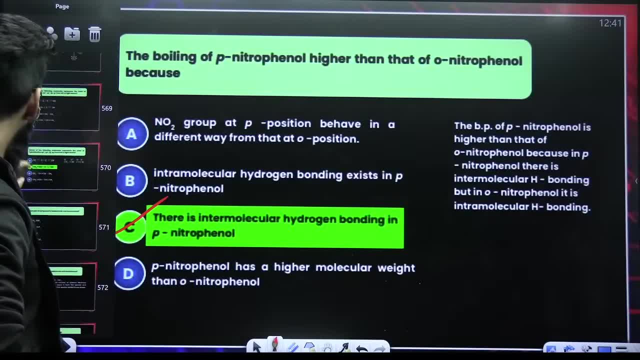 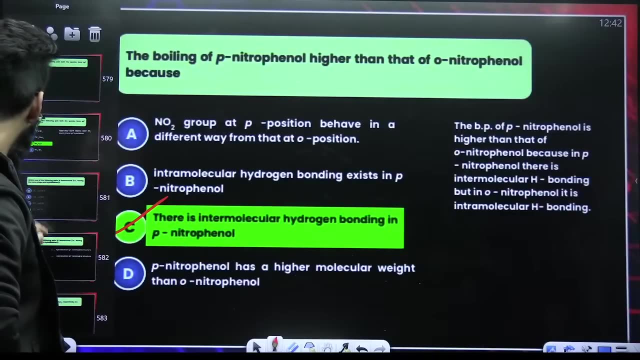 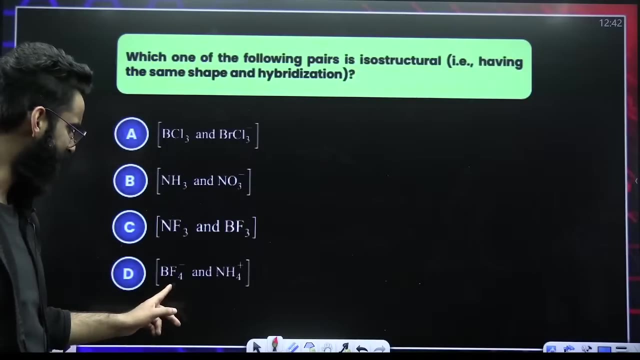 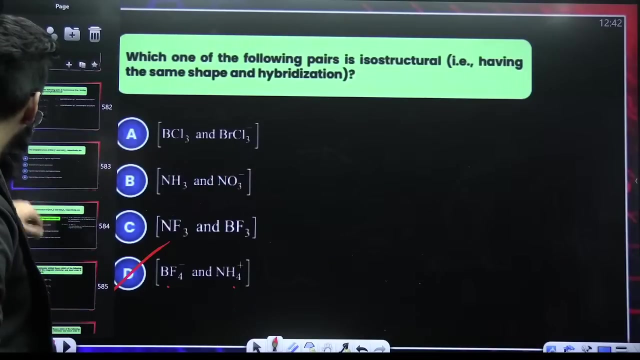 Now what is left? Just a second. This is done. What about this one? Which of the following is isostructural? I think you can easily solve it. Take the type: it's AB4L0. this, also AB4L0 type, is same right. so no need to check, no need to check over. 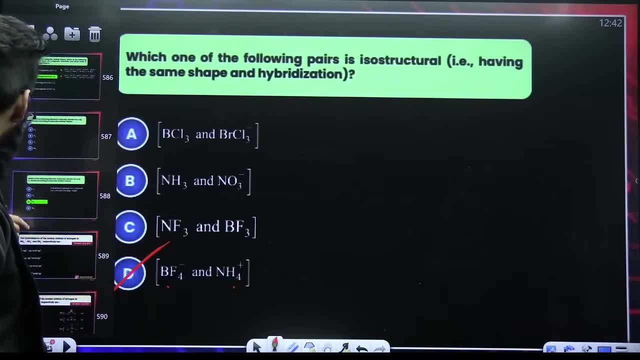 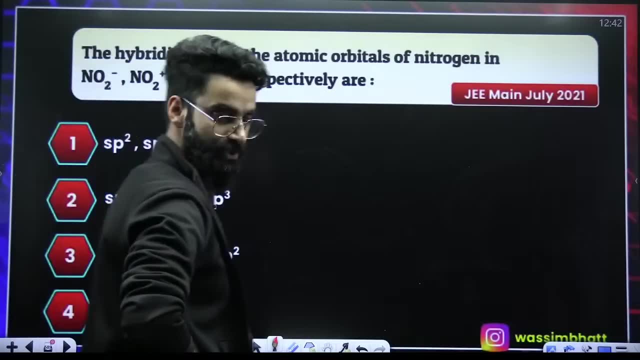 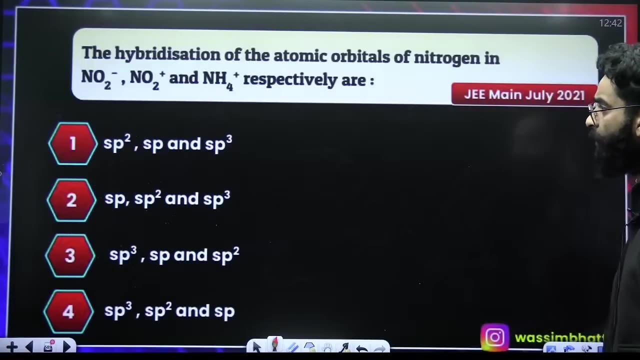 here. all these are same questions. let's solve some J equations which have been asked. okay, let's try to solve some J equations. let me see if you can solve them or not. this question has been asked in your J. mains 2021. hybridization of atomic orbitals- NO2 negative. NO2 positive. 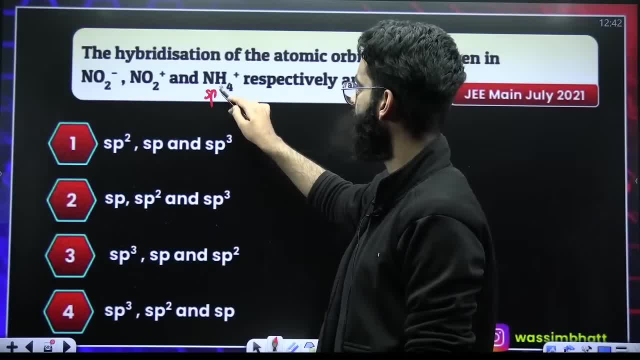 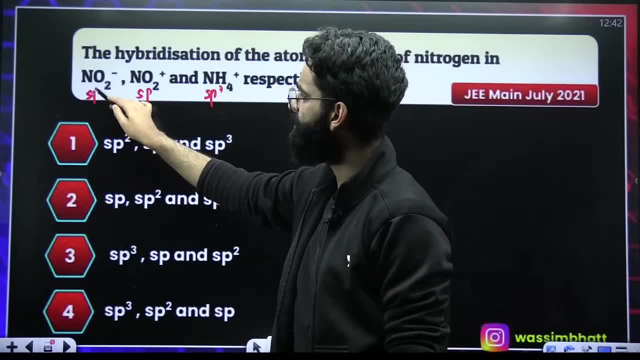 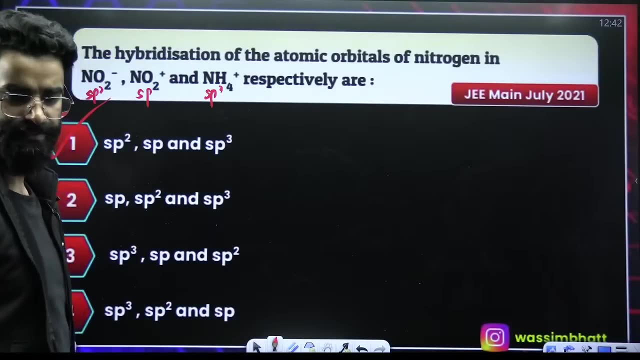 and NH4 positive. NH4 positive is directly SP3. right, this one is what this one is, SP. this one is in 5 plus 1, 6, so this is SP2 done. SP2, SP, SP3, option A: yes, now be active, guys. now be active in the chats, because now the questions are all your mains questions, okay. 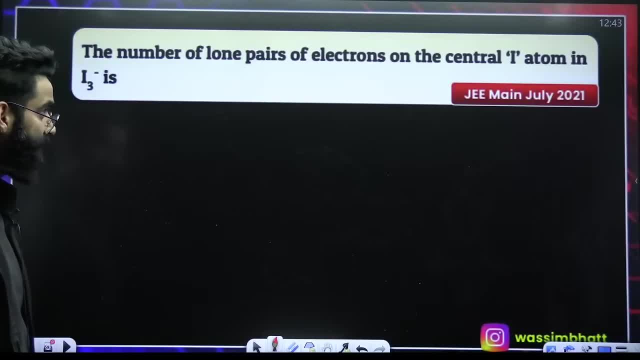 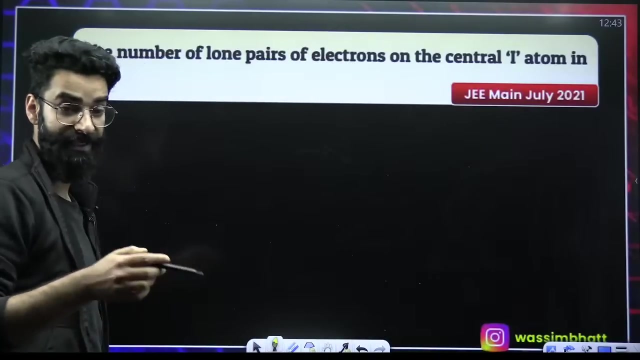 what is the answer of this question? the number of lone pair of electrons on the central iodine. here he is mentioning central iodine, so it has to be 3, right? he is asking about the central iodine, so answer has to be: what answer has to be 3. if it was total lone pairs on I3, then 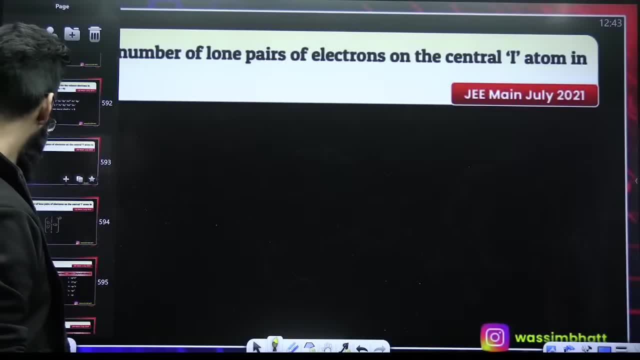 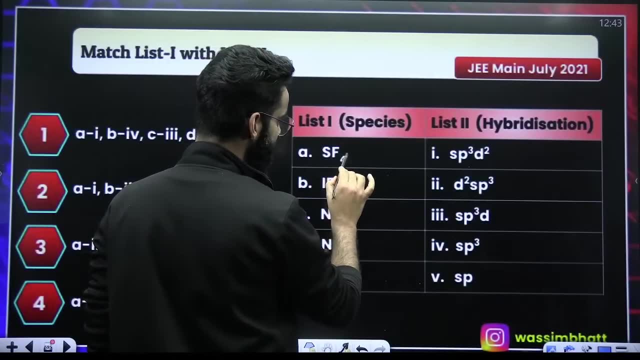 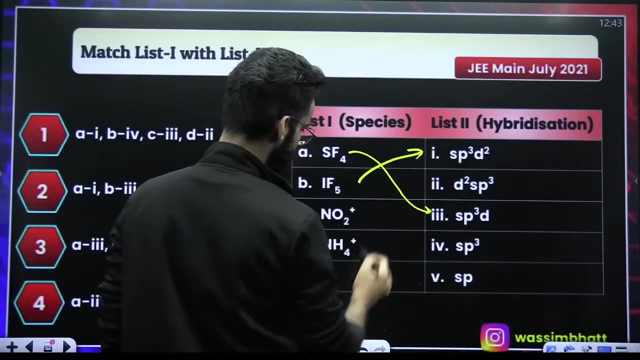 its answer was 9: SF4, SF4, AB4L1, SP3D, IF5- 5 sigma 1 lone pair. 5 plus 1. 6. SP3D2- NO2 negative- 2 sigma 0 lone pair. SP- NH4 positive- SP3. 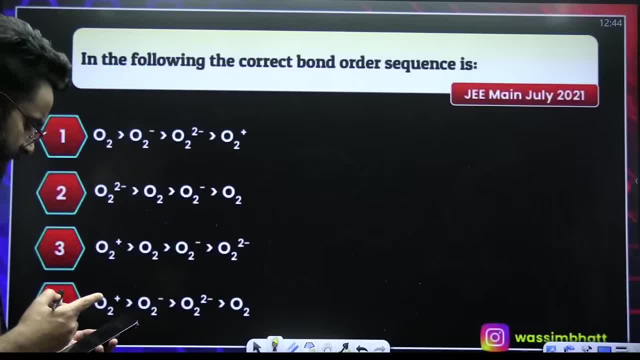 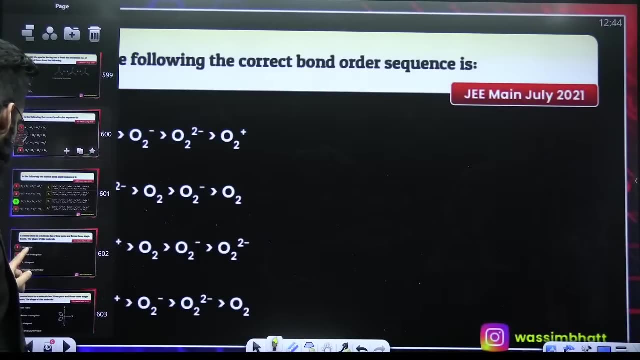 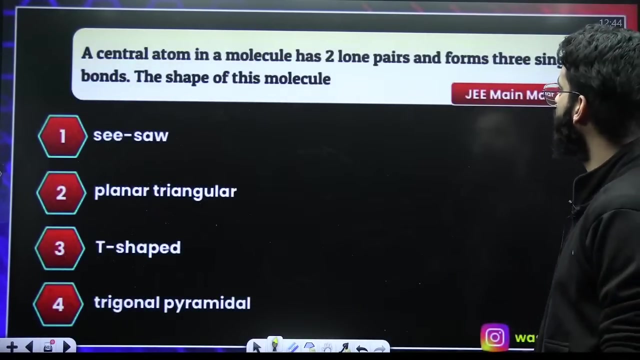 what about this one? this question we already solved, if you remember, few minutes back with this question. we already solved correct bond order sequence. correct bond order sequence. we already solved this question few minutes back. J2021. what do you think about this one? 2 lone pairs- 3 single bonds. 2 lone pairs- 3 single. 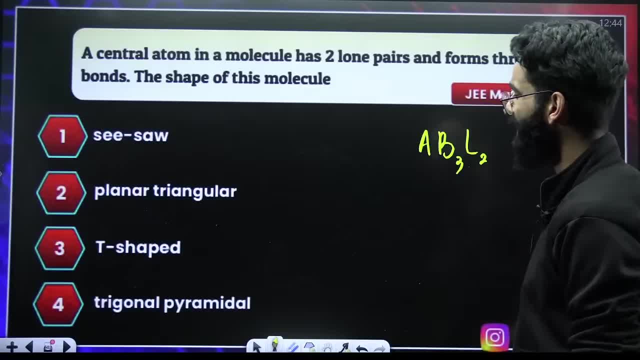 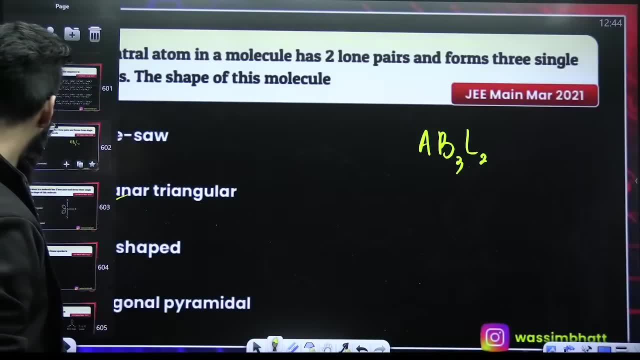 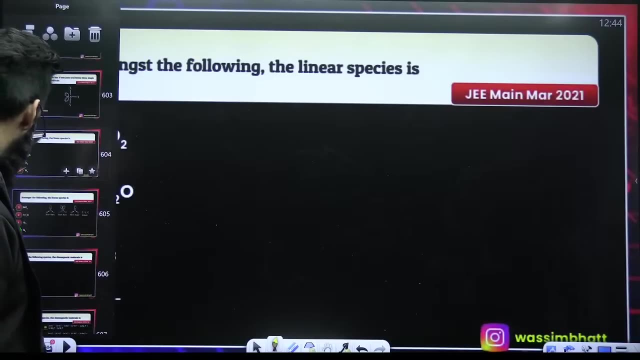 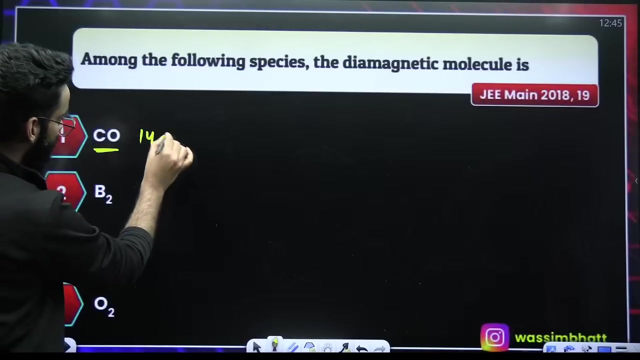 bonds: 2 lone pairs, 3 single bonds. AB3L2 T shaped. AB3L2 T shaped. among the following linear species: it is N3 negative, no need to check etc. which is the following: is diatomic molecule. carbon monoxide is a 14 electron species, all the 14 electron. 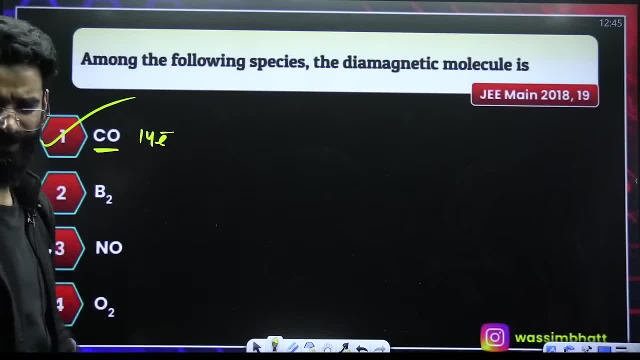 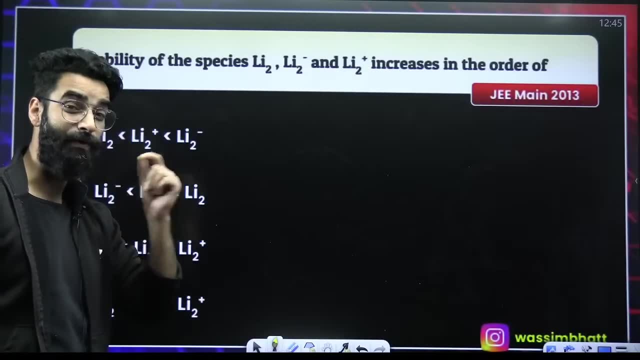 species. they have no unpaired electrons, so they are diatomic. when you write their molecule orbital configuration, right stability order: stability order. what do you need to do? write the molecule of orbit configuration. check the bond order 1, which is more bond order, more stable, if there are. 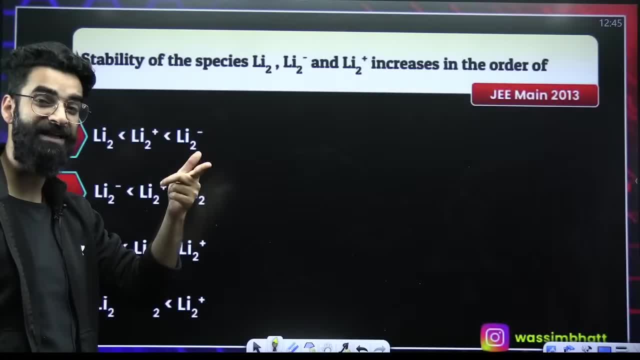 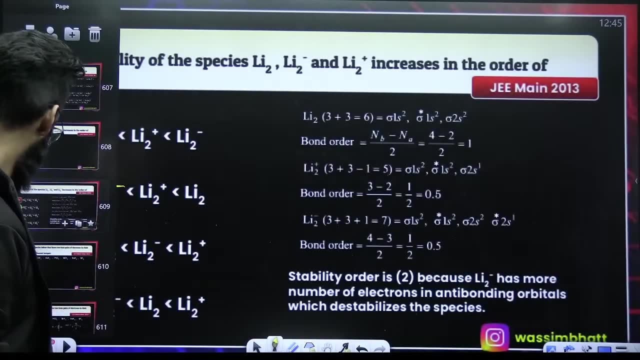 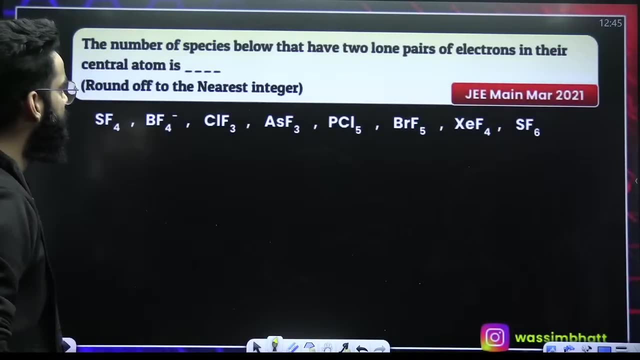 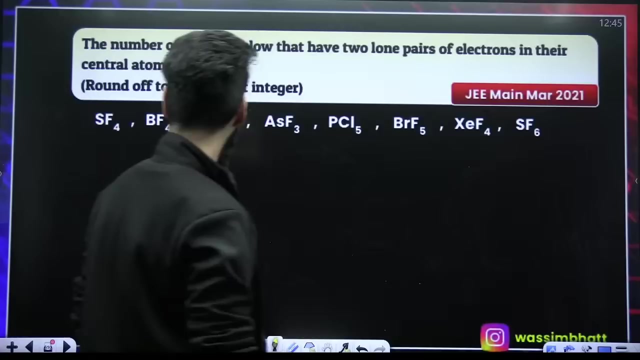 2 species having same bond order. then check their anti-bonding electrons more than anti-bonding electrons. lesser the stability right. option 2: number of species: The number of species below that have two lone pairs of electrons that have two lone pairs of electrons in their central atom, two lone pairs of electrons in their central. 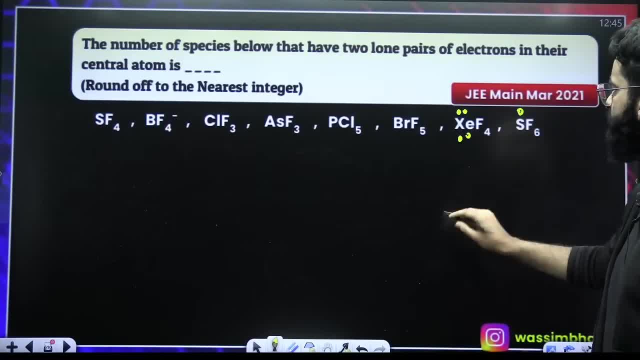 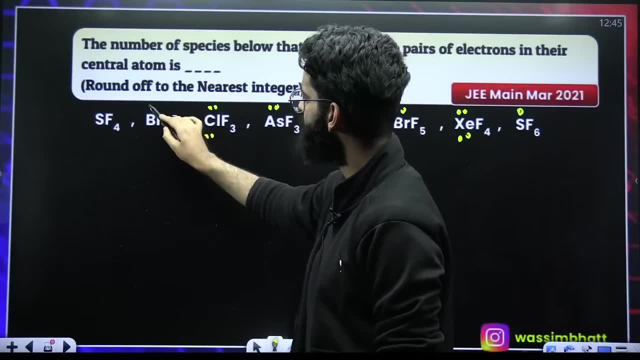 atom SF6, no lone pair here. two lone pairs, one lone pair, zero lone pair. one lone pair, two lone pairs: zero lone pair, one lone pair. The number of species having two lone pairs here you have got two lone pairs here you. 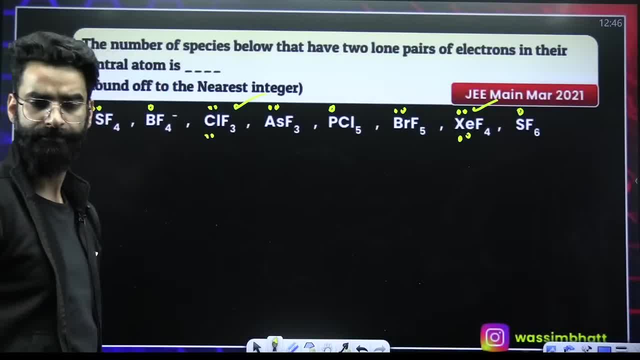 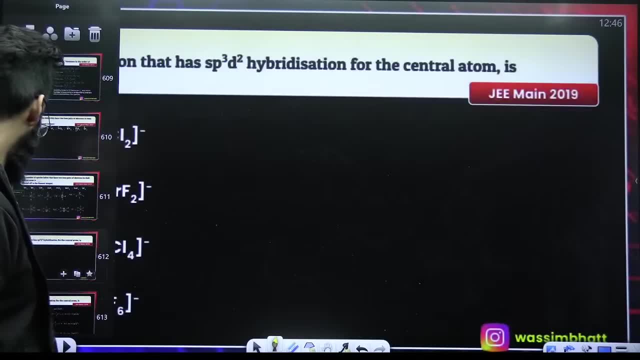 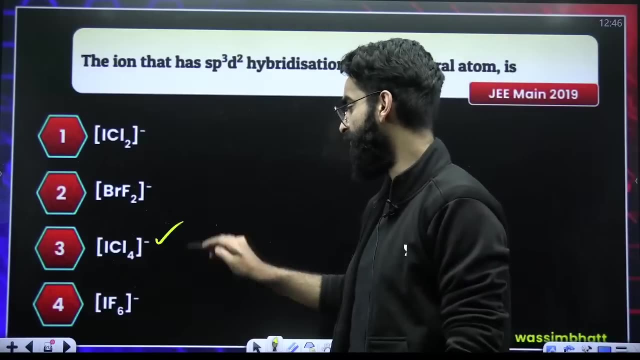 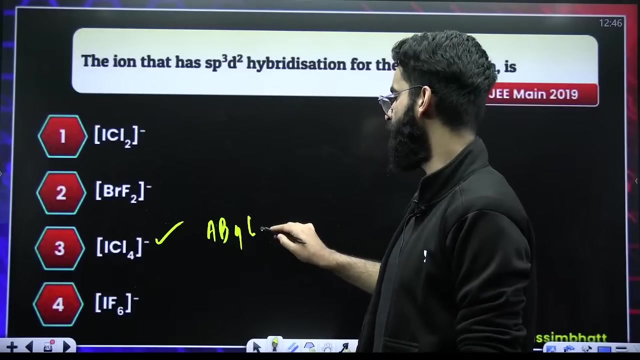 have got two lone pairs. Answer is two. only answer is two. only right answer is two. only The ion that is sp3d2 hybridization. the ion that is sp3d2 hybridization. if you look at ICL4 negative, ICL4 negative- it is of the type AB4, AB4L2, static number is 6, sp3d2,. 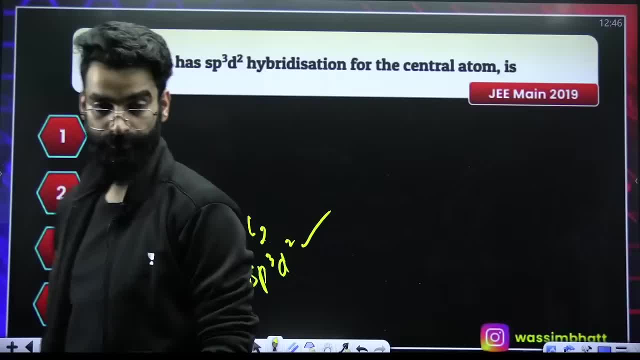 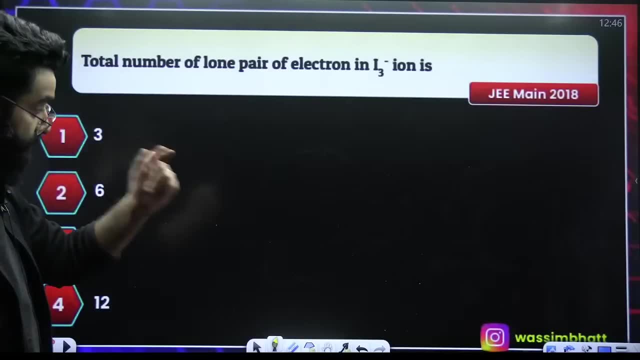 right, sp3d2.. That is what we have to check, correct. Rest you can do on your own. you can check them out Now. this is the question. J means 2018, total number of lone pairs in I3, total number of. 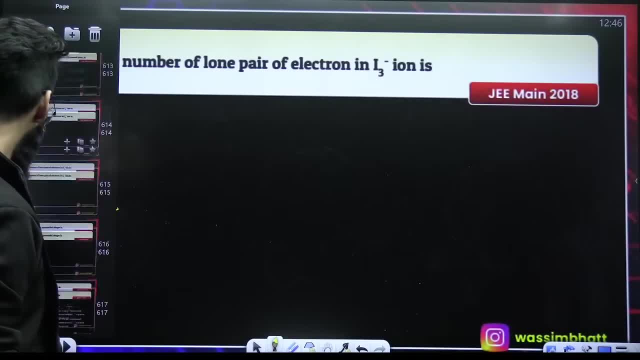 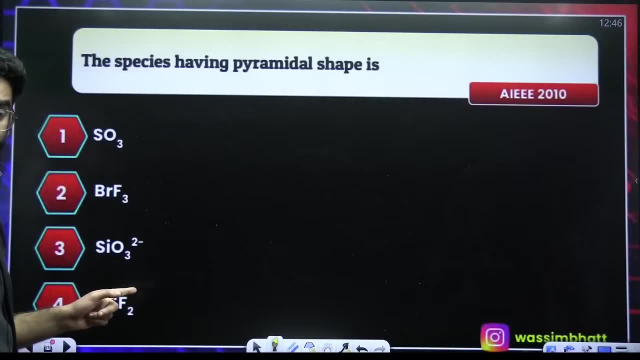 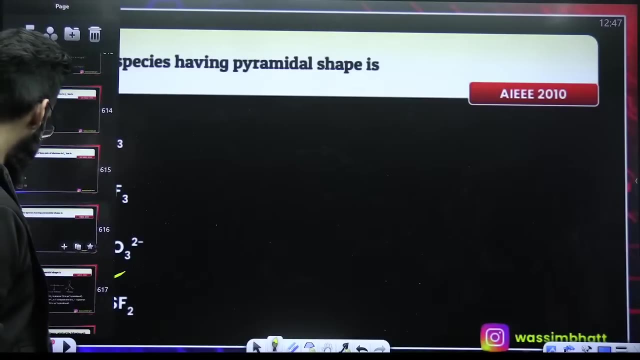 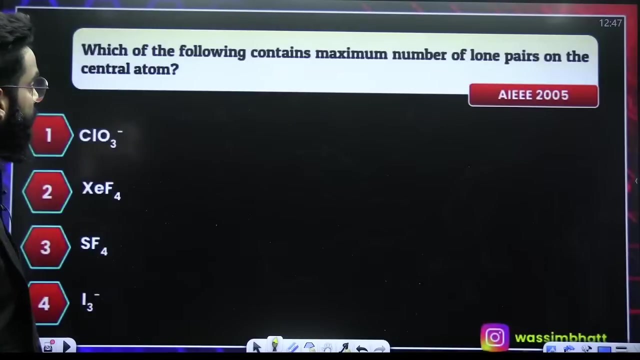 lone pair means 9,. okay, This is also the question which we solved long back. This is also J means AEEE question, the species having pyramidal shape. it is OSF2, OSF2.. Which of the following contains maximum lone pair on the central atom? 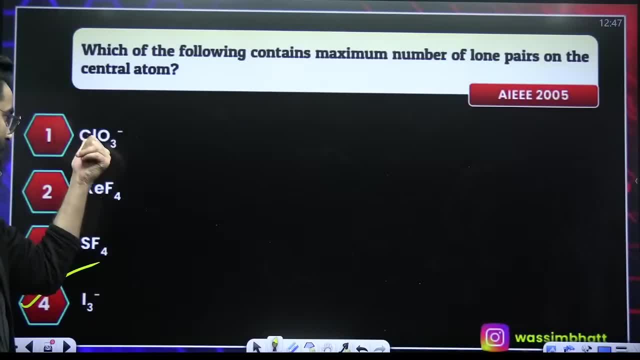 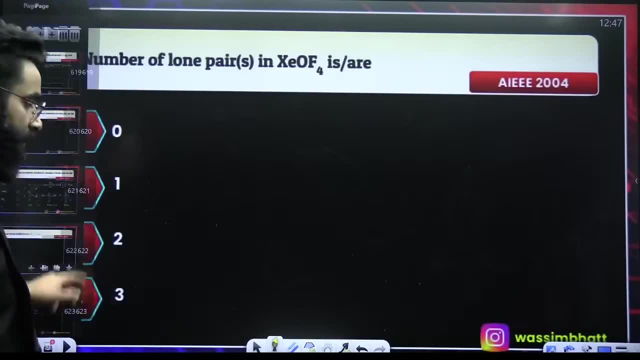 On the central atom: 3 lone pairs, 1 lone pair, 2 lone pairs, 1 lone pair. so maximum here Number of lone pairs in XCOOF4, number of lone pair on the central atom. on xenon that 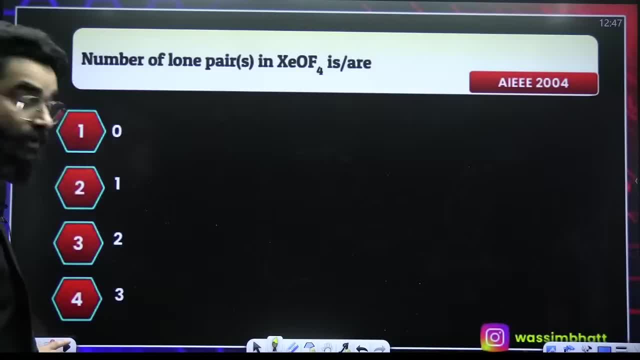 will be 1,. right, If you remember that bond angle equation which I showed you, How many pairs, How many 90 degrees are there in XCOOF4, there was 0, 90 degree, right? do you remember there? 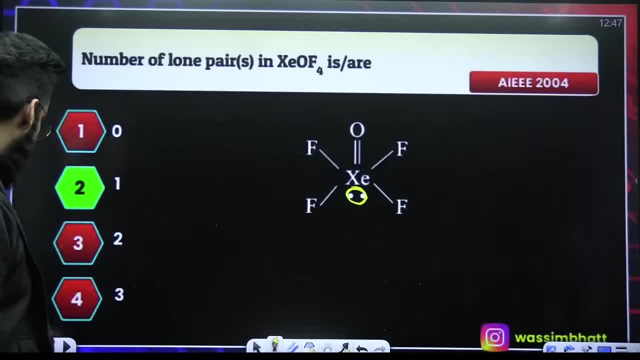 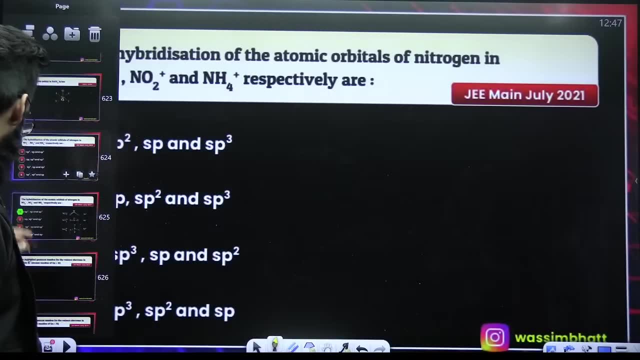 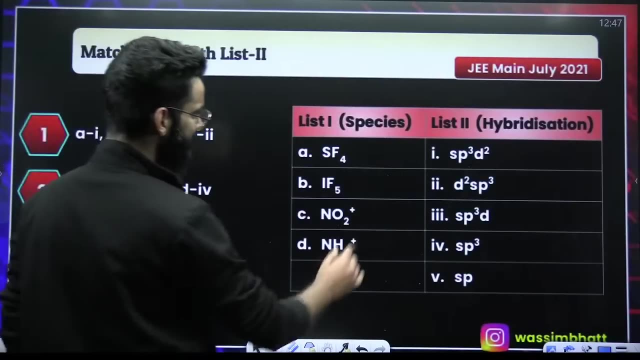 was 1 lone pair. there was 1 lone pair. This question we have already solved. this question is already solved. okay, This question you can solve easily. SF4 means sp3d, IF5 means 5 plus 1, 6 sp3d2, NO2 positive. 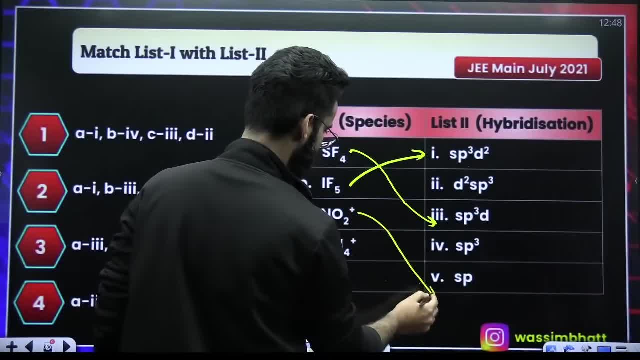 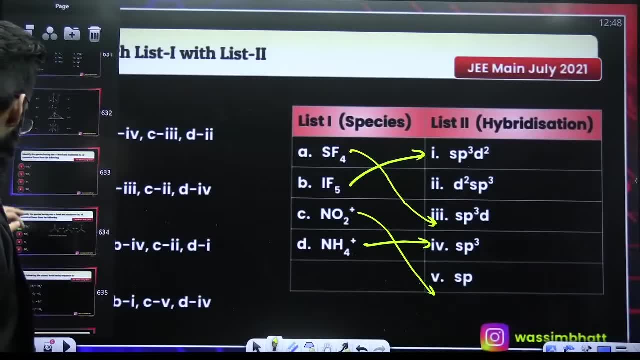 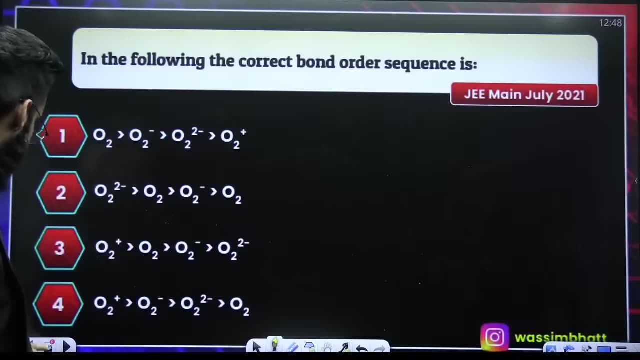 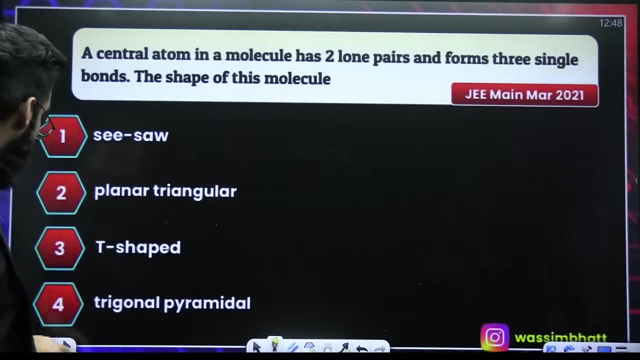 means what It means. sp NH4 positive is sp3, even this is already solved. it is a solved question. Even this bond order question is already solved. even this is already done. This is already done. 2 lone pairs, 3 single bonds. T shaped molecule linear species N3. 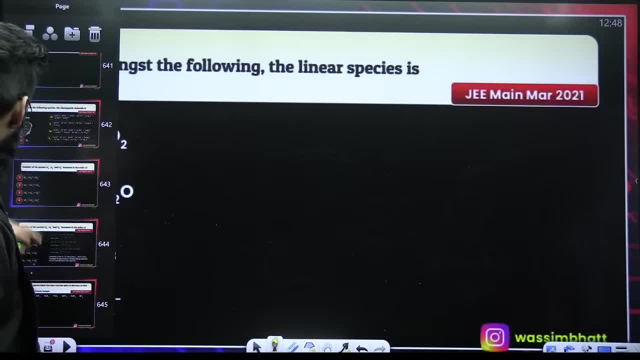 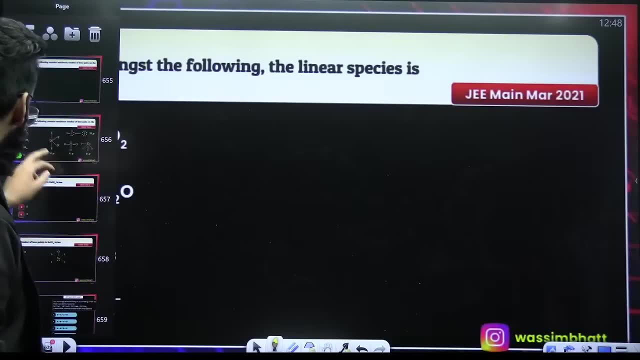 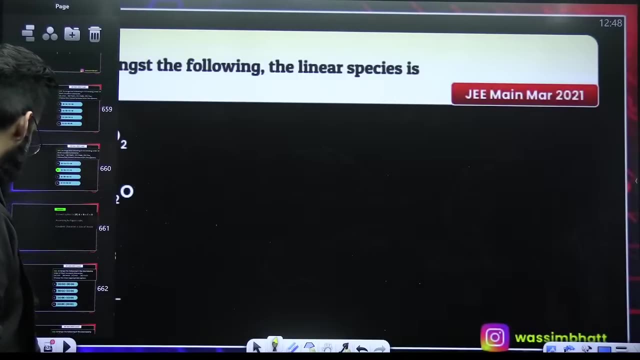 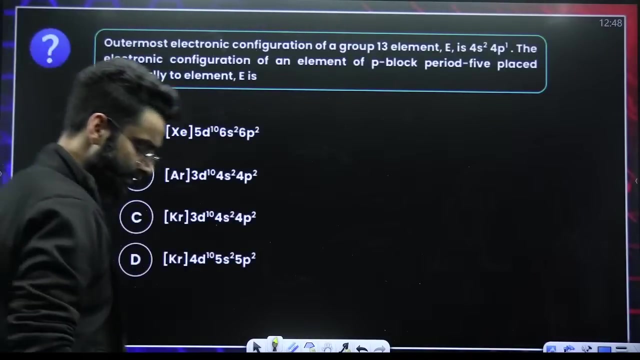 negative. this is already solved again. Just a second, I think that's it, guys. Now let us start few questions of periodic classification. Periodic classification has not much of variety, by the way. Periodic classification- there is no variety. 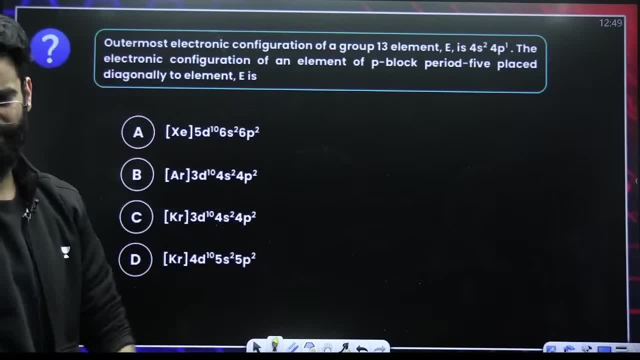 There are only few types of questions Which you should know about period of classification. There's a few questions. The actual variety was in chemical bonding and I believe you can easily solve chemical bonding equations from now on. What is the answer of this one? 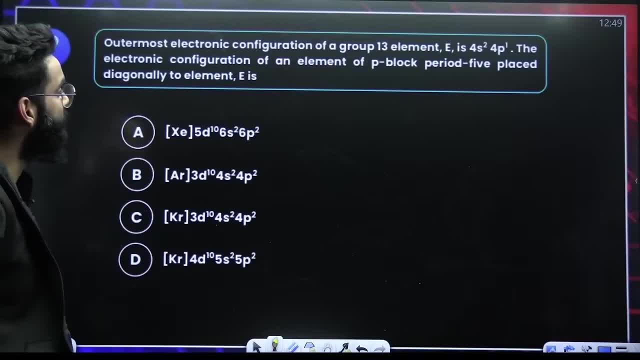 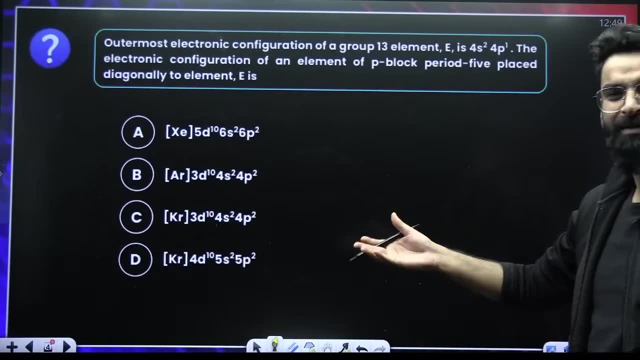 I'm sorry Outermost. electronic configuration of group 13.. Group 13.. Group 13. It will not take more than 20 minutes. After 20 minutes, we'll end the session, You don't need to worry. Okay, Let's complete it. Why to take the break? Group 13. The electronic configuration. 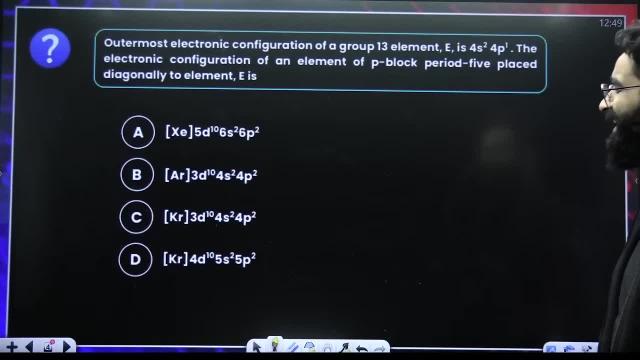 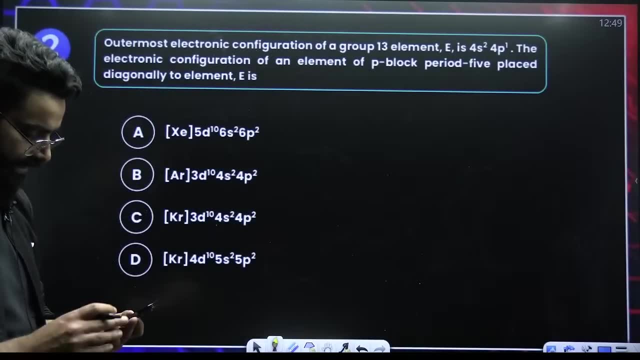 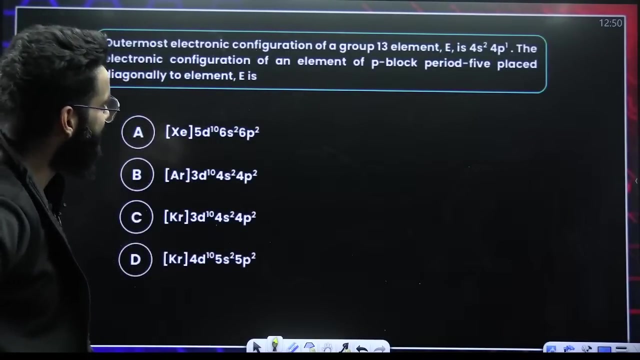 of the element of the p block Period 5, placed diagonally to the element e, is: What do you think about this one? What do you think about this one, guys? Quick, Quick, Outermost. electronic configuration of group 13 element. Group 13 means. 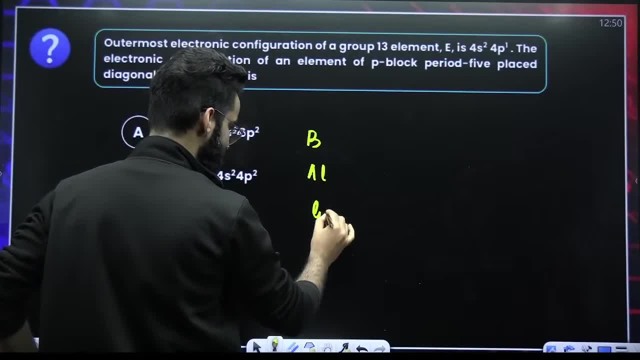 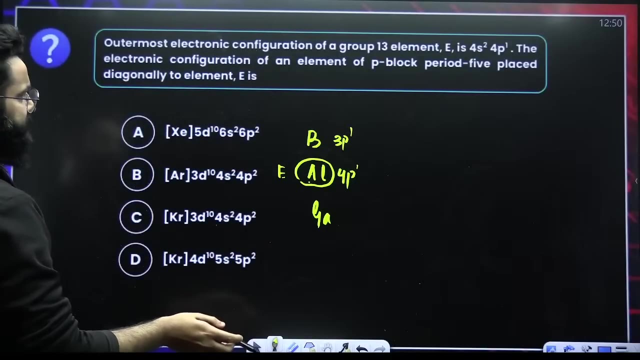 boron, aluminium, gallium. Boron's outermost configuration is 3p1.. Aluminium is 4p1.. So he is talking about the element aluminium. So e is your aluminium. first of all, The electronic configuration of the element of the p block placed in period 5.. This is period 4, placed in period 5.. 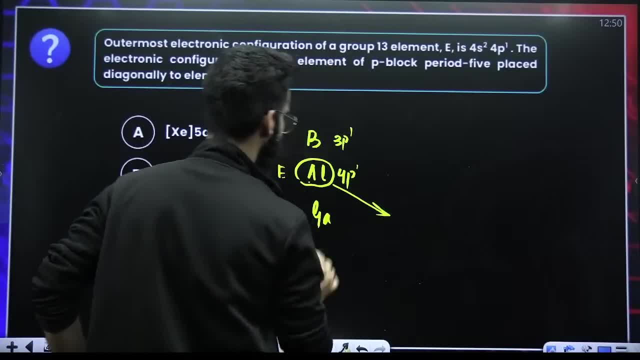 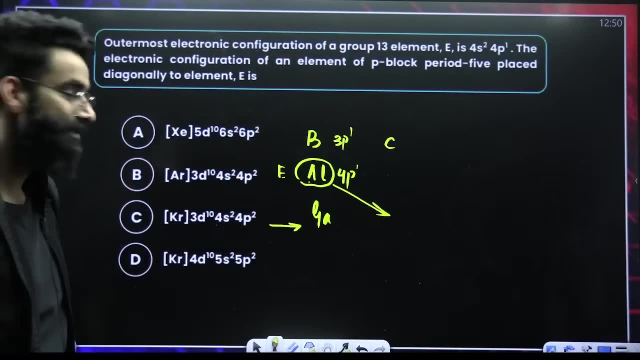 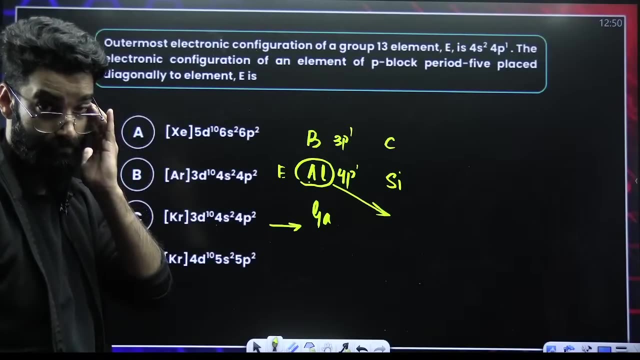 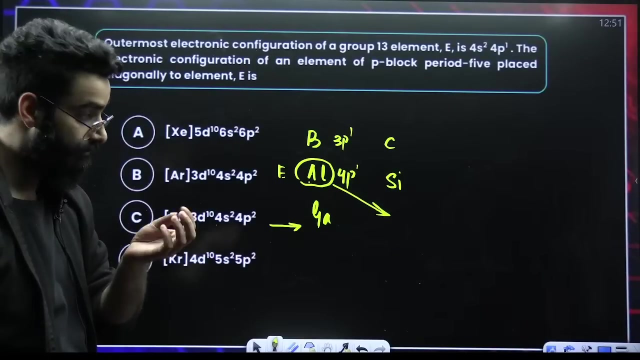 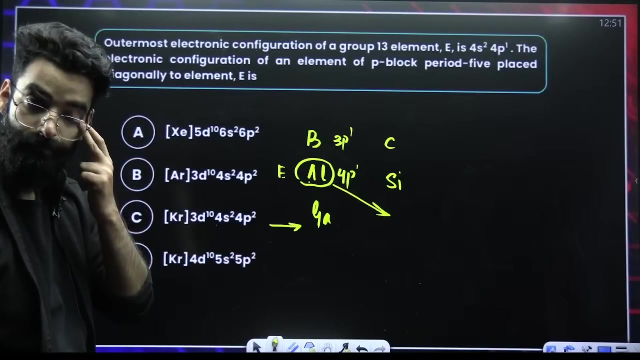 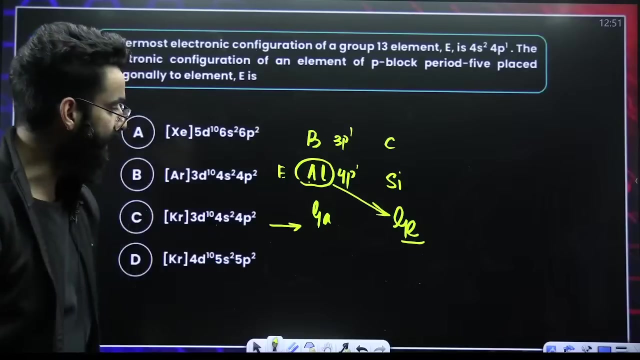 Diagonally to the element Over here. Over here, Boron Carbon, Right? Perfect, Now, guys, after this, Silicon, Now tell me the answer. What are you waiting for? What are you waiting for? This was 4p1.. This will be 5p1.. Right, This will be 5p2.. This will be 4p2.. 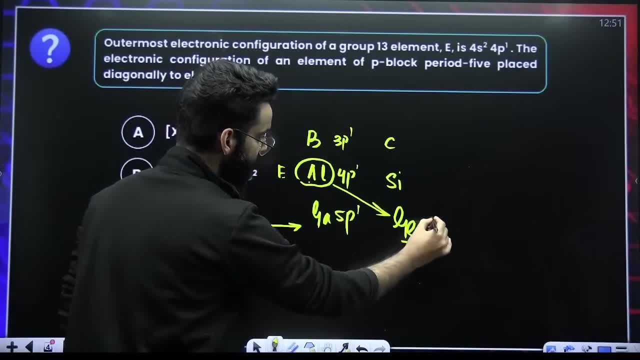 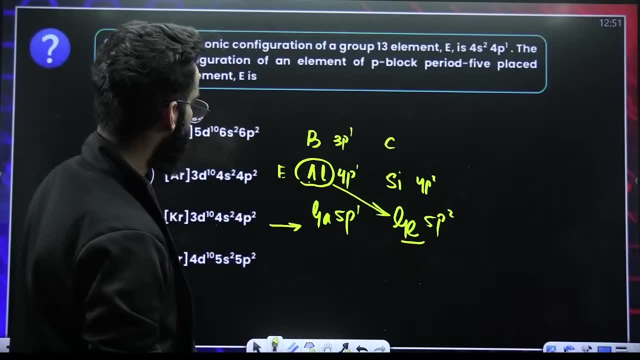 Not 5p1,. Boron iswith a mistake. How are we underground…. Boron's configuration is 6p1.. Good, This was 4p1.. I'm going to wait something. Boron, Liam 樹. This was 4p1.. This will be 5p1.. Right, This will be 5p2.. Sigh, What are you for? We took time, forBERMAN Bowden. What are us until now? Just wait 10 seconds. 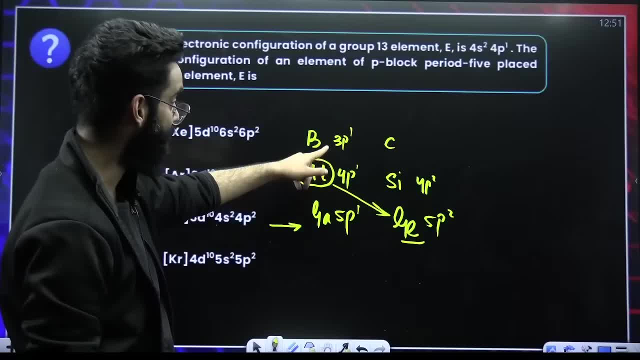 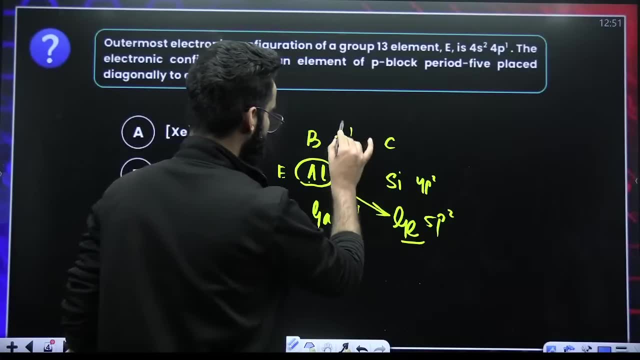 What are you waiting for? What are you doing? What are you waiting for? What are you waiting for? This was 4p 1.. This will be 5p1.. 2p1, right, I wrote 3p1.. This is 2p1.. This is 3p1.. This is 4p1.. This is 4p1.. Just a second. 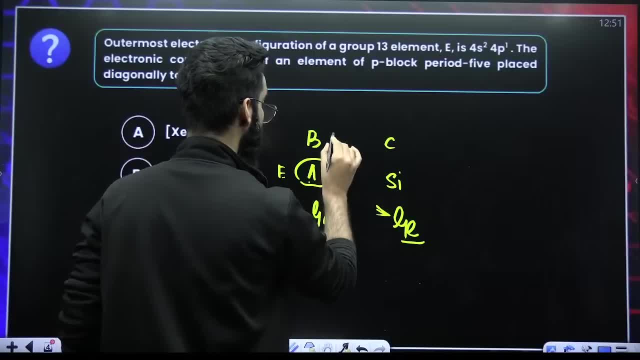 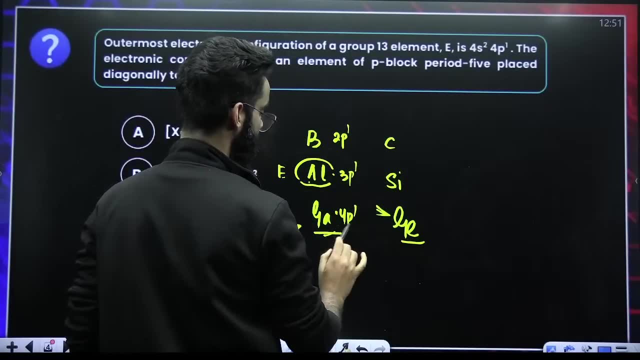 Just a second. Just a second. This is 2p1.. This is 3p1.. This is 4p1.. He was talking about which element? 4p1.. Perfect, He was talking about 4p1.. He was talking about this gallium. 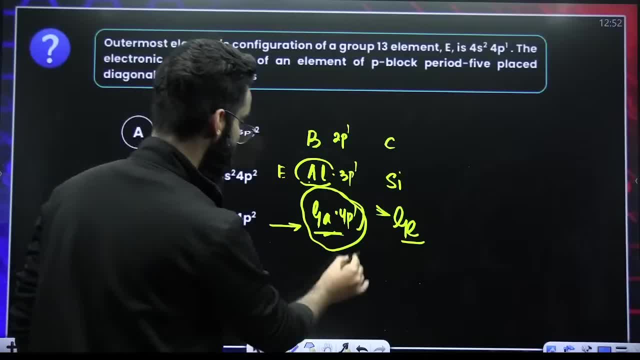 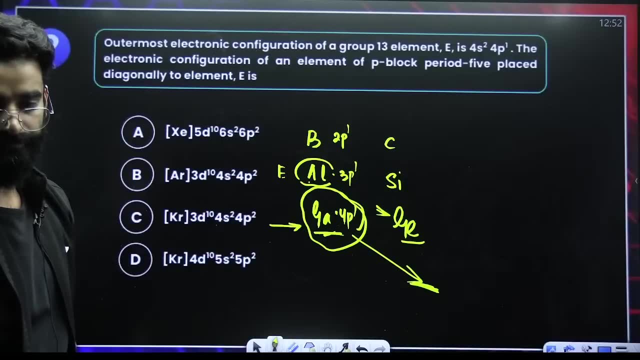 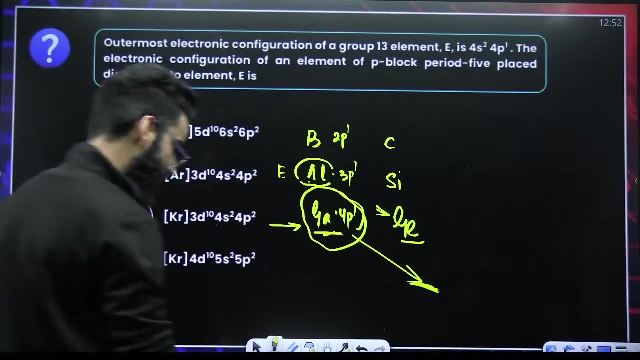 not aluminium. He was talking about gallium, not aluminium. Now we have to see which one is diagonally related. Which element comes here? Which element is here? Which element is here? Is it tin? If you do not remember the elements, also see, you can do it like this. If this was, 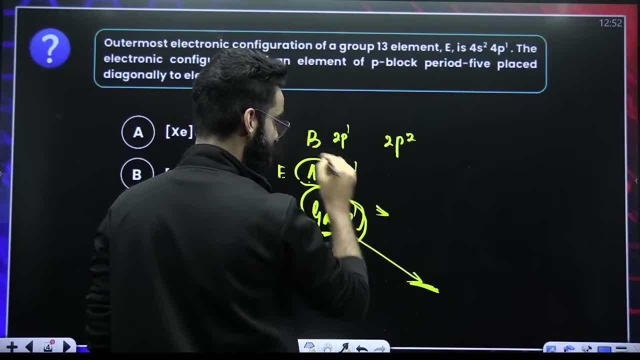 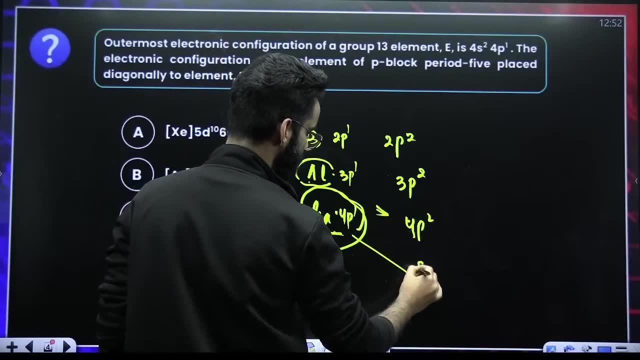 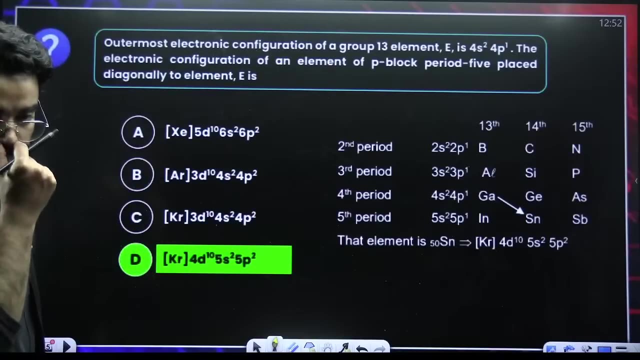 2p1,, then this is 2p2.. That means carbon. This was 3p1.. This will be 3p2, right, 4p1.. 4p2.. 5p2.. So where is 5p2?? Right, Got it Perfect, Alright. 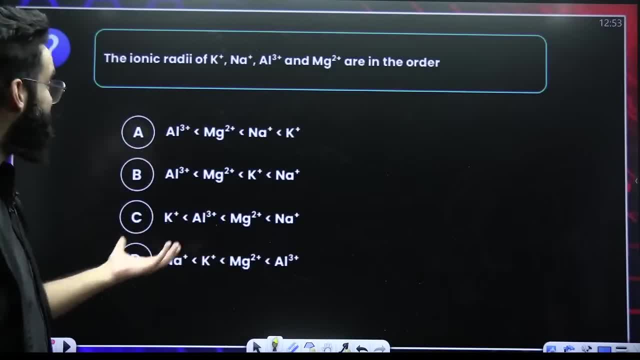 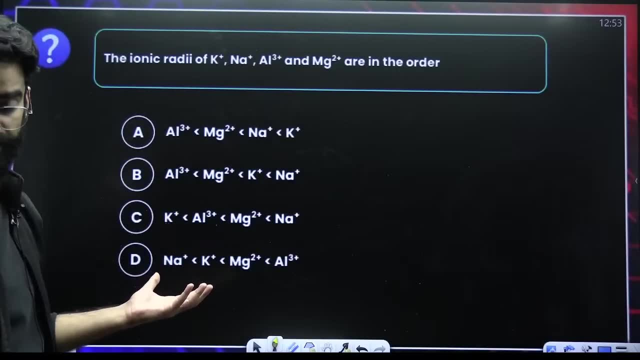 This sort of question you can easily solve, I believe Easily means easily. Ionic radio of K positive, Na positive, L tri positive, Mg, di positive- All are isoelectronic species. More effective nuclear charge. More effective nuclear charge means lesser the size, More. 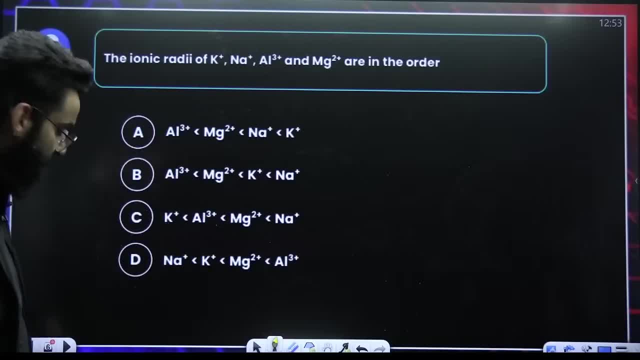 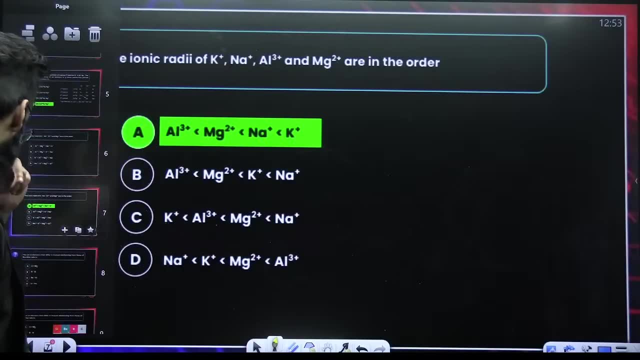 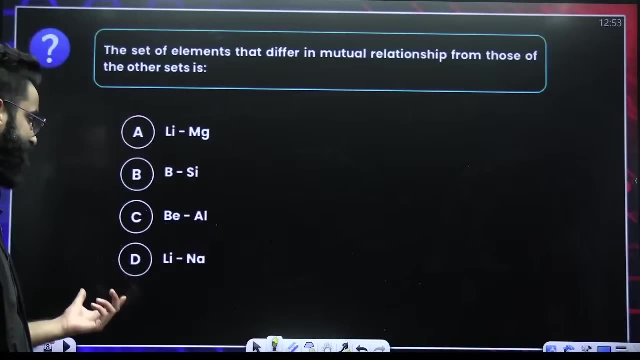 effective nuclear charge means lesser the size, Right? This sort of equation we have already solved, Yeah, Perfect. Let me see some different type of questions. What is it, The set of elements that differ in mutuality, Mutual relationship, from those of other sets? What do you think? Lithium and magnesium? 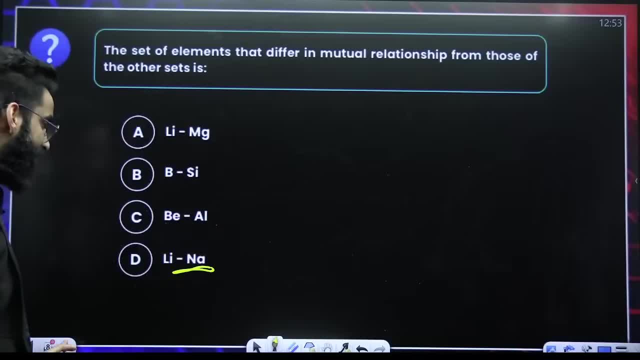 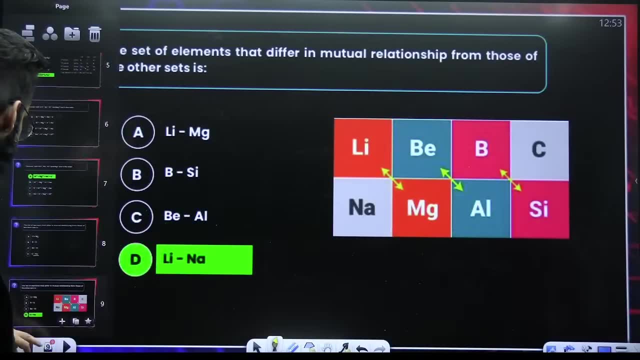 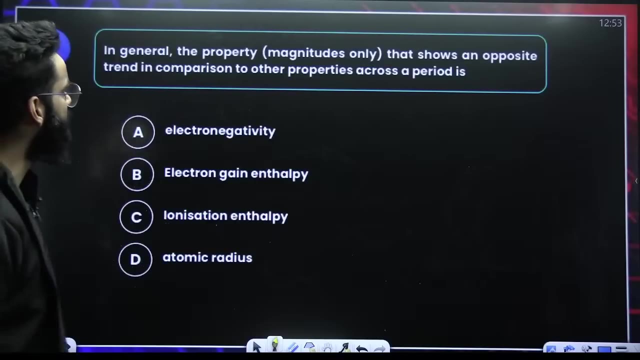 they are diagonally related. They are two. They are two. This one, Lithium sodium, they are not diagonally. See, these two are diagonally related. Diagonally related. Diagonally related, Correct, But these two were not diagonally related. In general, the property that shows: 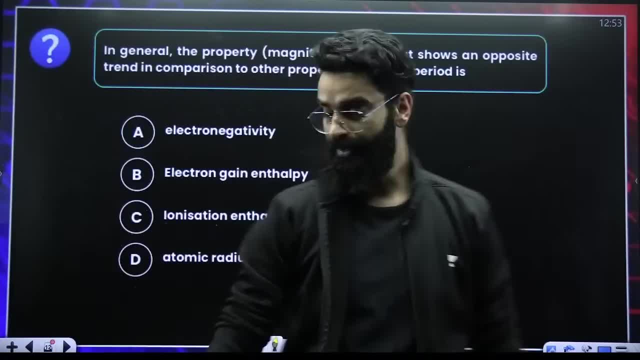 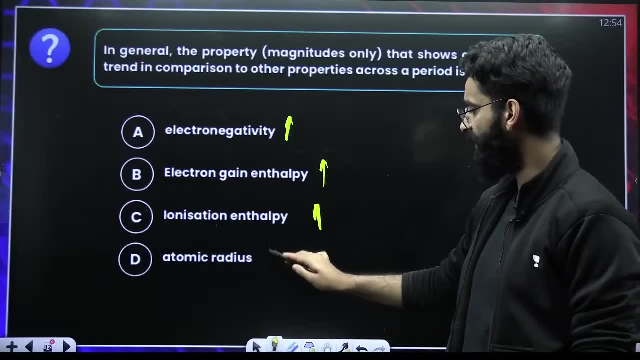 an opposite trend in comparison to other properties across the period. Across the period, electronegativity increase. Across the period, electrongainenthalpy increase Increase. Ionic energy increase. Right Atomic radius across the period decreases. So this is showing reverse of what others. 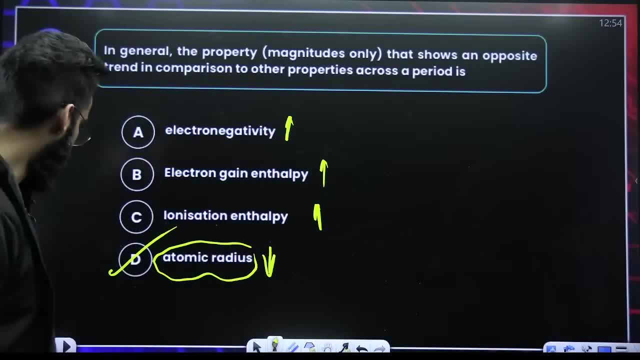 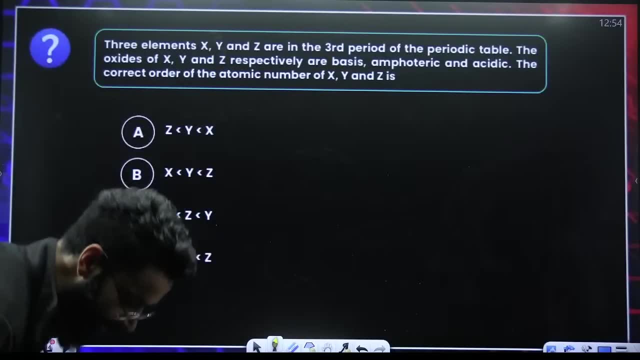 show. So option D: Odd one out, Odd one out, Odd one out. Look at this one, Look at this one. The elements x, y and z in third period of the period table: The oxides of x, y and. 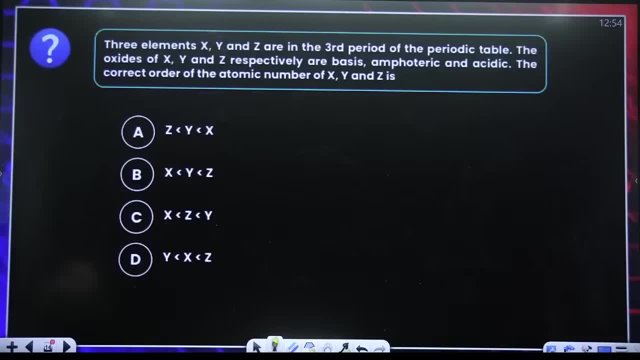 z respectively, are bases, amphoteric and chloroplasts. Why? Because if these two are single, then at least for the next set of elements they will be same number of elements: Right, The, and basic, amphoteric and acidic, Which forms basic oxide. 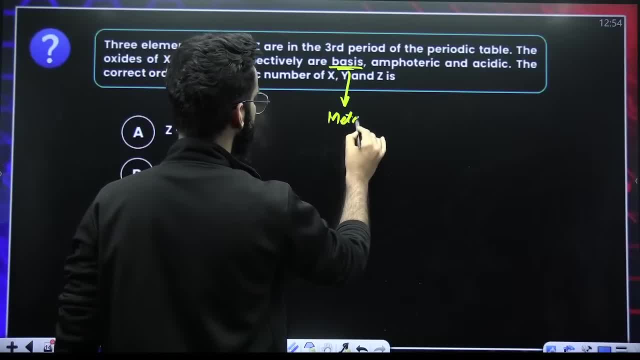 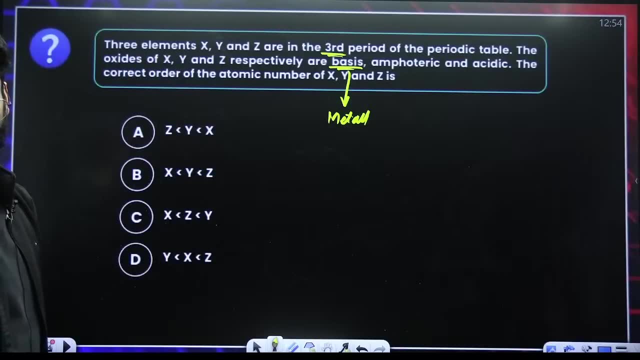 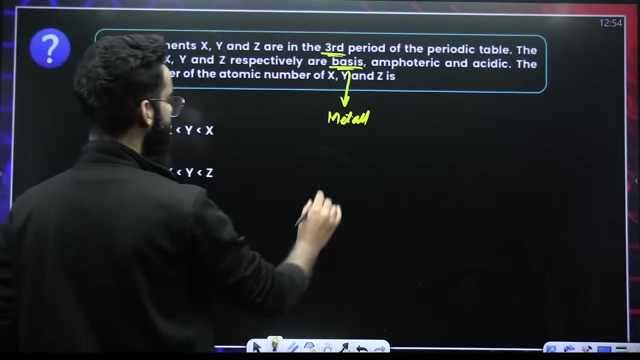 Metals form basic oxide. right, Your metals perfect, right? He is talking about group 3.. He is talking about group 3. Hydrogen is group 1. Lithium is group 2. Group 3: is your sodium perfect? 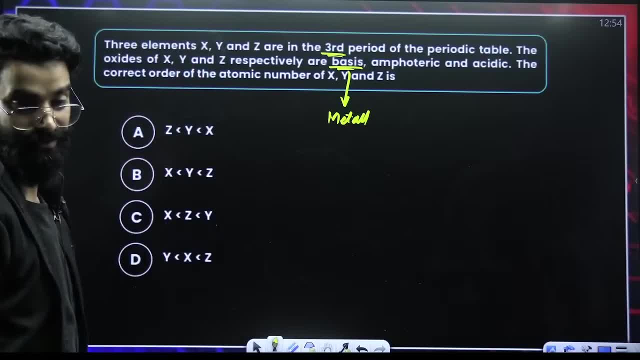 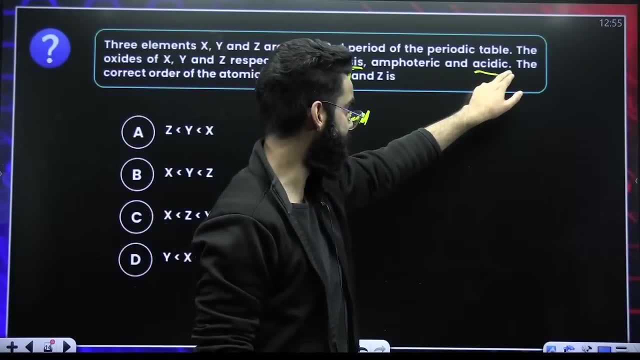 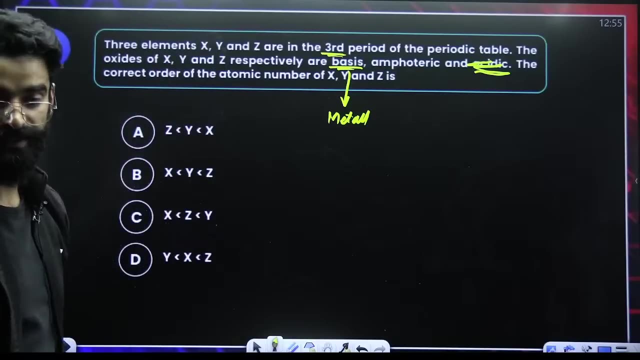 Group 3 is your sodium perfect right. Basically, metals forms basic oxides, Non-metals. non-metals form acidic oxides. Non-metals form acidic oxides And metalloids. what do they form? Metalloids form amphoteric oxides. 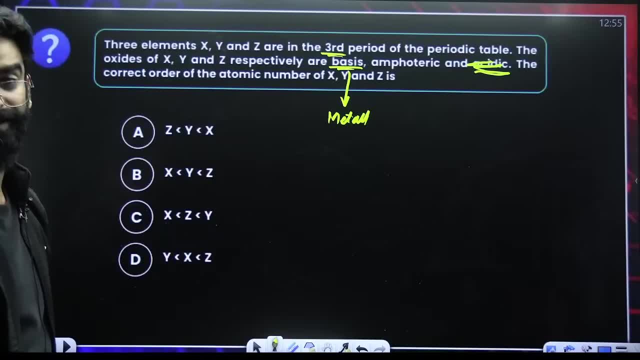 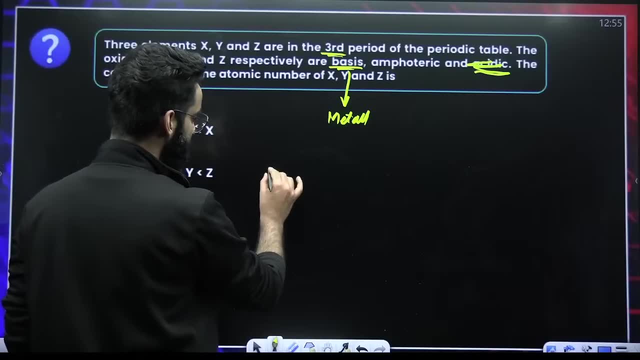 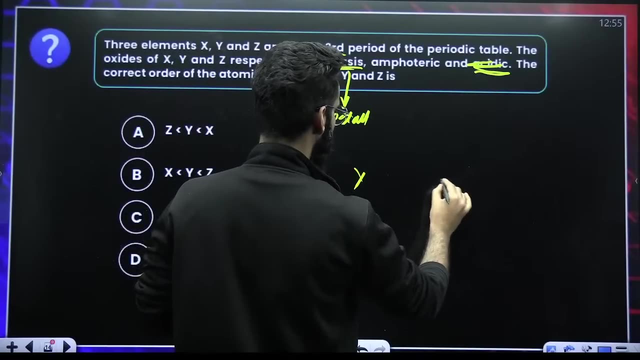 Now I think you can easily solve. You got the hint. You got the hint right, You got the hint. And X is forming basic oxide, So it has to be. on the extreme left, Y is forming amphoteric oxide. in the middle right, Acetic is formed by Z non-metal. 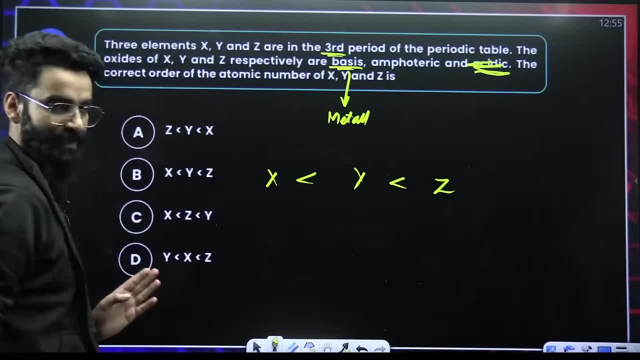 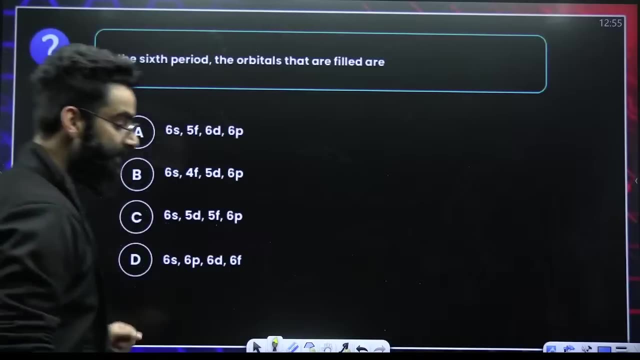 So atomic numbers, atomic numbers, Atomic numbers will be like this: because they belong to same period, It is shown they are third period elements. right, They are third period elements. I hope this is clear. I hope this is clear. In the sixth period, the orbitals are filled. In the sixth period, the orbitals that are filled. 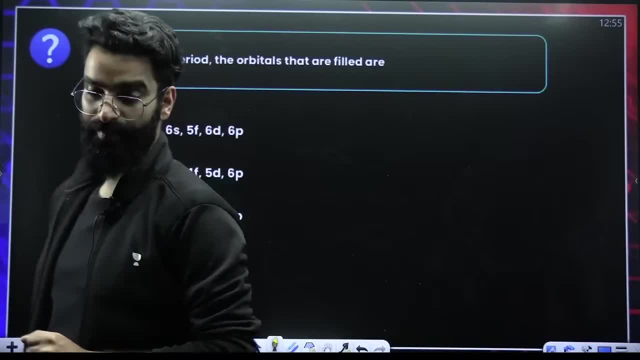 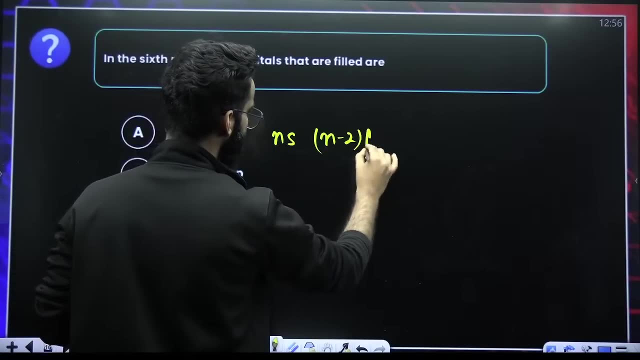 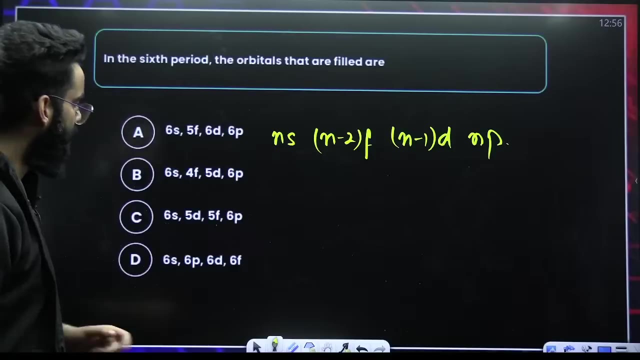 Sixth period: orbitals that are filled, Orbitals that are filled. Orbitals are filled in this manner: NS, N-2F, N-1D right And NP Over. here the maximum principal quantum number is 6.. 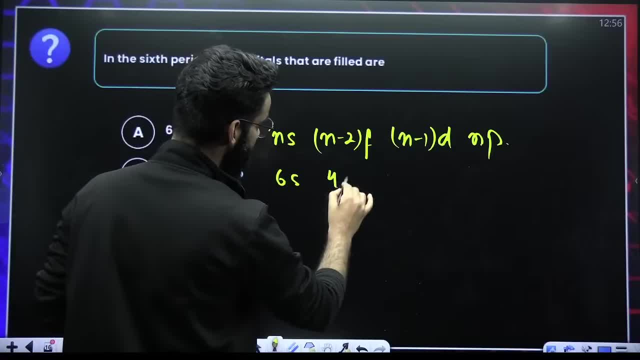 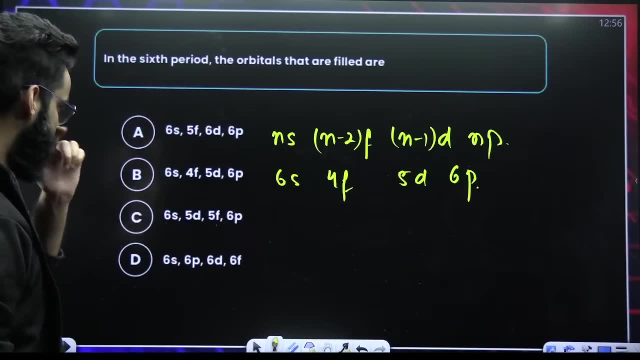 N is 6.. If N is 6,, so this is 6S. 6-2 is 4S. 4F. 6-1 is 5D. This is 6P. Do you see any order like this? Do you see any order like this? Option B: Remember it. 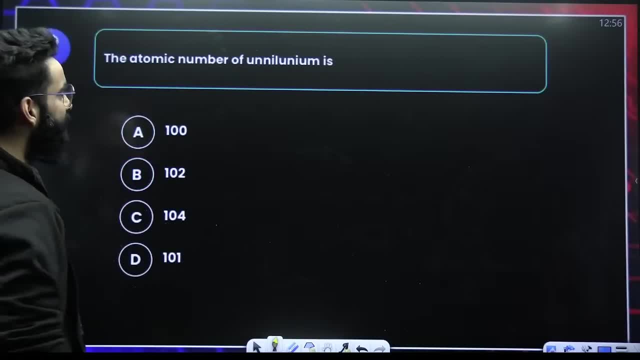 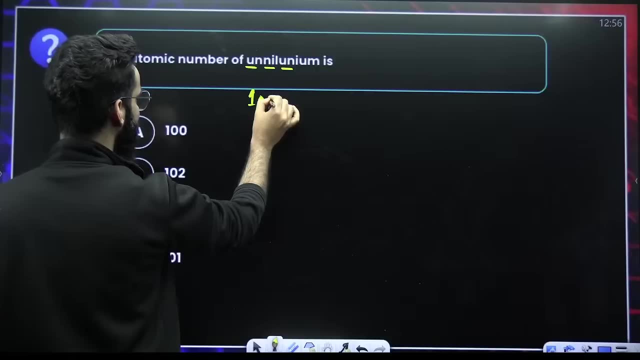 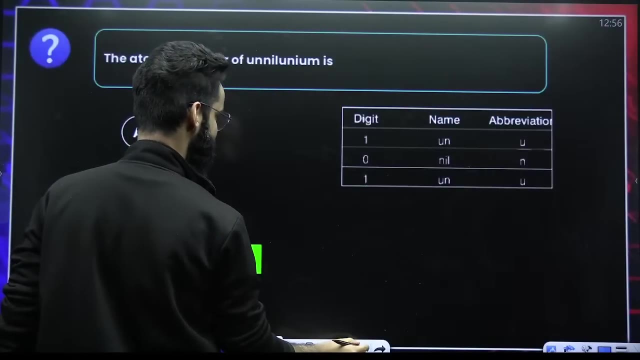 Atomic number of An-Nil-Anyam: An-Nil-Anyam right. An-Nil-Anyam correct. Sorry, Anyam-Anyam, Sorry, sorry, sorry, sorry, sorry, An-Nil-Anyam, Just a second. 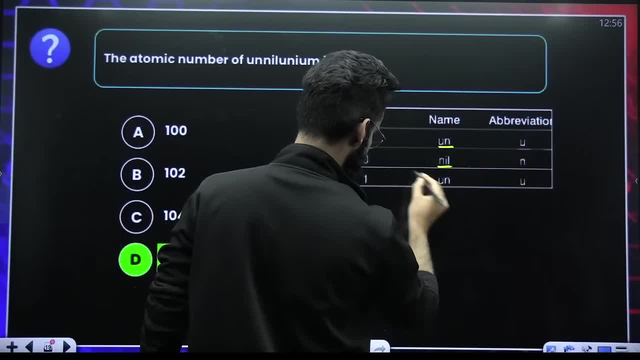 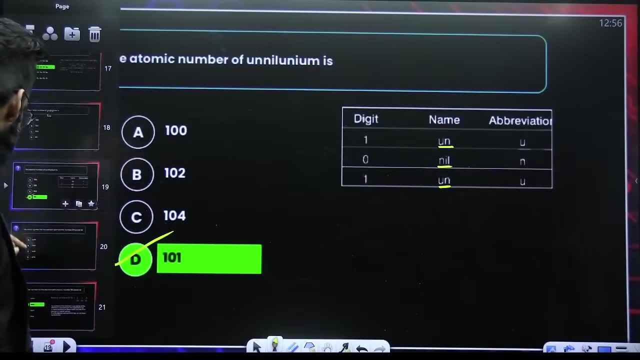 Right. 1 is An, 0 is Nil and 1 is An correct, So it is 1, 0, 1.. So, An-Nil-Anyam Okay. The IUPAC symbol of the element with atomic number of 119.. 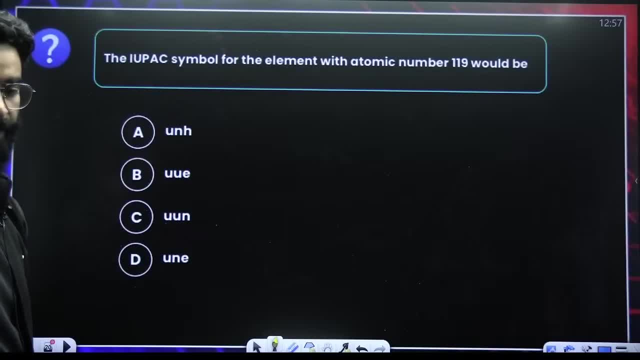 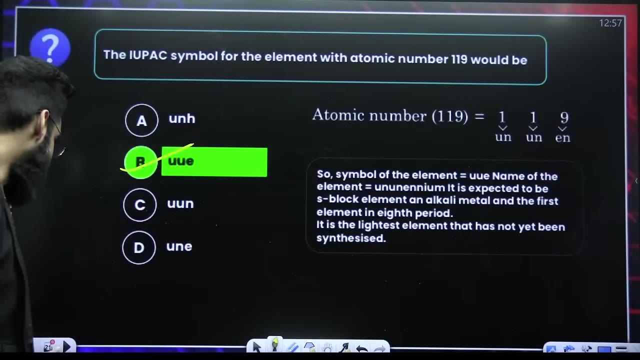 119.. An-An-Anyam Right, Correct. One is An, one is An, Nine is En-En. So what is it? It is An-An-Anyam U-U-E. Alright, The element with Z-E. 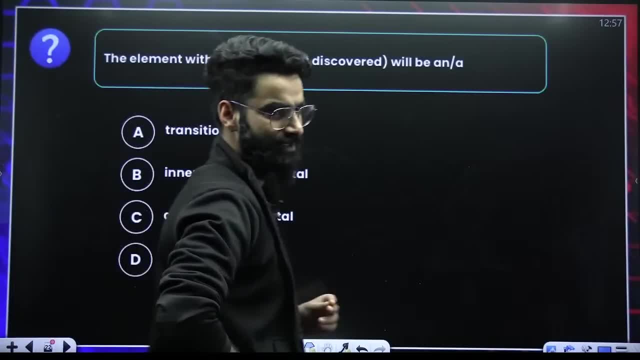 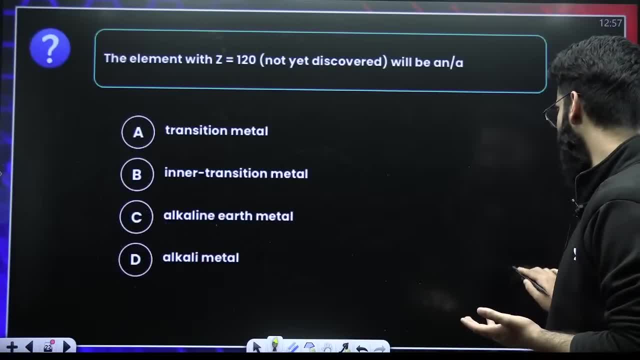 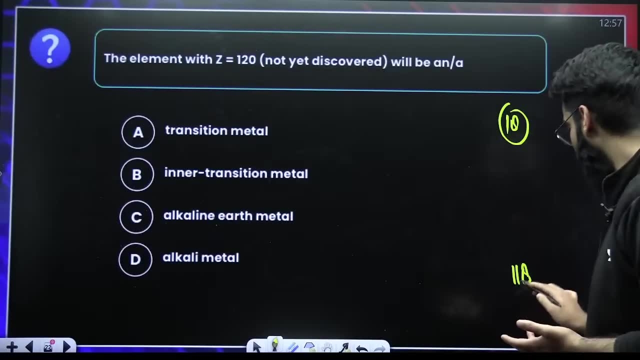 118 elements till now And that 118th element is a noble gas. That's present at group 18.. That's present at group 18.. Perfect, So 109, 119 element. that will be again in group 1.. 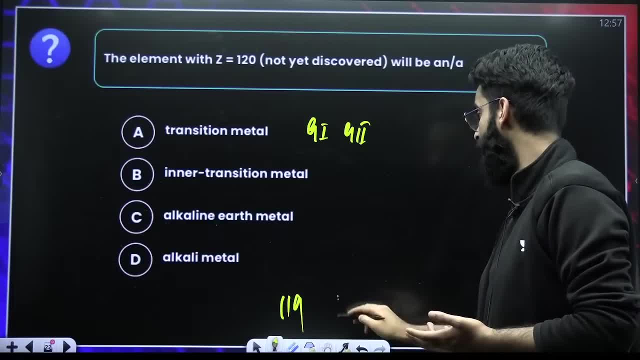 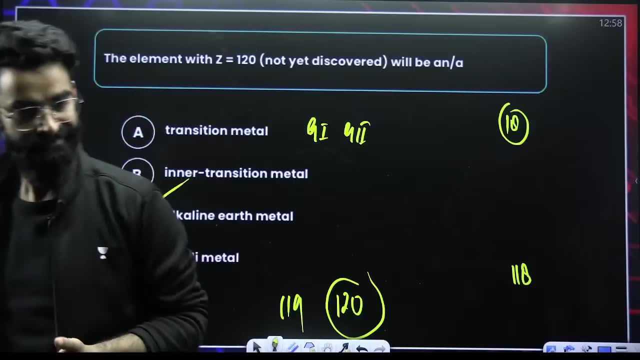 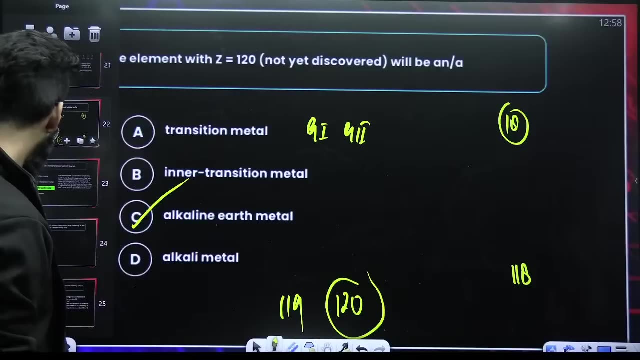 119th will be in group 1.. 120 will be in group 2. So 120 will be in group 2.. Group 2 means alkaline earth metals. Correct, Right guys. The group number: the number of valence electrons. 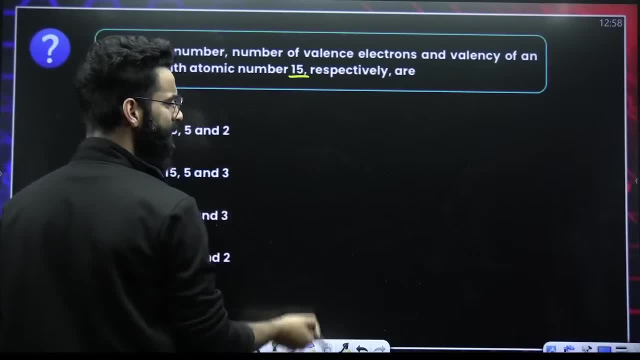 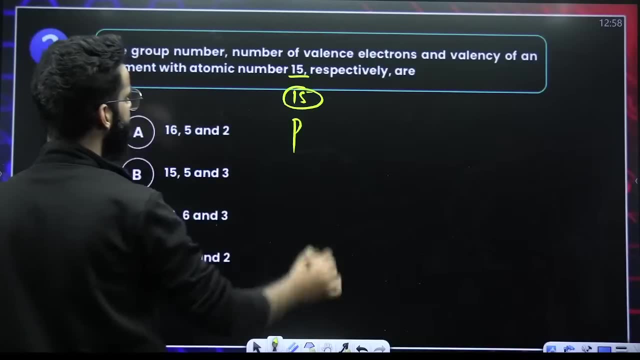 and valency of the element with atomic number 15.. Atomic number 15 means phosphorus. Right, He is talking about phosphorus. Perfect Phosphorus belongs to 15th group, Number 1.. Right, 15th group, Valence. 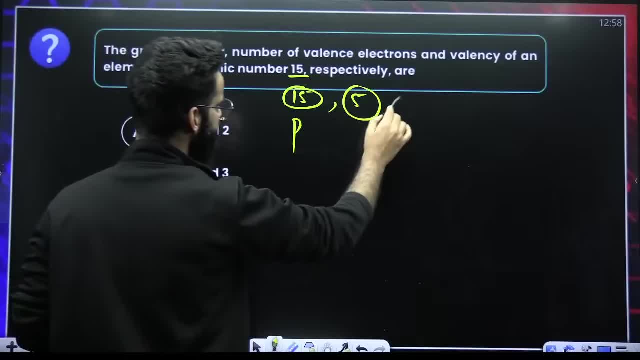 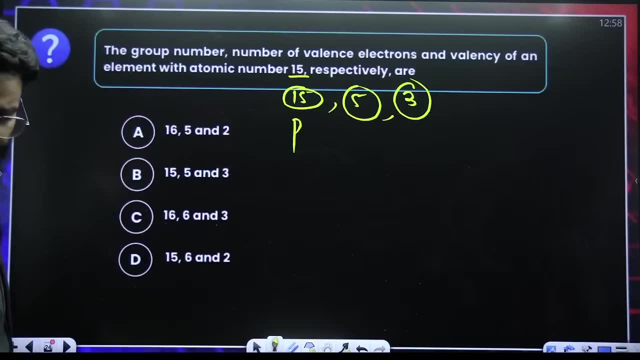 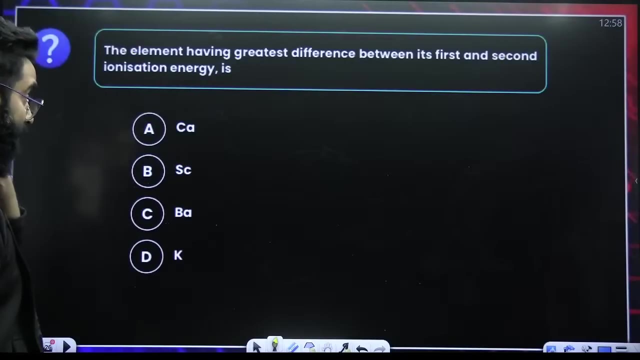 electrons are 5.. Valency is 3.. So 15, 5,, 3.. 15, 5, 3.. Is that Done? 15, 5, 3.. Alright, The element having greatest difference between 1st and 2nd. 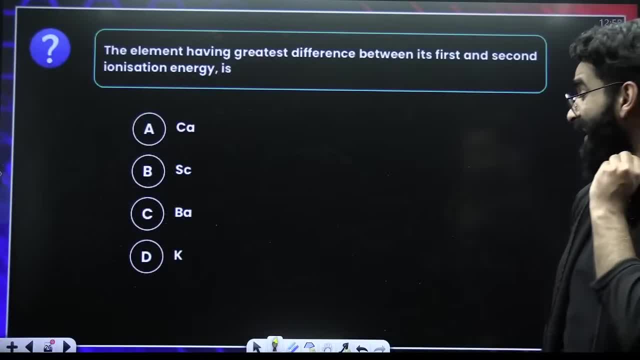 ionization energy. Greatest difference between 1st and 2nd ionization energy. Greatest difference between 1st and 2nd ionization energy: What do you think Greatest difference between 1st and 2nd ionization energy? 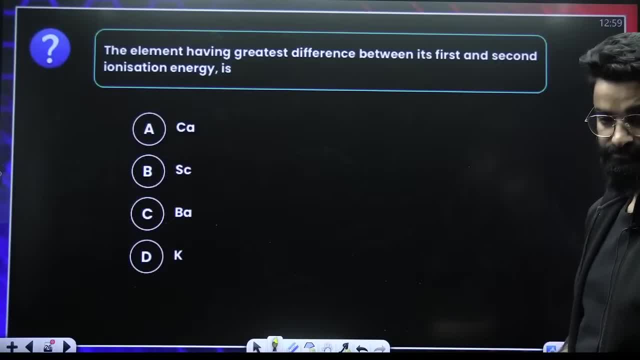 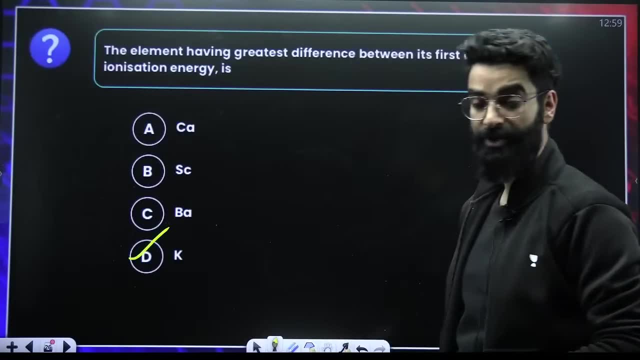 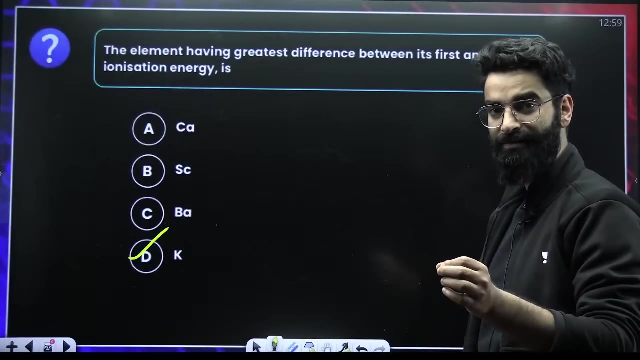 It is potassium, Because this is the only group 1st element. Perfect In group 1st elements. once you remove the 1st electron Right, It attains a noble gas configuration. So to take one more electron out from the noble gas. 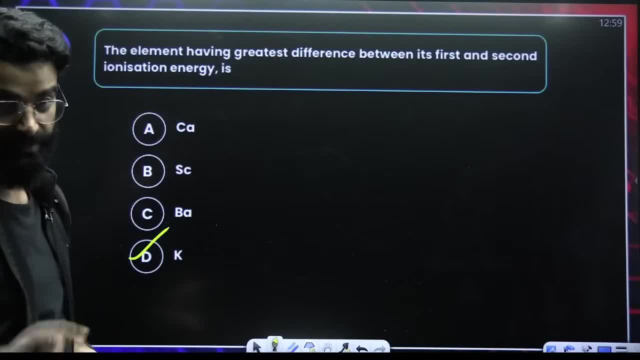 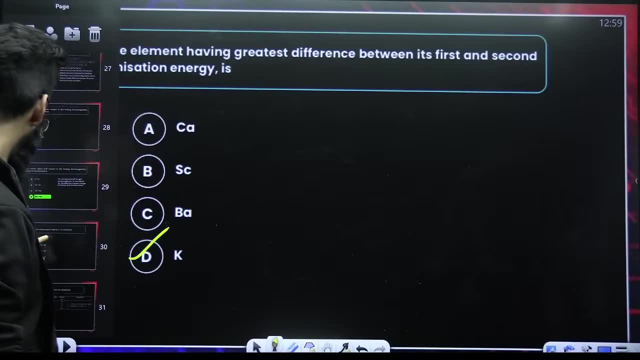 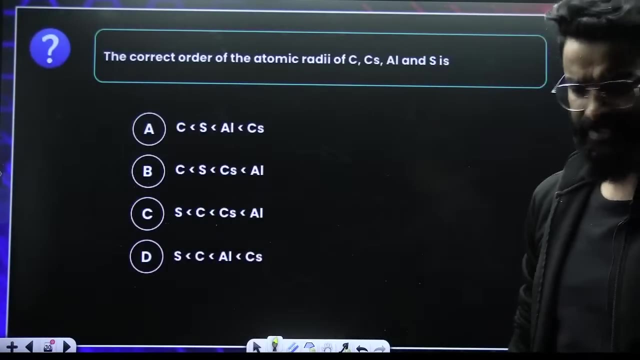 configuration. you need to supply more energy, Right. So difference between 1st and 2nd ionization enthalpy is lot This, I believe you can easily solve This question. I believe you can easily solve Carbon, cesium, aluminium, sulphur- the character of order of atomic radius. 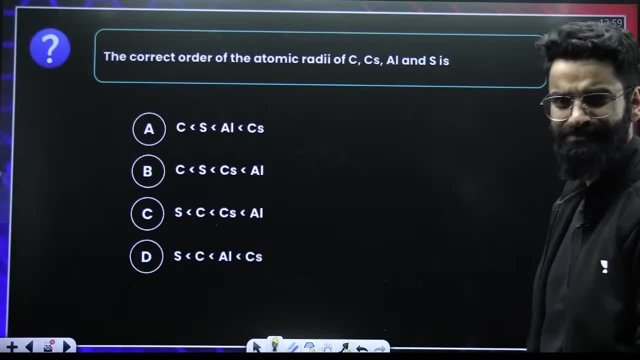 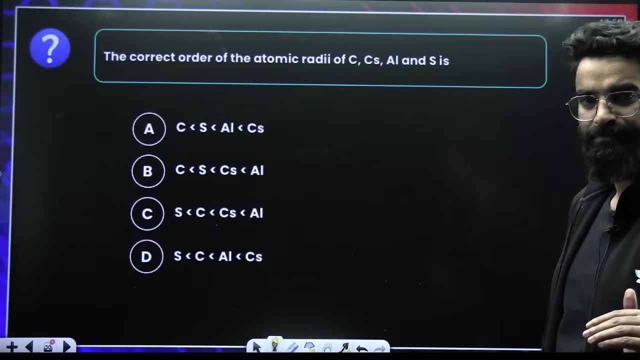 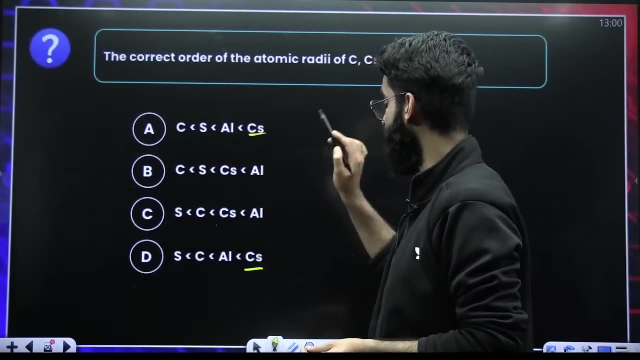 Cesium is at the bottom of the period table. right, You know it. Perfect: Lithium, sodium, potassium, rubidium, cesium, correct. So it will be having maximum radius, so cesium will have maximum radius. cesium will have. 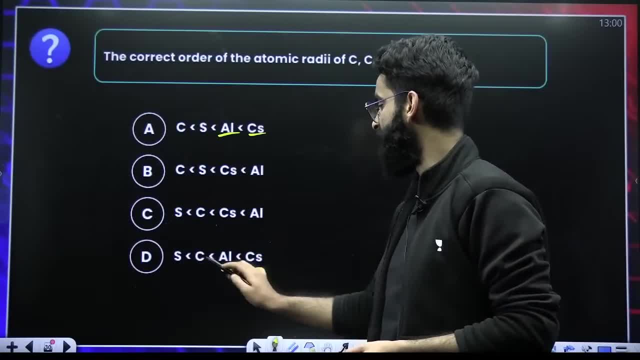 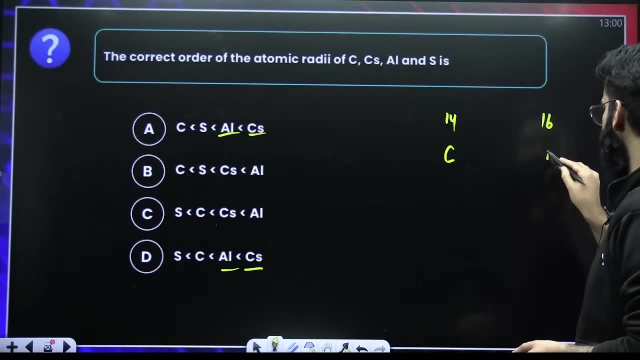 maximum radius right. Leave aluminium aside. Now sulphur and carbon. sulphur and carbon. This is, for example, carbon, which is group 14, group 16, oxygen, and here you have got sulphur, here you have got sulphur. Now compare, compare, compare. 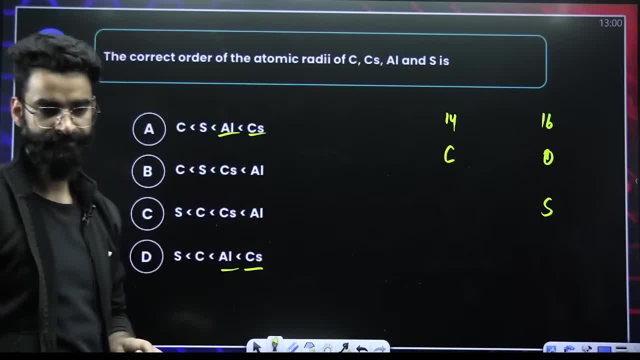 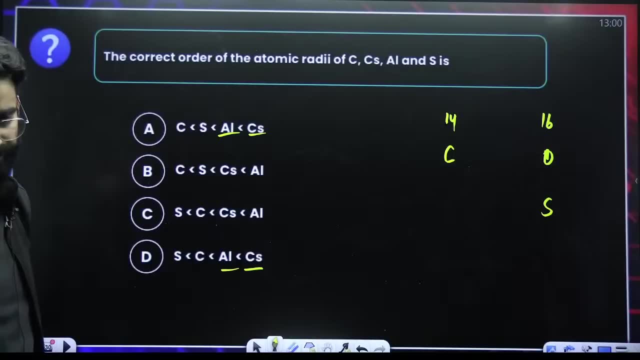 Which one will be having more size, carbon or sulphur. What do you think? Which one will have more size, Carbon or sulphur? Their period is different here. their period is different here. period is different here. Which one has got more size, carbon or sulphur? 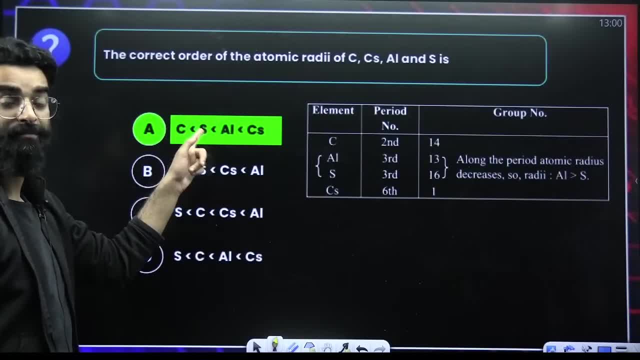 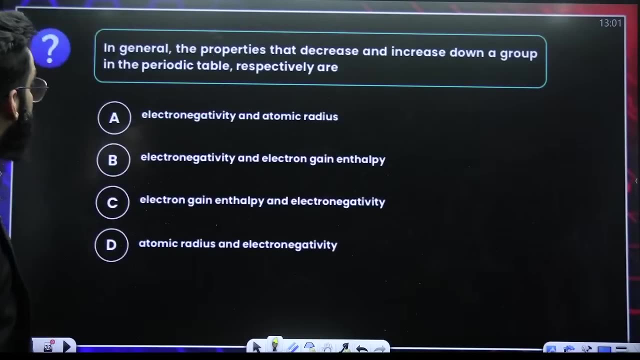 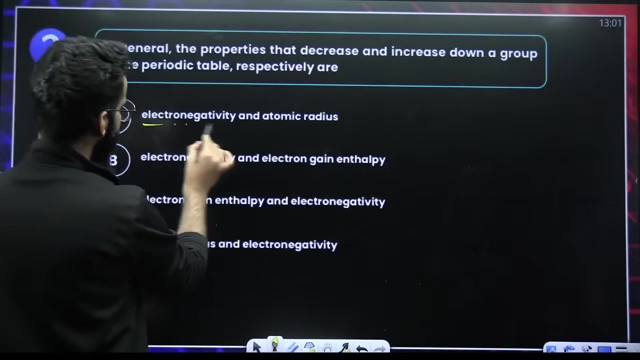 Sulphur has got more size than that of what? Than that of carbon. Why? Because in sulphur right there are more shells. period number is not same right. What is it In general, the property that decreases and increases down the group? electron negativity. 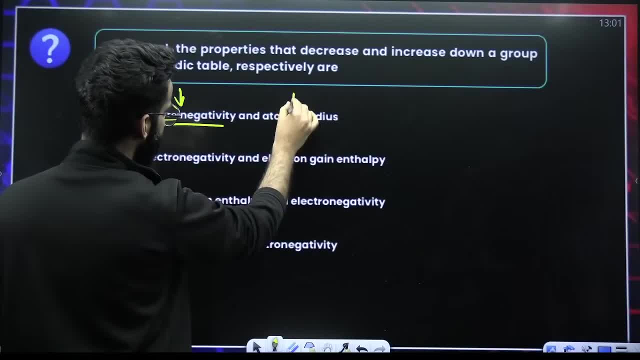 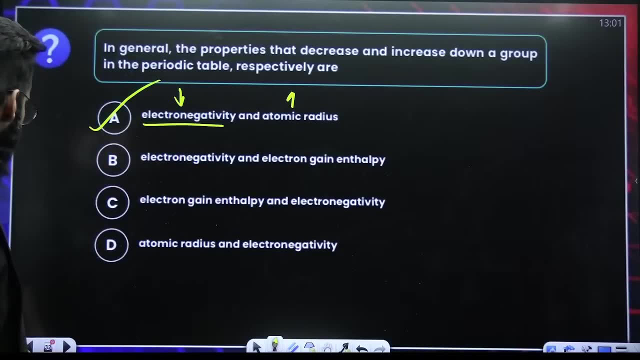 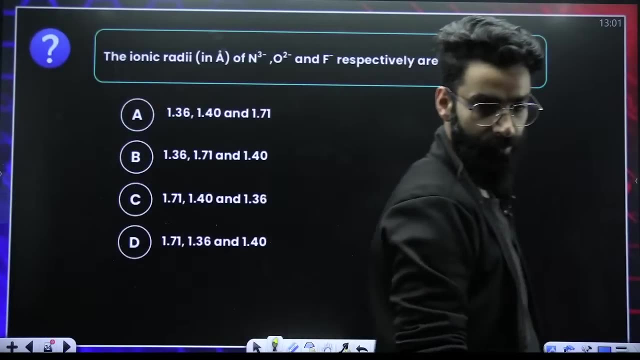 down the group decreases atomic radius down, the group increases. I think this is the answer, right, That's what you have to check The property that decrease and increase down the group. yes, Okay, what about this one? What about this one? 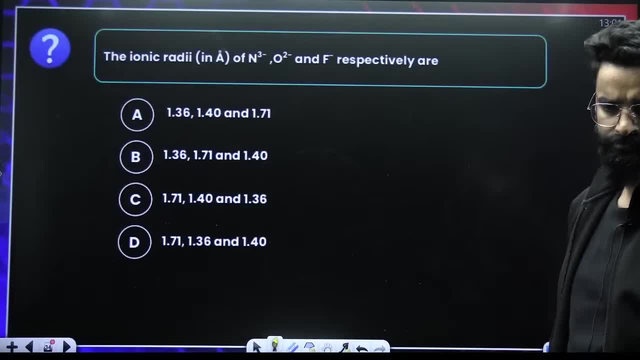 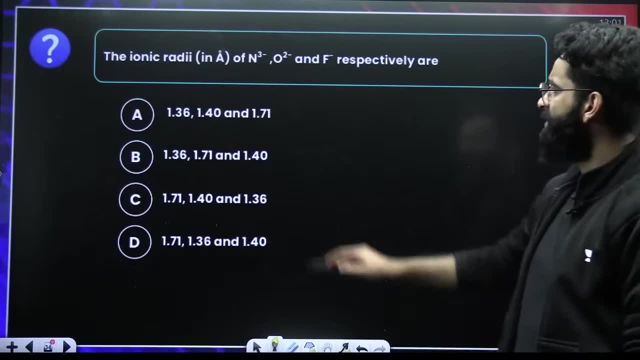 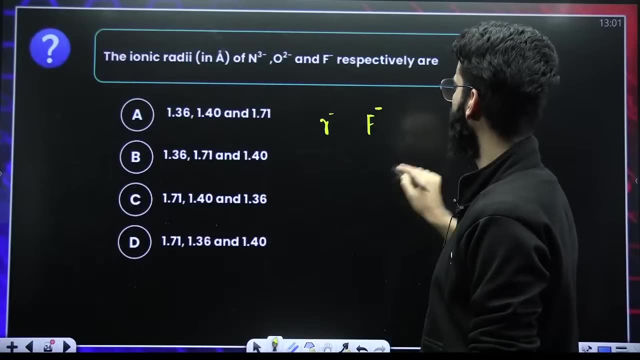 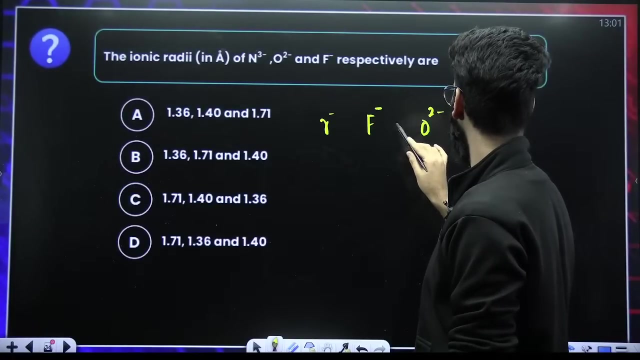 What about this one Ionic radius? see, these are isoelectronic species, right? these are isoelectronic species. least radius will be for F negative. maximum radius will be for N tri negative right And O di negative. is that the middle? 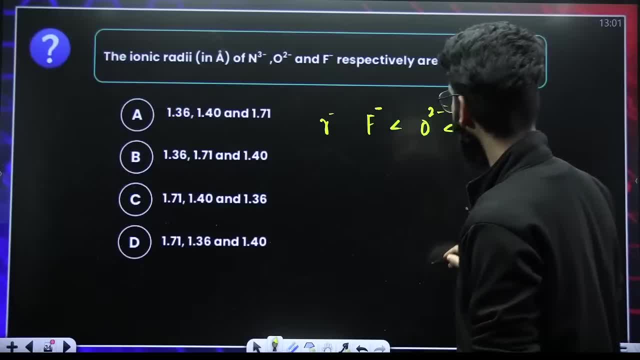 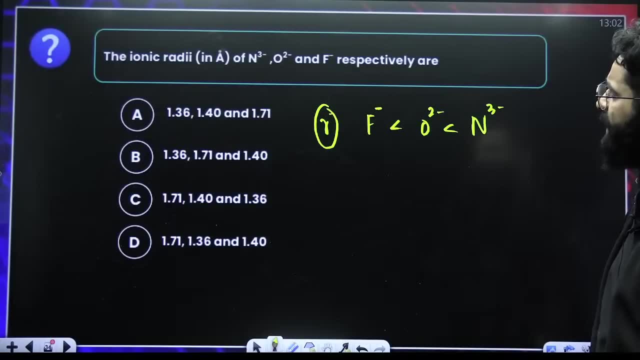 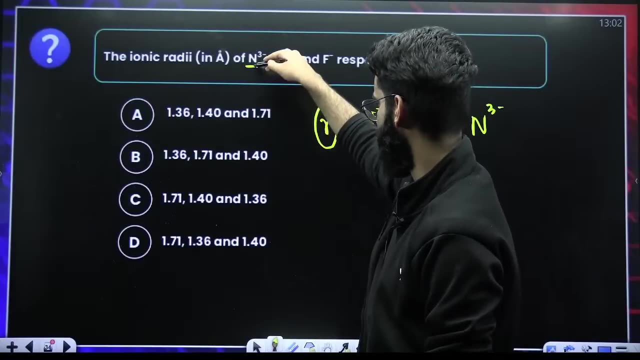 Or did I write the reverse? No least, perfect, least. So this is the order of the radius: N trinegative will have maximum radius. N trinegative will have maximum radius, So maximum radius: N trinegative should have maximum radius. 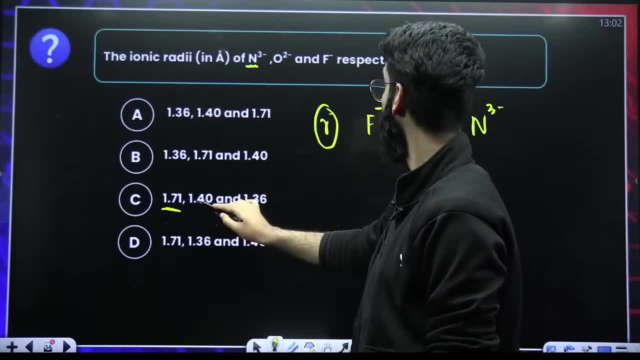 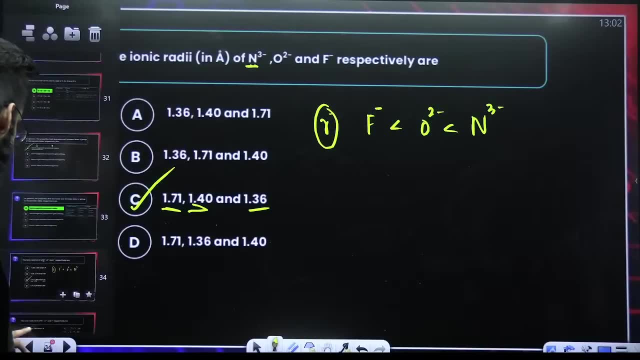 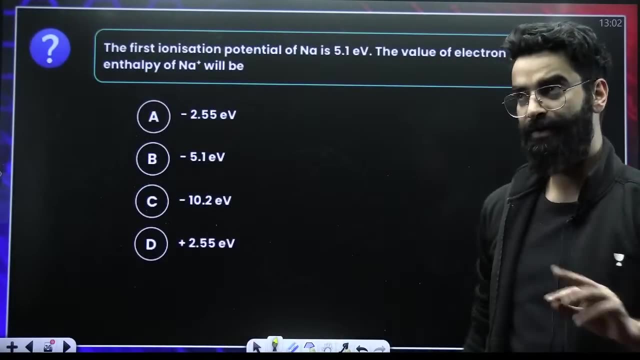 Maximum radius is how much? 1.71.. Then Then 4 denegative, Then this Option C: Right Option C: The first ionization potential of sodium is 5.1 electron volt. Electron gain, enthalpy. 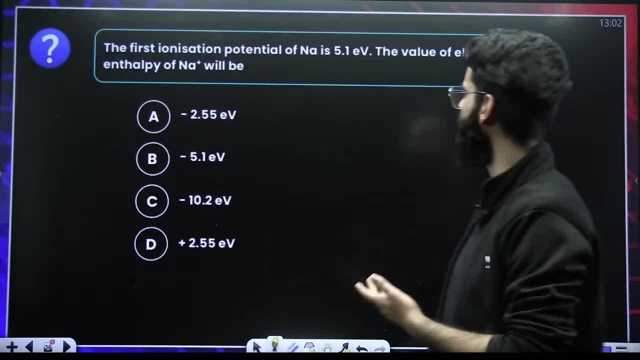 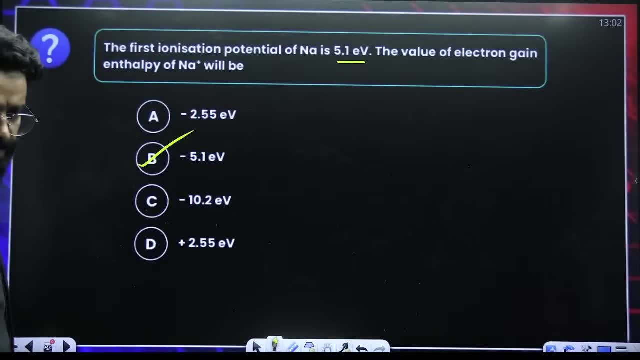 The value of electron gain enthalpy, Which is reverse Right. So if it is plus 5.1, it has to be minus 5.1.. Simple, Simple guys. Okay, The set represents the correct order of first ionization potential. 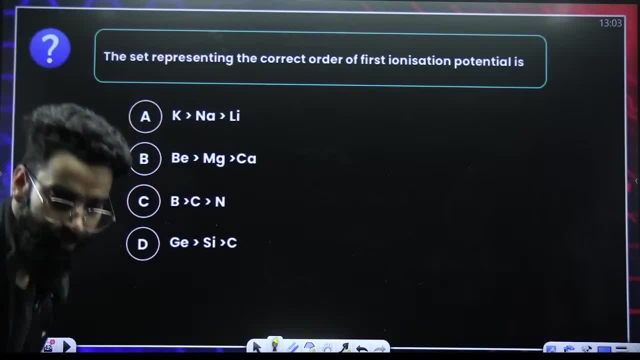 The set represents the correct order of first ionization potential. Can you check it out? Can you check it out, guys Quickly? Can you check it out quickly? Yeah, Quickly, guys. Corrects the set representing the correct order of first ionization potential. 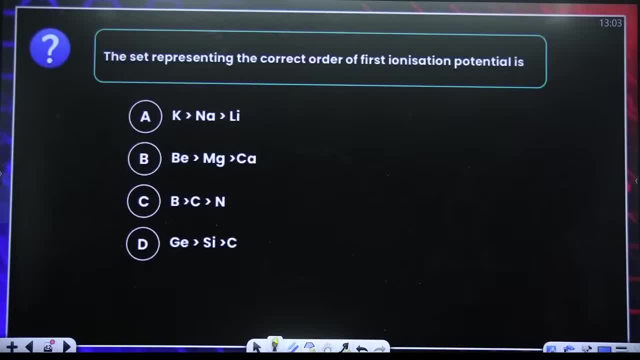 Down the group ionization potential decreases. Down the group ionization potential decreases. So beryllium will have maximum, Followed by Magnetium, Followed by Calcium. Which one is correct? Which one is correct? Which one is correct? 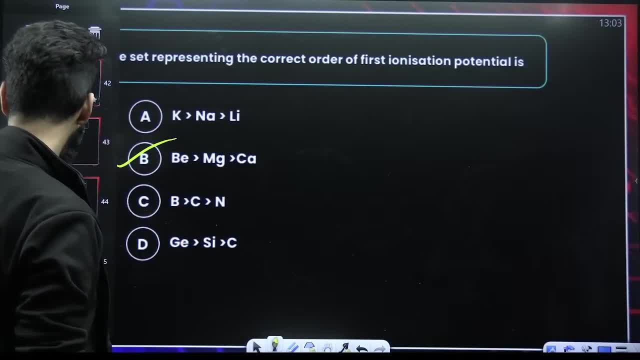 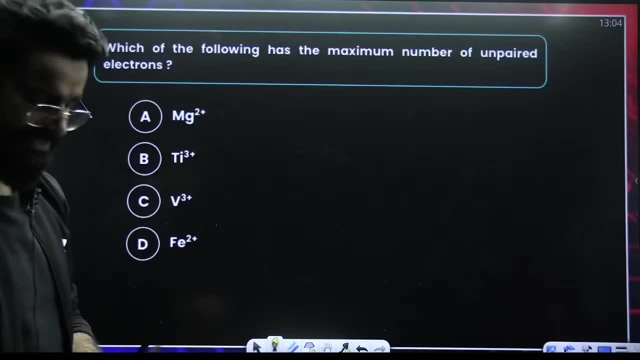 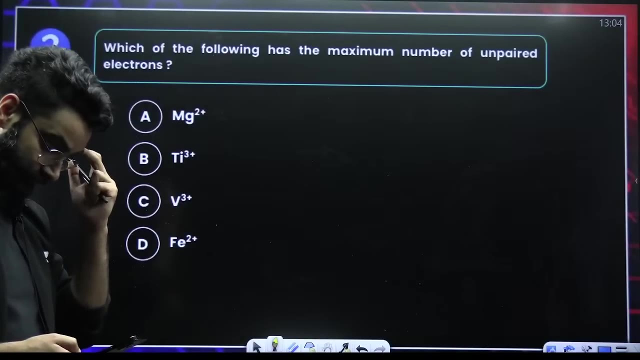 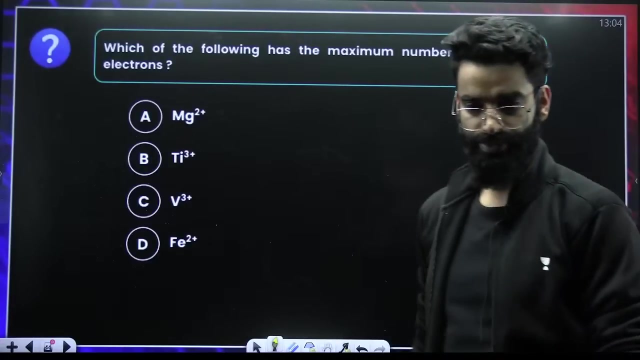 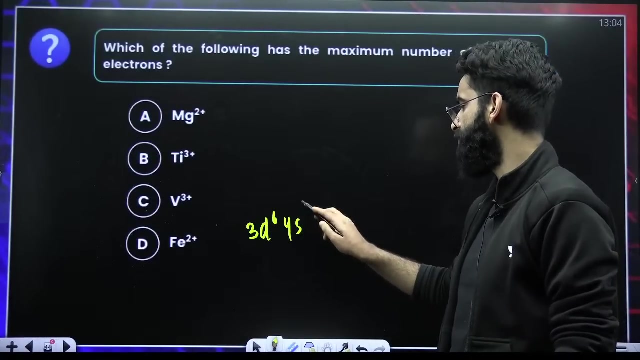 it is B. which of the following has maximum number of unpaired electrons? quick: maximum number of unpaired electrons. maximum number of unpaired electrons. if you look at Fe di, positive iron has got 3d6, 4s2, so take 2 electrons out. 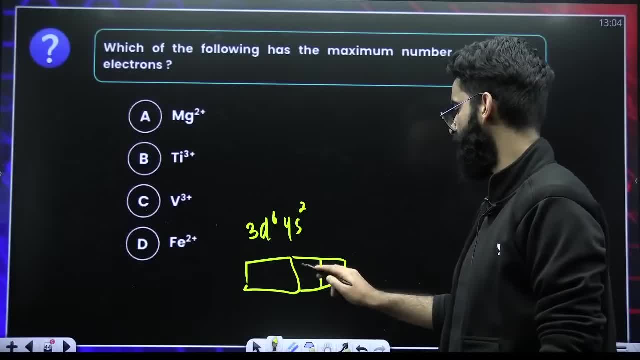 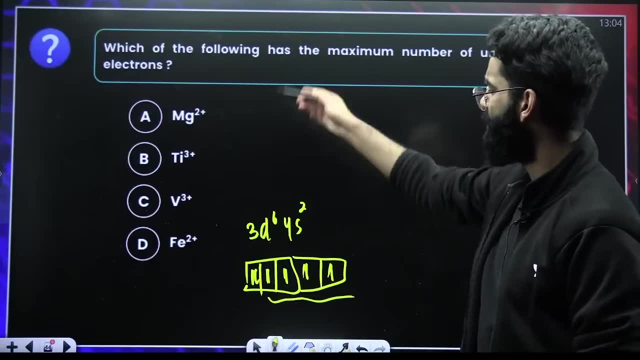 it is 3d6. it is 3d6. it is 3d6. 1, 2, 3, 3, 4, 5, 6, so 4 unpaired electrons here. similarly, you can check the rest- this will have maximum unpaired. 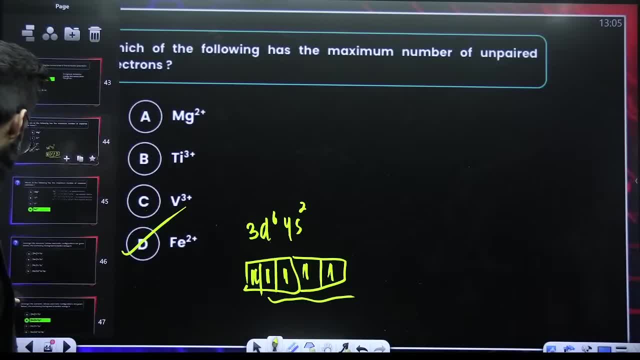 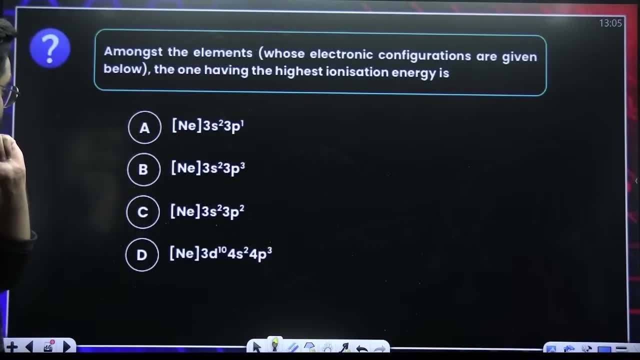 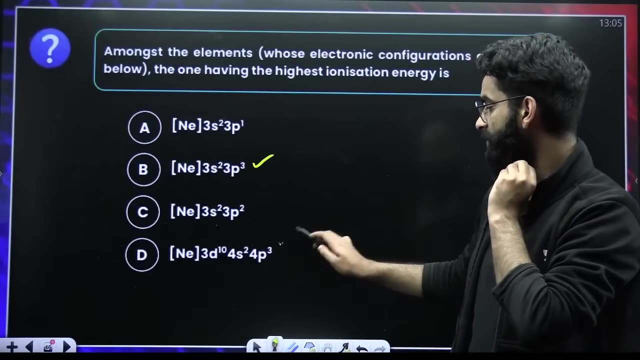 electrons here. this will have maximum unpaired electrons here. among us the elements whose electronic configurations are given, the one having highest ionish energy, highest ionish energy. this is half filled. this is also half filled. 3p3, 4p3, right, so half filled. 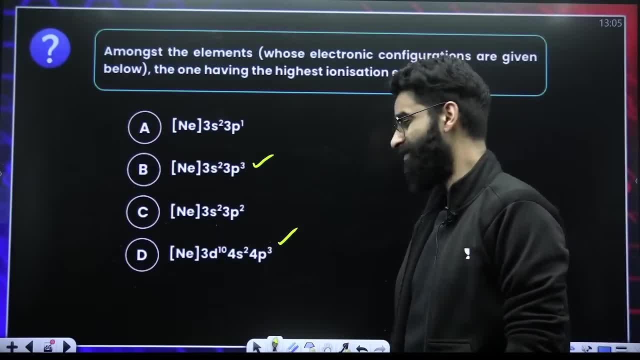 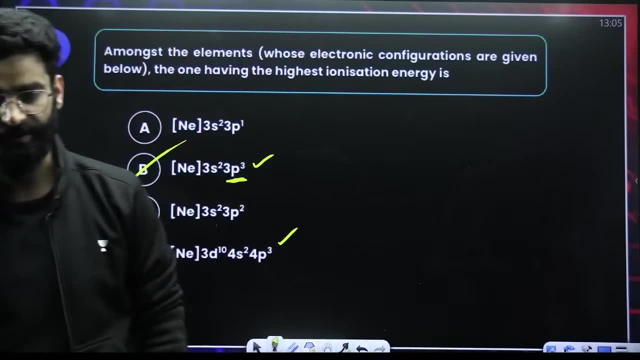 configurations are more stable. to take electron out from then you have to supply more energy. but this is 3p3, this 4p3. this is closer to the nucleus, so this is difficult to take out. more energy is needed. this is difficult to take out. 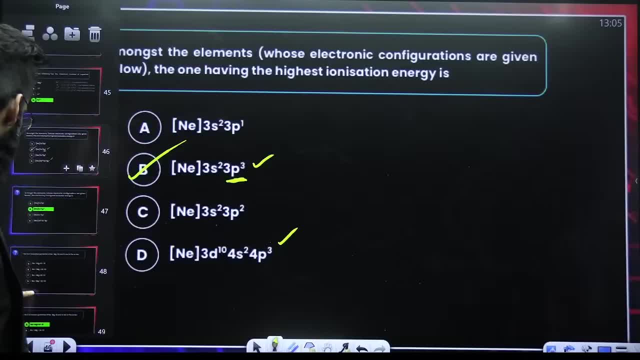 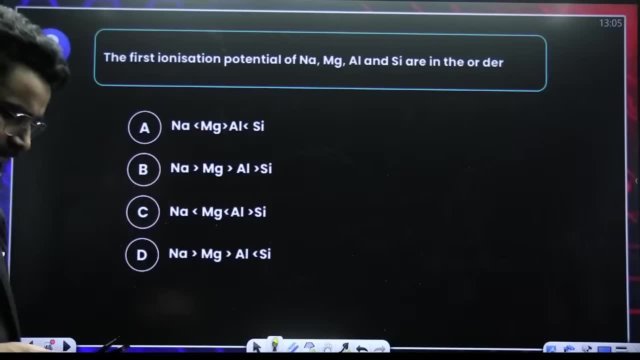 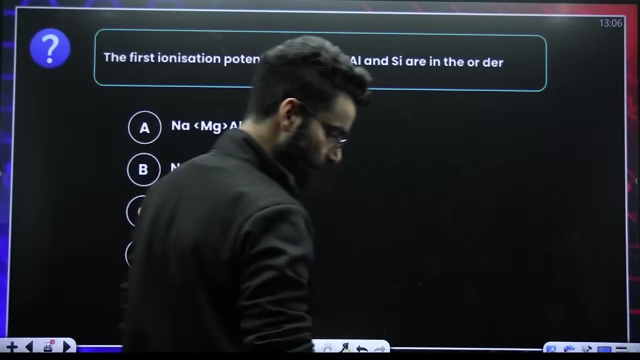 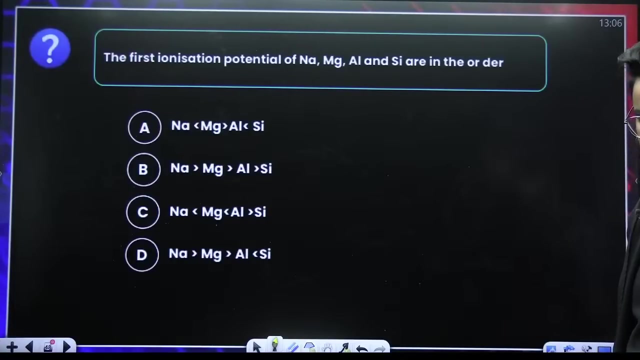 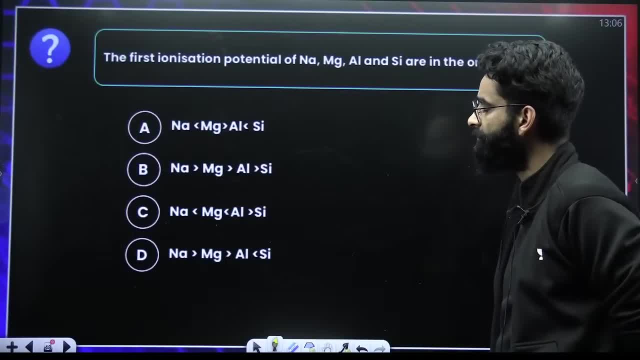 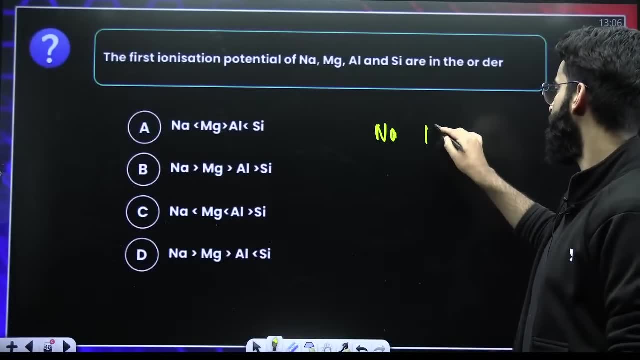 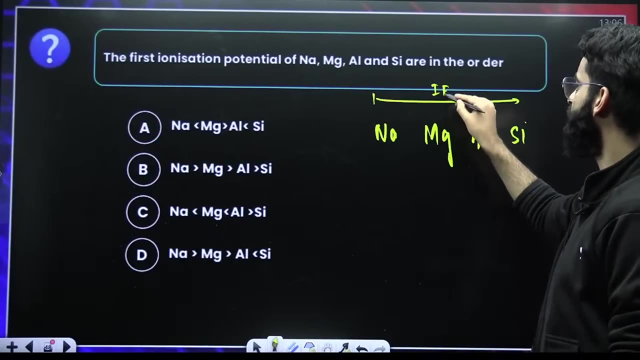 1 sodium, magnesium, aluminium silicon. they belong to same period. right sodium magnesium, aluminium silicon. they belong to same period. on moving from left to right, ionish energy increases. ionish energy increase. so this has to be the order. this has to be the order. this is the. 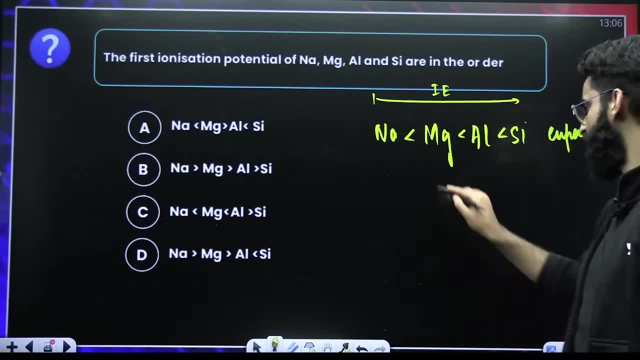 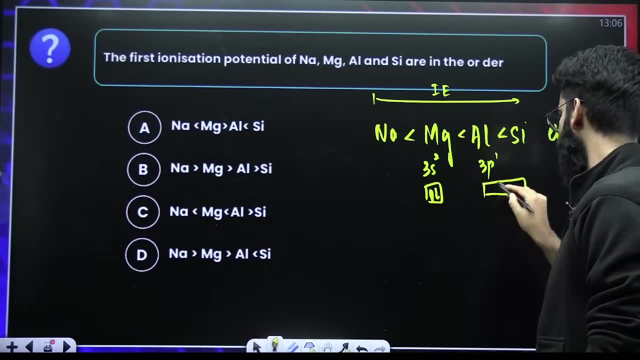 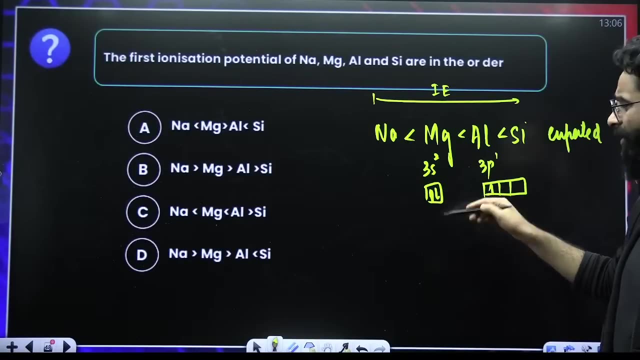 expected order. but is this going to be actual? no, ps2 configuration. here you have got 3p1 configuration, perfect ps2 configuration. 3p1 configuration. this completely filled. this is filled, this partially filled, or you can say s has got more penetrating penetration power to take the electron out from here. you have to supply more energy, so ionization potential. 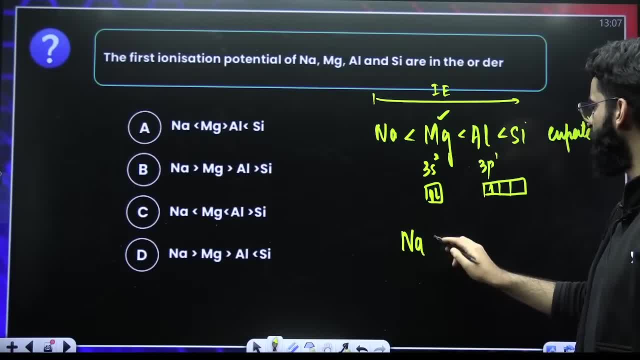 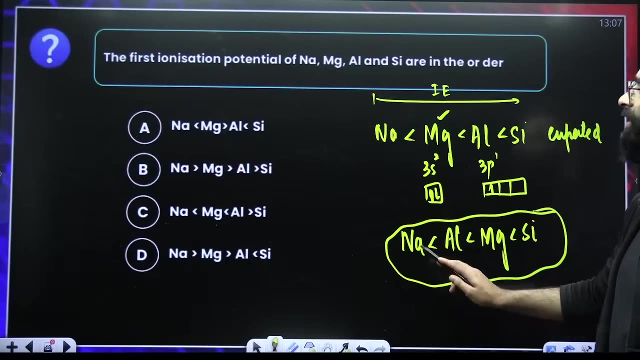 of magnesium has to be greater than that of ionization potential of just a second. yes, ionization potential of magnesium has to be greater than that of aluminium. just everything is same. is there any option like this: sodium has got least, then magnesium, but magnesium has got greater than aluminium. perfect it. 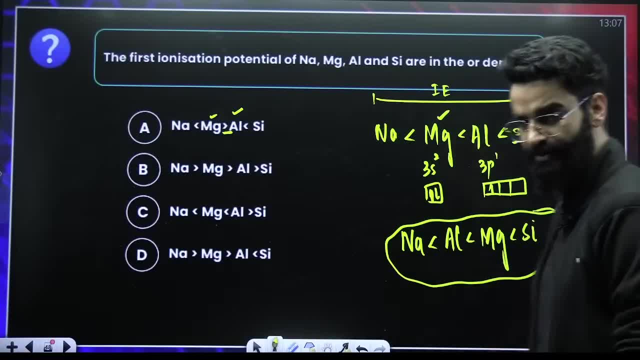 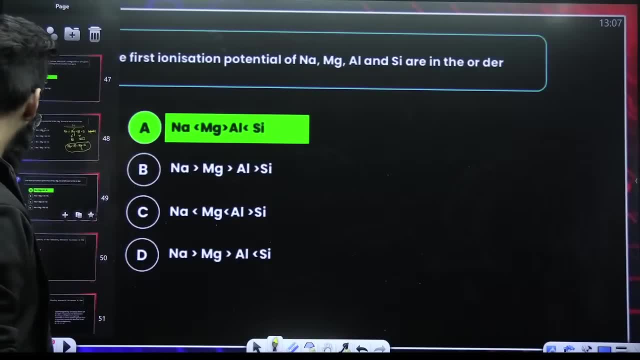 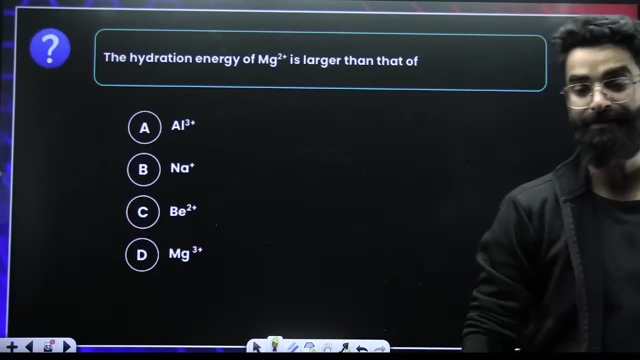 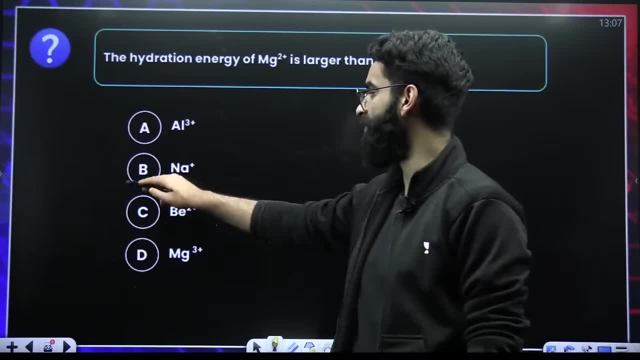 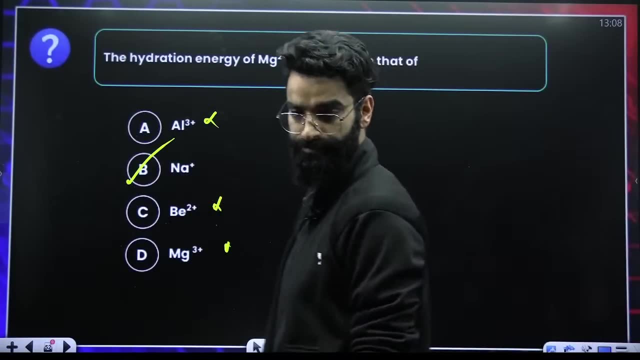 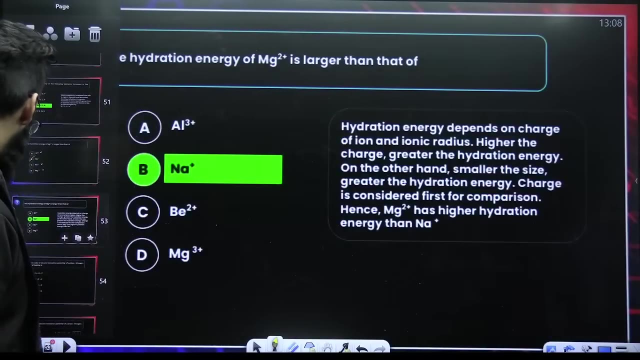 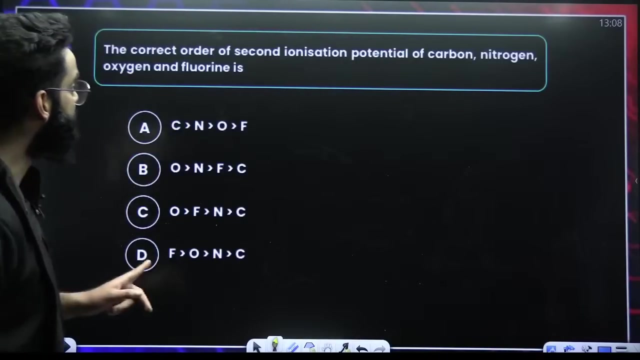 energy of mg di positive is larger than it will be larger than any positive right mg dipole. less than this. it will be larger than any positive follow it will be larger than any positive. the correct order of second ionization potential. the correct order for the second. already you. 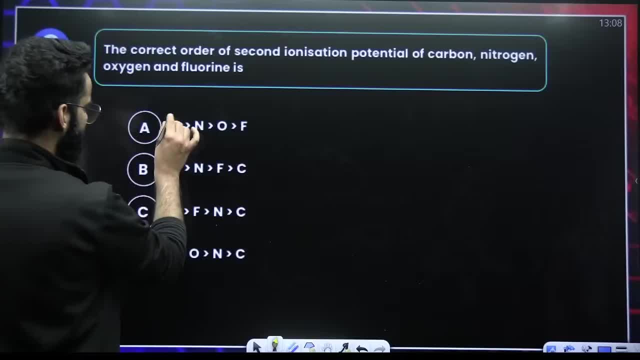 have taken one electron out to the second potential. there is a further potential. in the second potential is fixed salt презид status of oxygenhan, then off the treatment. so when you take one electron out from carbon it becomes 2p1 configuration. this becomes 2p2. 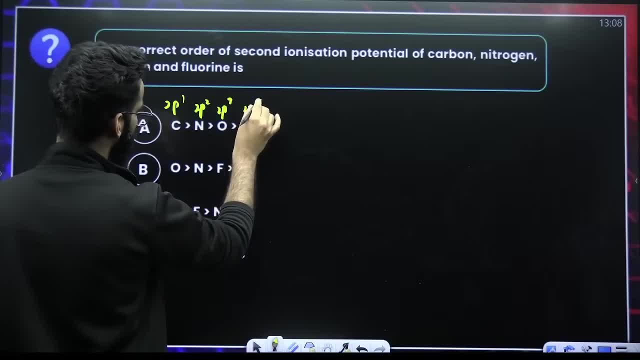 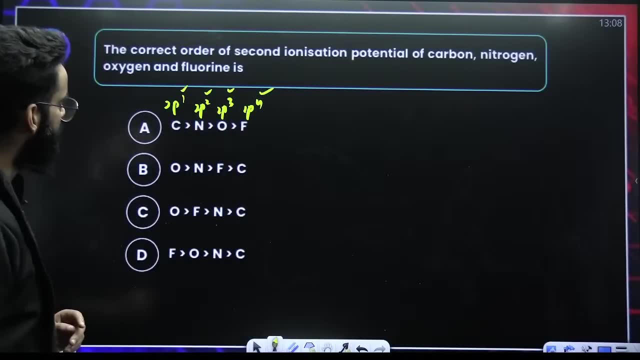 configuration. this becomes 2p3 configuration. this becomes 2p4 configuration. correct, now you have. take one electron out from these, from these configurations. so second will be maximum for oxygen, second will be maximum for oxygen, perfect, and after oxygen it's, it's evident, it's going to. 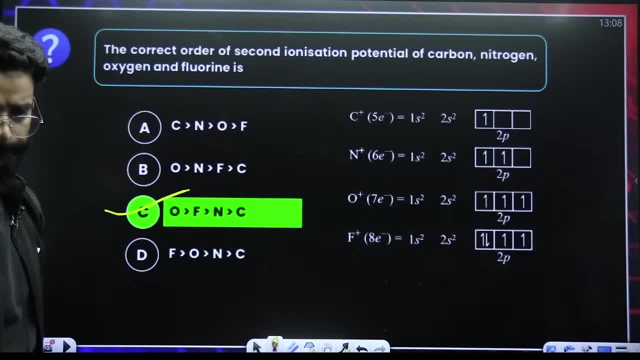 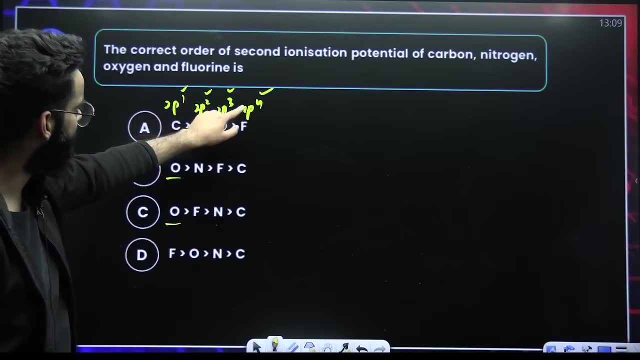 be then fluorine, etc. etc. okay, right, i hope you got what i said. one electron here, one, two electrons here, three here, four here, because we have already taken one electron out. now the second electron here has to be taken from 2p3 half field configuration, so second ionization potential. 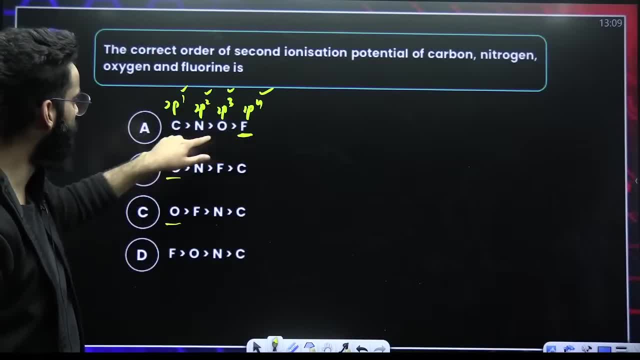 of oxygen is more here. the electron has to be taken out from 2p4 and the electron has to be taken from 2p2. but this is fluorine right, 2p4 configuration, 2p4 configuration. you here you have got more protons right, more protons, so to take electron out from here. 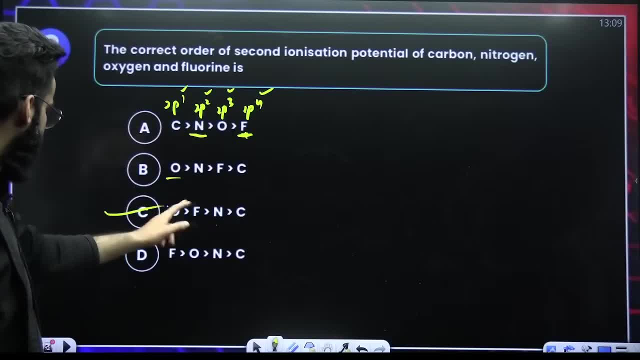 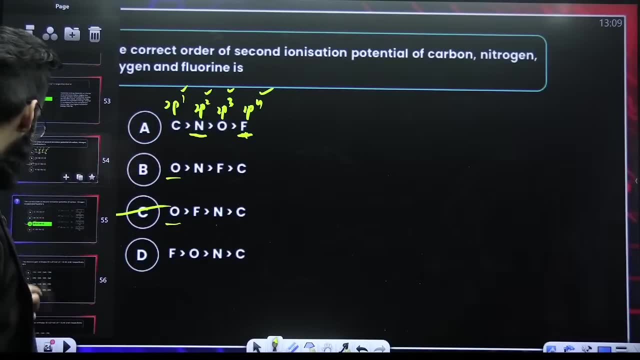 right. that will be difficult as compared to 2p2 configuration. that's why i told you option c is the answer. that's why i told you option c is the answer. someone is saying option d- hoga, i told you option c. still you are saying option d. okay, you write option d in your exam. 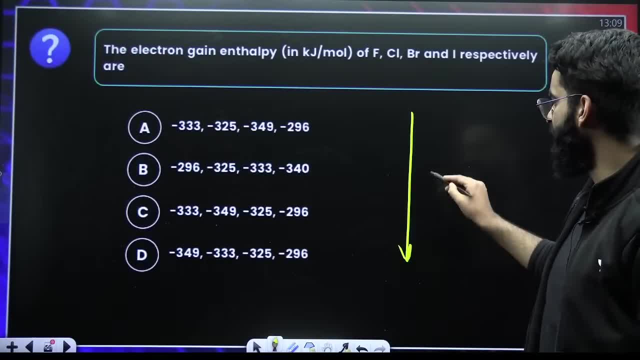 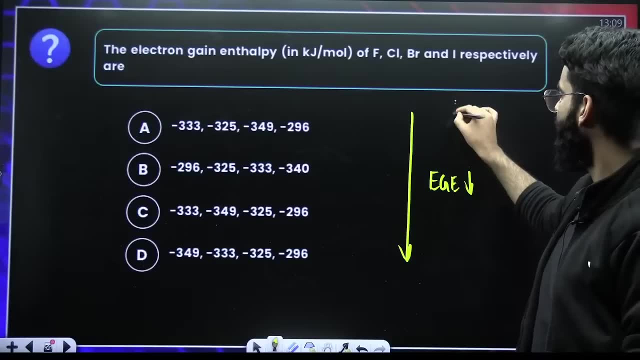 all right. electron gain enthalpy. on moving from top to bottom, electron gain enthalpy decreases right. on moving from top to bottom, electron gain enthalpy decreases right. so fluorine should have maximum, followed by chlorine, followed by bromine, followed by iodine. but due to smaller size of 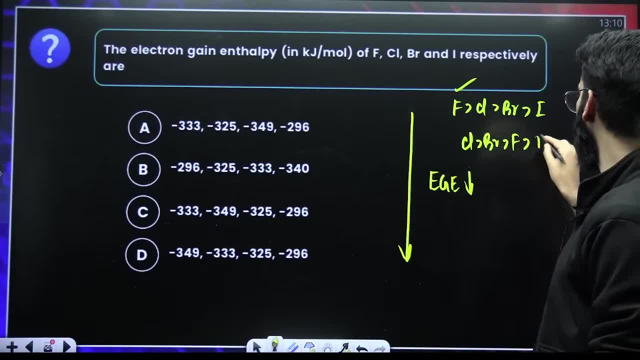 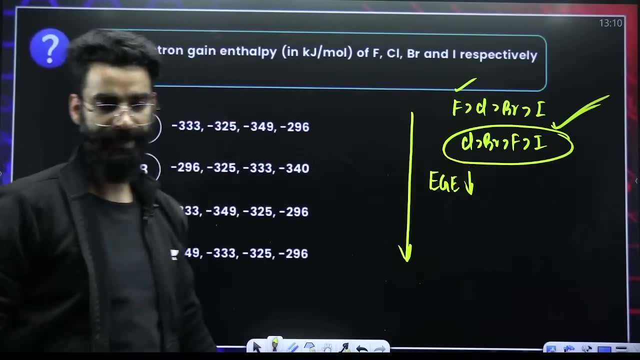 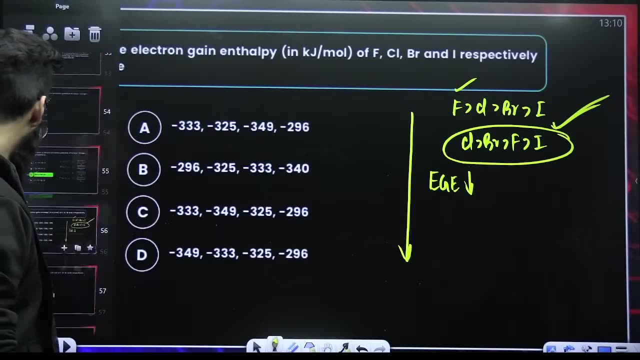 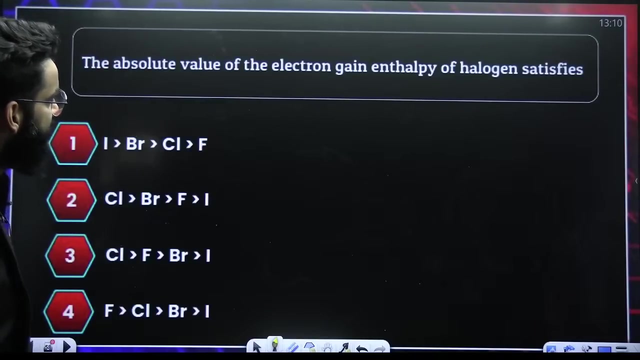 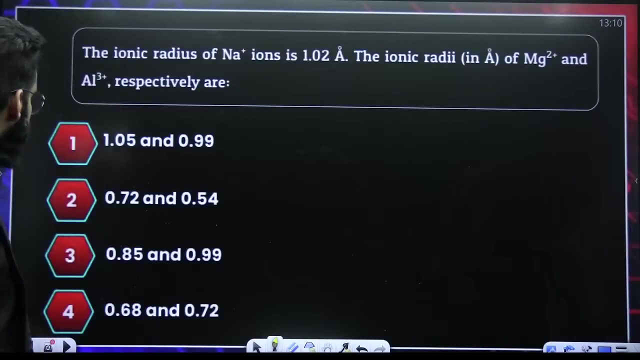 chlorine. the order gets reversed. chlorine comes at the third spot, right, and this is the actual order. this is the actual order. this is the actual order of electron gain enthalpy. okay, this is the actual order of electron gain enthalopies, so that's not a quelle. 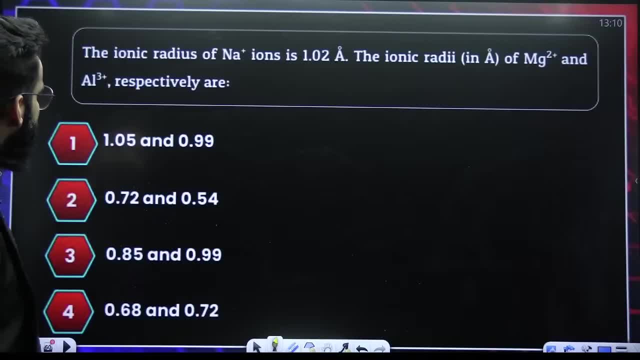 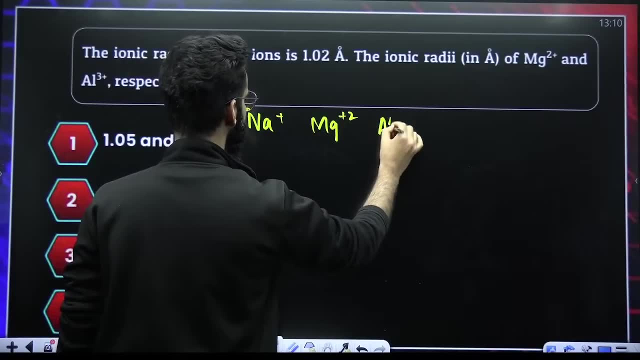 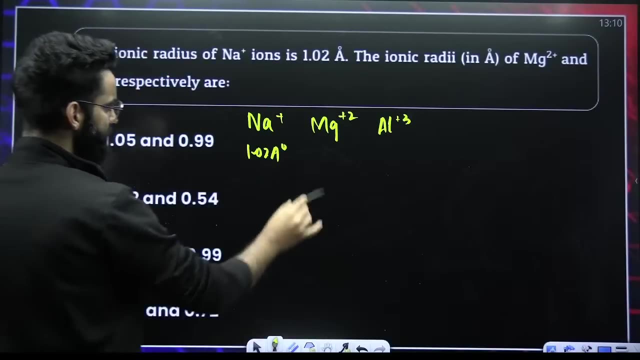 absolute value of electron gain. enthalpy of halogens. i told you clbr, fluorine i, option 2. the ionic radius of na positive. is this: the ionic radius of mg diphes to an l tri positive will be positive, right. Its radius is 1.02 angstroms. 1.02 angstroms. Now size will be maximum. 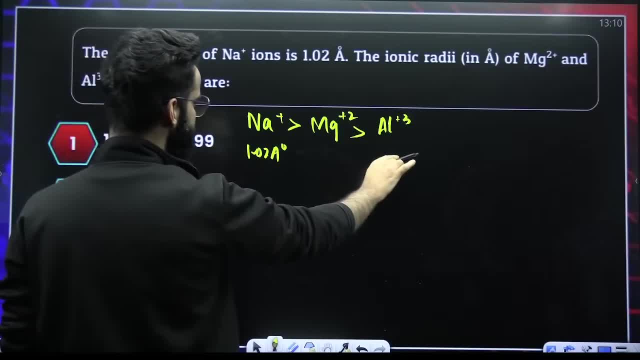 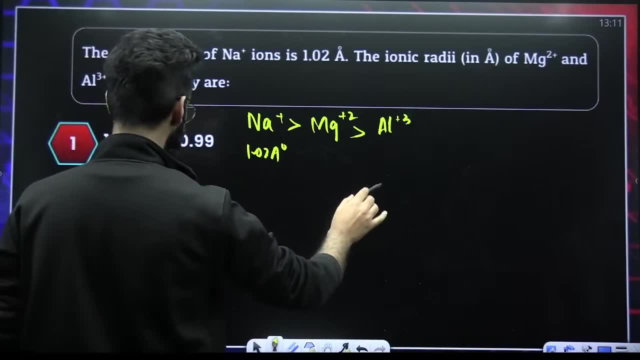 for this right. So AL tri positives radius has to be the least, Which is the least one, Which is the least one: 0 point. This has to be least. This has to be comparatively more So it has to be, I believe, 0.72 and 0.54, right, These are the only options which. 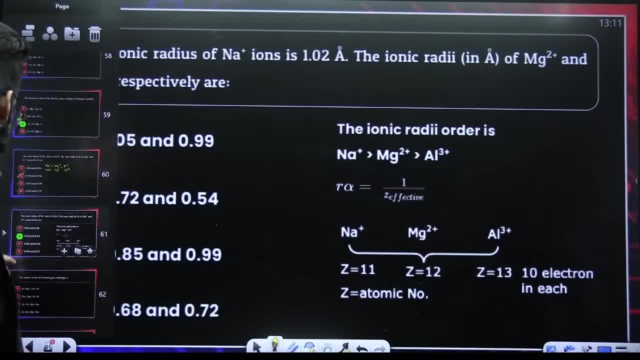 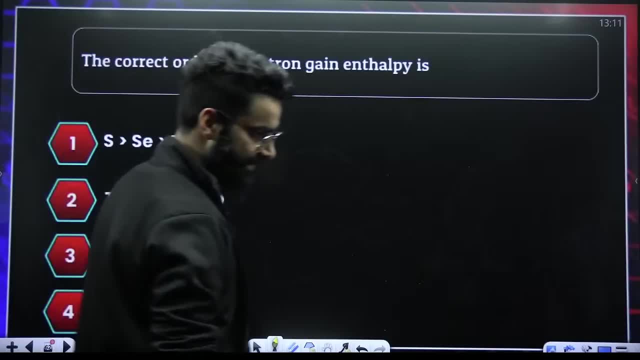 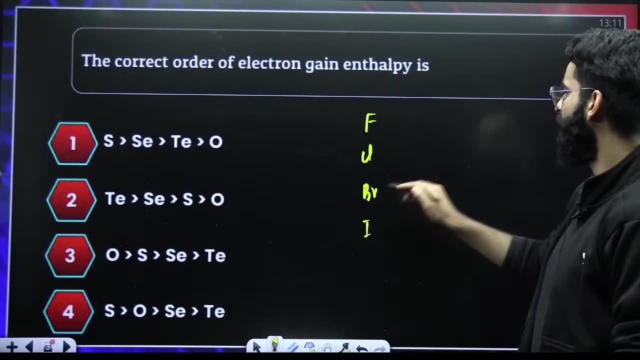 are satisfying our condition. Okay, These are the only options which are satisfying our condition. The correct order of electron gain enthalpy: See, as I told you, you have got group 17. Fluorine, chlorine, bromine, iodine, acetylene, right Group 16. Oxygen: 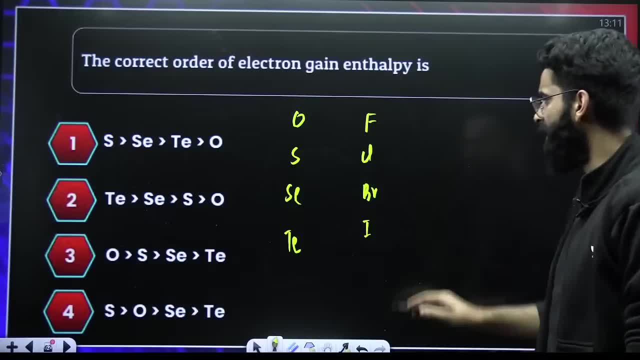 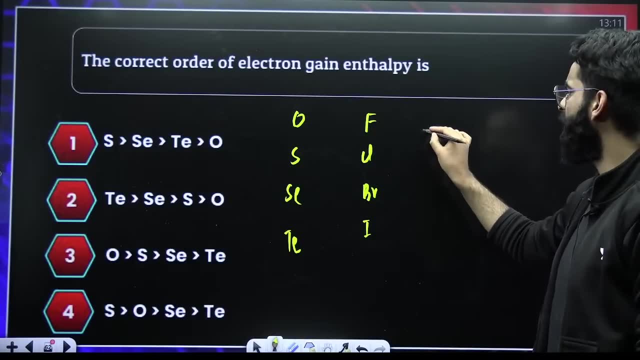 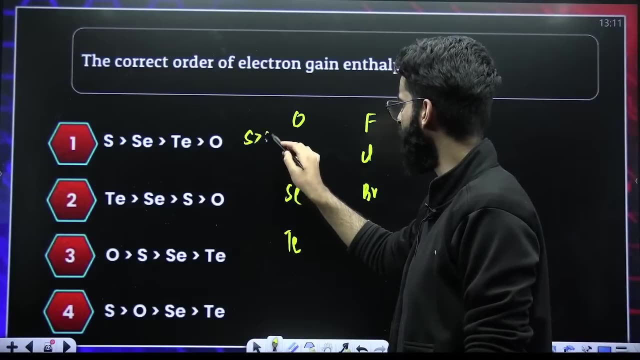 sulphur S et Perfect On moving down the group. generally electron gain enthalpy decreases. right Electron gain enthalpy decreases but chlorine has got more electron gain enthalpy than the fluorine because of the smaller size of fluorine. Similarly, sulphur has got more electron gain enthalpy. 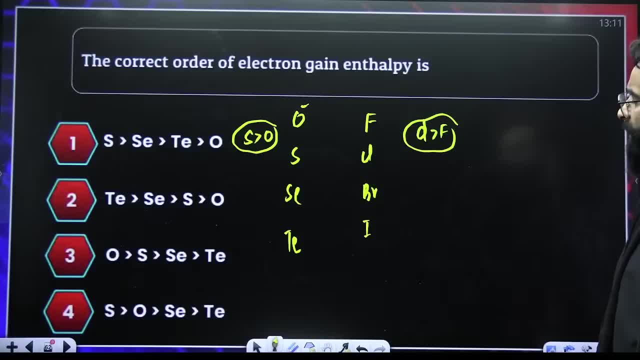 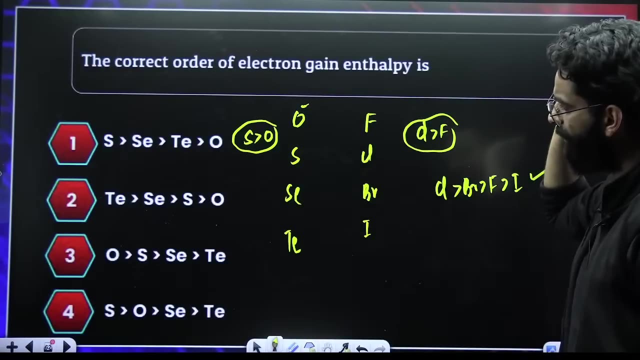 than oxygen because of the smaller size of oxygen. Perfect, The order here becomes the final order. here becomes, as I told you, Cl, then Br, then F, then I. This is the actual order of electron gain enthalpies. Here. what the order becomes, Oxygen comes at the end. 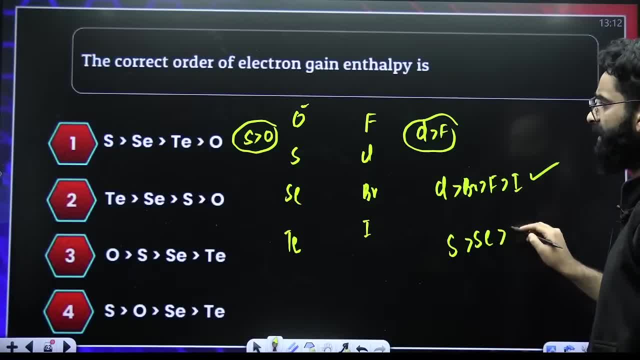 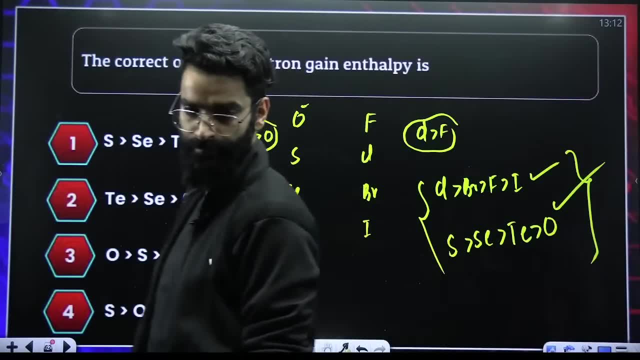 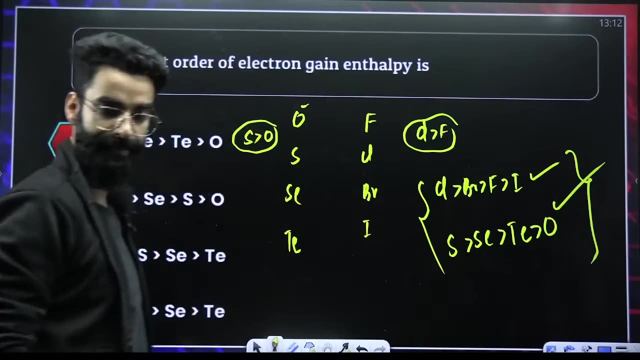 Oxygen goes to the end. So here the order is sulphur, Se, Te and oxygen at the end. These are the actual orders of electron gain enthalpies. right In case of group 17,. fluorine does not go to the end. Fluorine takes the third spot, but here oxygen goes to the end. I hope. 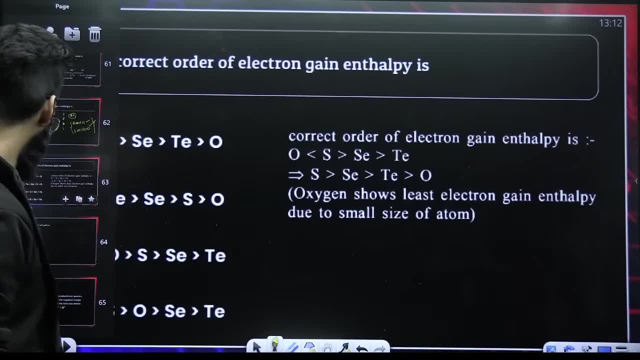 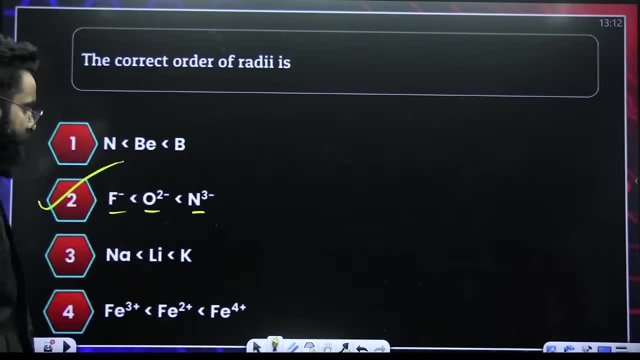 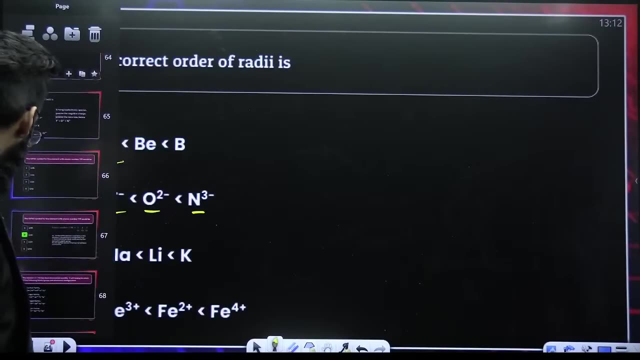 I am clear what I said: The correct order of radius. These are isoelectronic species, right, And they are given with correct set of radius: more, less, less. Guys, all these sorts of questions, we have done What? 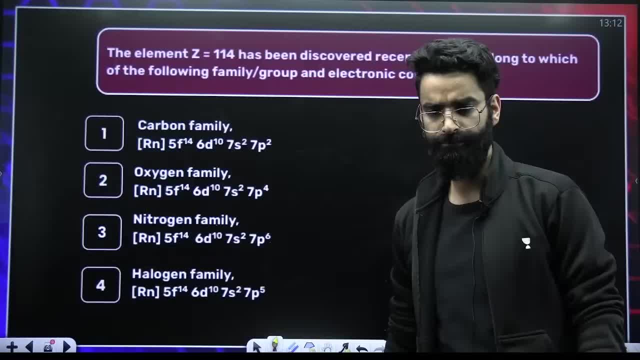 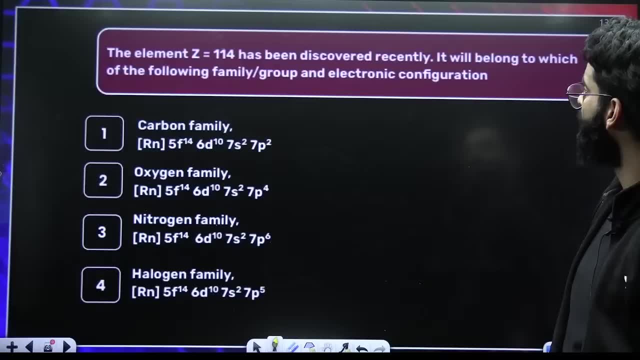 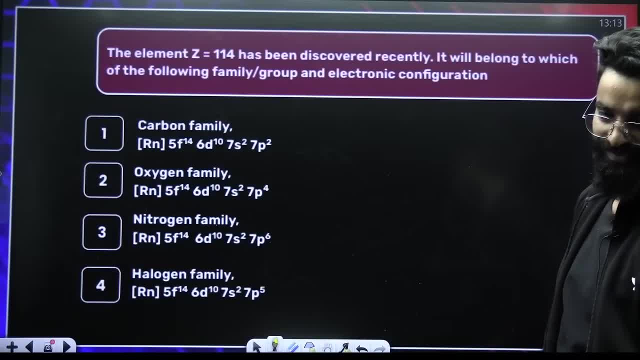 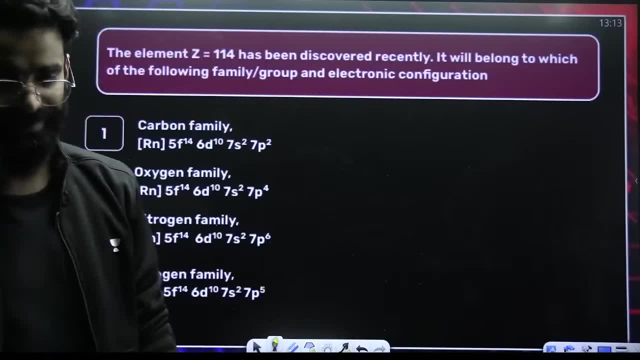 would like to join them, And this is an elite sort of class. utilise this class, And I will certainly cover some more conversations, more技ift methods next time. Guys, I am going to go ahead and fast-forward it. So: Z orthogonal unit, Kepler unit. All right, So that is where it happens, So vegetable. 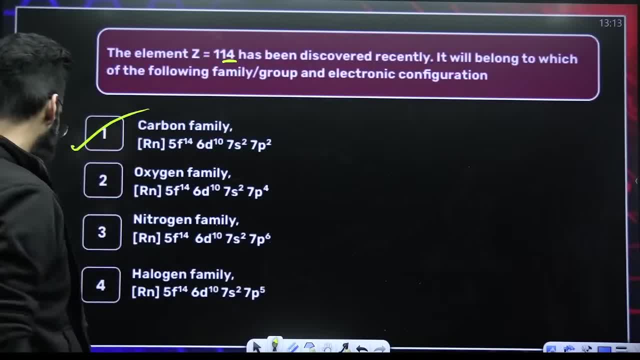 unit here has some side sayinclasses as others. The final has got sub ha Bilderして there. In this I would like to show that Ba Bagelung region starts off. Goodbye there. What does that mean? Yesterday we have seen this. 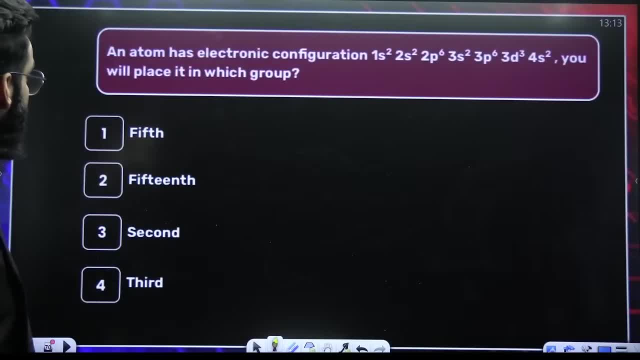 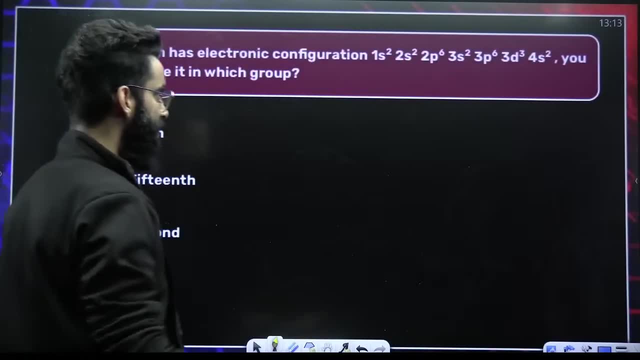 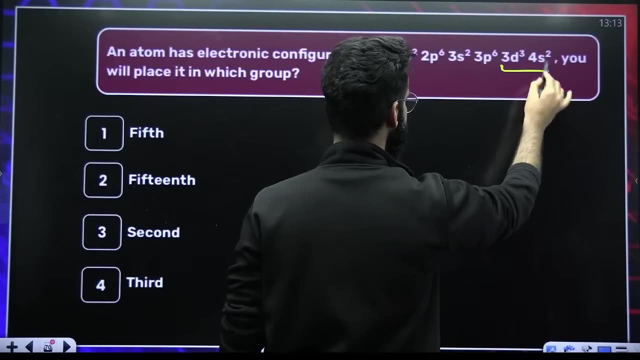 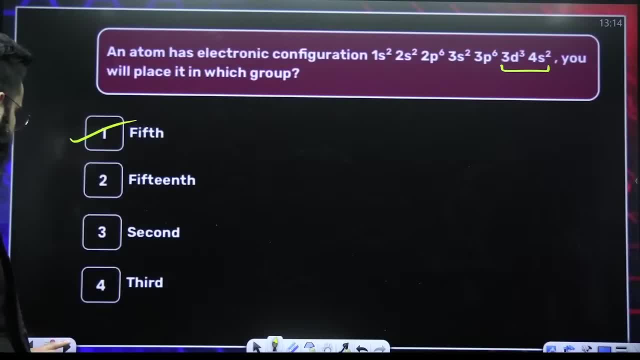 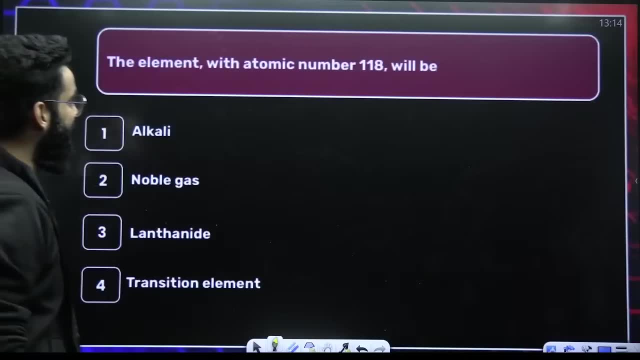 3 plus 2 is 5.. 3 plus 2 is 5.. Yes, 3 plus 2 is 5.. The element with atomic number 118, last, That is a noble gas, right, It comes in group 18.. It comes in group 18.. So 119 will again come in group 1.. 120 will come in group 2.. This question we already solved many a times. Iso-electronic species 1. Let me see if there are some new questions. 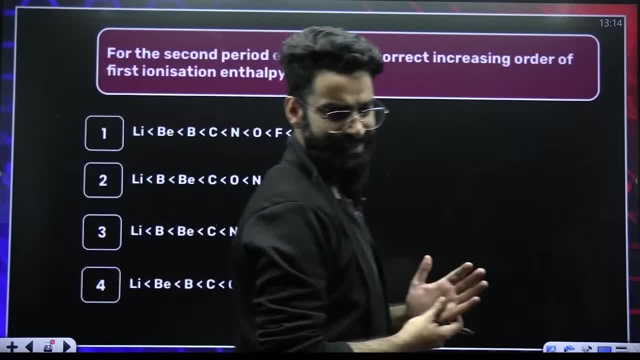 Okay, what do you think about this one? These are second period elements which are given to us. We have to arrange them on the basis of ionization, energy Ionization energy: Lithium, Beryllium, Boron, Carbon, Nitrogen, Oxygen, Fluorine, Neon. 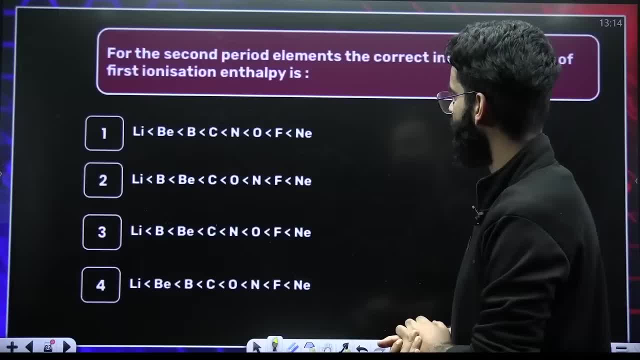 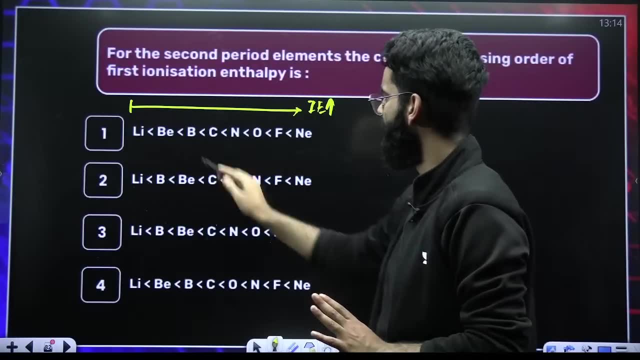 Right, This is the expected order. This is the expected order. Ionization energy moving from left to right increases, But here you have to interchange the positions, Boron. No, it's wait, Boron, you have to keep here. 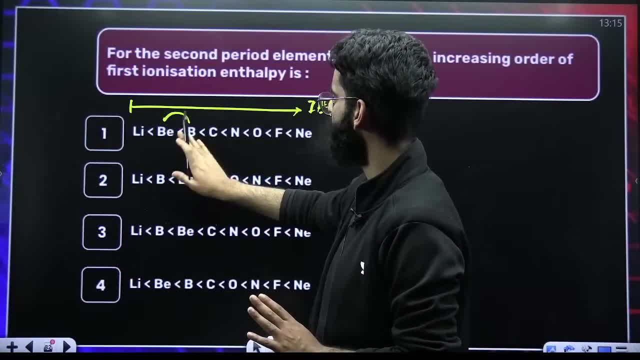 Beryllium you have to keep here, Similarly Nitrogen, you have to keep here. Beryllium, you have to keep here, Similarly Nitrogen, you have to keep here. Beryllium, you have to keep here. 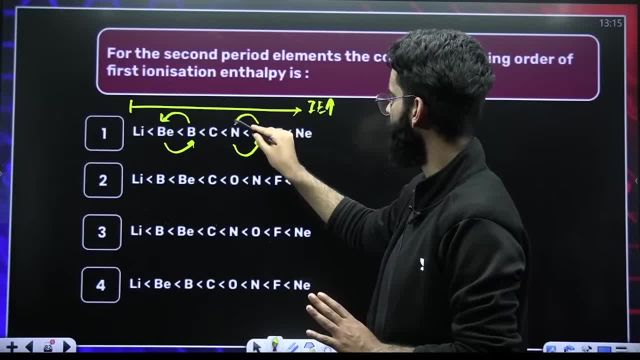 Similarly, Nitrogen, you have to keep here, Oxygen, you have to keep here. What is the logic? Logic you already know: Because of the half-filled configurations, Because of the half-filled configurations. So actual order will be what? 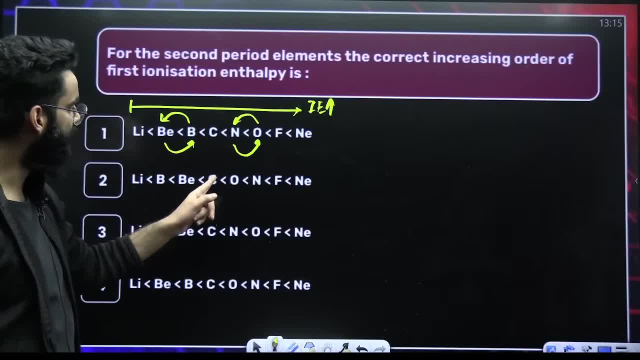 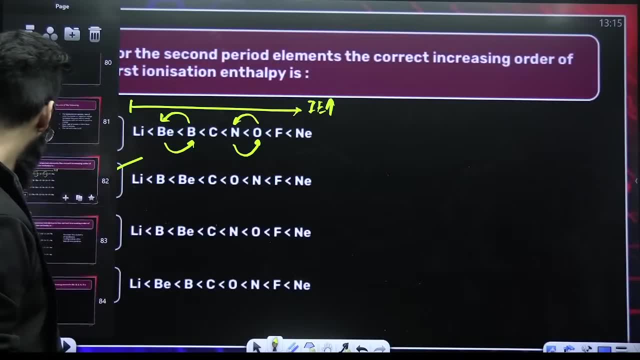 Actual order will be: Lithium, Boron, Beryllium, Carbon Oxygen, Nitrogen, Fluorine, Neon. This will be the actual order. This will be the actual order. Okay, This will be the actual order. 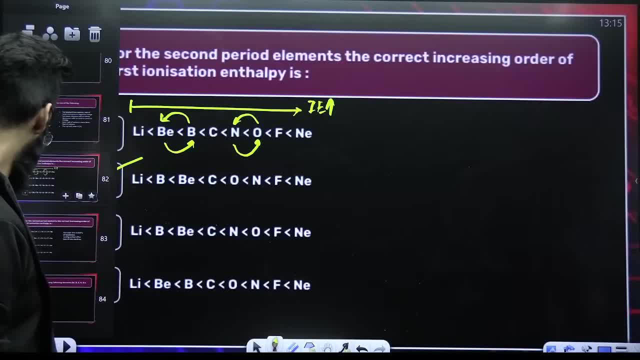 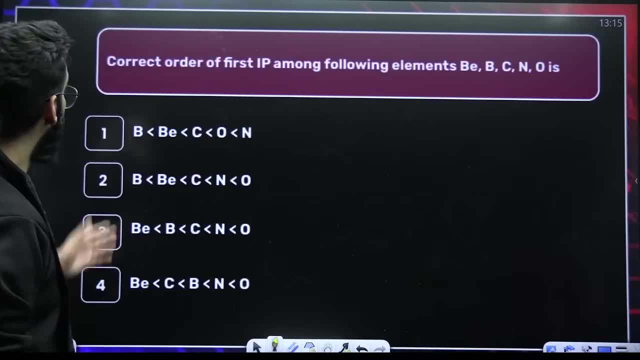 This will be the actual order, Correct order of first ionization potential of these. what do you think Done Which one- Nitrogen of course- will have maximum right? Half-filled configuration: That's the only option which says nitrogen has more. 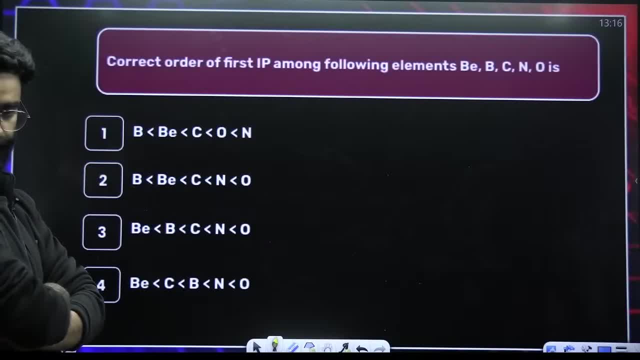 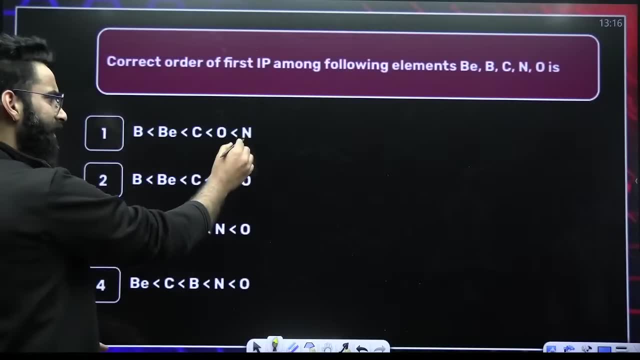 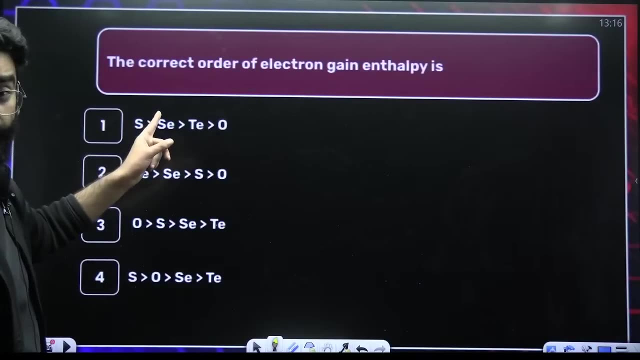 Electron gain. enthalpy order- op group 60,. nitrogen oxygen goes at the last. oxygen goes at the last. Guys, just give me a second. Nitrogen goes at the last. Oxygen goes at the last. Guys, just give me a second. 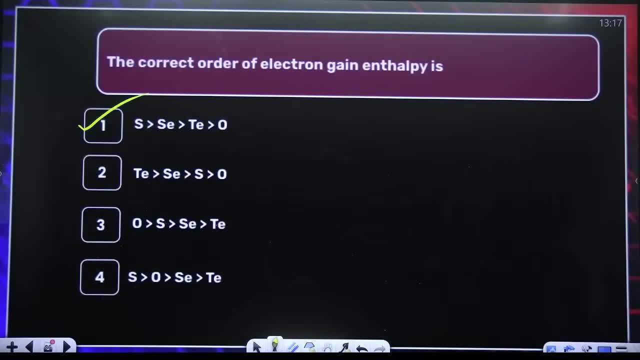 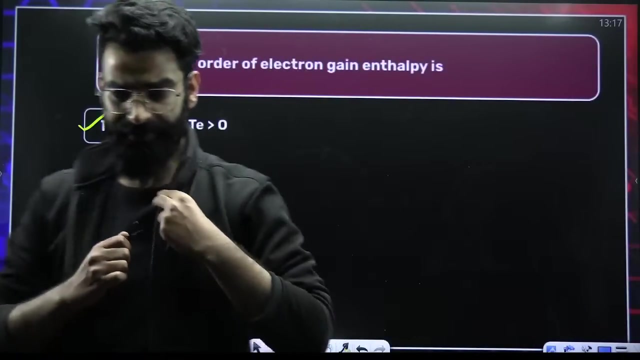 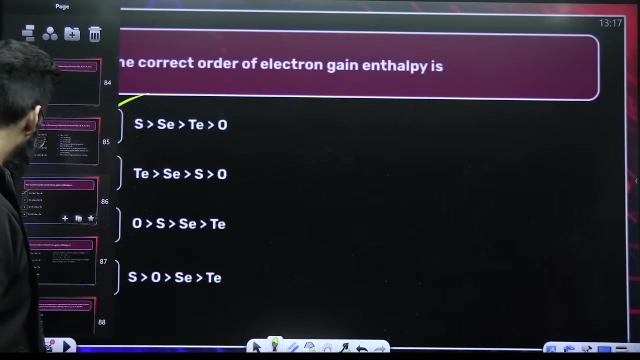 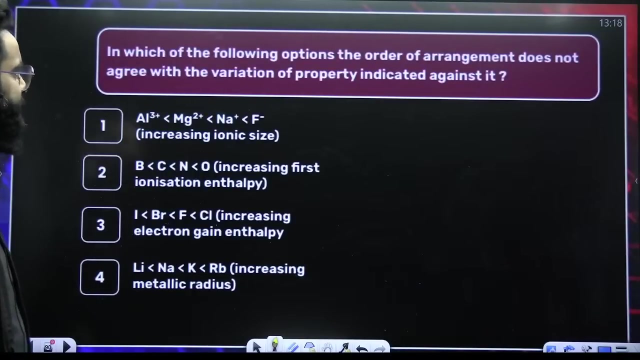 Oxygen goes at the last Oxygen goes at the last Oxygen. Okay, this is done. This is done. Look at this particular equation. in which of the following options the order of arrangement does not agree with the variation of property? with the variation of property indicated against. 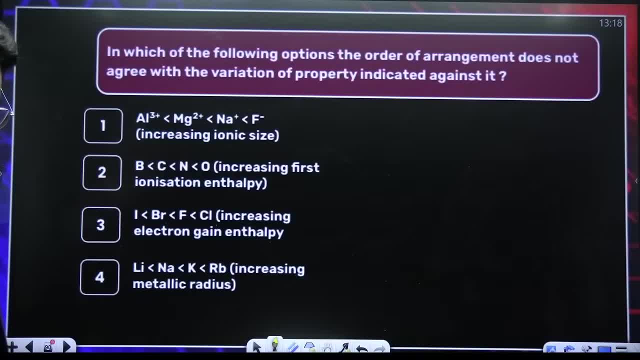 it Quick. is this electron gain enthalpy order? Is this ionization energy order? Does not, agree, Does not? What is the answer of this question? You know nitrogen has got more ionization energy. first ionization energy, then that. 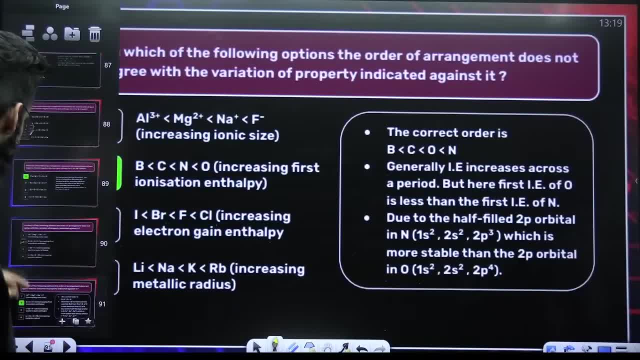 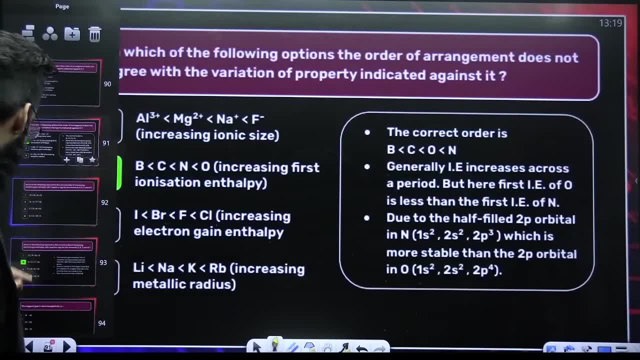 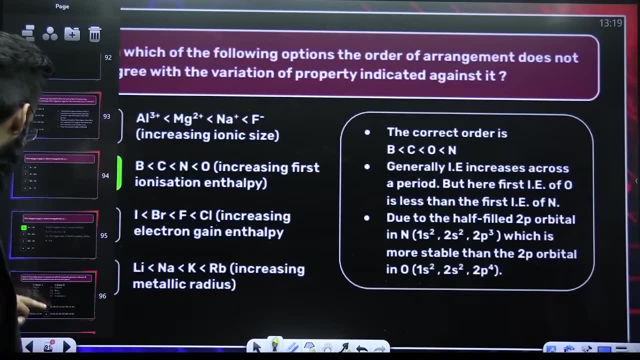 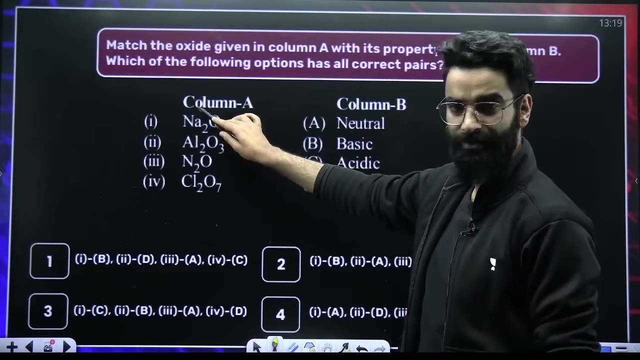 of oxygen. So this is wrong. This is wrongly matched. Rest: everything is correct. These are some oxides you have to check. This is a metal oxide group. first, Right Metal oxides. what do they do? They form basic oxide. 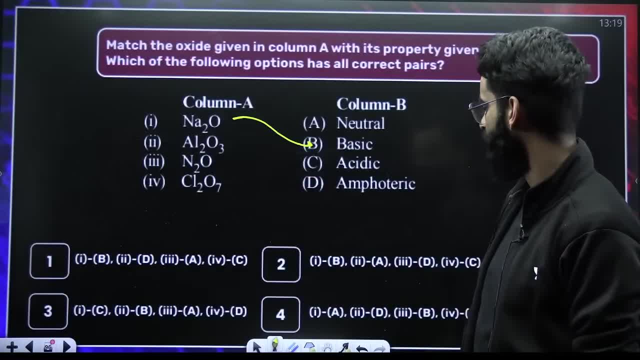 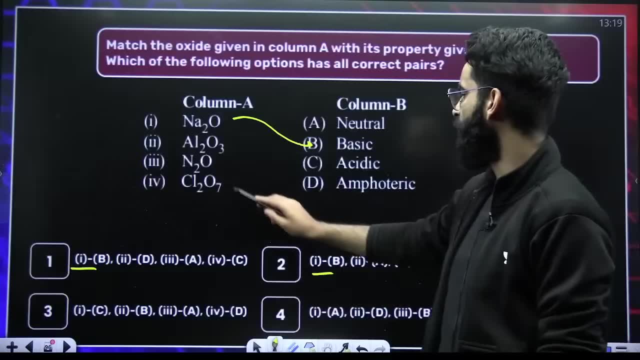 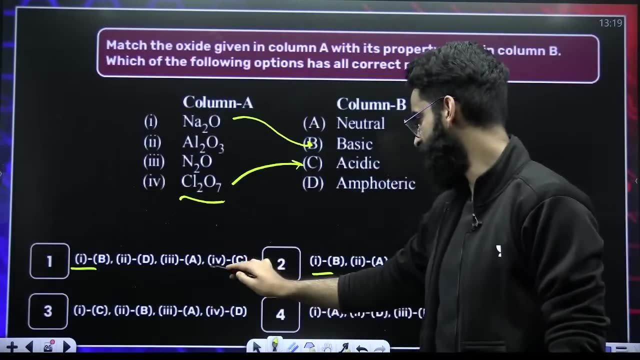 This is basic, Perfect. So 1, you are connecting with B, So it is option A or option 2.. Now Cl2O7, non-metallic oxide. it forms the acetic oxide. 4 with C, 4 with C, 4 with C.